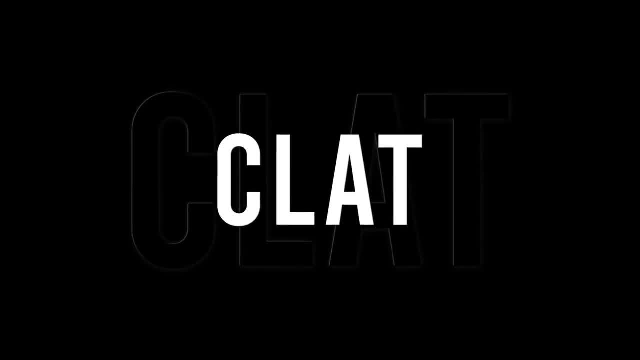 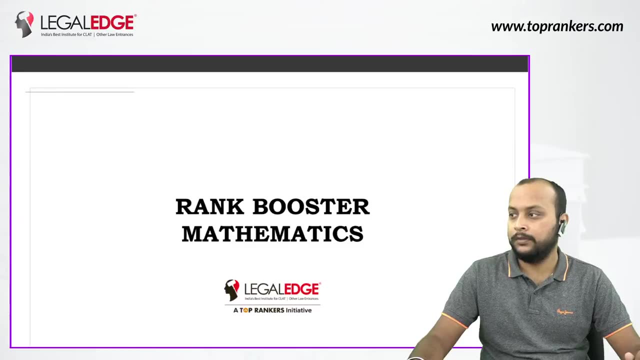 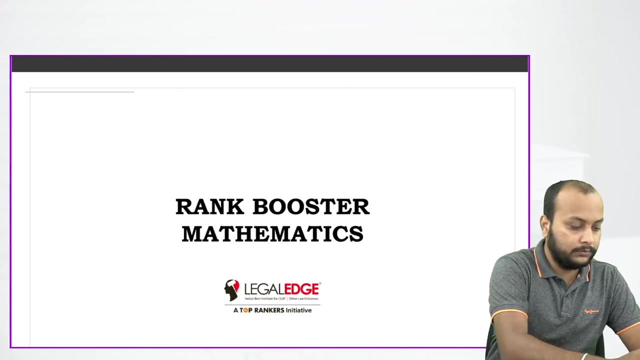 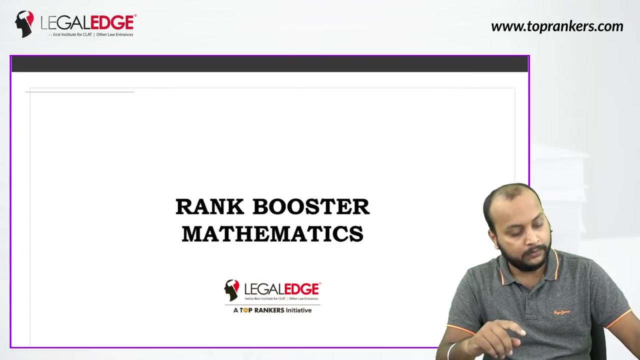 Very good afternoon to all of you. Am I perfectly audible? Am I perfectly audible? Am I perfectly audible? Can you tell me we are perfectly audible and visual? Then we'll start with the session. Okay, So Now, after CLAT, the next target is ELITE, right? 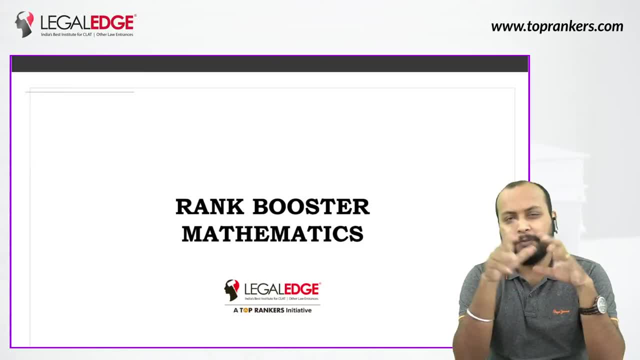 Ready for that. If I talk about the Mathematics section, according to the ELITE paper, there has been a pattern going on. Until now, the ELITE has not changed its pattern in the Mathematics section, or, if you say, overall, Overall. now we will discuss about all the subjects that your faculty will discuss with you. 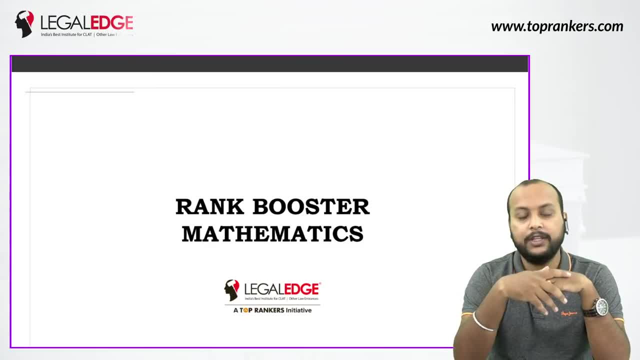 but in the Mathematics section their pattern has never changed. basically The patterns, the questions, the chapters in which they ask the normal questions. they ask the fixed questions right. Apart from that, there are variations in one or the other question. 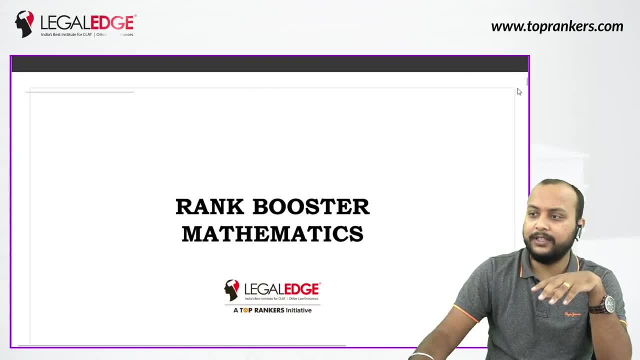 otherwise, their pattern is as it is going on. Whatever is their, The questions that have been asked previously or the patterns that the ELITE has followed, basically there has not been any change in them. They are as it is going on. 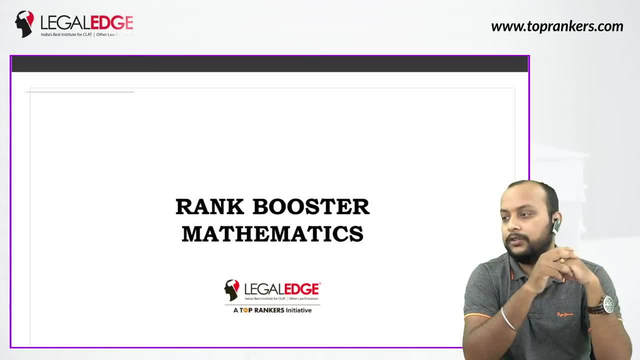 So, in the same pattern, we will attempt a number of questions today And We will attempt questions In between. if there is a requirement that a theory should be discussed with you, then it will be discussed, But mostly we will focus on the number of questions that will be practiced. 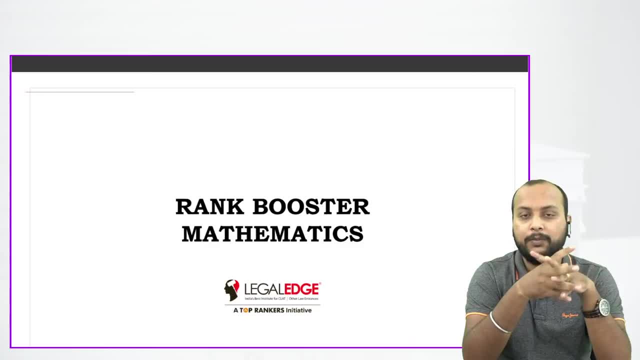 Because these questions- either the previous questions or the ones that have come in the ELITE, or the chances of them coming- I am saying this because these are some topics that are continuously being asked. We are going to solve the questions of those topics here. 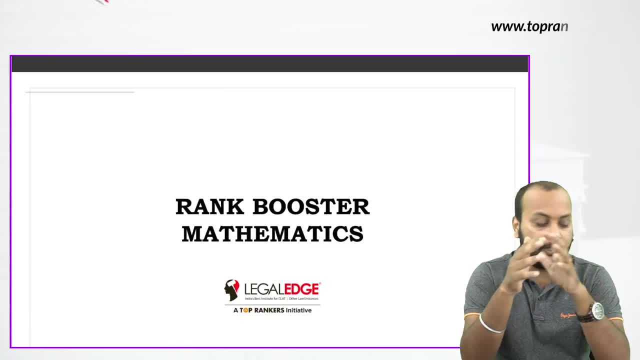 So If at some point in those topics it will seem that its concept and its theory should be discussed, then we will discuss its theory there as well, In the brief, without going into too much detail, without going into too much into its concept. 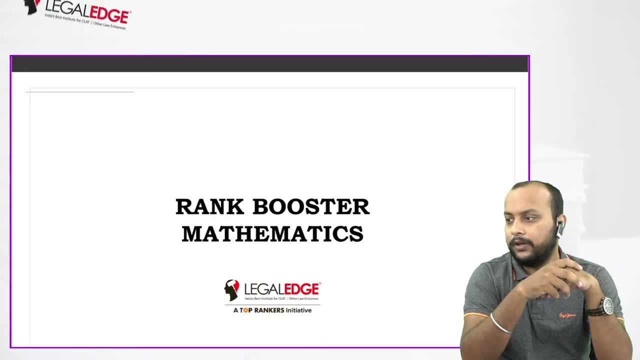 what we will do is we will take it as a brief introduction. Okay, Just give me one minute. 1.. Okay, A, B, C, D, D, D, D, D, C, D C. 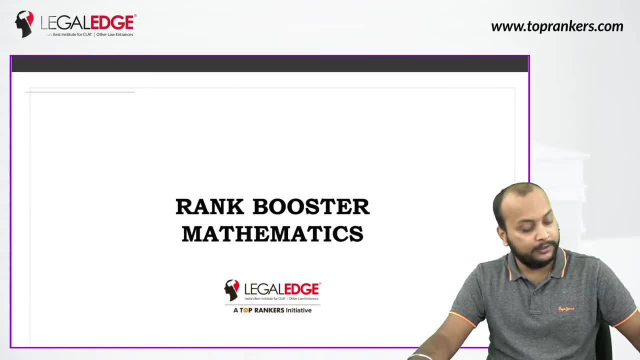 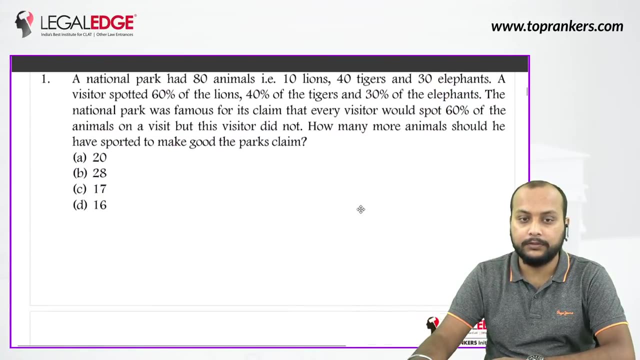 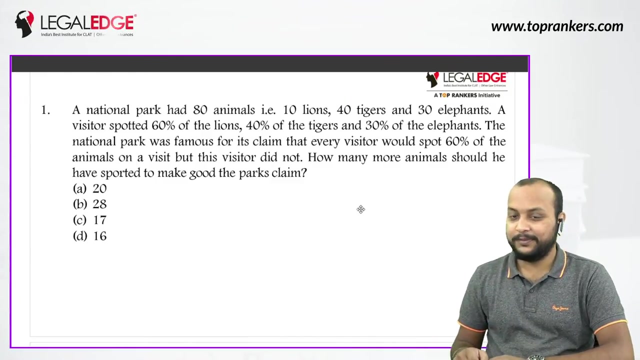 1., 2., 3., 4., 5., 6., 7., 8., 10., 11., 12.. The first question based on percentage Answer. meanwhile, let me tell you that the chapters are important, whose questions are asked repeatedly in the elite. 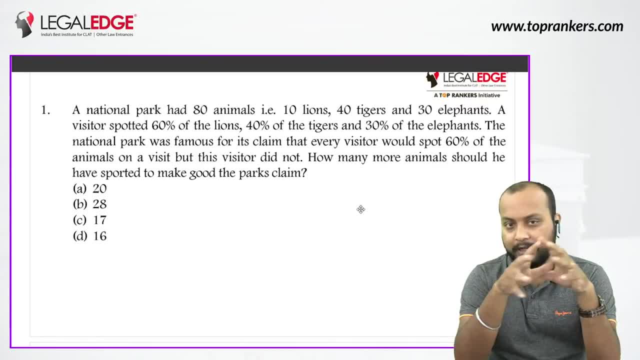 So let me tell you the names of those chapters. meanwhile you will solve these questions. The chapter is percentage. it has 8 questions: Profit and loss, Hand speed, distance, Time and walk, Race and proportions, Probability and PNC. Either probability or PNC. 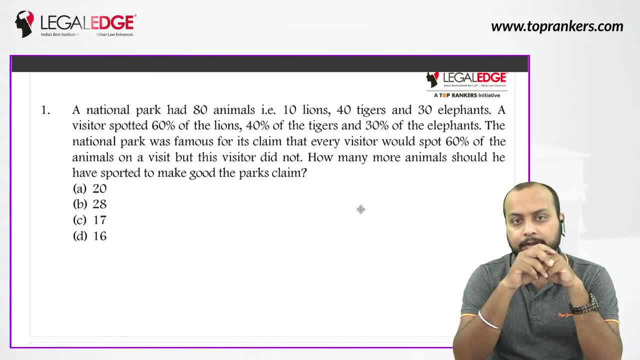 Sometimes we do two, but mostly one has to come And average Now in average. ask about arithmetic mean, progression or average. Both are the same thing. Arithmetic mean is called average And progression can also be applied to it. So arithmetic progression or arithmetic mean? a question is mostly asked from them. 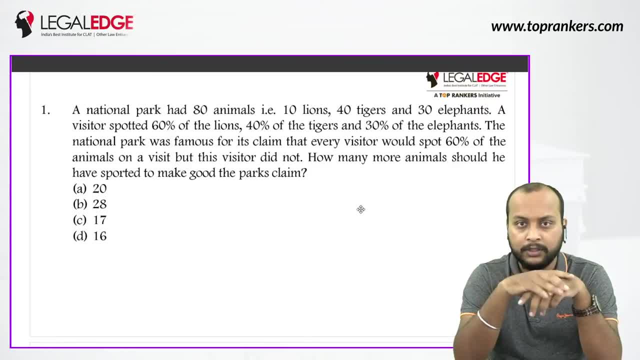 So these are the 6-7 chapters whose questions are asked, And don't forget to subscribe to our channel, Thank you. And also 8 questions of numbers, Which means just consider 8 questions are fixed from these chapters. The other two questions have various variations. 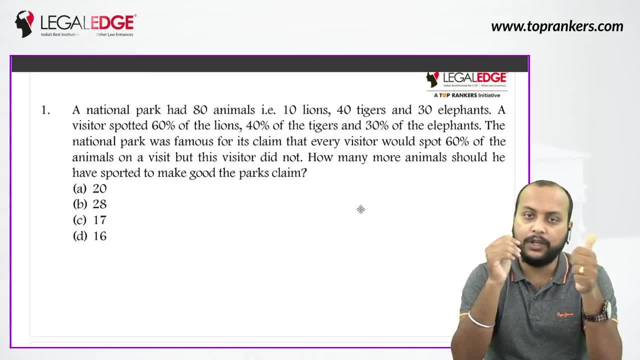 It also comes in a repetition that some topic has two chapters or one, Or some other chapter is introduced. Somebody has asked the questions from the partner of allegations, But mostly they are asked from them. So two answers have come, 17 and 17.. 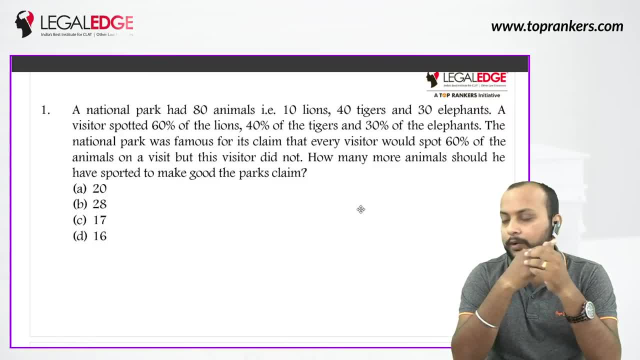 Two answers: 17.. The question is easy. level of difficulty will be taken to the difficult level. easy to moderate level. keep it 1 or 2,. max to max 2, but keep it 1, on average. there is only one question whose level of difficulty goes above the moderate level. 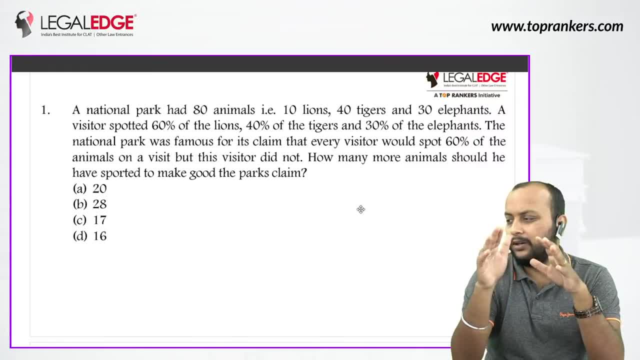 Otherwise, all the level of difficulty will be taken to the moderate or below moderate level. out of 10,, 8 to 9 questions on average level, moderate level or below moderate level. All the answers have come. mostly everyone has answered C, so C is the correct answer. 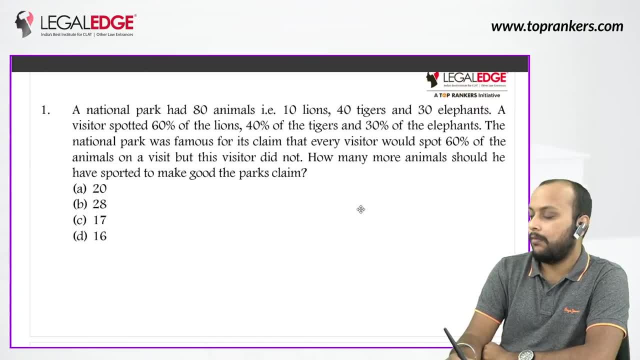 Let's discuss 80 animals and look at this line: Claim that every visitor's spot is 60% of the animals, 60% of the animals, so 80,. total number of animals is 80, and the spot is saying that at least 60% of the visitors will do it. 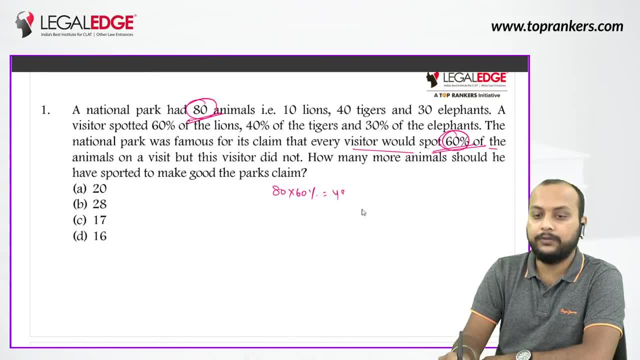 So first of all let's see: 80 is 60%, that is equal to 48.. How much is 60% of the animals? 48.. Now let's see how much is given 10 lions and how much did we see in 10 lions. 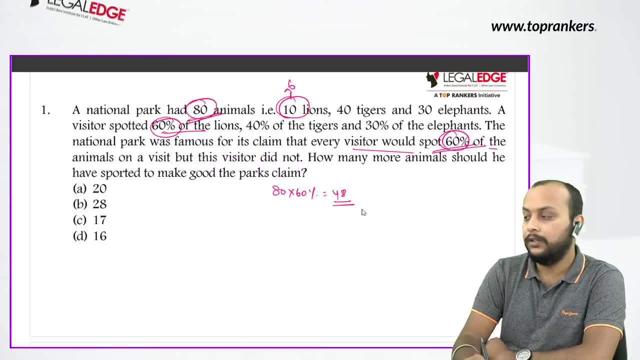 60% of the lions. So how many lions visited? 6.. 60% of the 10 lions: 40 tigers out of 40 tigers: 40%. So how much will be 40% of 40?? 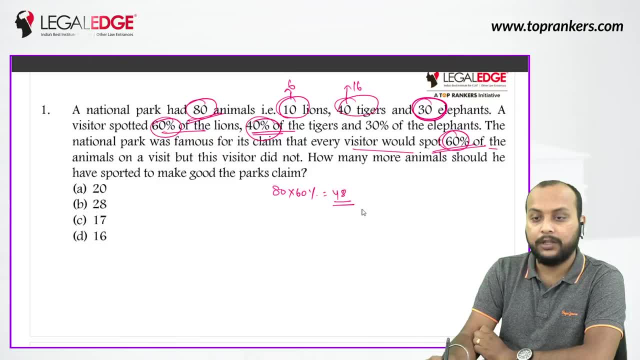 16. And 30 elephants, and how much did they visit in 30 elephants? 30%. So how much is 30% of 30? 9. So how much did they spot? 6 plus 16 plus 9.. 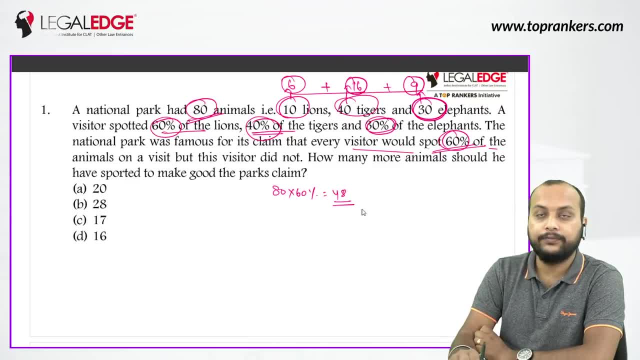 That is equal to How much? 31. 31. So how much did they spot? So 31 spots. How much did they do Out of 60% according to the claim 48. So how many more elements are required for the spot of the animals? 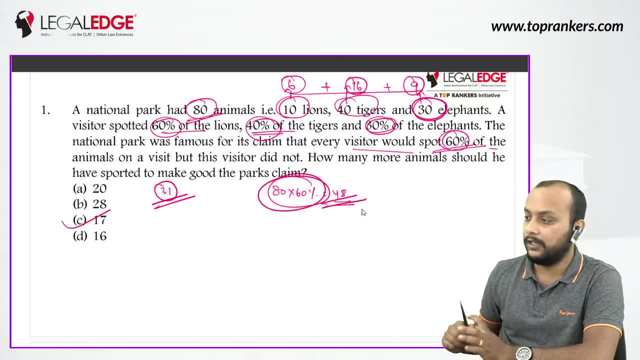 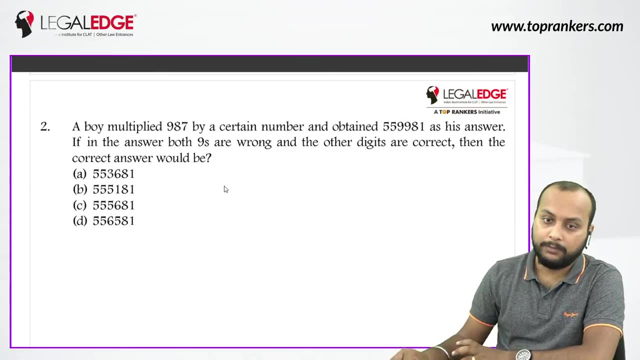 C 17.. So we just need to do data calculations here. Okay, Any problem, Let's move on Now. this is based on numbers: Y multiplied 987 plus 64? No, we haven't done that. We don't know the answer yet. 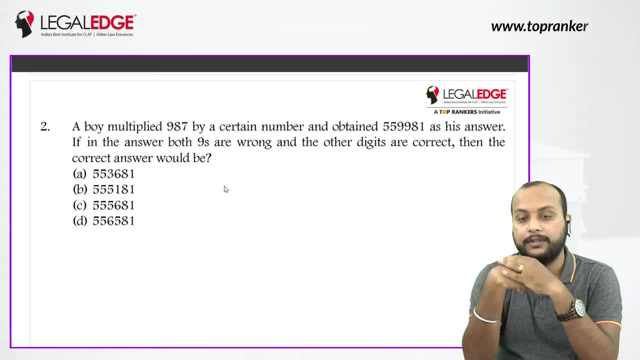 Let's try again: 4.. 987 by a certain number and obtained 559981 as his answer. If the answer- both 9s- are wrong and the other digits are correct, then the correct answer would be Chahawali. Thank you. 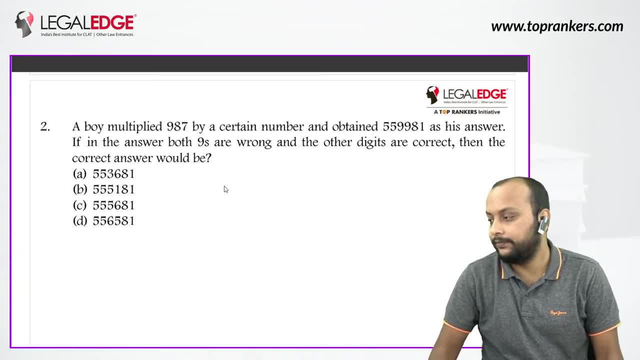 You can write it after the end of the video. It will be live now, right? Allahi's answer is 55181. Is 55181 correct? It is wrong. You have to solve it. Don't cheat in ABCD. Don't cheat in ABCD. 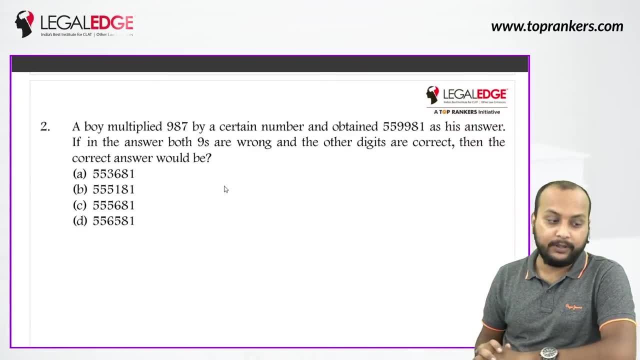 Ananya has answered A 5553681. Did you understand the question? The question is that we have multiplied a certain number by 987.. We have multiplied it by 987.. Okay, We have multiplied 987 by a certain number. So what is the result? 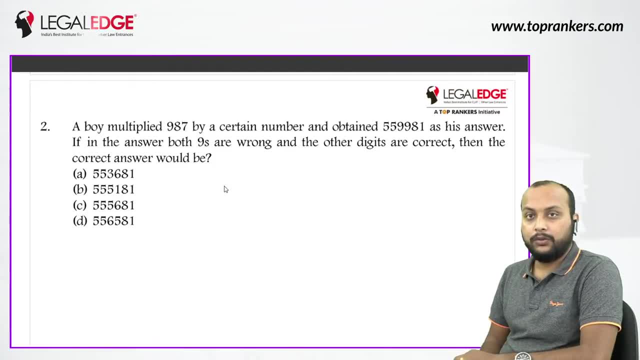 559981. So the result is wrong. The two 9s are wrong. He has written the wrong result. That means he has multiplied it wrong. So what will be the correct multiplication? That is what we have to ask. Let us look at this ID. 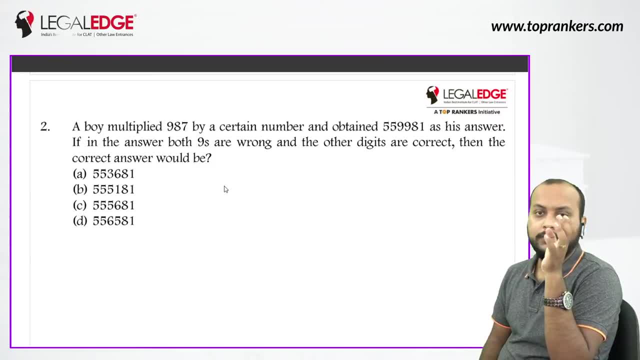 You can write your answer now. Okay, here you go. Need of number is Team 5: Again, change the number. Yeah, you will change the number Because it is appropriate, right? Yes, Those are wrong answers. That is very wrong. 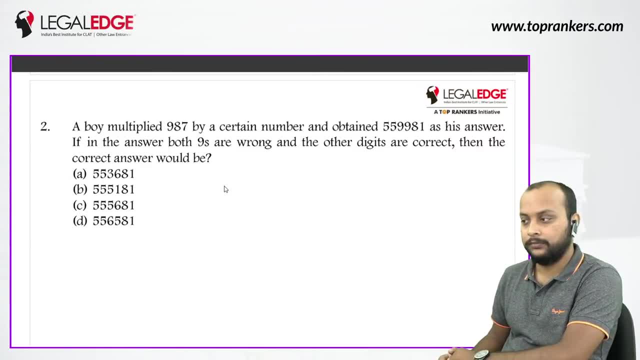 So we have multiplied by 9 in this 2.. Yes, As I discussed, C is the correct answer. yes, C is the correct answer. I tell you you try it still. yes, C is the correct answer. how to make it see that there is a question. 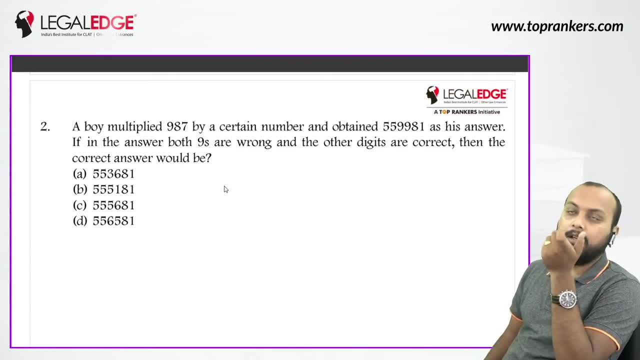 here, factorization is a sub-topic- in numbers, prime factorization. we will make it here and that is the easiest method to solve such questions. what is prime factorization? any composite number. divide it in prime numbers. that is prime factorization you must have. 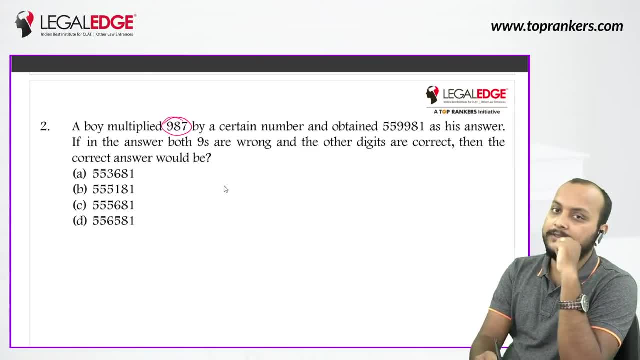 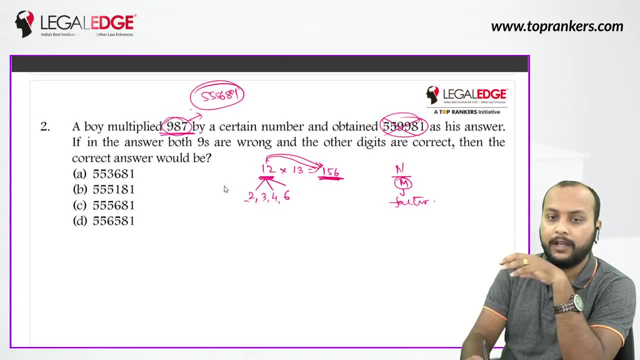 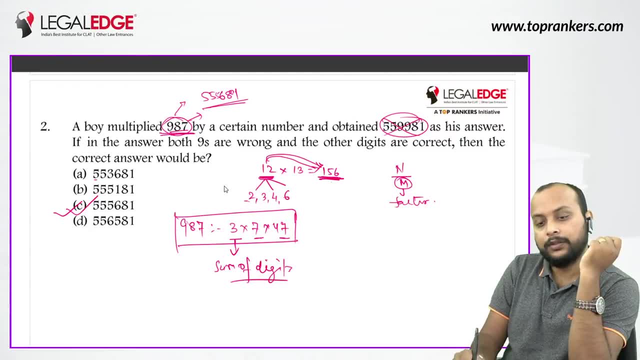 sum of digits: 5 plus 5 is 10,, 10 plus 3 is 13,, 6 is 19 and 8 is 27,. 28 is 28. is 28 divided by 3?? No, this is also not the answer. 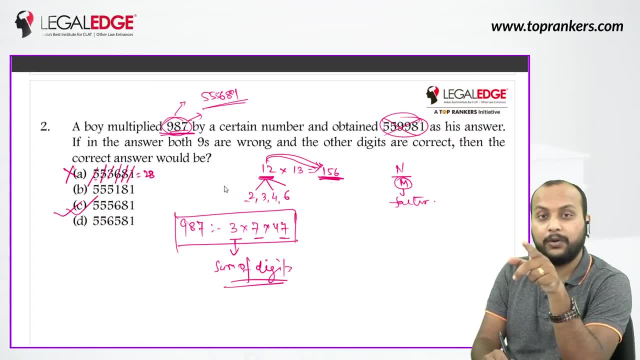 this is not the multiple of 987,. if it is the multiple of 987, then it is also of 3,. if it is the multiple of 12,, then it is also of 3, it is also of 2,, it is also of 4, and it is also of 6,. they also have their factors. 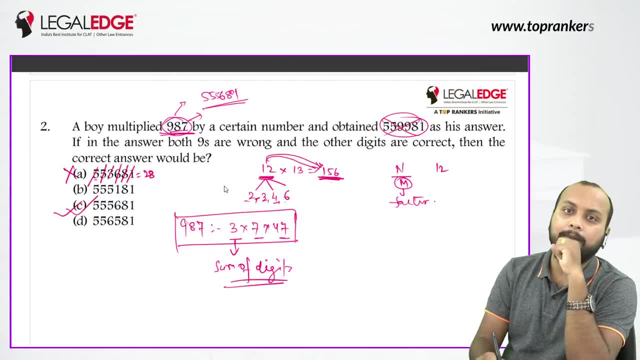 if it is not the multiple of 3,, then it is not the multiple of 987. the second one is 15, 15 plus 1 is 16,. 21 is 25. this is also not the same. similarly, if you see the third one. 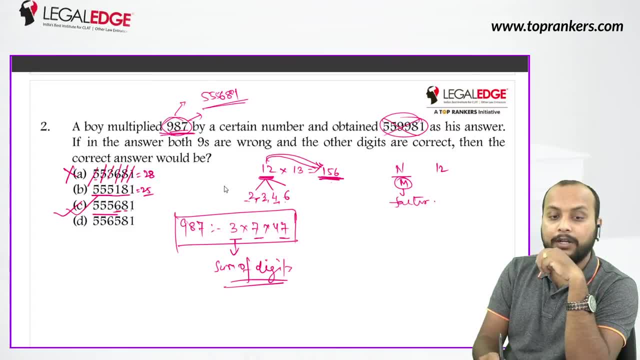 15 plus 6 is 21,. 21 is 29,. 30. this is the sum of 30,. this is the multiple of 3,. let's check the last one before going from 7,. if the last one is not the multiple of 3,, then this will be my answer. 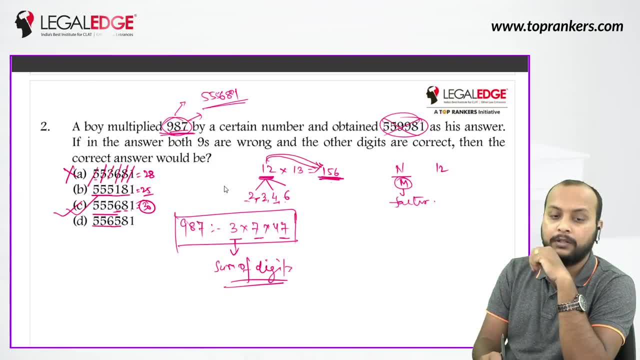 10,, 16,, 21, 28, 29. no, this is also the sum of 30,. this is also the sum of 30. so both these numbers, C and D, both are the multiples of 3. now what will you check next? 7, so let's keep C. 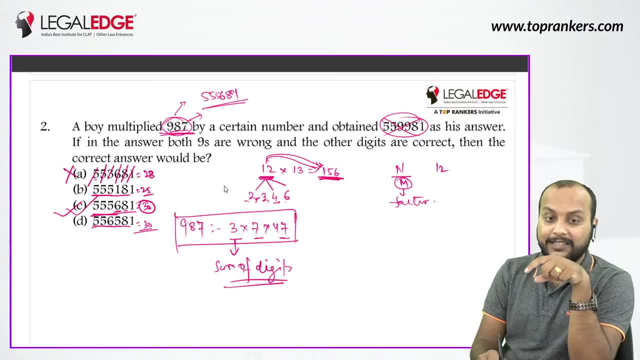 now you check 7. with whom? with D you will check 7 with D. we have made triplets. I have told you the method. it is a very simple method. we have made triplets, we have minused it, so it is 27. 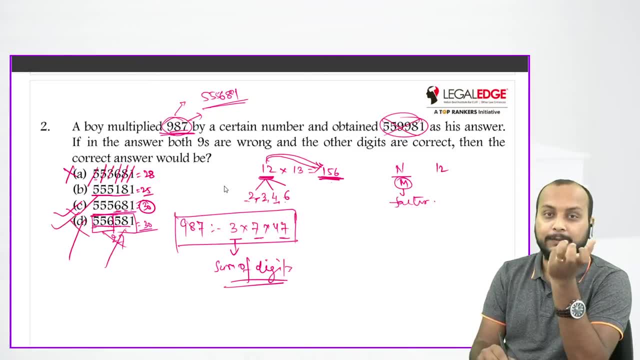 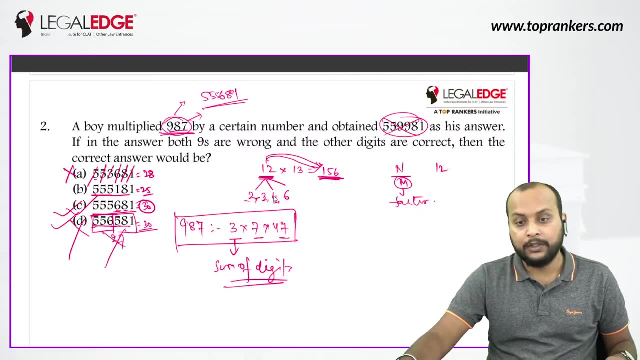 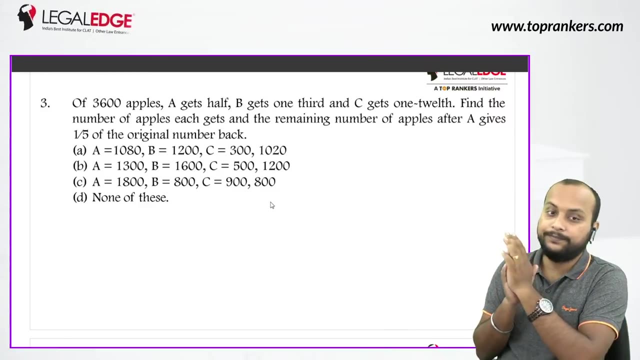 so what is the answer? C? C is the correct answer. now move to the next one. so any number, if it is divided, then it will also be divided by its factor. it was just a small concept. move to the third one. this is a general equation based question. 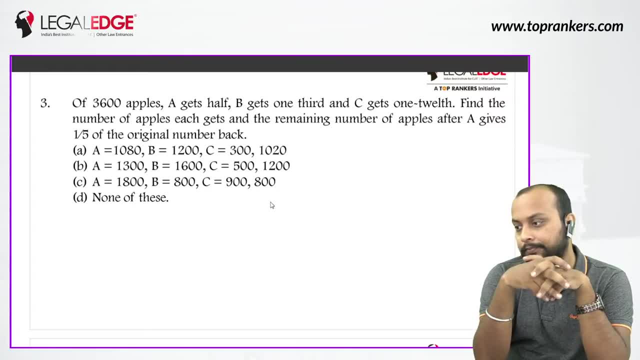 1,2,3, 0,2,3, 3,4,5, 3,3,4, 4,4,5, 4,4,7, 8,8,9, 7,8,9, 0,11,9. 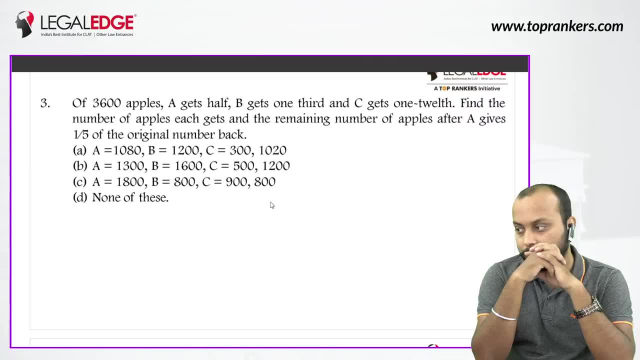 0,12,12, 13,36, 4,12,13, 2,4,5, 3,49,2. you and now these C and D- both answers are coming- make it it looks like, if you solve it, it will come easily. 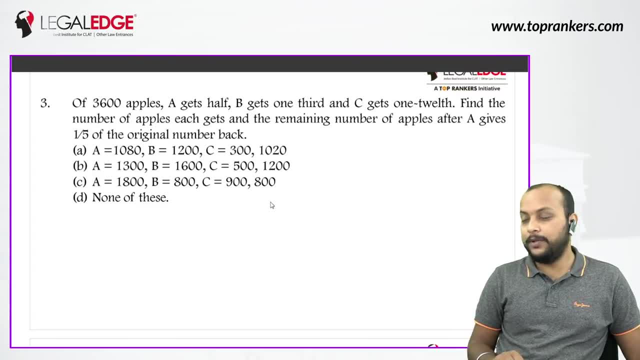 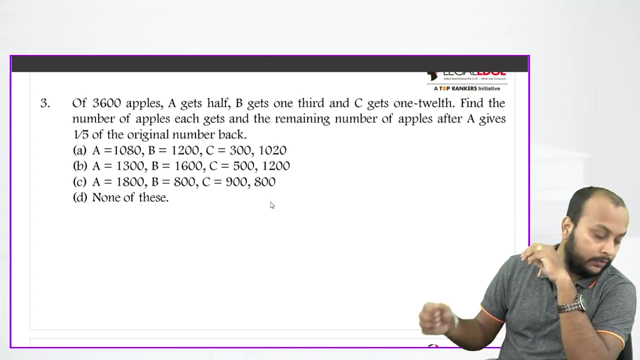 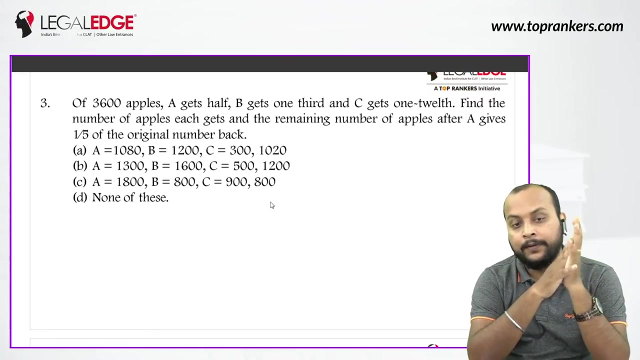 that's why mostly I in classes, in sessions, I remove options. you guys start cheating. what will happen? I have 20, sure? confirm the C and D. both answers are coming. a isn also available. wow, out of 3600 apples, a gets half. now how easy it is. 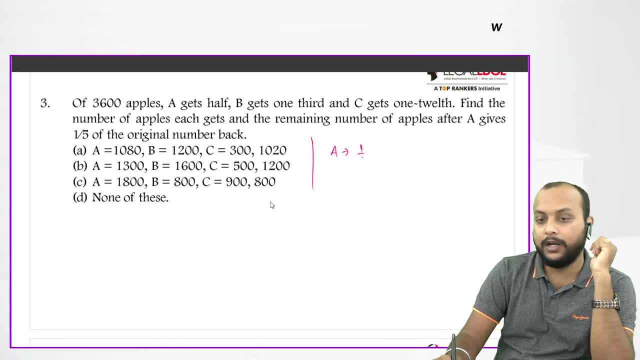 a gets half, so a gets half of 3600. that is equal to 1800. so option a and b are cancelled out because a has the same value: 1, 0, 8, 0 and 1: 3 double 0. so a and b are cancelled out. 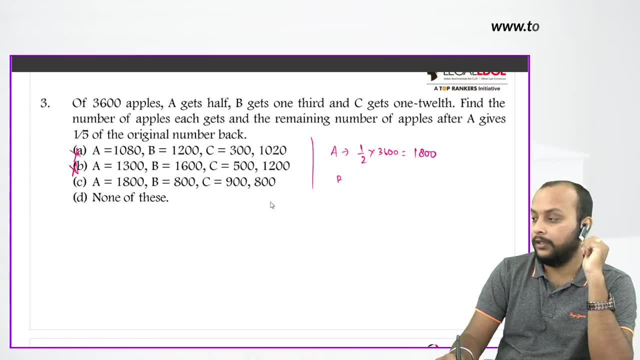 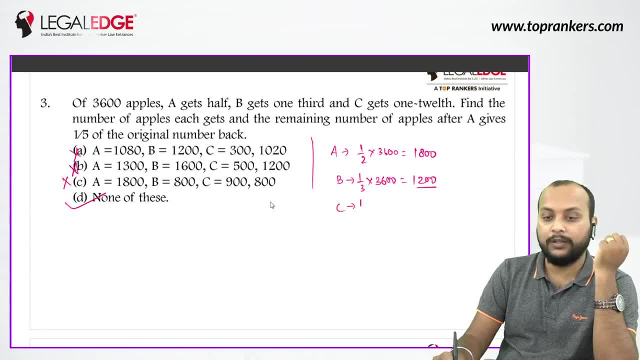 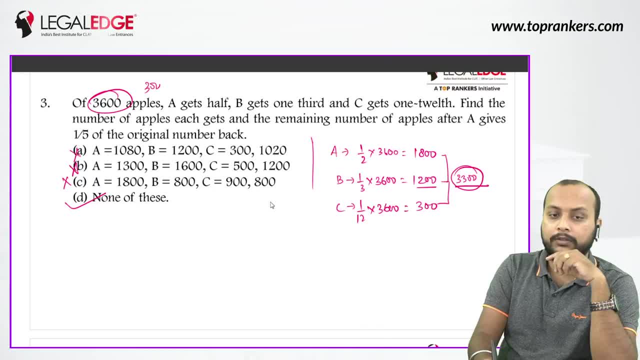 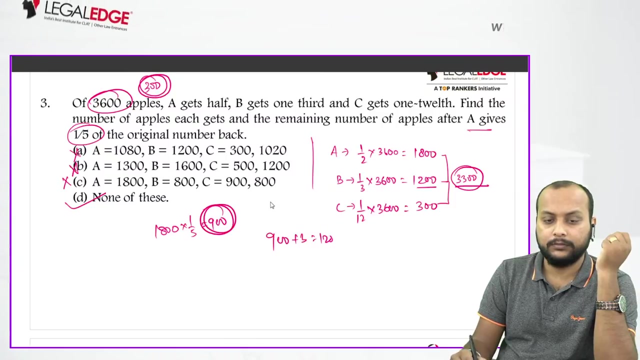 so how much is left? 3600, 300. after that, a gives 15, so a gives 135, so a got 1800 and it gives 15 and 900. So the remaining amount is 900 plus 300, that is equal to 360, so the remaining amount will be added to this. 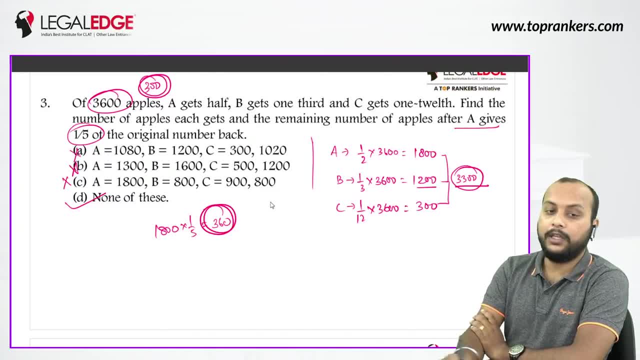 So the remaining amount is 100 plus 300, that is equal to 120.. So the remaining amount is 120 plus 300, that is equal to 1020.. But we will reach here only when our options match. 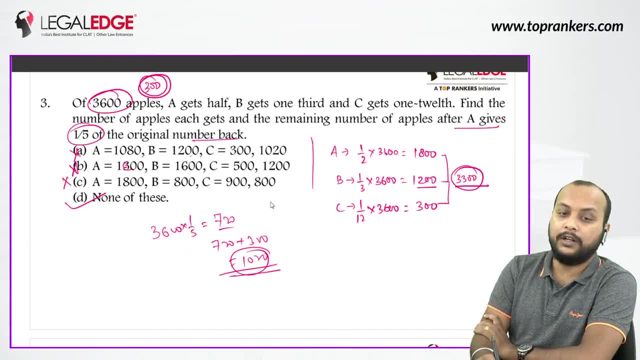 If the options are given like this, then we will check what will be the next step. Right, But we will not check here now. 3600 apples: A gets half, B gets one-third, C gets one-twelfth. Find the number of apples each gets. 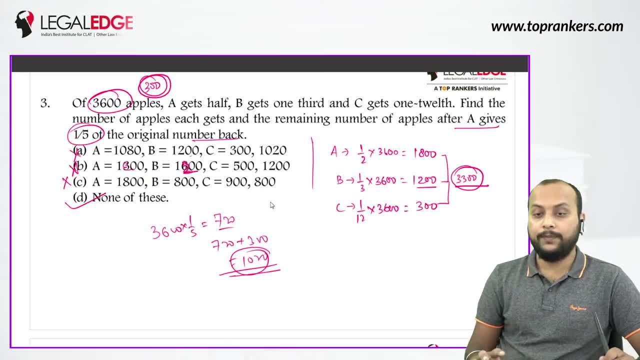 And the remaining number of apples after A gives the original number of back Right. So we have discussed about how much we got earlier. So the A option that you are talking about will not be correct, Because, first of all, this is the matter. 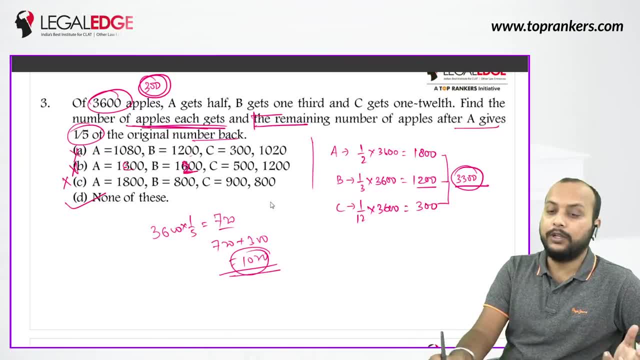 First of all, what did we say? How much did everyone get? So how much did everyone get? He got 18.. He got 12.. He got 3.. Now, how much is left? We have discussed about that. that A has returned. 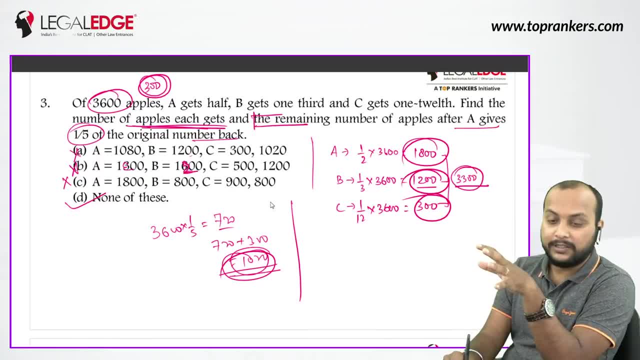 So this is the remaining part. If we say that, after returning back, how much does he have? Then we say that A has 1080.. B has 1200.. C has 300. And the remaining amount is 1020.. 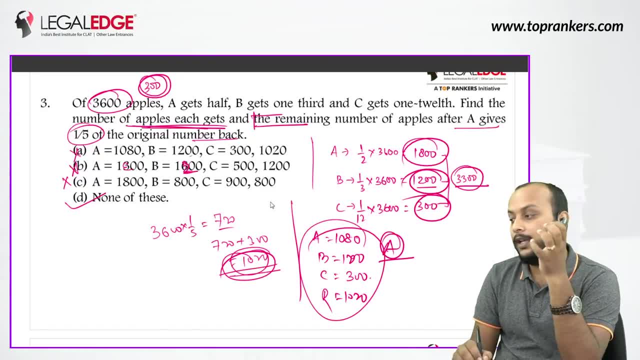 Then what is the option A, After saving the remaining? After saving the remaining, what is left after A returns? Then he asks you. So your answer would be A, Because A has 1800.. He has returned 1800.. 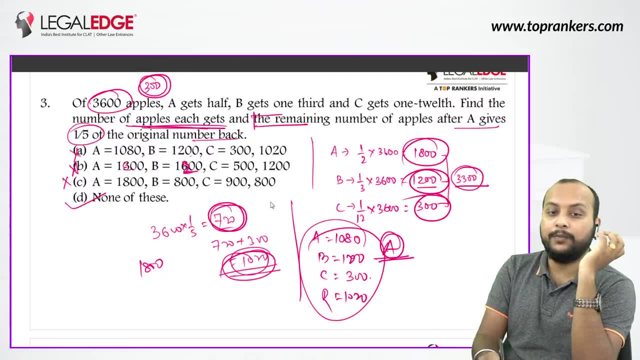 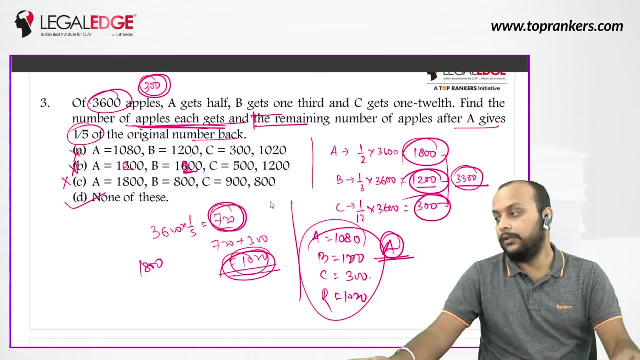 He has returned 1720.. But in the starting the number of apples each gets How much did he give first? So He asks you that, Okay, Let's go. Now let's go to the question number fourth. 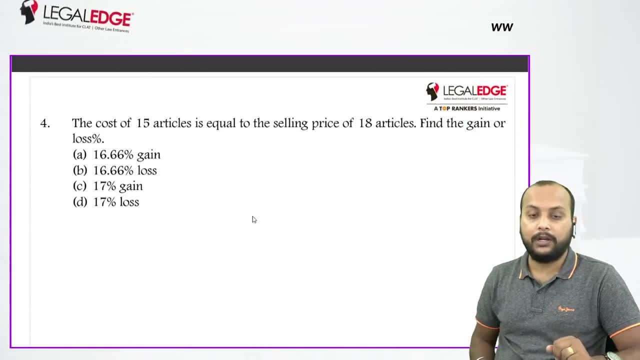 Based on profit and loss. Nishant, how many questions we discussed today, Let's see, Out of 35, 30. Around More than that, Let's see. It depends on your speed. As soon as you solve the question, you will move forward with the questions. 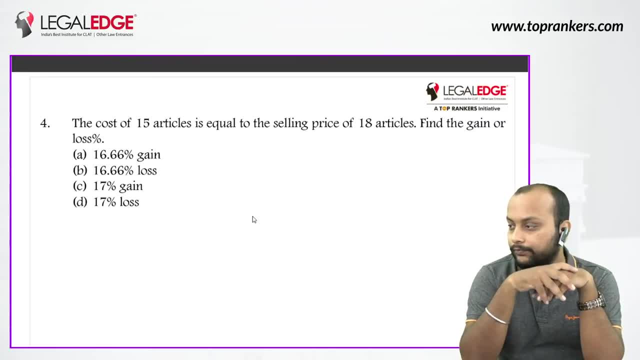 Okay, So let's see How many questions we discussed today. Let's see Out of 35,, 30. Around, More than that Around. You say word passing. The answer is: two döifie cost of 15 article is equal to the selling price of 18 articles. find the gain or loss. 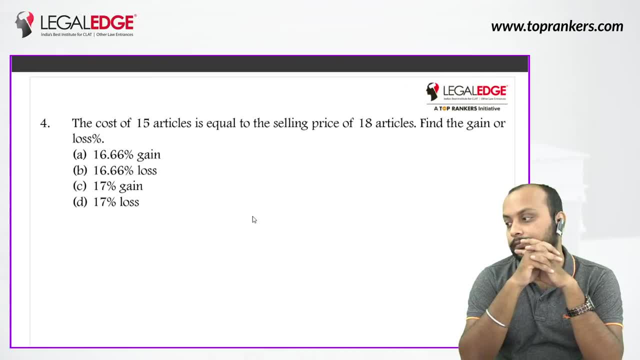 per site a and B. do on society that a and B. let's see that love. but right is 17 for 16.66. you have to gain over a 16.66. other loss of a liquid: 17 many. but are you not a or b? 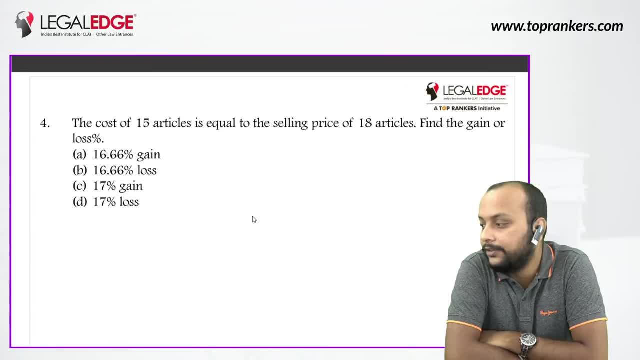 the answers. very good, there they can or get the answer. then let's see you again. a and b try to tell you offline paper mode. offline paper mode allowed, allowed headache okay, standing speaking and P it. he excited but didn't do west. It takes a lot of time. 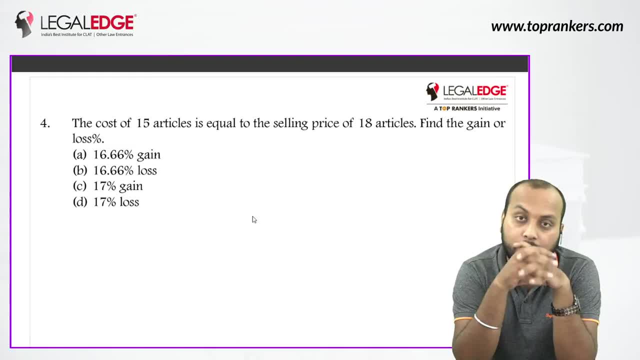 This is why I am telling you this. I am telling you this before the elite, Most of the people I talked to in the client's web host. they were complaining that I wasted 10 minutes. I lost 10 minutes in this. I got less time. 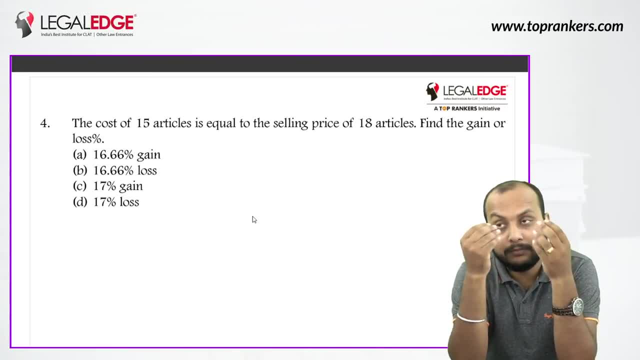 Pressure increased Or I couldn't attempt that section, Couldn't attempt anything, Okay, So to avoid this, keep your mind-maker from the beginning. I told you this earlier. This happens in offline paper mode. In online paper mode you don't fill OMR. 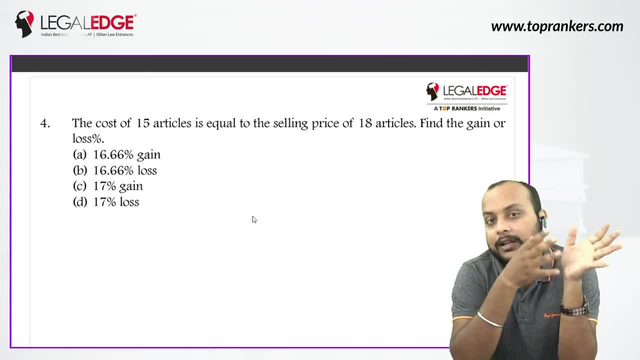 You keep doing 7 next, 7 next, 7 next. So time is saved there. But which is the different form of online? Offline is different. This is the form of offline Here in filling OMR in signature: disturbance. 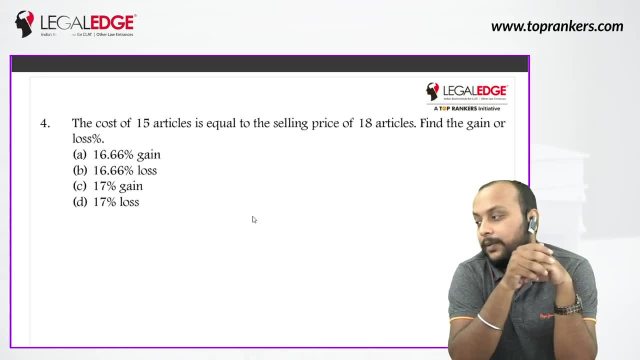 time is consumed And we pressurize you to waste paper, So this will not happen. Okay, Next, what will be the answer to this question? The correct answer for this question is B 16.66% loss. Cost price of 15 articles is: 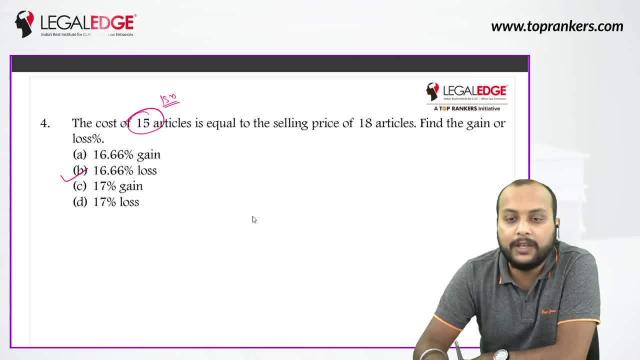 Rs 15.. Okay, And what is that Selling price of 18.. So what will be the cost price of 18 articles? Suppose the price of 1 article is Rs 1.. So the cost price of 18 articles is: Rs 18.. Now what will be the cost price of 15 articles, of 18 articles? See 18 articles and 15 articles. Both are cost price. The cost price of 15 articles is the selling price of 18 articles. 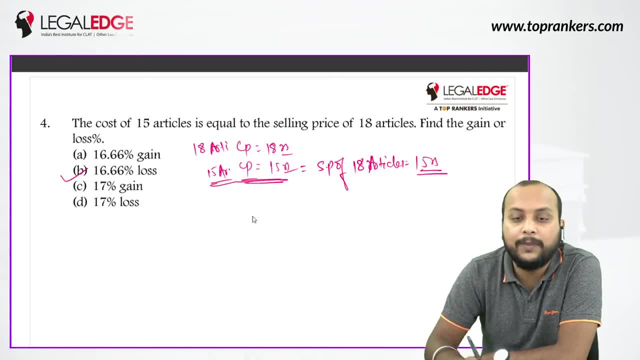 So what will be the cost price of 18 articles? Rs 15.. So the cost price of 18 articles is Rs 15.. Sorry, the selling price of 18 articles is Rs 15.. Cost price is Rs 18.. 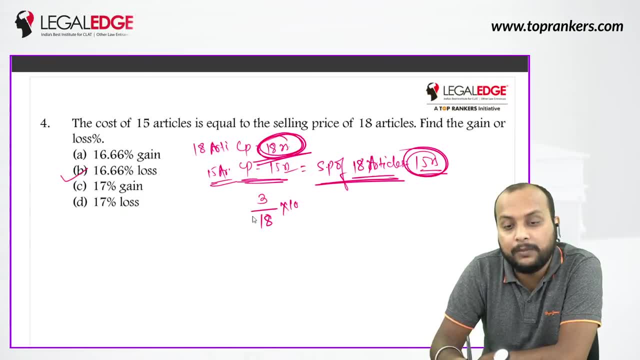 cost price is Rs 18 multi by 100.. Don't solve here, This is 1 by 6.. Sometimes they solve here only 1 by 6 is 16 points. 16 points and 16% loss- Very good. 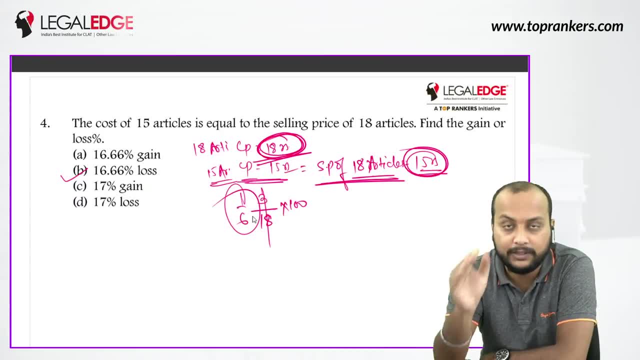 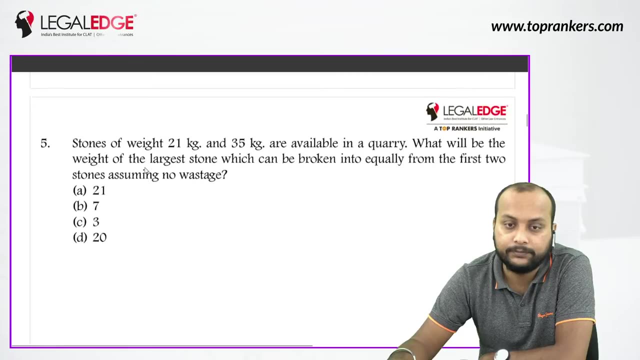 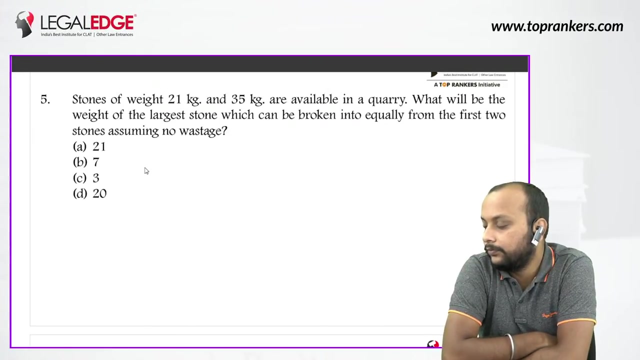 The answer was 16 points and 16% loss. Right, If you have also played the game, then you will know the basis of it. Okay, Next question is number. Thank you, Thank you, Thank you. Which topic application is it? 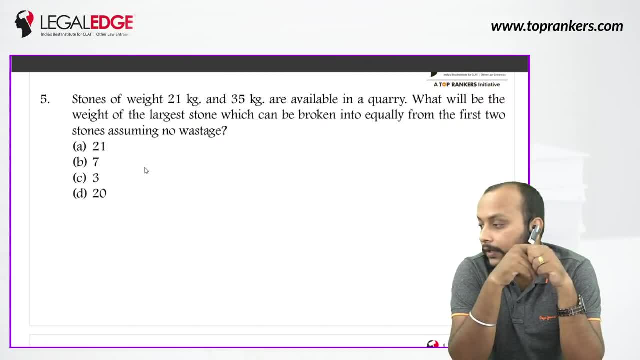 This question is belongs to HCF and LCM. HCF and LCM. This is the basic problem of HCF and LCM. It is said that these are 21 kg and 35 kg stones. We have to break them. Broke it into equally. 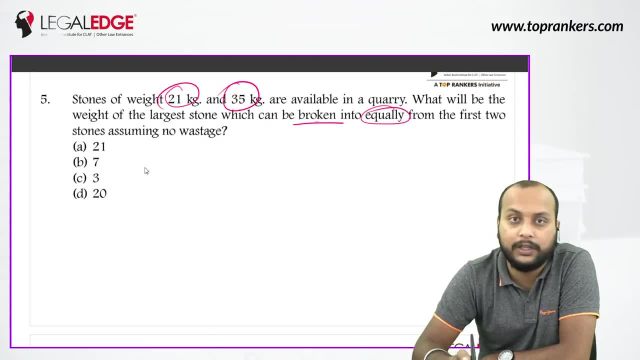 Okay, From the first two stones, And there should be no wastage When you break these two stones. it means that in this, what is the largest stone? How much will it be? It should be equal And there should be no wastage in it. 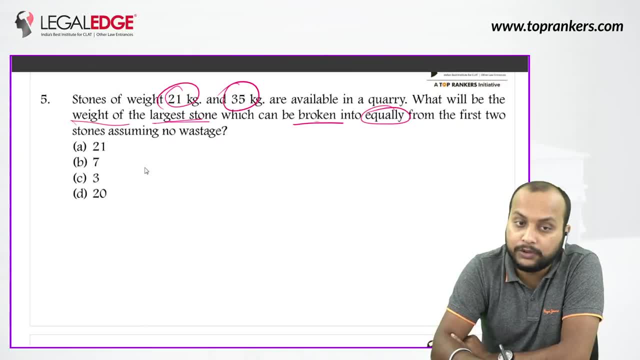 Sometimes I have asked you here that weight. Sometimes I ask the number of stones. Number of stones, Sometimes I ask the number of stones, How many will be Of equal weight? I will tell you both in the same question, What you have to do. 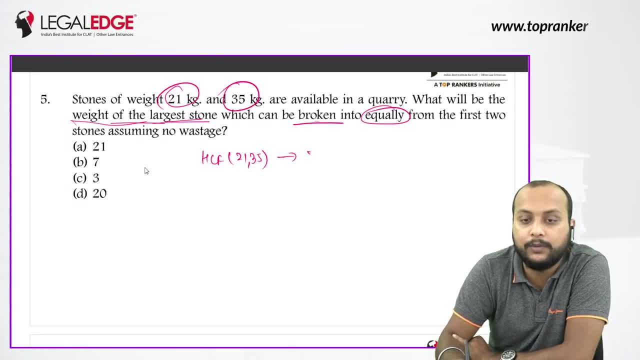 see: take out HCF of it, 21 and 35. HCF of this will be 7.. Okay, So if we break stones of 77 kg, then how many stones will I have of 21 kg? 3 stones. 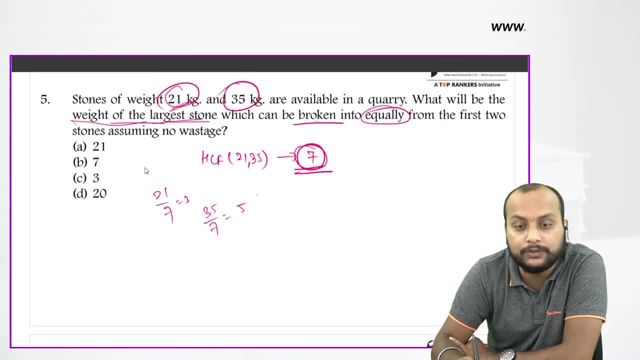 And how many stones will I have? of 35 kg, 5 stones. So how many stones will I have in total? 8.. Okay, There will be 8 stones Whose weight will be 7 kg. All of them will be equally weighted. 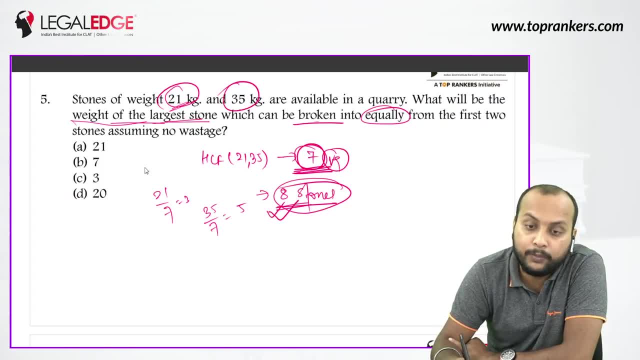 And how many stones will be in total. So sometimes it will ask you the number of stones, sometimes it will ask you the weight of the stones. So what will be your answer? accordingly, If you have been asked the weight, then 7 kg. 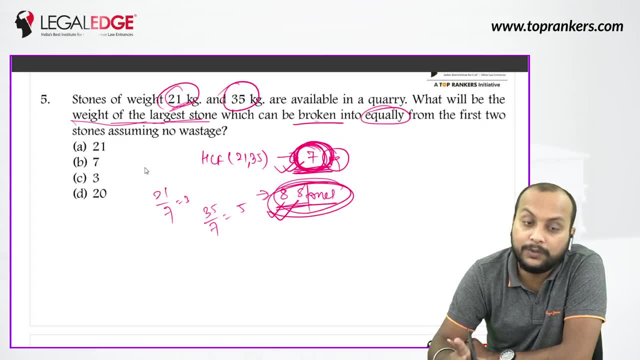 If you have been asked the number, then 8 stones. If you have been asked the weight in this question, then the answer will be B 7.. Clear, Clear. These questions are asked in another way. I will tell you here only. 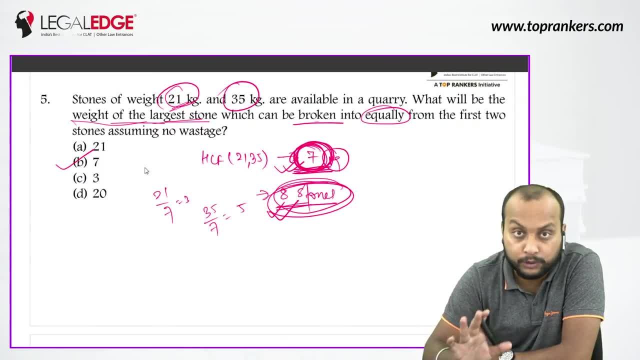 Don't get confused. These type of questions are asked. How will you be asked? I will tell you. One will say that there is a rectangular floor and marble is to be put in it. And how much is this floor? It is of 20 by 16.. 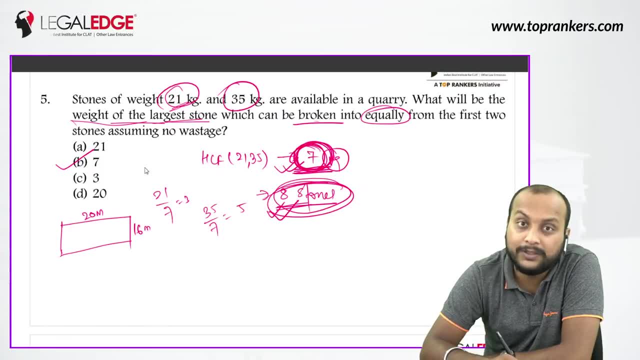 20 meter out of 16 meter. Minimum number of tiles. It will ask you the minimum number of marbles or tiles. Minimum number of square tiles. It will ask you this: What will be the requirement of minimum number of square tiles? 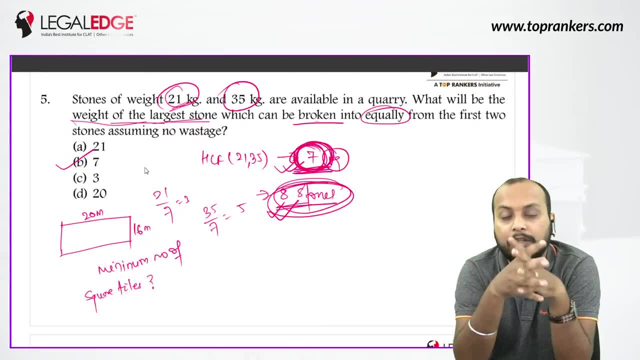 How will I be able to do the flooring of this entire floor? It is a rectangular floor. Its length is 20 meter and 16 meter. Tell me what will be the answer to this question? It is the same type of question. It is on HCF LCM base. 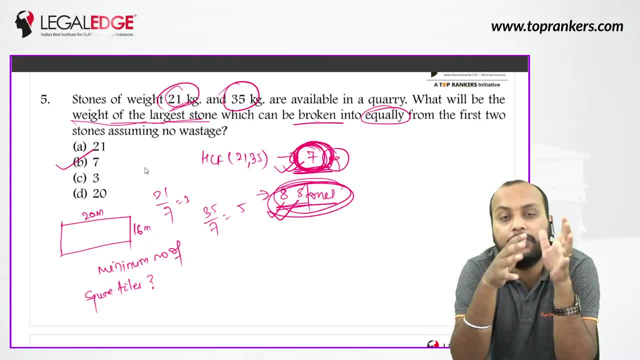 I have done it. here only These type of questions are asked. It is a rectangular floor. Its length is 20 meter and 16 meter And you have to tell that minimum number of square tiles required for the flooring of that floor To do flooring of that floor. 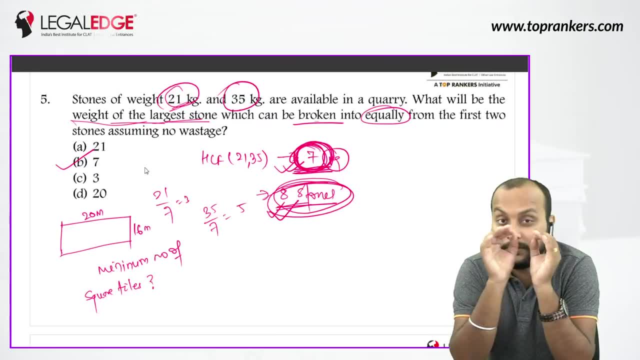 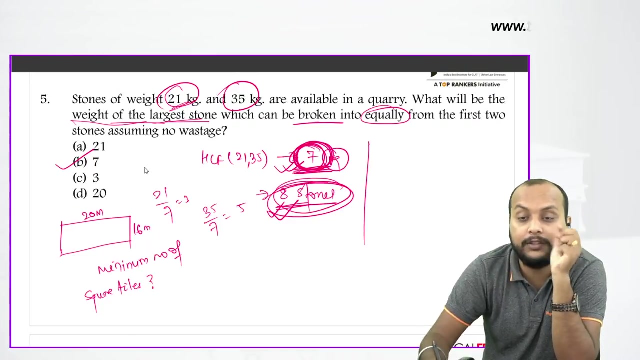 what will be the requirement of minimum number of tiles? How much size of tiles we need? It should be square: The required size. Let's do the div: How many tiles? correct answer is 20 to 0. answers ka hai. yahan pe ish chisko dekho, as it is question tha, lekin apan ne galat kya diya. 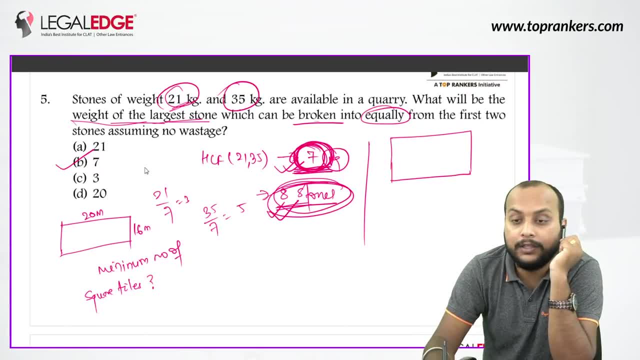 so humano yi rectangular, mere paas floor hai Yi diya hai, 20 M L and 16 M Width Boley Squared tiles. lagabia quat number are HCF of 20 and 16.. Why will we take HCF? Because it should be the factor of both, because it is called square. 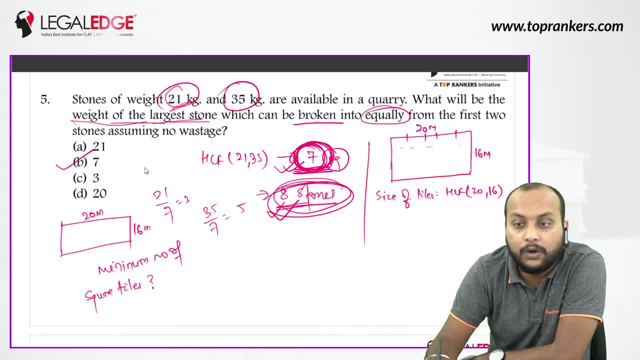 So it should be completely divisible by 20 and completely divide by 16.. So we will have to take HCF in this way. So what will be the HCF of this? 4.. So how many tiles do I have to take? I have to take tiles of 4 by 4.. 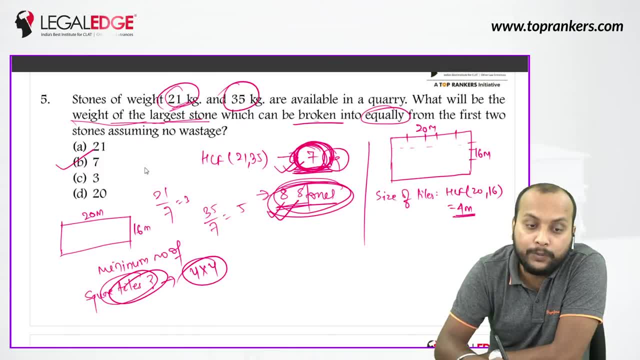 And if I put 4 by 4 tiles here, then I will have the requirement of minimum tiles. So what is the total area of the floor? 20 by 16.. And what will be the area of tiles 4 by 4.. 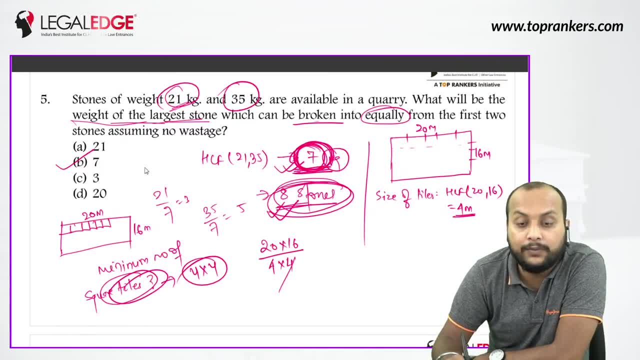 So this will be the number of tiles: 4 by 4,, 4 by 4.. How much do you have? 20.. You will have the requirement of minimum 20 tiles. Do you know when 80 tiles will be made? 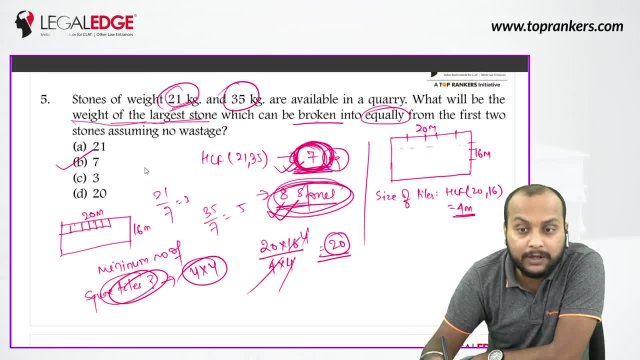 When you will take tiles of 2 by 2.. So that will not be minimum. 2 by 2 will be minimum, 2 by 2 will be 80.. Now if I take 1 by 1, then it will be 160 tiles. 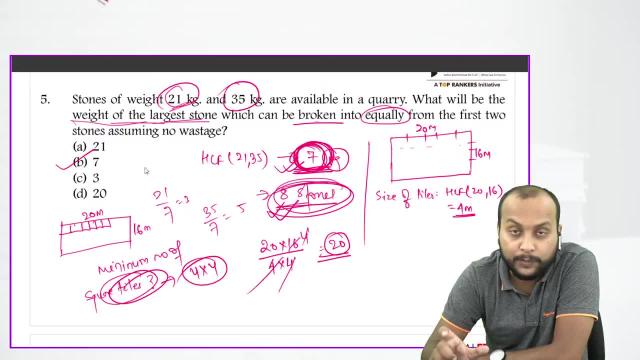 Ok, So I will take tiles of 4 by 4.. And how does this 4 meter come From HCF? And what will we do? We will divide area by area So we will get the number of tiles. We will get the number of tiles of minimum required. 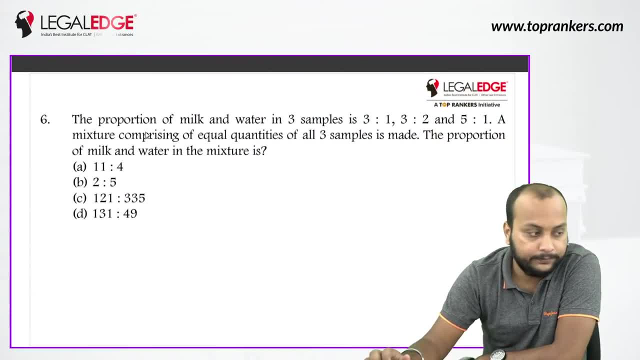 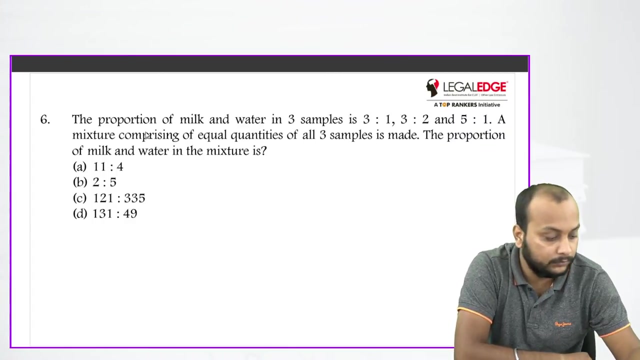 Ok, Next question, number 6.. What is the highest proportion of tiles? Less than 1 proportion, How many tiles will be made? 1. How many tiles will be made? 1. you a, d, a or d? don't answer that. 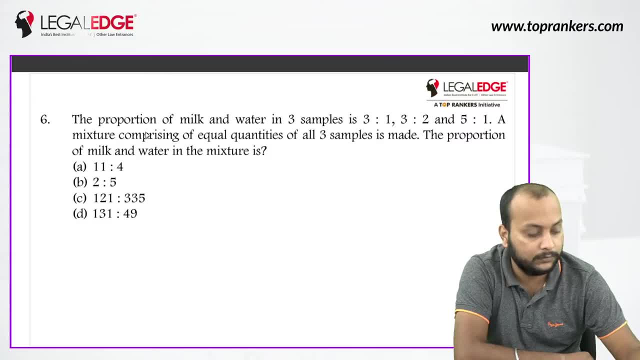 eleven is two, four. okay, d is the correct answer. one thirty one is to forty nine. one thirty one is to forty nine is the correct answer. let's see how to solve the proportion of milk and water in three samples. is three is to one, three is to two. 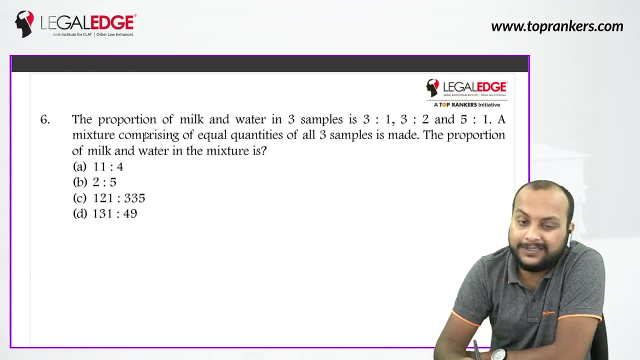 and five is to one. so three samples: sample one milk and water, sample two milk and water and sample three milk and water. so milk, water, milk, water, milk and water. first milk. three is to one, so out of four part milk is three, so milk is three by four. 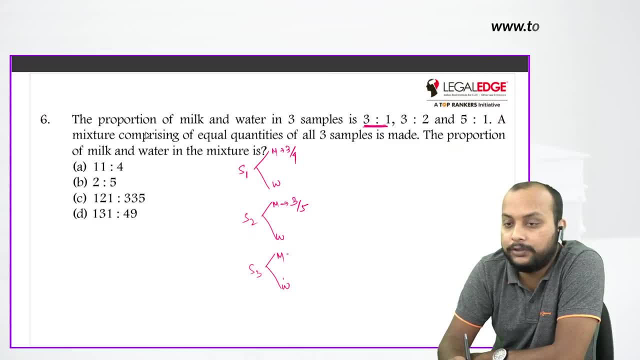 second: milk is three by five. third milk is five by six. this milk portion after milk. next is water. if water 3 by 4, then water is one by 4. here water is two by five. here water is two by five and water is one by six. 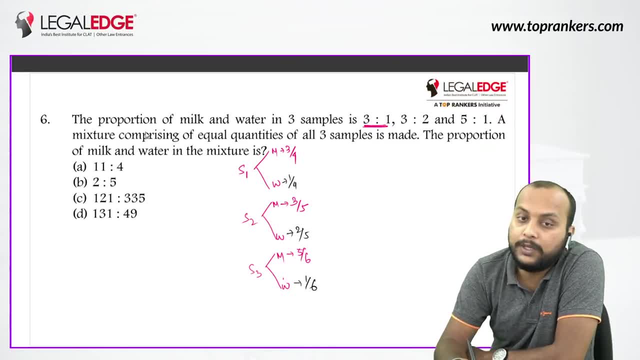 what is the next question? using quantities equal to this, we have to make the learning more efficient and easy with of them. If you want to mix all of them in equal quantities, then take all of them. So how much milk do you have? If I make a mixture, then how much milk do you have? 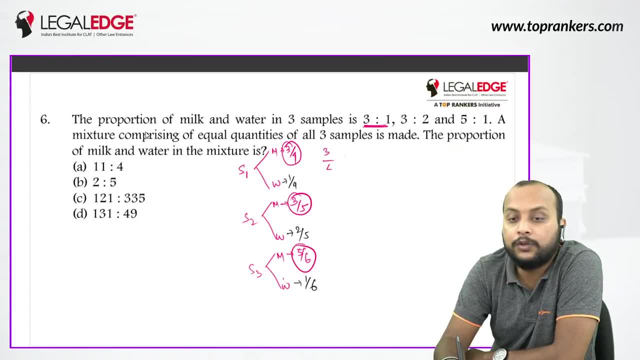 3 by 4 plus 3 by 5 plus 5 by 6.. So milk is 3 by 4 plus 3 by 5 plus 5 by 6.. So how much will be its LCM value? 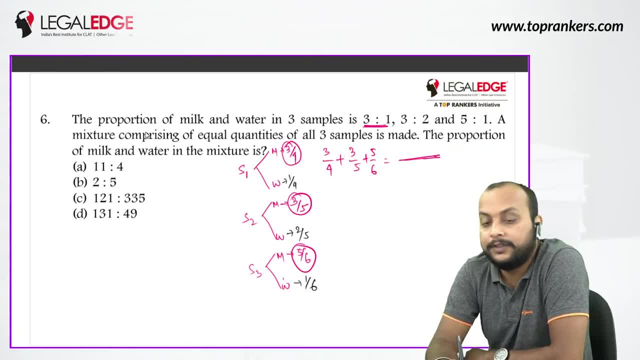 What is the LCM of this one? 60.. 60 or something else? LCM is 60.. So how much is its LCM? LCM is 15 into 3 is 45,, 12 into 3 is 36, and 10 is 50.. 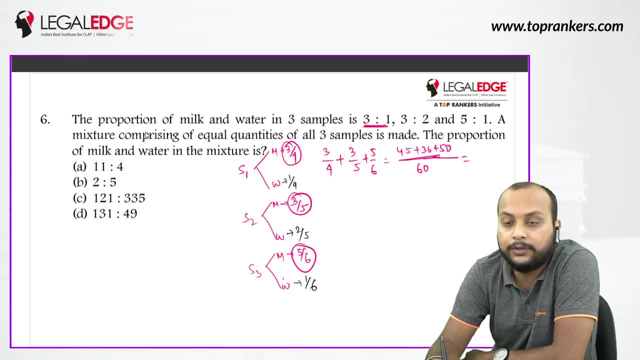 How much will be its LCM 86 plus 45.. 131 upon 60.. This is the milk value, Then water. Now we have this milk. What is the water? 1 by 4 plus 2 by 5 plus 1 by 6.. 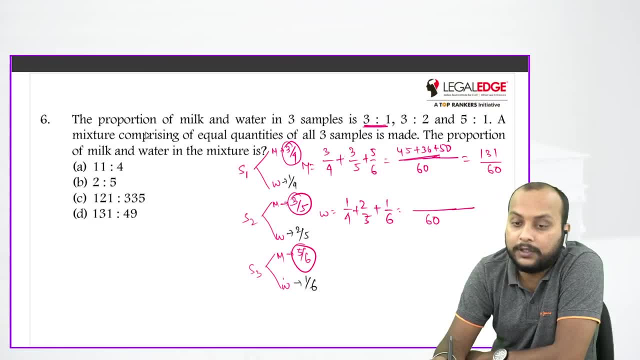 How much will be its LCM? 60. So LCM is again 60. So 15 plus 12 into 2 is 14.. 24. And 10. How much do we have? 49 upon 60.? 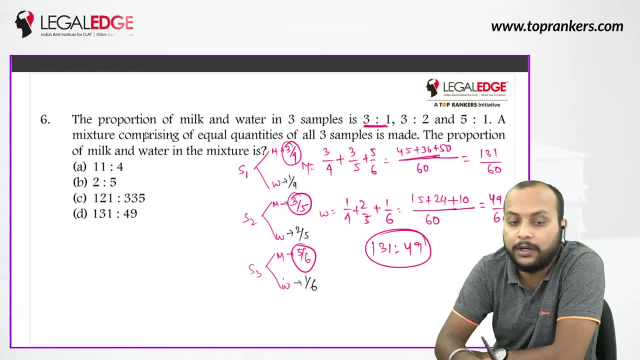 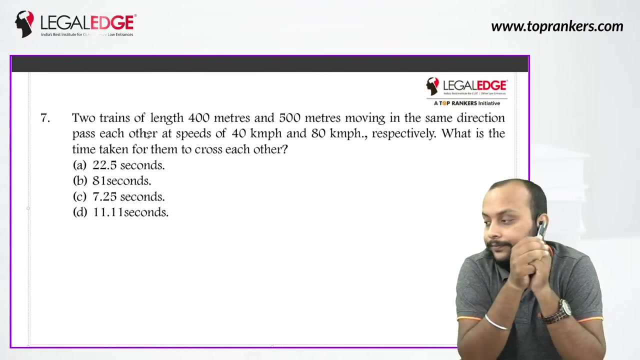 What ratio do you see? 131 is to 49.. Option number B: Here I have, Here I have, I have, I have Here B. Here you have B, I have B. B is in the direction of K. 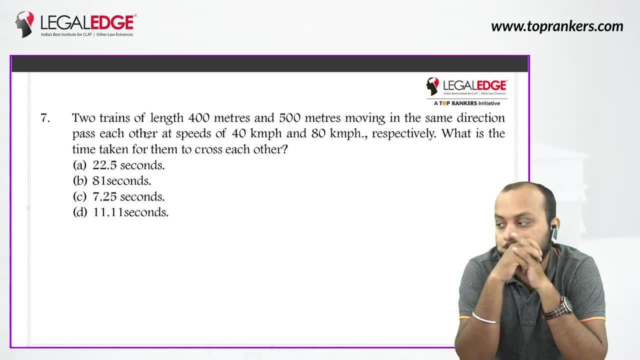 It is B. B is in the direction of V. This is the difference. Next, The difference is: It is in the direction of V. It is in the direction of V. You understand? Yes, This is the difference. Yes, 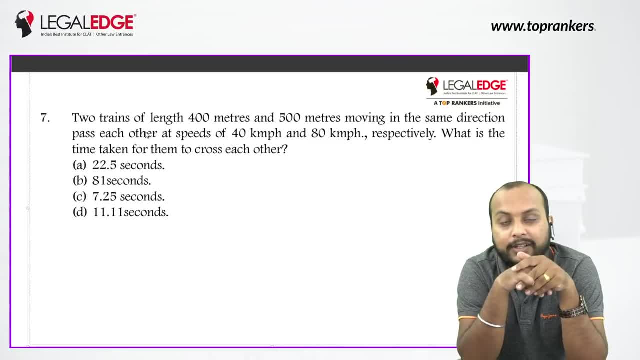 If I am talking about L, Yes. what is the time taken for them to cross each other? what is the answer for question number seven? time speed distance made train-based. question A, B, A, D. all the answers have come. no one said B. say B too. say B too. A, B, C, D. all will be done, someone will be right. 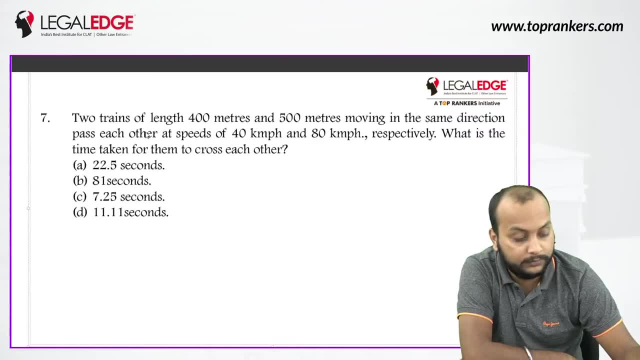 right till now, A, D and C have come. Priyanshu's answer has come B. ok, two trains, if they move in any direction, be it same direction or opposite direction, what distance do we take here? what is distance when two trains are passing each other either in opposite direction or in the same direction? 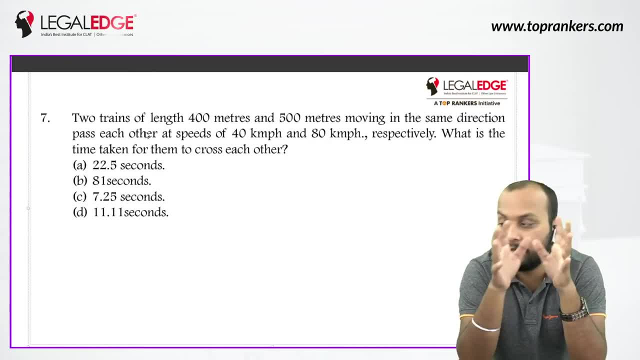 what will be our distance? because as long as distance time-speed-distance can be done, distance equals to speed into time, or speed equals to time, or time equals to distance upon time, or time equals to distance upon speed. if we are asked time, then we will have to divide it from speed. 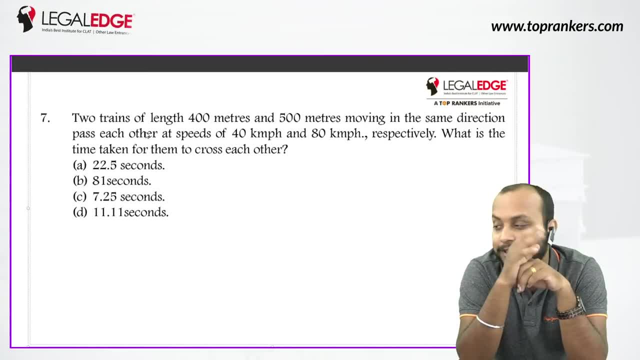 what will we have to do to take out the time distance upon speed? so what will be the distance if two trains move in same direction or opposite direction? so what will be the distance? distance is equal to length of the both trains, so distance will be sum of length of train. 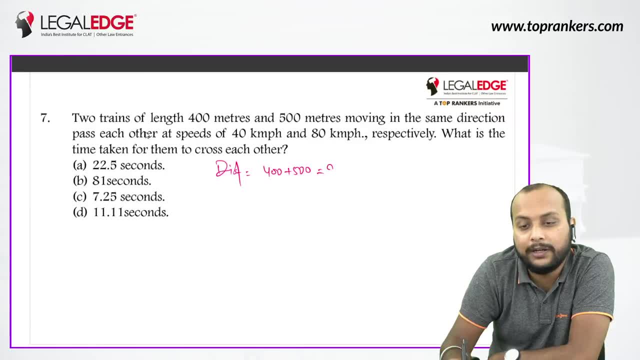 400 plus 500, that is equals to 900 meter. What will be the speed? The speed depends on the direction. The direction will be opposite or same direction. The speed depends on the direction. Here the direction is same, So the speed will be minus. 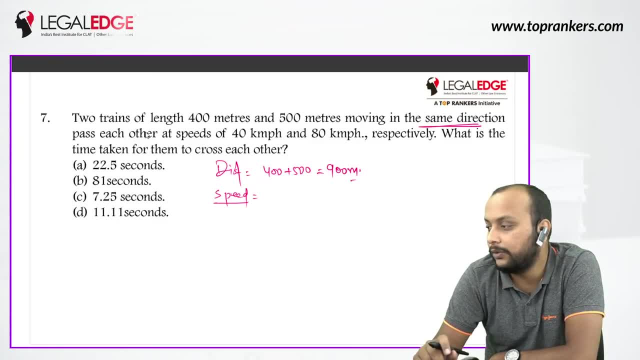 If it was opposite direction, then what would have happened? Let's do addition Here. the direction is same, So what will be the speed? The difference will be 80 minus 40.. What is the speed? 40 kilometer per hour. 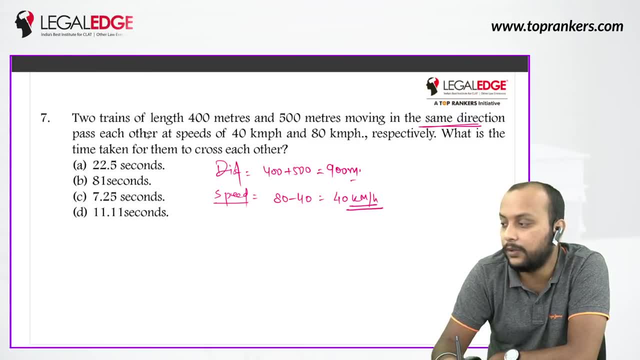 We will take care of the unit. Whenever you solve the question of time, speed and distance, The unit will definitely take care Here. the distance is given as 900 meter, Whereas your speed is given as kilometer per hour. So what will you do? 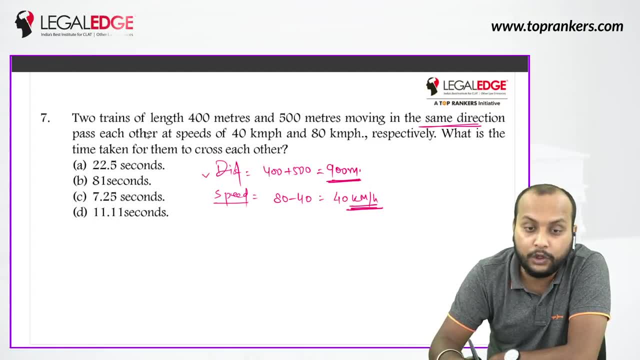 You will convert one. You don't have to do both. Either you convert the distance or the speed into meter per second. We have to take out the time, So what will be 900 divided by 40.. Distance upon speed. But I am converting the speed into meter per second. 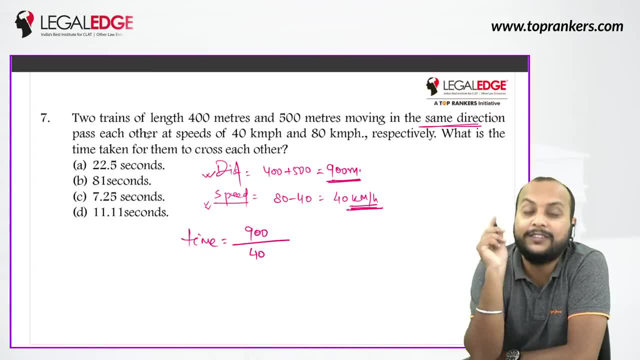 Because all the answers are given in seconds. That is why I will not convert the distance into kilometer. I will convert the speed into meter per second, Because the answers given in options are given in seconds. So what will happen from here? I will convert the speed into meter per second. 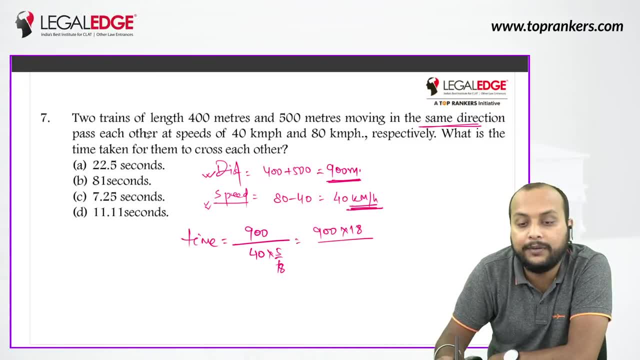 Whatever the answer will be, it will be your answer. So, 900 multiplied by 18, divided by 40, into 5.. This will be your answer. Okay, From 0 to 0 and from 5, it will be 18.. 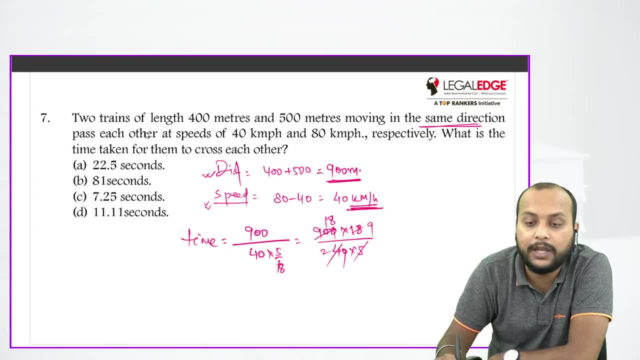 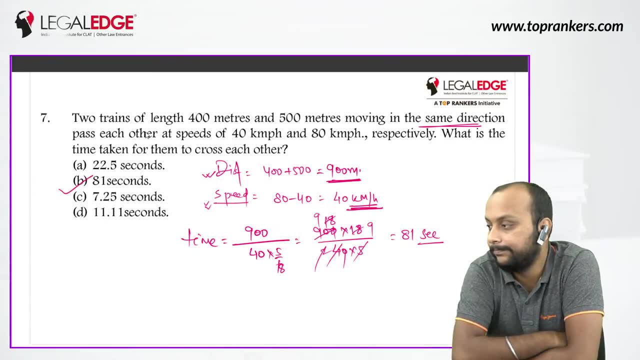 And from 4 it will be 9.. And from 2 it will be 9. And from 2 it will be 9.. How much did it come 81 seconds? Option number B: Clear: Yes, Very good. 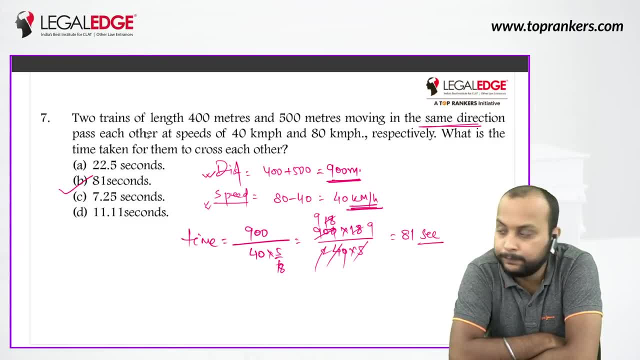 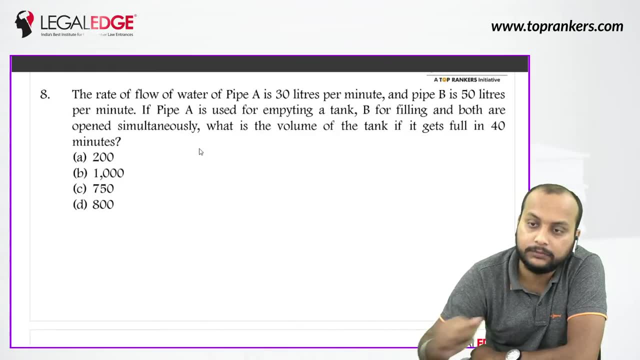 Any doubts, Come forward. Okay, Next one Question number 8.. Term and work application. That is, pipe and systems. Question number 8. Term and work application. That is, pipe and systems. Question number 8. Term and work application. 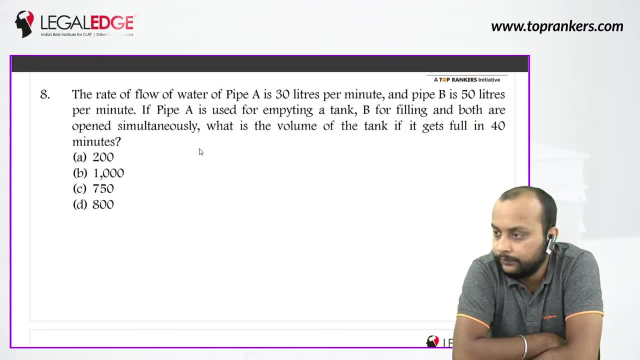 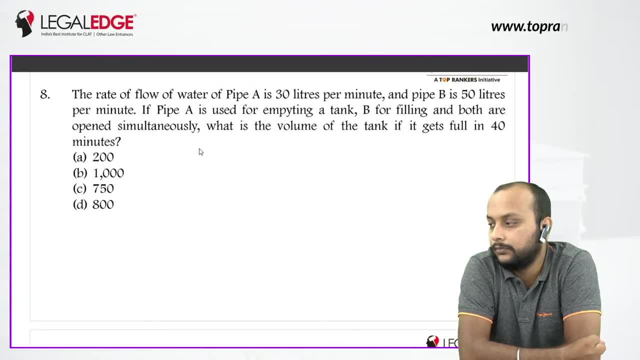 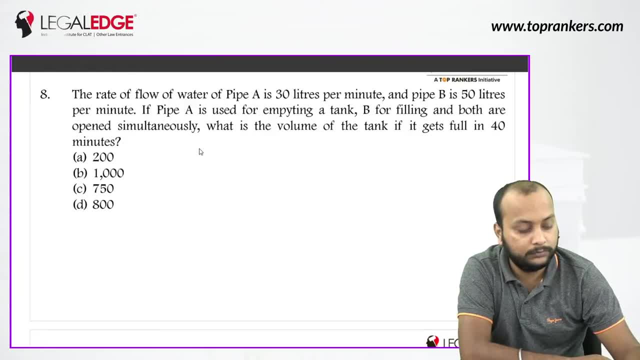 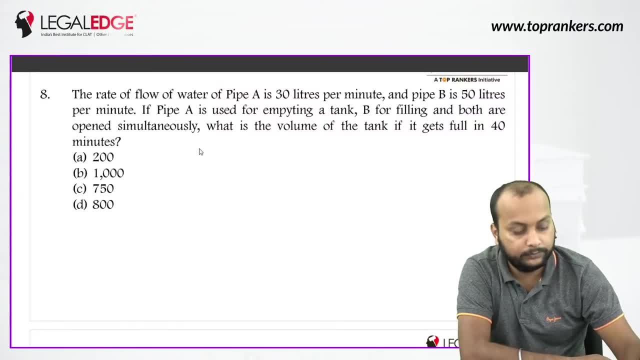 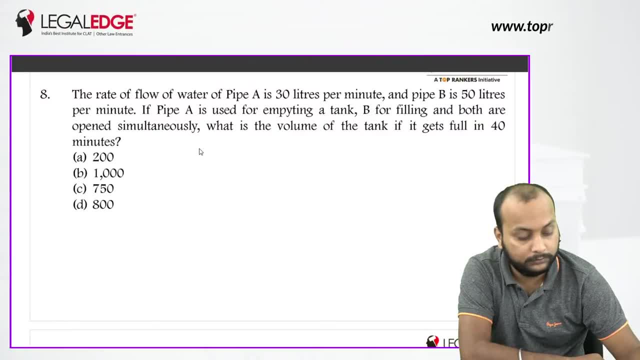 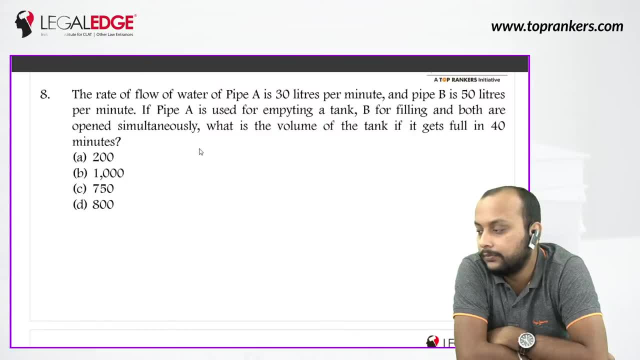 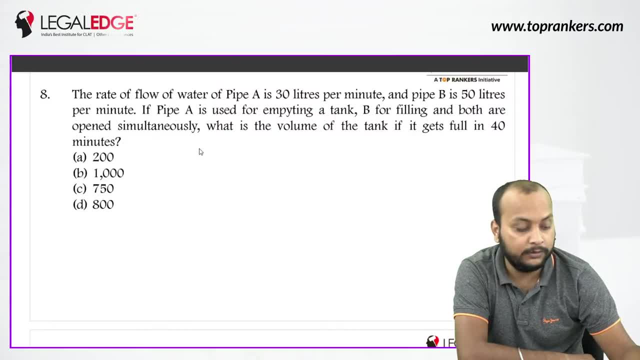 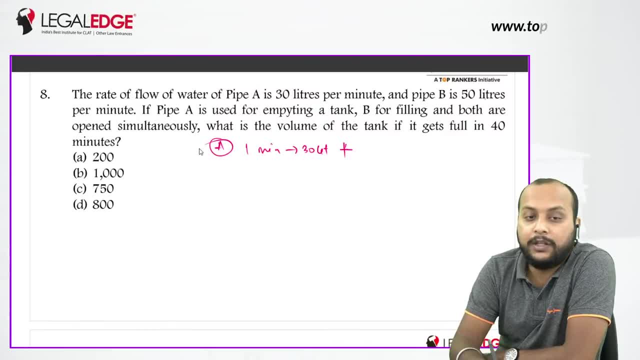 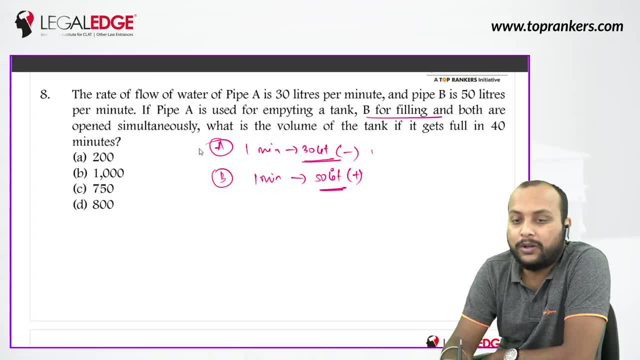 Term and work application. That is pipe and systems. Question number 8.. Term and work application- That is pipe and systems. Question number 8.. Term and work application. Question number 8.. Term and work application- Question number 8.. 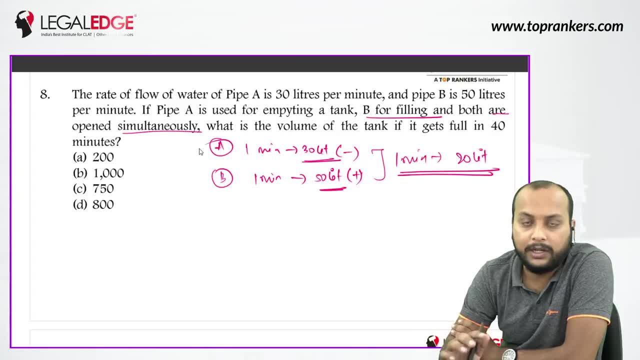 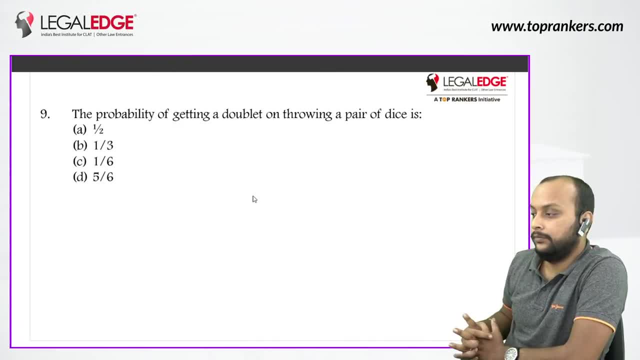 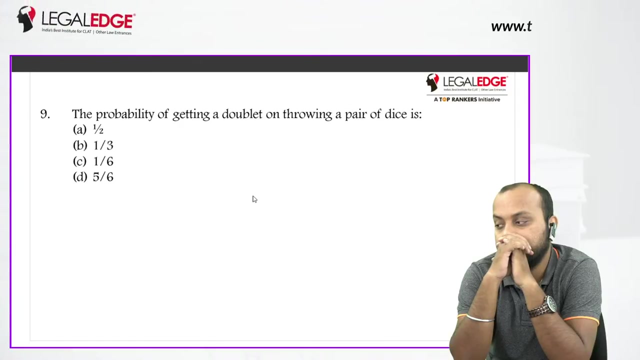 Question number 8.. Term and work application. Answers are coming. you must be enjoying it. if answers are coming, then it is fun. We will discuss about that later on. If we do one thing at a time, then it will be better. 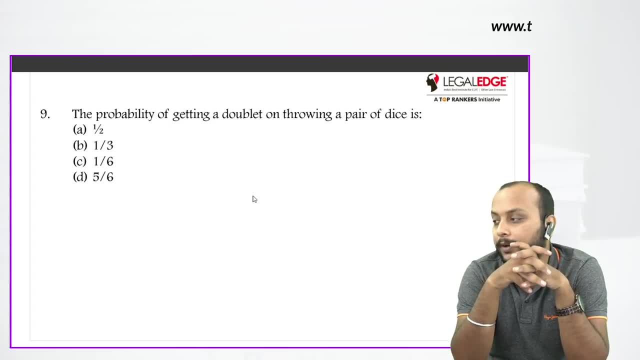 For this also. We will come to that later. We don't have deadline for that. We have to give reply within 2 hours. We have to take admission. We can hold that till the class is going on. We will discuss on that. 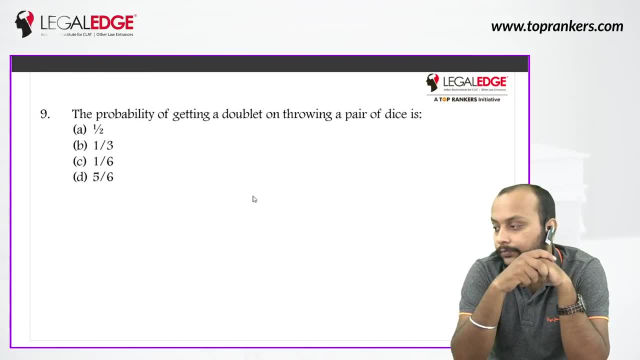 The probability of getting a doublet on throwing a pair of dice. How much is the sample space of dice? What will be the sample space of dice Throwing 2 and throwing 3 or throwing any n numbers of dice? First of all, what is the probability of getting the probability? 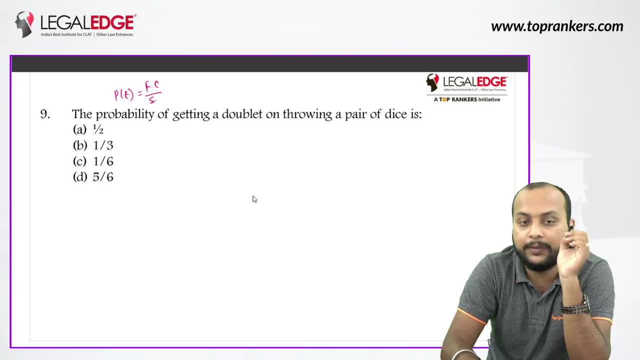 P-A: probability of the event. Favorable case upon sample space. What do we need in dice sequence? First of all, we need sample space. What is the sample space? 6 is to power n. 6 is to power n. 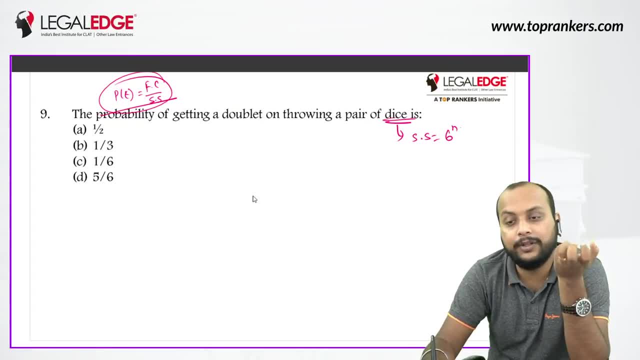 Where n is the number of dice or number of terms. How many dice have you thrown here? Pair of dice, That means 2 dice. What will be the sample space? 6 square, that is equal to 36.. Okay Now. 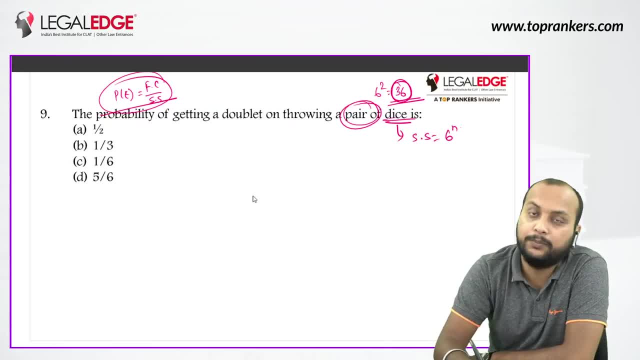 36 is the sample space. Probability is favorable case upon sample space. So how many cases will favor me to get a doublet? See these cases. 6 is to power n. So if I see the cases that will favor me to get a doublet, 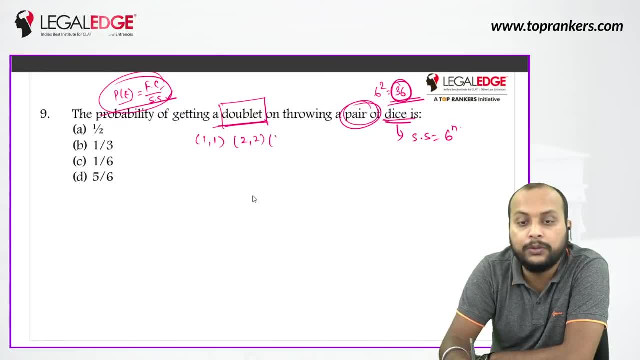 So 1 on both dice, 2 on both dice, 3 on 3.. 4 on 4., 5 on 5. And 6 on 6.. So total 6 cases are there And if I get any of these, 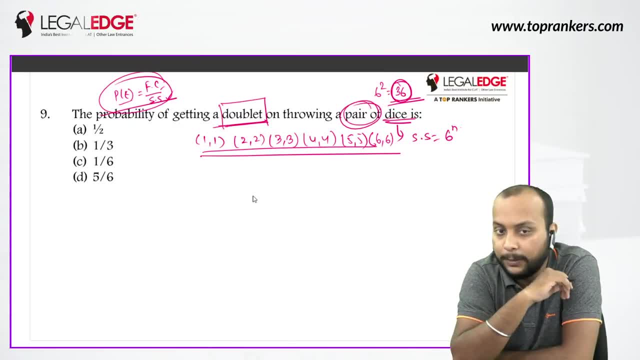 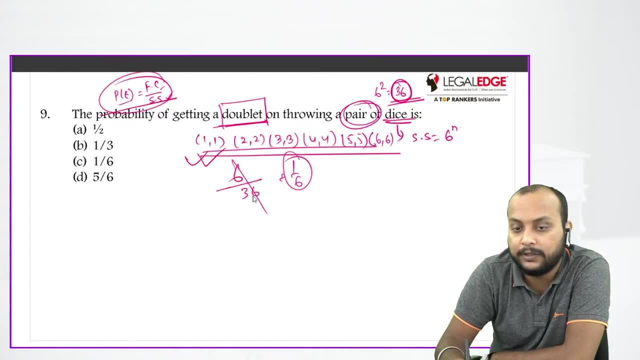 Then all the conditions given in this question will be fulfilled. So how many cases will favor me 6. And how much is the sample space 36.. So what is the answer? 1 by 6.. What is the answer? 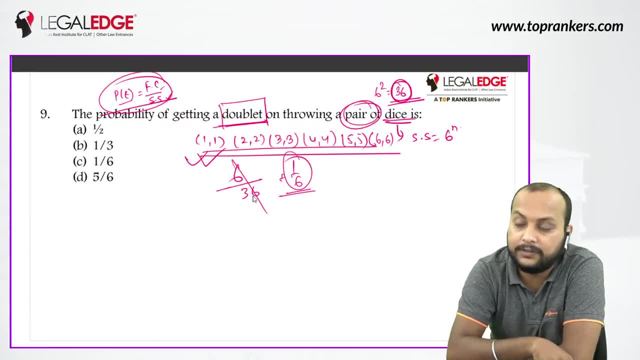 1 by 6.. So option number C is the correct answer. Option number C is the correct answer. Option number C is the correct answer. So if I have a random number that is more than 24.. If the number a is less than 24, that's it. 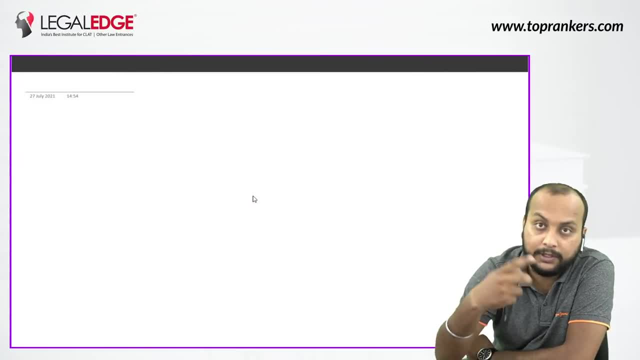 So this is what I want to tell to you. So let's see how we are doing here. Find out if you have 1 or 2 positive solutions for diamond- See first table on the graph. On this table I will explain more about both 1 and ALT of models as swap, which are 76,. 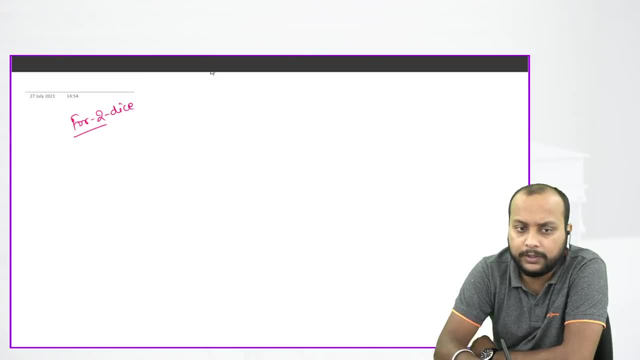 If someone was asking me yesterday then I would have said that we will see. you have a lot of things. those who know it is a good thing, those who do not know it. note it down carefully: whenever you will come to the question of dice probability, you will not have to make a case. and what happens by making a case, the chances of mistakes increase. it increases because if there is a difference in one case, then the answer will be wrong. it is two dice in two dice. your sample is six square, that is. 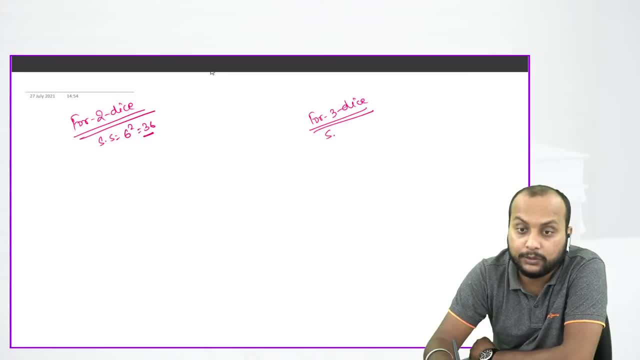 equals to thirty-six, and if there are three dice, then the sample will be six cube, that is equals to two hundred and sixty, right? so these two things now the total case is two hundred and sixteen. here it is thirty-six. how many cases will you make? we have to check that the case is not repeated. if any case is not left, then the chances of error increase, and if one case is also missed by mistake, then the answer is wrong. so I tell you in both the cases what to ask. it asks sum right that both the dice are thrown. two dice are. 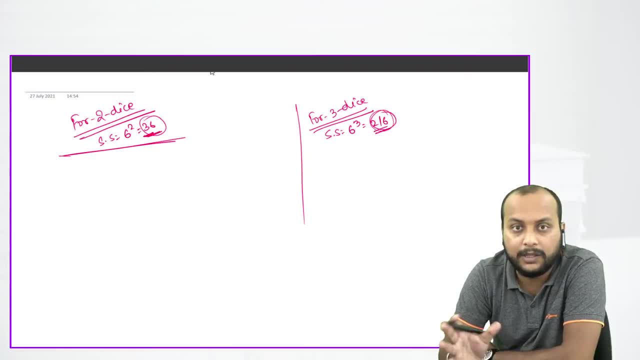 thrown, then what will happen in both? what comes to sum sum is coming, sum two is coming, sum three is coming, sum four is coming, sum five is coming, sum six is coming. so what will be its probability? favorable case upon thirty-six. 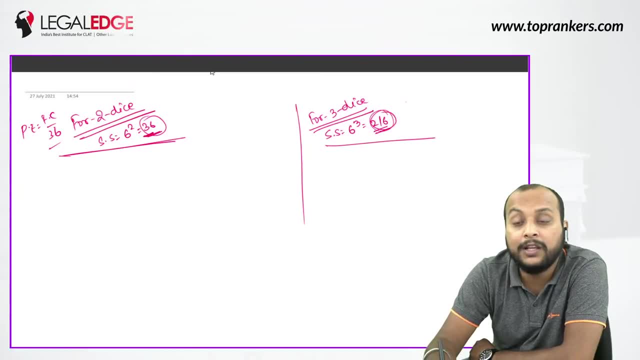 I wrote thirty-six in the sample space and here what will be the probability, sample space, favorable case upon two hundred and sixty. so in the case of sum, when you are asked then what can be its favorable case, I will tell you a table of them. remember them and remember this. 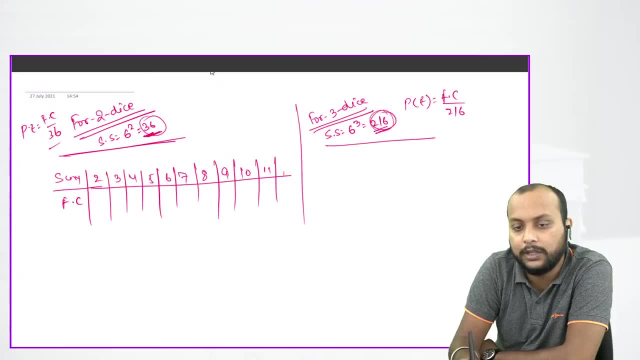 what will you remember? you will remember automatically. it is so easy that there are no problems. if you throw two dice, then the minimum is two, there are two, one, one and the maximum is 120,. two have six, six, there are nine, seven, eight and nine, so it comes one. 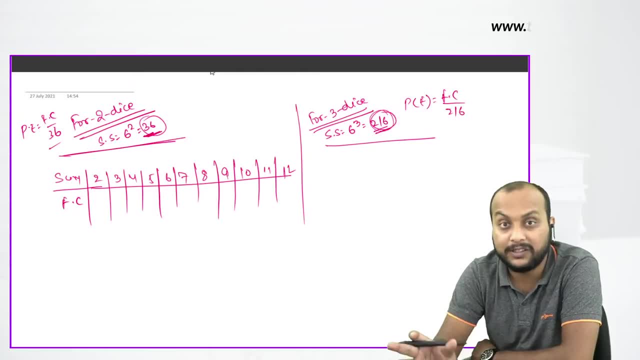 one, one, one three, one four, six, four, and the sum will be three, six, three, one, six, and if the maximum is one, one, that would be two, and the maximum of the six positions will be twelve. the rest will be included in this. 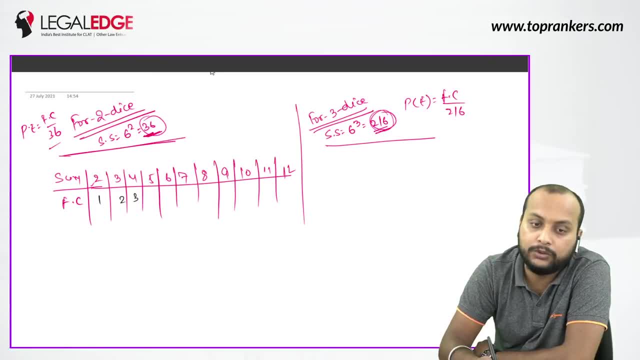 So when a favorable case happens- 1,, 2,, 3,, 4,, 5,, 6,, 5, 4, 3, 2, 1, these are their favourable cases. if someone asks: tell the probability that sum 7 has to come. if you throw 2 dice, then what will you do in 7, see how many cases are there- 6, and 6 will be divided by 36, answer will be 1 by 6, that will be the answer in 2 dice. similarly, for 3 dice, I also give ok. you also take care of that favourable case. 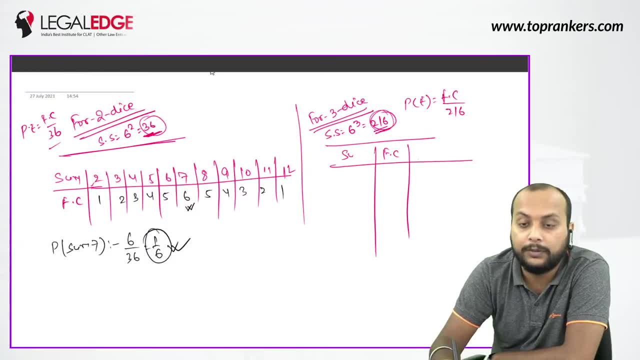 and in both sides I am writing sum, because here common part is there. so minimum sum in 3 dice will be 3, because 3 dice will have 1, 1,, 1,, 4,, 5,, 6,, 7,, 8,, 9,, 10,, 11,, 12,, 13,, 14,, 15,, 16,, 17, and 18,. 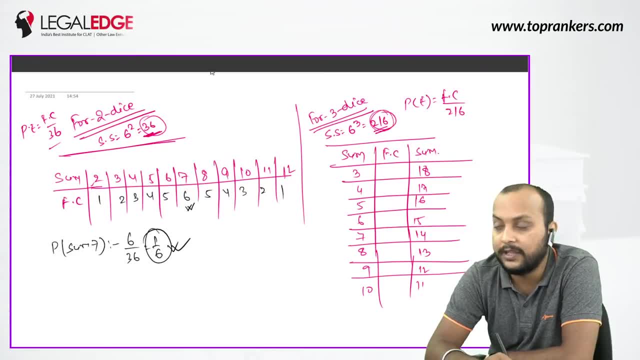 so maximum 18 will be there. so these 3 dice will have 6,, 6, and 6, so favourable case is 1,, 3,, 6,, 10,, 15,, 21,, 24,, 27,. 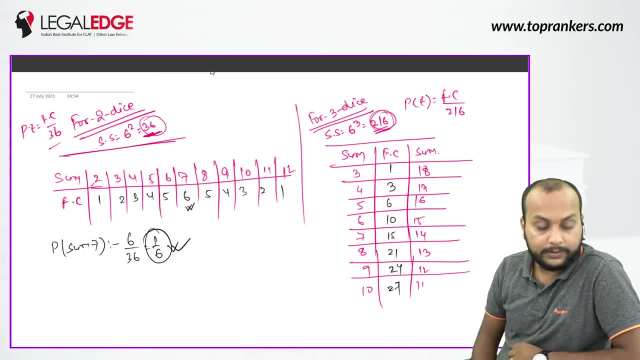 ok, now you can memorize it. you can put questions on it. so remember, if you ask questions in front of 3 dice, then you can prefer 3 dice table. you will never have to make a case example in 3 dice I asked you find the probability of getting a sum of 11, in which, in 3 dice, how many cases will have to be made? 27,, and when you will make 27 cases then it will consume a lot of time and cross check will also have to be done. so if you remember this table, then we can directly say 27 upon 216,. 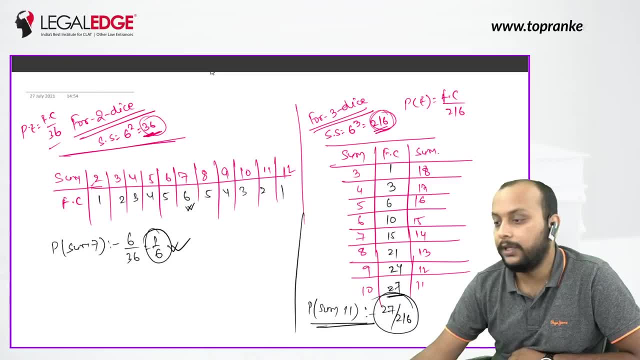 1 by 8 will be there by canceling out, ok, but we can calculate. so 27 upon 216 will be there for 2 dice as well as for the 3 dice. ok, it is not more than 2 dice. any exam, competitive exam, according to your law, interest test, whether it is elite, MHCT, whatever it is, BLAT, whatever it is. your questions above 2 dice have not been asked yet, but still we should do the questions up to 3 dice. 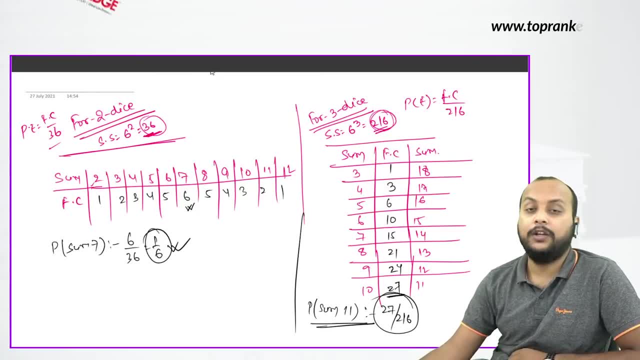 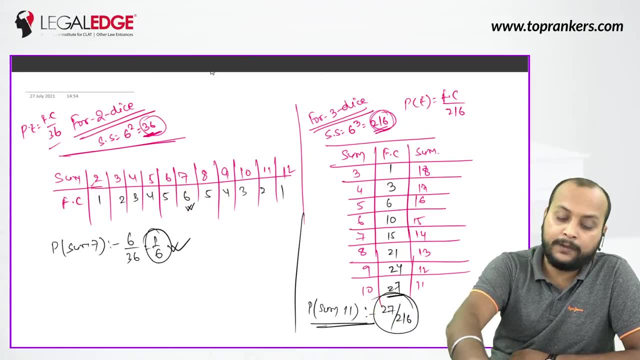 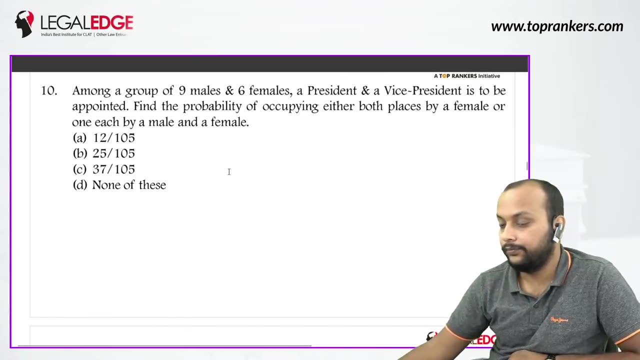 sometimes, if you increase the level of questions and ask us 3 dice, then we should be able to do it. we should know it. ok, come on. move to the next question, number 10, based on combination. Anuja is there in this or not? these questions are on the pattern on which elite questions are asked. 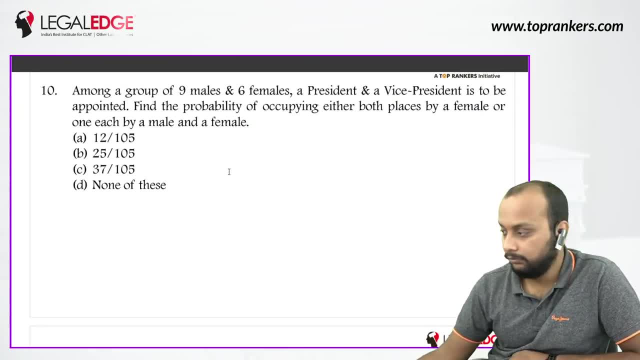 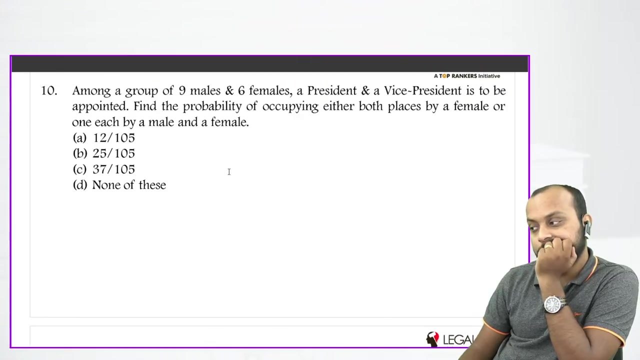 based on the same pattern, he- let's to- certain generalで expressed: GAS negative N is relative relative negative ITH ti-. then start practice with timer. with timer on all subjects. don't use timer on mobile. use timer on analogue watch, otherwise timer will be set. 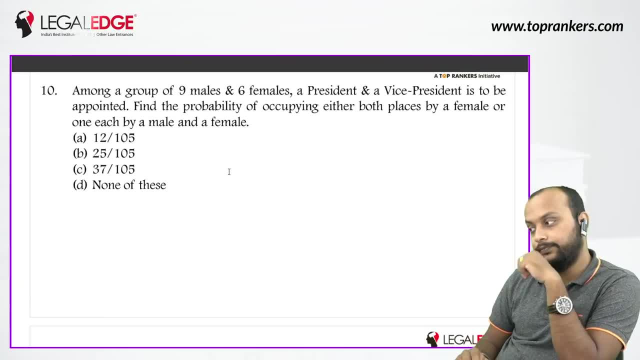 here, among a group of 9 males and 6 females, a president and a vice president is to be appointed. find the probability of occupying either both places by a female or one each by male and a female? easy question of combination cards answers. i d answer is the correct. 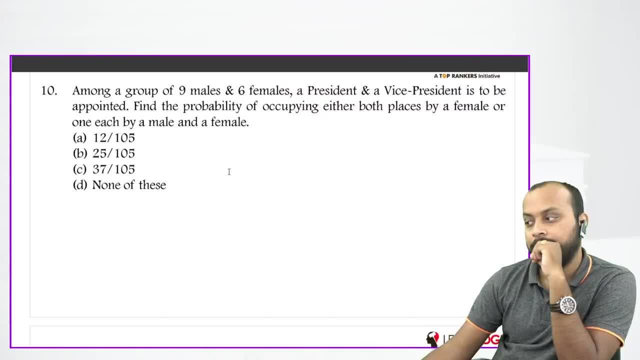 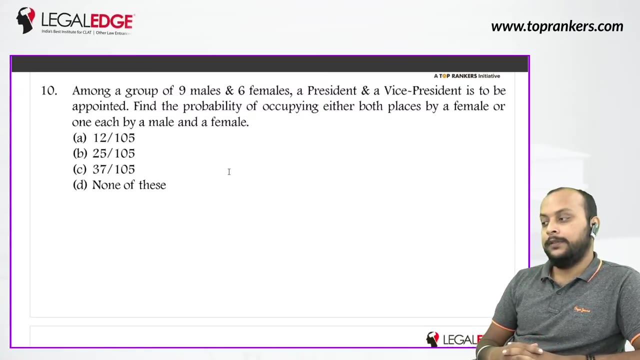 the correct answer. correct answer questions, sir. questions Very good. Yes, 69 upon 105.. Aditya, Correct B is the correct answer. Group of 9 males and 6 females. Okay, Now we say: group 9 males and 6 females, A president and a vice president. How many seats are there? 2. Okay, 2 places are there. Both places are given. 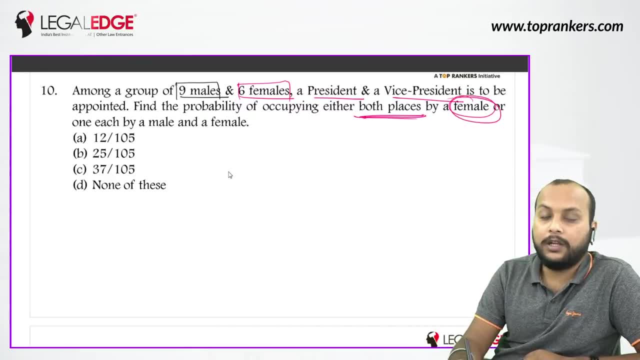 Now on both of them. either you have to keep it female or what we can do is on the place where there are 2, it should be female First case And the second case should be 1 male and 1 female. 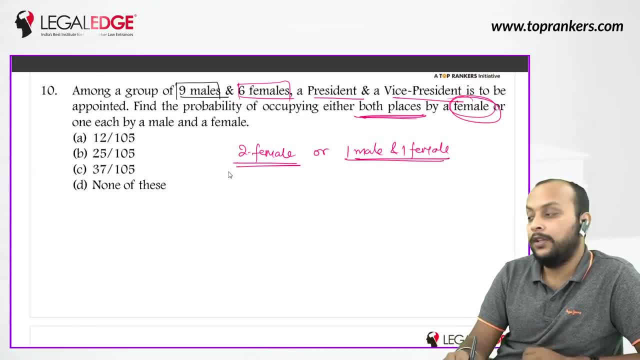 1 male and 1 female and 2 females. Both cases should be there. How many total females do we have? 6.. Okay, How many total cases do we have? How many total females do we have 6.. Now, from 6, the 2 places both the president and vice president. we have to give it to the female, So 6C2.. From 6 females, we have to select 2 females. 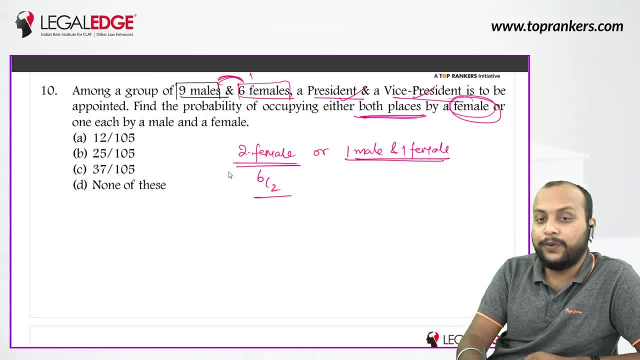 Total number of persons, if you see it is 15.. You are selecting out of 15.. So upon 15C2, this is our method of selecting 2 females- That both the places, both the president and vice president, should be male and female. So 6C2 upon 15C2.. 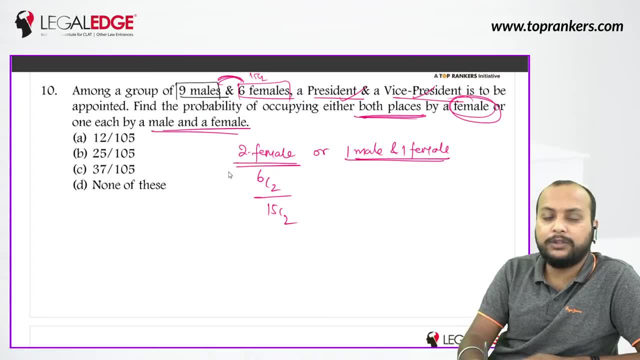 Either 1 male and 1 female. Now, each by 1 male, It can be anyone. Now, if the president becomes male, then vice president will become female. If vice president becomes female, then If it becomes male, then what will be the president? It will become male. It will become female. 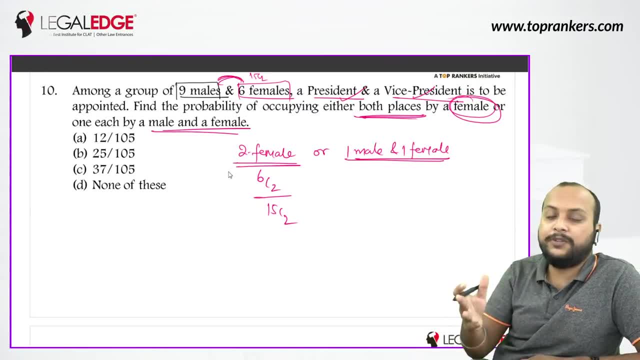 So you have to keep it alternate. That means the president and vice president can be done in male-female. So we need 1 male and 1 female From 9 male, 1 male, 9C1 into 6C1.. Because we need both. That is why we need 2.. 1 male and female upon 15C2.. What will happen next? 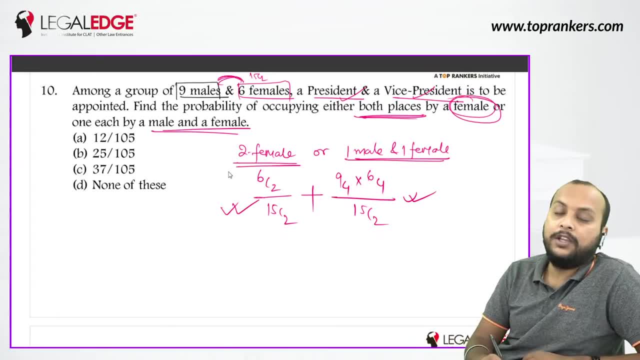 Plus, Either you go with this or you go with this, You will solve them. From today, you will get none of these. 69 upon How much is this? 15 upon 105.. Plus what will be this? 54 upon 105.. So what will be 69 upon 105.. Option number D. 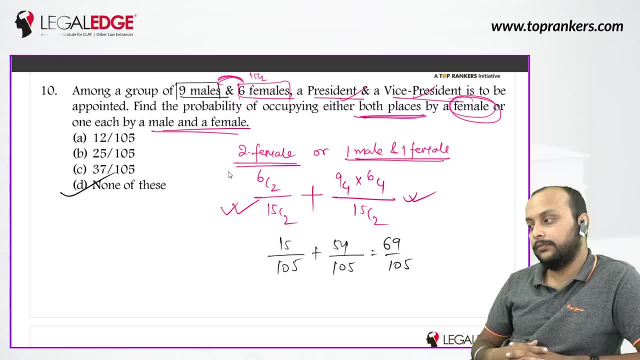 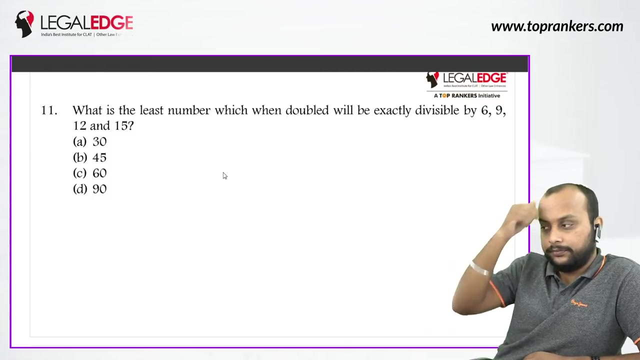 One time you will have to write prisons. Éмо a sea of sample смерcei divideyeaá. Take now move on to the next one, Question number 11.. What is the least number which, when doubled, will be exactly divided by��에? 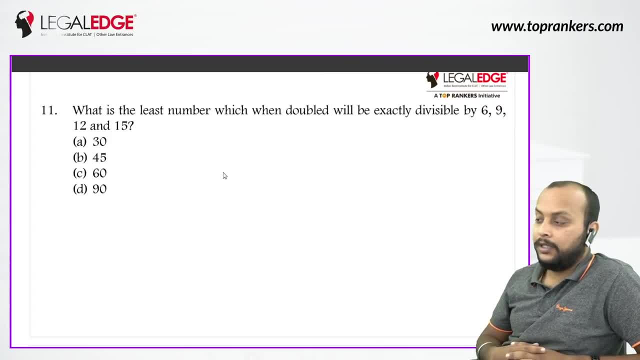 divisible by 6, 9,, 12 and 15.. 6, 9, 12 and 15.. Exactly divisible. Thank you. B, C, D. All three answers have come so far. Hence the correct answer for this question is D 9, 0. 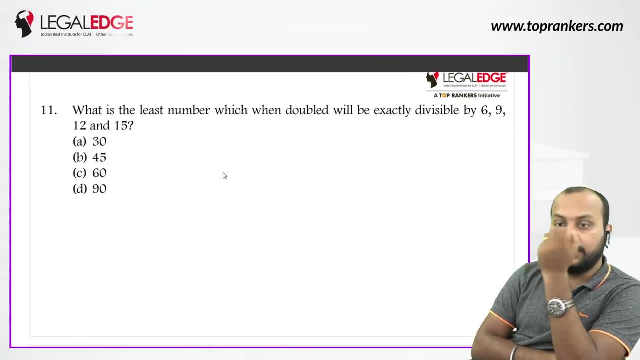 What is the least number which, when doubled, will be exactly divisible by, And whatever number it is 6, 9.. 12 and 15 will have to be completely divisible. So in this case we will find LCM. Whose LCM will you find? 6,, 9,, 12 and 15.. What will be its LCM? What will be its LCM? 180 will be its LCM. Let's see how to find it. First method is prime factorization. 6 will be written as 2 into 3.. 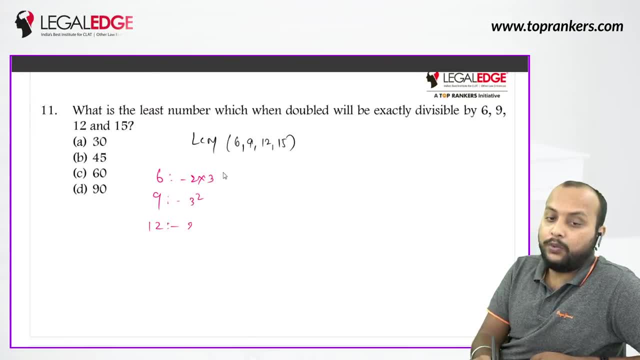 9 will be written as 3 square, 12 will be written as 2 square into 3. And 15 will be written as 3 into 5.. So the highest power is LCM. LCM will be written as 3 square, 2 square and 5.. 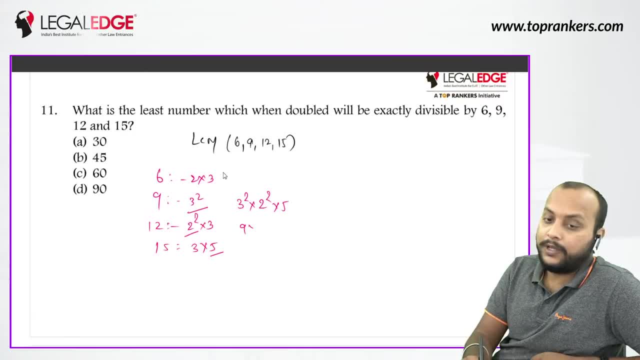 LCM will be written as 3 square, 2 square and 5.. 9 into 4 into 5, that is equals to 180.. This will be our LCM. Okay, This is our LCM. What is the LCM of the second method? 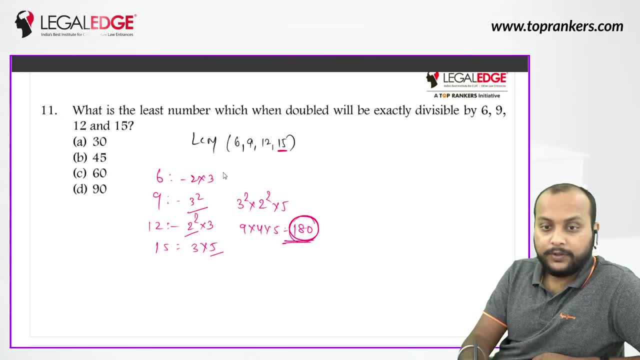 Take the largest number, 15.. Okay, The LCM will be more than 15 or equal to 15.. I have already told you that the LCM of the second method is equal to the largest number. So the answer of LCM will be more than 15 or equal to 15.. 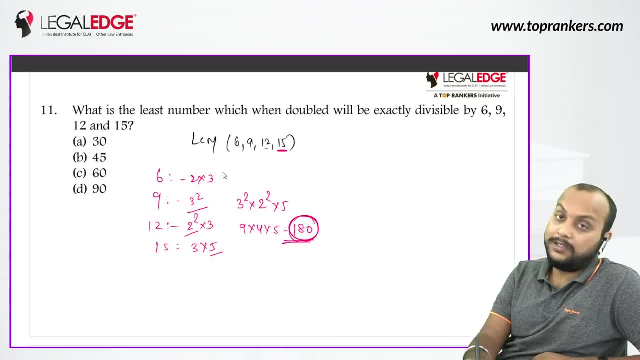 Now you don't know that the LCM of 12 and 15 is not equal to 15.. There should be something else. So what will you do? Take the LCM of 15 and 6.. Take the LCM of the largest and smallest. 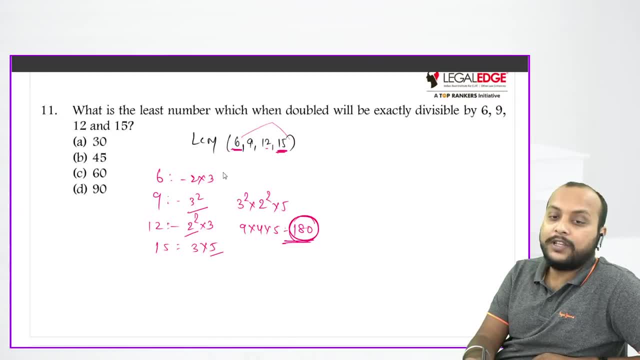 Take the LCM of the largest and smallest. So how much is the LCM of 15 and 6?? The answer is 30.. Did you get it? The answer is 30. I am telling you to solve it orally. Understand it carefully. 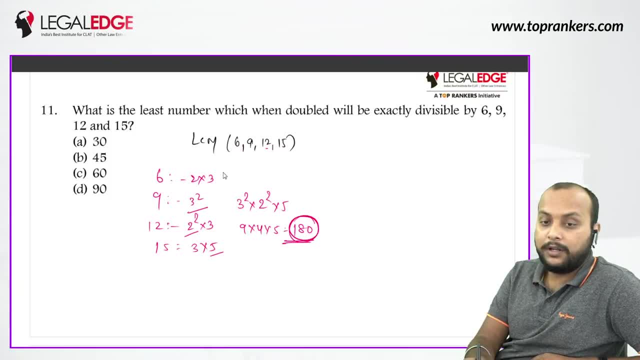 I am telling you how to solve the orally LCM. I was asking you how to calculate the fast LCM. If you follow this method, you will get the time here. How do we do it orally Now? you see that there is 15 here. 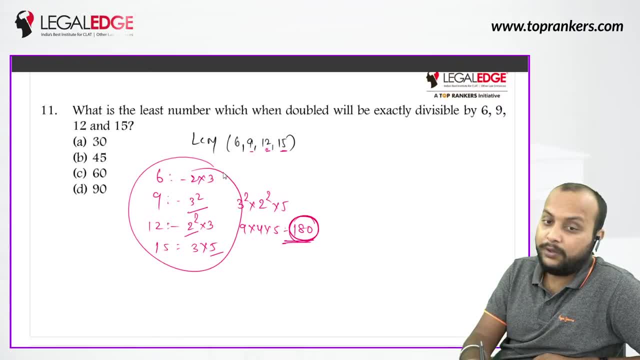 There is no factor 12 in the table of 15.. Neither there is 9 nor 6.. So there will not be 15 LCM. Why not? Because the rest of the small numbers are not its factor. There is no factor of 15.. 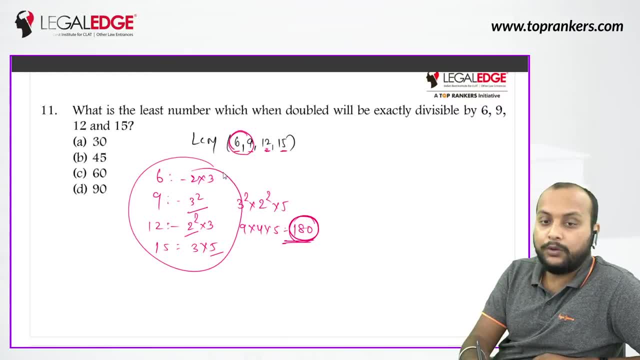 So now, what will you do here? Take the LCM of these two. See, the most important method, The LCM of 6 and 9, will be 18.. You can do it easily or morally. If you take the LCM of 18 and 12,, then this will come. 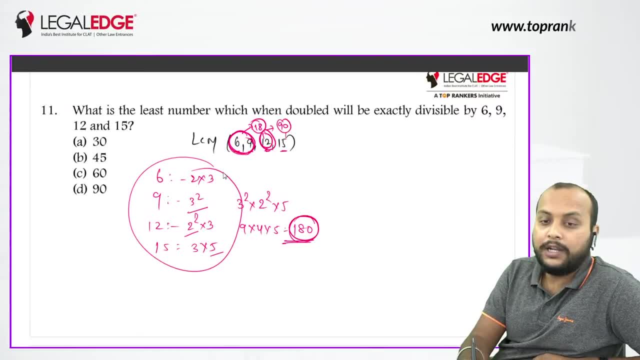 How much does the LCM of 18 and 12 come 90.. And how much will the LCM of 95 come? It will not come 90.. The LCM of 80 and 12 will come 72.. 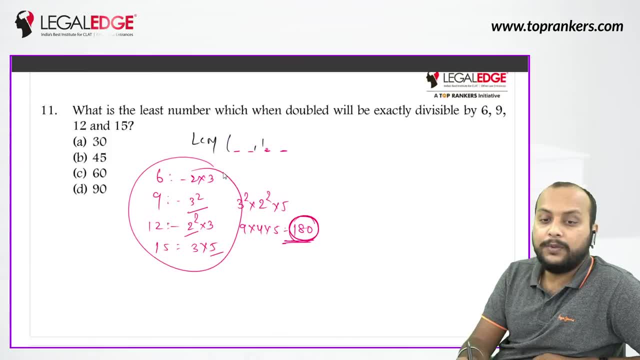 And then how much will it come? 180.. So in this way you can easily calculate orally. If you practice then it is easier to calculate orally. So 180 is done. So I told you to do half, Because the number that will be divided. 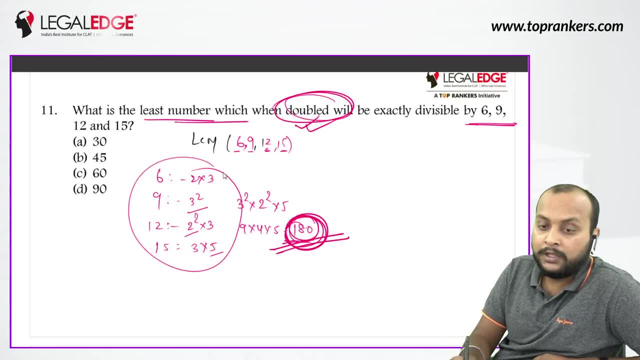 the number that is asked should be double. That is, the number that is asked is double. So what is the double of 90?? 180.. The correct answer is 180.. Now move to the next one, Question number 12.. 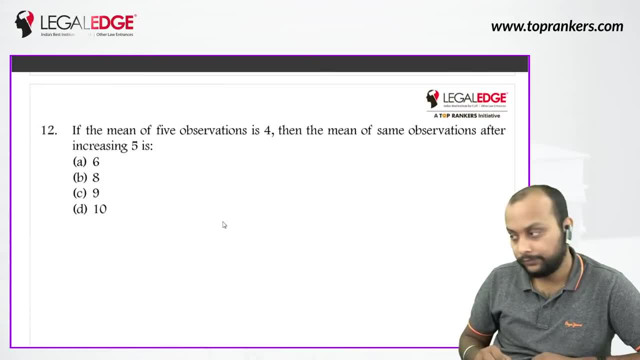 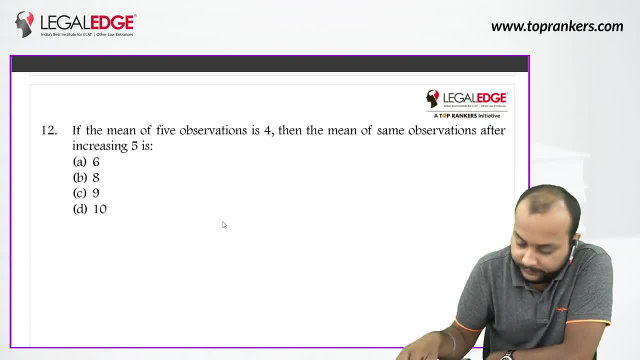 now i will tell you how did you solve this question. mostly people did this. the mean of five observations is four, so here is the sum. what will come 5 into 4 equals to 20.. Now he said: increase all the numbers by 5.. 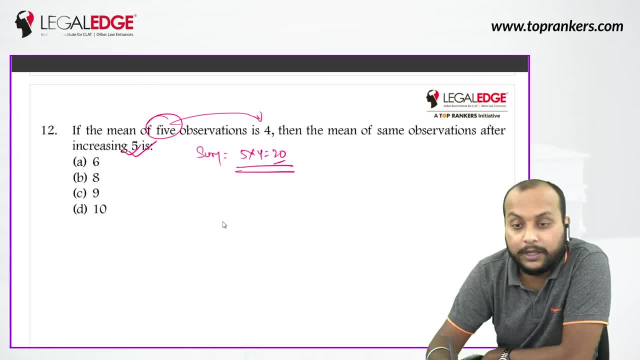 So it was 20.. If you increase all numbers by 5, it will be 20+. If you increase all numbers by 5, so if you increase 5 by 5, then 5 into 5 will be 25.. 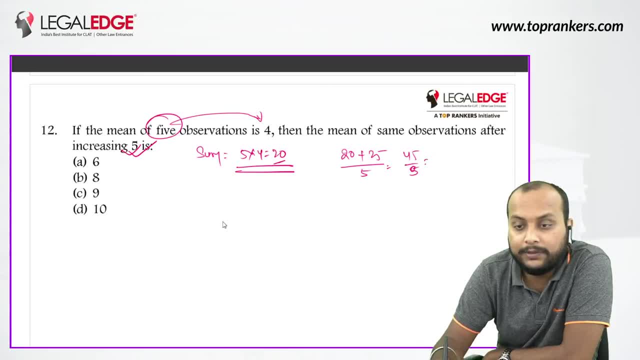 The average will be divided by 5.. So 45 by 5, that is equals to 9.. Some people might have done the same, For example x1, x2, x3. Or if you have 5 observations, then a plus b plus c plus d plus e. 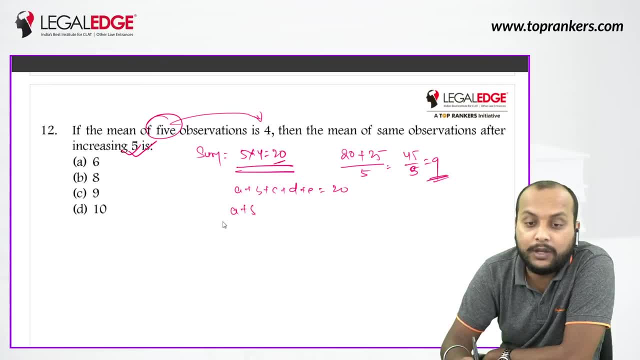 will be equal to 20.. Everyone has increased by 5.. a plus 5 plus b plus 5 plus c plus 5 plus b plus 5 plus e plus 5 divided by 5.. So the value of a plus b plus c plus d plus e. 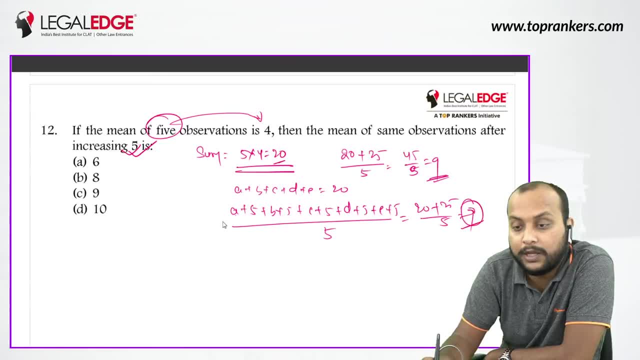 is 20 and 5 times 5 is 25 by 5, that is equals to 9.. Some people might have done the same Right, But this is not needed. Questions could have been solved directly If the average of the observation is 5,. 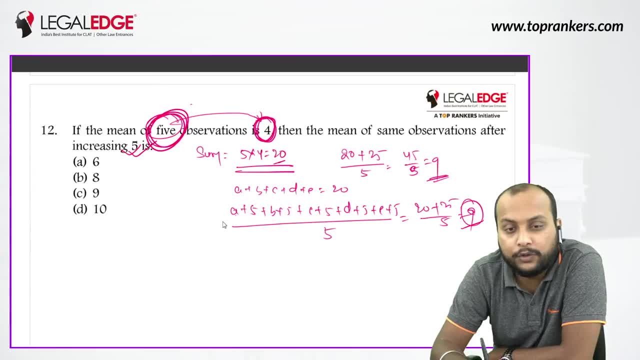 then its average is 4.. If I increase all the observations by 5,, then increase the average by 5.. This is the method, This is the rule of the average, Or you can say that this is the funda of the average. 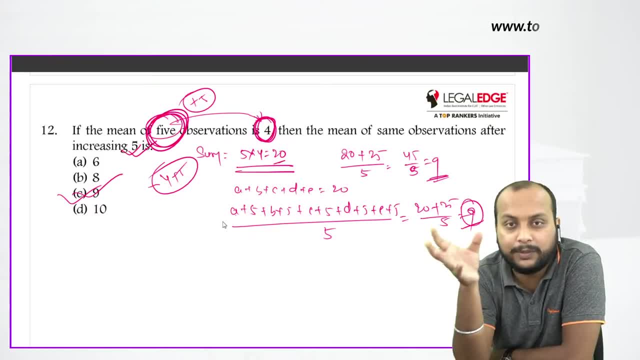 What you can do is if all the numbers have increased by a constant number, then the average will increase by the same number. No doubt about that. If the observation has increased by n, then the average also increased by n. Right, If we have increased all the observations by n. then the average will also increase by n. If we have increased 5 observations by 4, then if we have increased 5 observations by 5, then the average will also increase by 5.. There will be no difference in that Right. 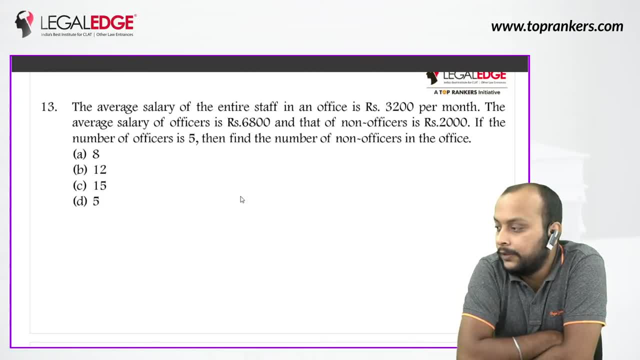 Now the fourth, third, thirteenth, Yes, yes, Sita. correct, This is the rule. You can also call it funda. You can also say that if all observations are increased by one particular number, then we can directly increase the average by the same number. 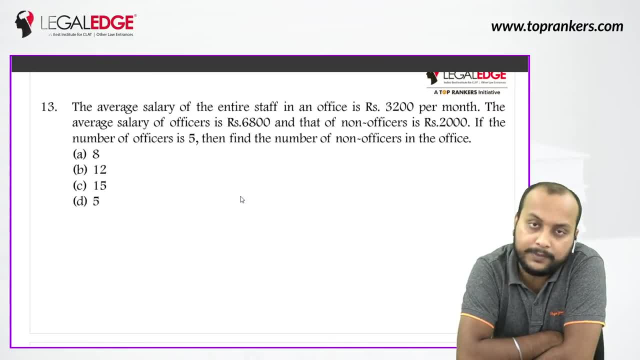 And even if you have not increased by the same number, then divide the increase and add it to the average. This also happens. I will tell you what method it is. It is also easy. It is easy, Suppose. I will tell you what method it is after explaining this. 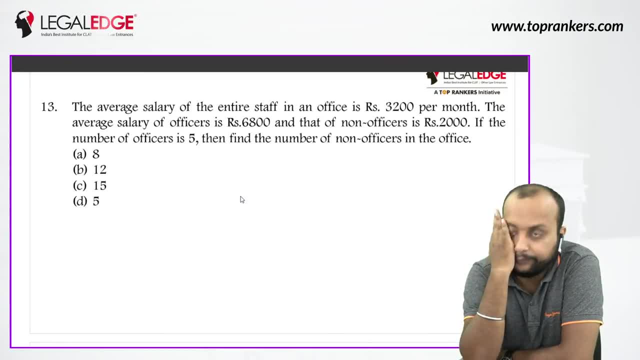 Yes, that is right. That is right Anyhow. the second explanation is: if you have increased the average by 5 or more, you can also say that if you have increased by 5, by 10, then you can add this. 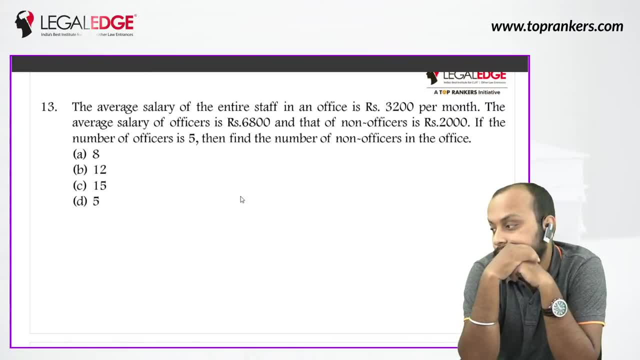 Yes, yes, that is correct. Next, if you have increased the average by 4, then, in addition to this, if you add this to the total number, you can say that you have increased the average by 5, and because the number of observations is reduced. 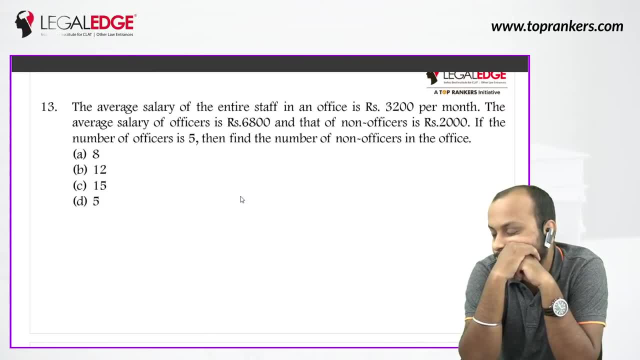 you can also say that you have increased the average by 5.. With this we can say that I am using both the languages- English mostly because I know his parents from Pan India are joining here, So don't worry about that. Mostly question in English. 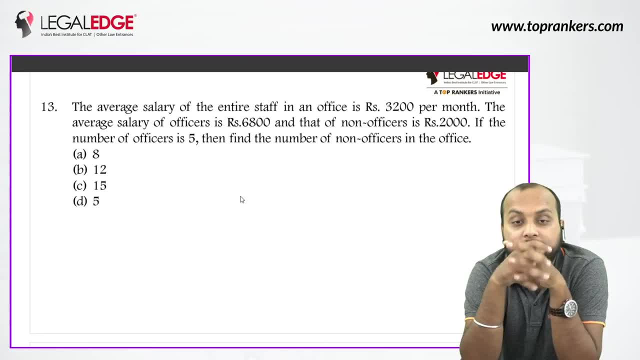 The correct answer for question number 30 is what the average salary of the entire staff is. The average salary of officers is 6800 and non-officers is 2000.. If the number of officers is 5,, then find the number of non-officers in the office. 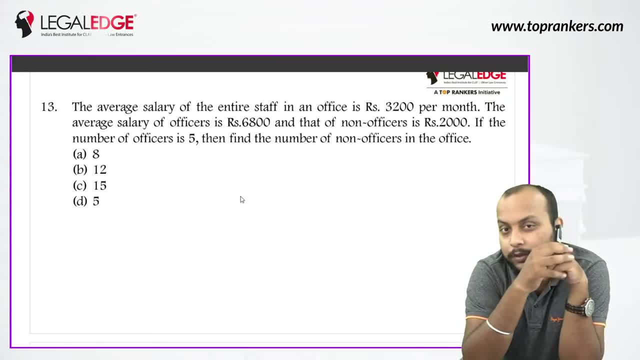 Now there are two methods to solve this problem. The first one is equation based. Mostly, you have applied the equation method, but the correct way and easiest way to solve this question is to apply with the allegation method. So how many of you have used the allegation method to solve this problem? 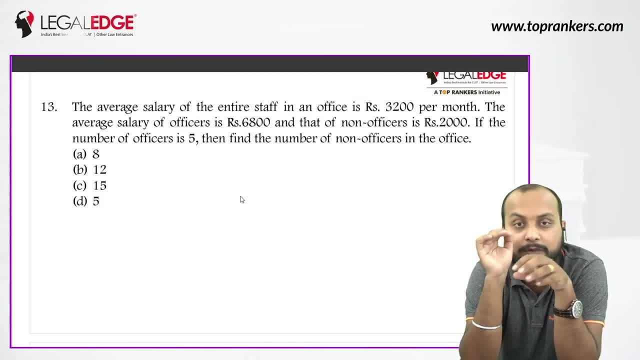 Because, with the help of allegation, this question has been solved within a second. So how many of you have used the allegation method to solve this problem? So how many of you have used the allegation method to solve this problem Within 10 or 15 seconds? 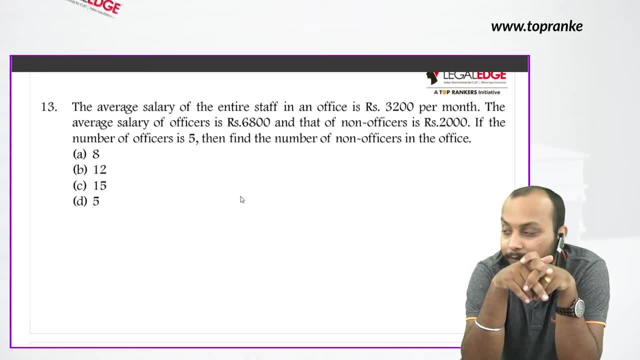 Not a second within a 10 or 15 seconds, but with the help of equations. But it's easy. Making with equations is also easy, but if I go with the allegation method, so to make with allegation is quite easy as compared to making with equations. 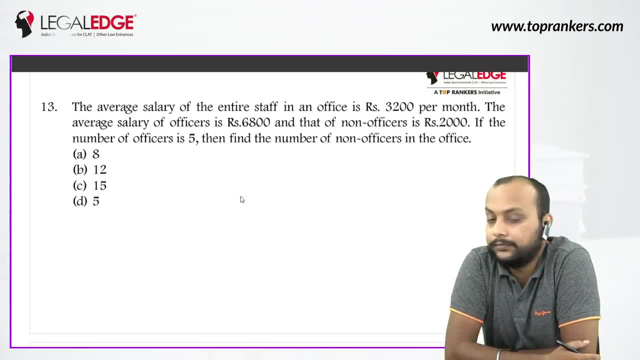 See Overall average is 3200 for officers and non-officers. Officers average is 6800 and non-officers average is 2000.. Officer- non-officer officers value is 6800 and non-officer is 2000.. 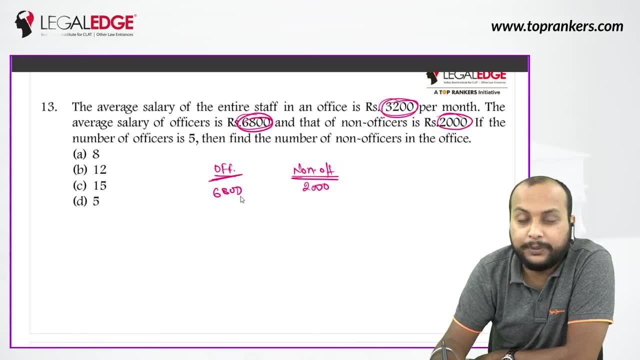 If we add both the values, the entire staff average is 3200.. How much is the average? 3200.. 3200. Use delegation: 3200 minus 2000 and 6800 minus 3200.. How much is this? 1200.. 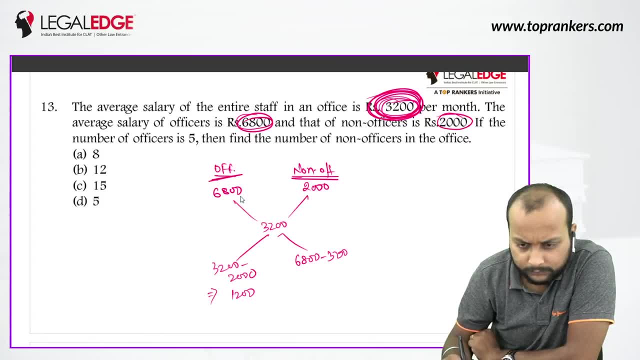 And how much is this? 3600.. So ratio is 163.. Ratio is 163.. Officers are 5.. So 5.. So, officer upon non-officer: How much is the ratio 1 by 3.. How much is the value of officer 5.? 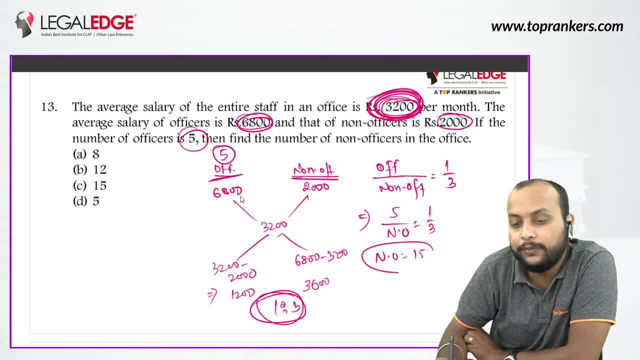 Non-officer has taken out the value, So non-officer's value would be 15.. So option number C- Allegation method, is always easy as compared to conventional method. Conventional method- The topic based conventional methods- are no doubt easier than our allegation methods. 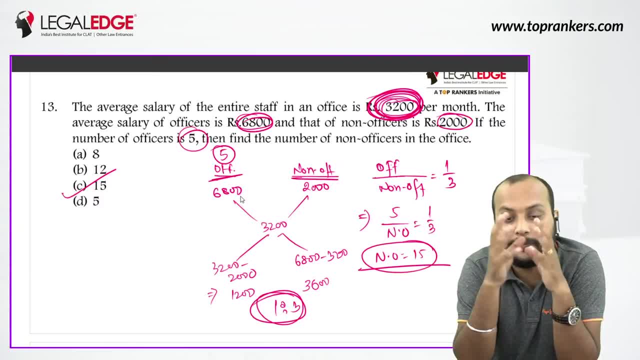 But allegations should be applied. We have to All the concept in allegations. If you apply wrong allegation it will be wrong. There are some requirements of allegation I have discussed in the class. Let's move on Now, move to the question number 14.. 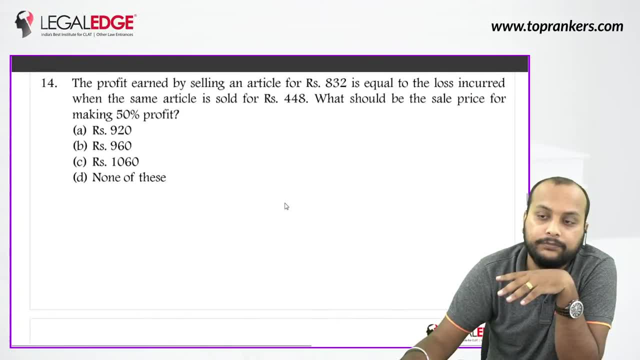 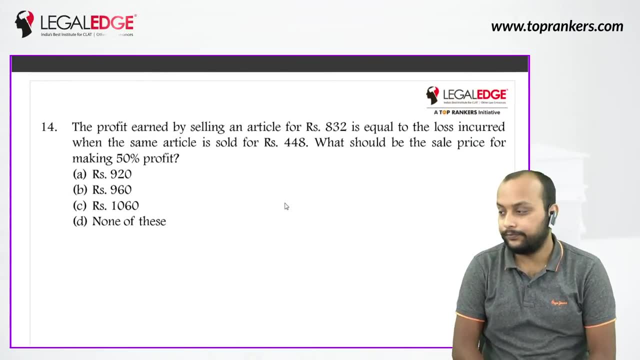 In this class, you have to Duncan At 2020,. will the syllabus change, Mona? Yes, there is news. there is a notification. the consortium has released something an institute has conveyed to you, or you have received this knowledge from the University of Watsip. it depends. 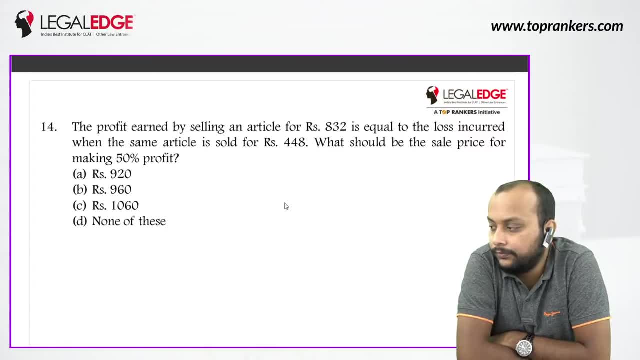 Answer for question number 14,. the profit earned by selling an article for RS 832 is equal to the loss in accord, when the same article is sold for piece 448,, what would be the selling price for RS 832?? The profit earned by selling an article for RS 832 is equal to the loss in the same article. what will be the selling price for RS 832?? 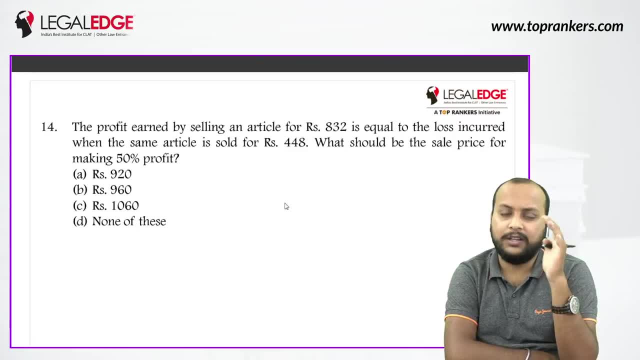 Let the cost price equal to x. let the cost price equal to x. let the cost price equal to a conventional method. So what is the profit here? The profit we got here is 832 minus x. Then the cost price is this much. so what is the loss of this? x minus 448.. 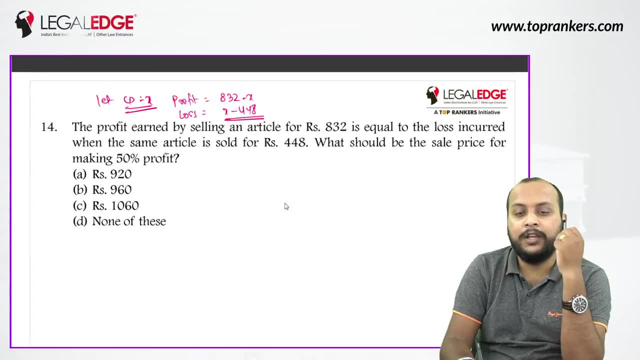 This is the loss. if you have given 448, 832 is the profit, you will equate both. the cost price will come. Don't do this. don't do this at all. How to do it again? See, whenever you see a question like this where you have given that selling an article 832,. 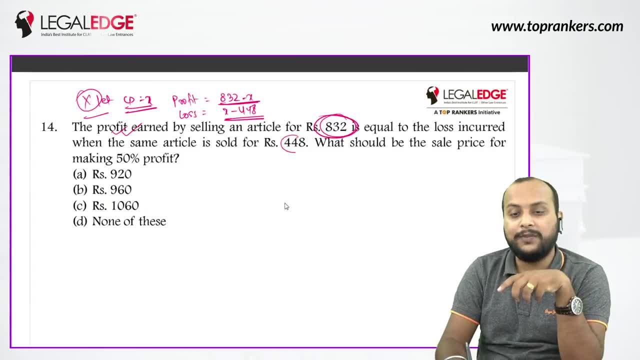 How to do it again. See, whenever you see a question like this where you have given that selling an article 832, you are getting a profit and selling the same article at 448.. You can change the digit, you can change the numbers. 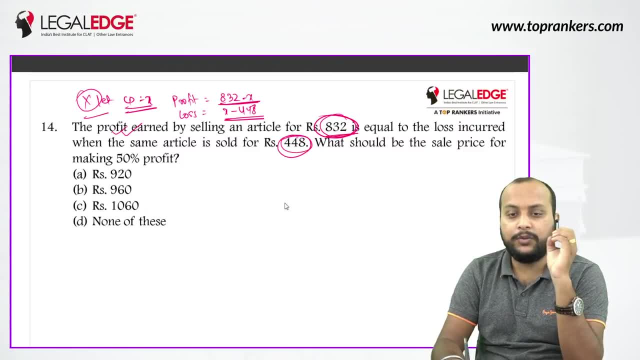 You can change the digit, or 832 or 448, you can change the value of these, But if you give that the profit you have earned, the same loss you have incurred. both are equal, Profit and loss. if you take out the direct CP, how will you take it out? 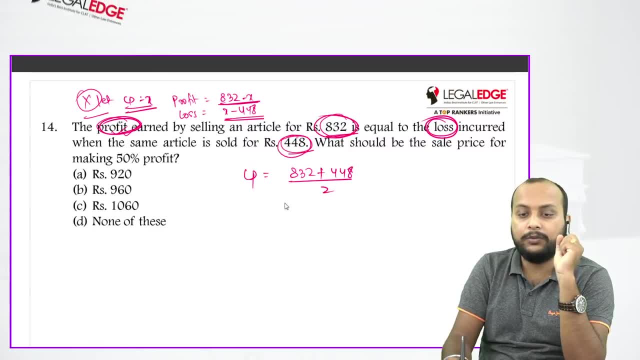 Take out their average: 832 plus 448 divided by 2, that is your CP. If you calculate this value, will come check how much it comes: 1260, right? 1260 divided by 2, how much will it come? 630.. 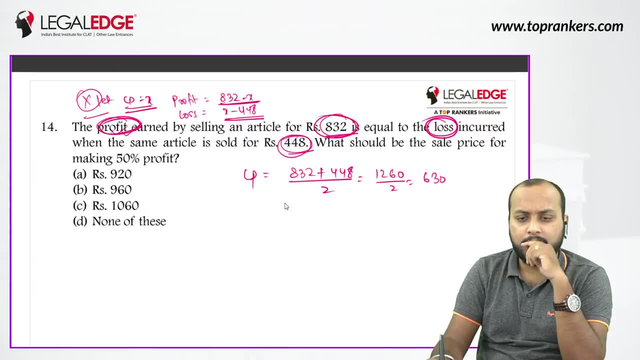 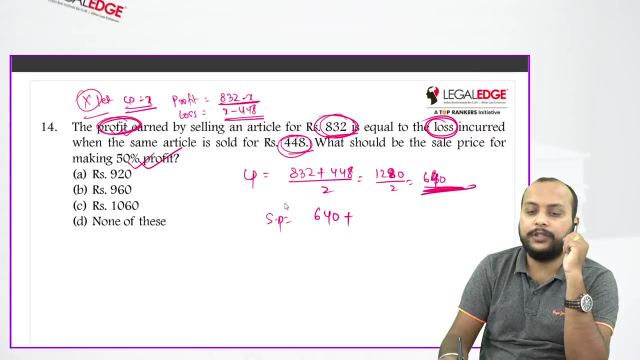 How much will it come? 80 will come, 640.. 1280. 640, cost price has come. You have to sell at 50% profit. how much will be the selling price? It is 640 plus 50% of this. so how much is 50% of 640? 320,? the answer would be 960,. option number B: 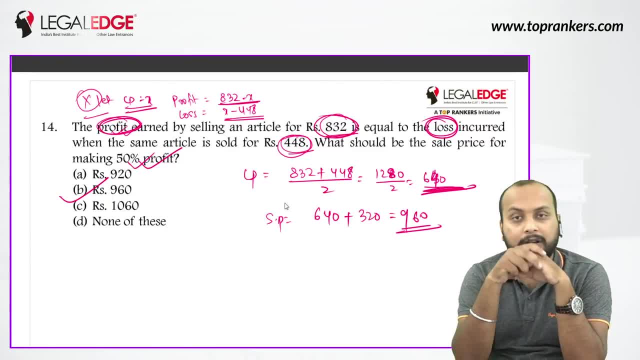 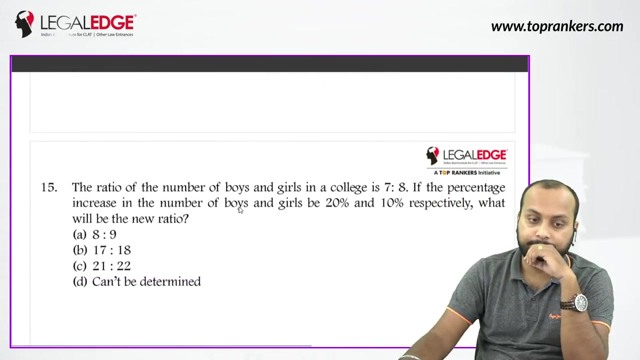 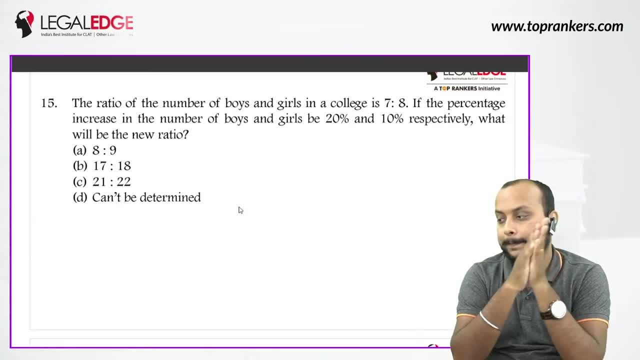 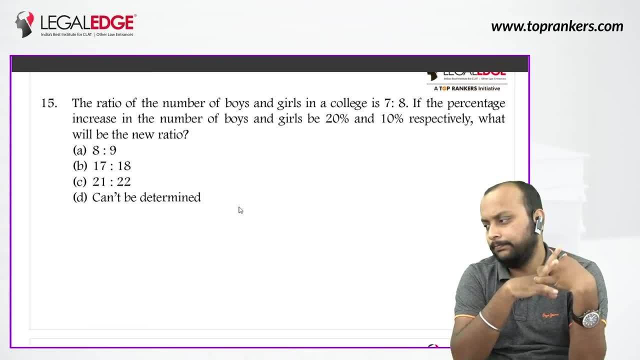 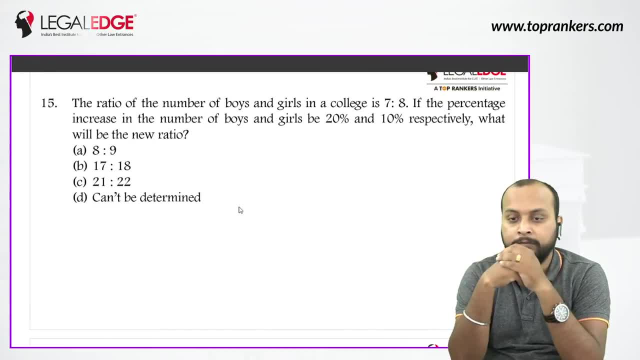 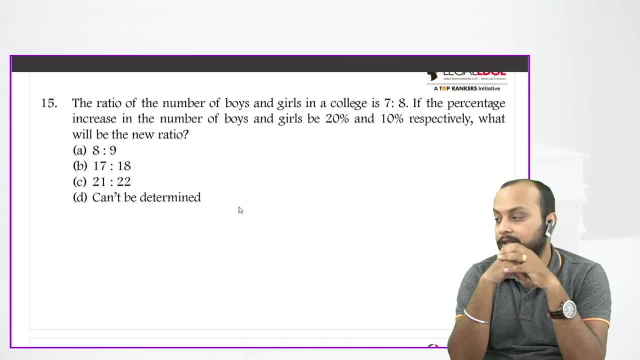 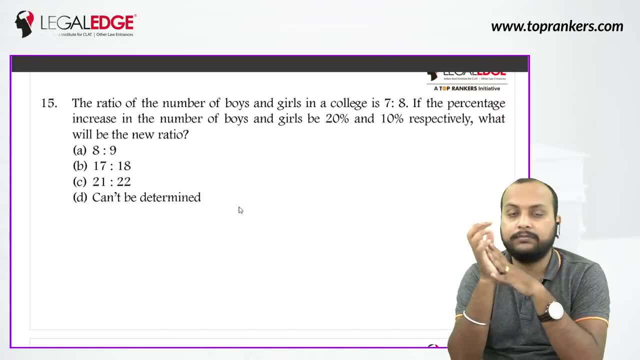 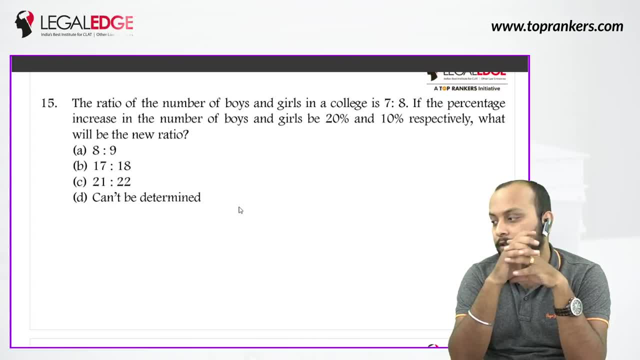 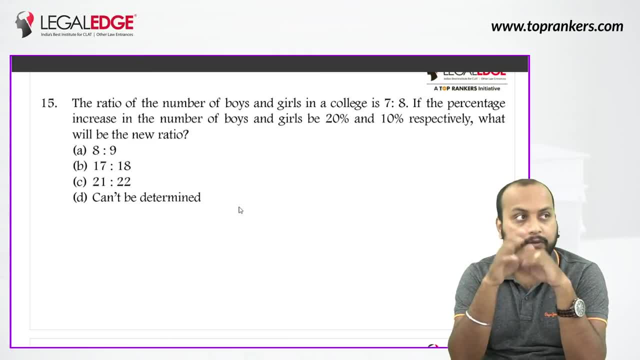 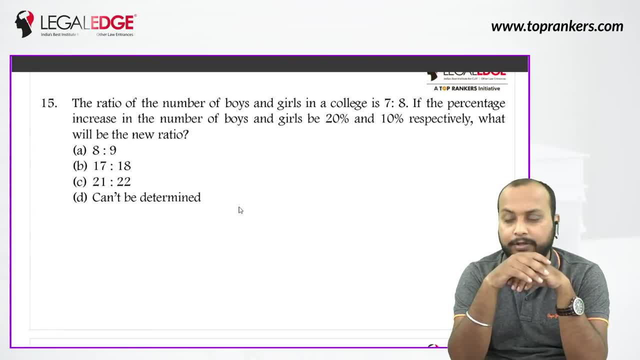 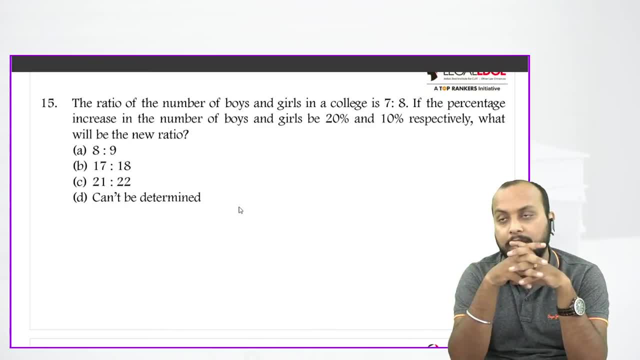 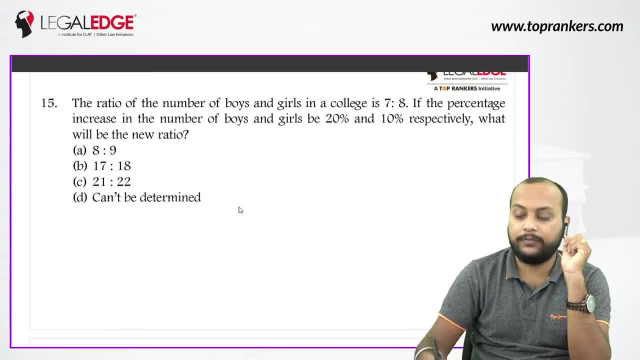 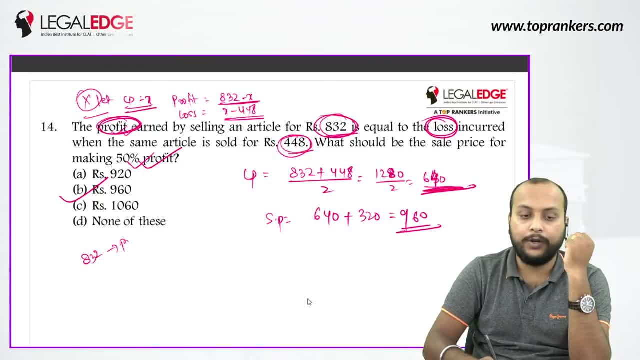 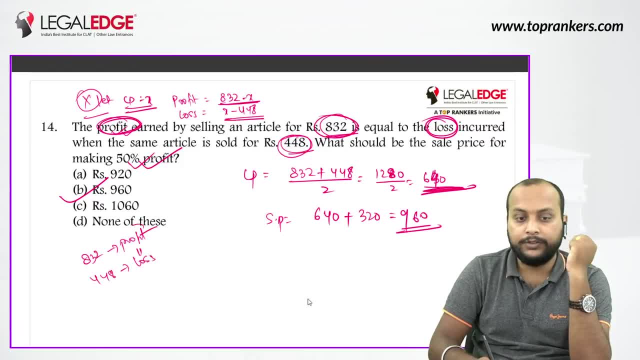 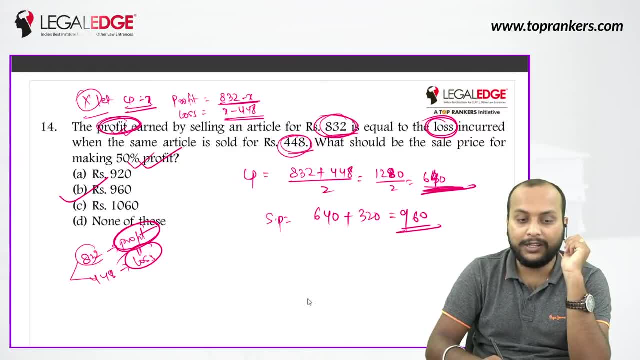 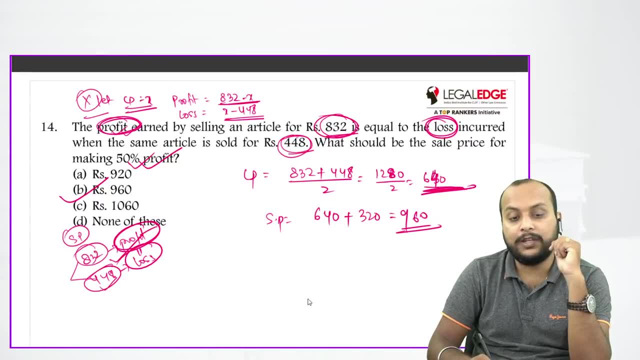 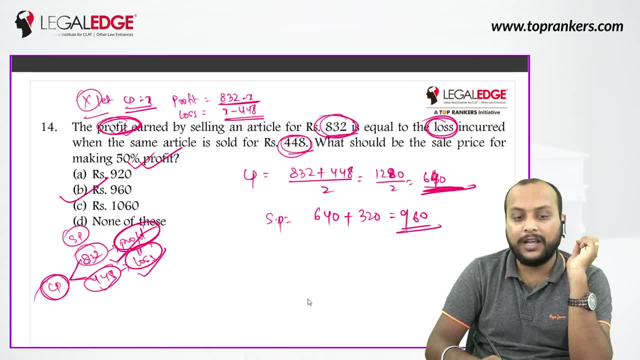 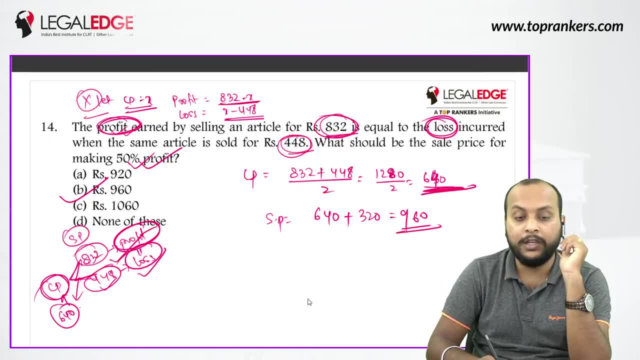 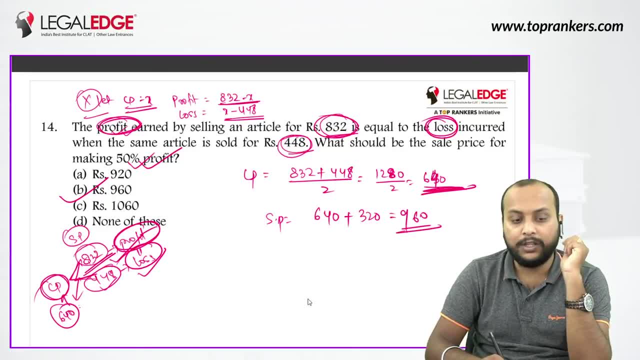 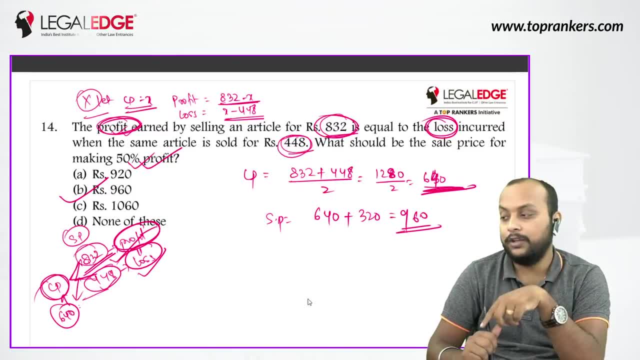 So option number B is the correct answer. So option number B is the correct answer. So option number B is the correct answer. So we will just take out the average from it. Now for the question number 15,. what will be the answer? 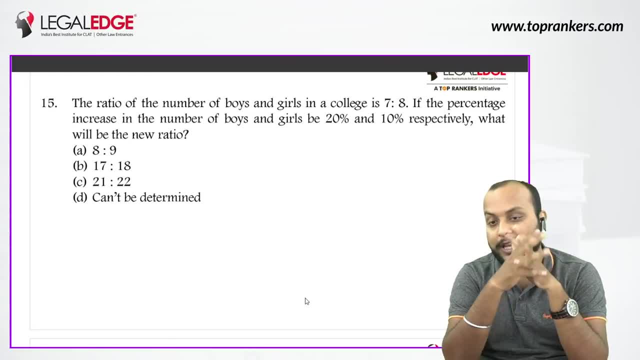 The ratio of the number of boys and girls in the college is 7 is to 8.. If the percentage increases the number of boys and girls, 20 and 30, 10. What will be the new ratio? Similarly, D is incorrect answer. The correct answer is C: 21 is to 22.. 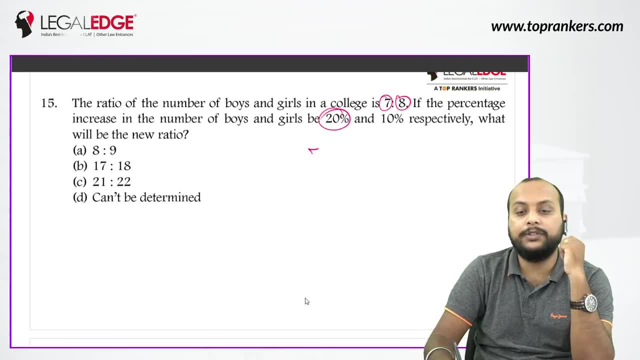 See, it is easy: 7 is to 8 is 20%. Increase the ratio of 7 to 20% And increase the ratio of 8 to 10%. What will be the increase of 7 to 20%? If you increase the ratio of 7 to 20%, it will be 8.4.. 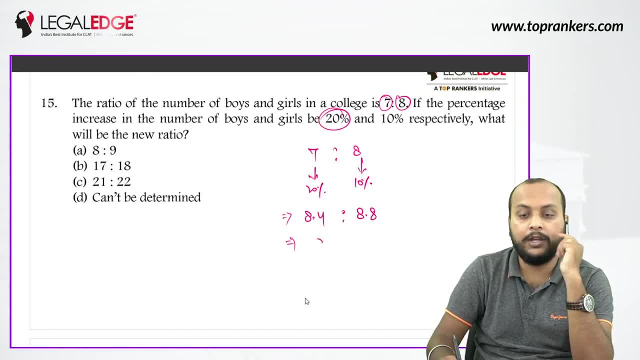 And if you increase the ratio of 8 to 10%, it will be 8.8.. So what is the ratio? 84 is to 88. This is not a standard ratio. What is the standard ratio? Smallest integer. 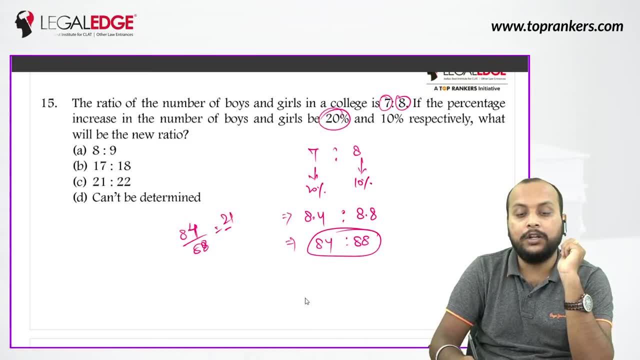 So 84 is to 88.. What is the smallest integer? 21 is to 22.. Option number C. Option number C is the correct answer. Option number C is the correct answer. See, it is easy. So let's have a 10 minute break. 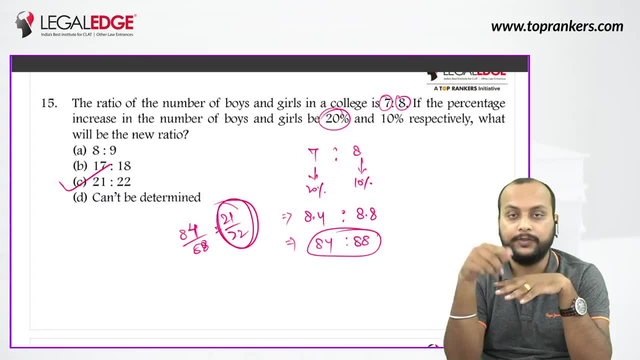 And we will back after 10 minutes to continue with this session. And now we have got questions. Now we are going to do some more questions. in 1.5 hours, 15 questions more. So we will do after this 10 minute break. 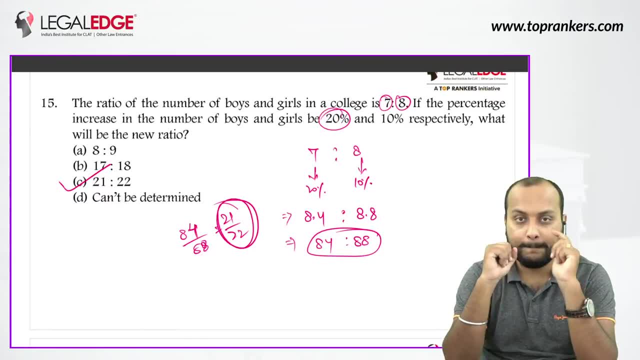 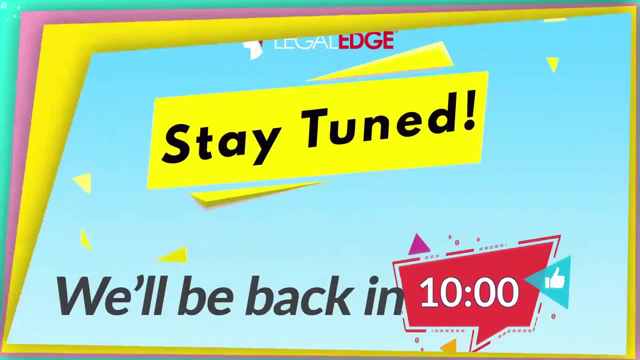 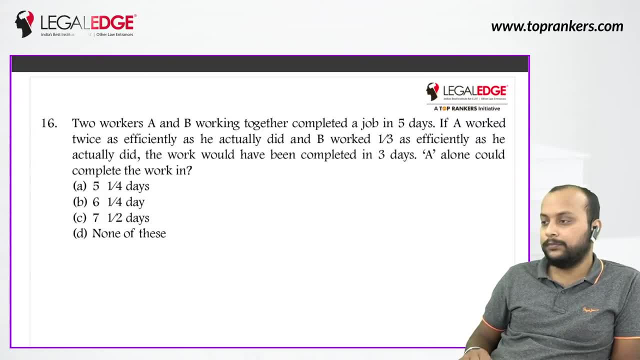 Two workers, A and B, working together, completed a job in five days. if A worked twice as efficiently as he actually did and B worked one by three, as he actually did, the work would have been completed in three days. A alone could complete the work. in how many days? okay? 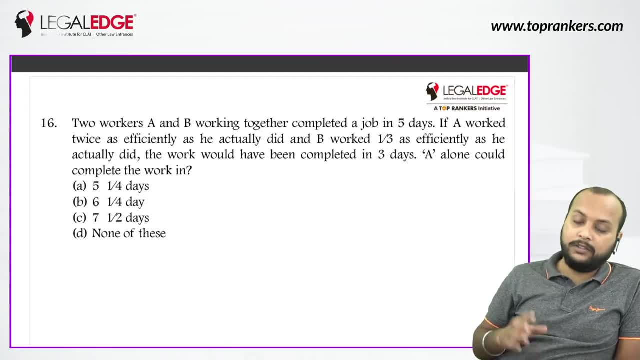 I have written a clarity paper. now hold it and sit. tomorrow the result will come as it came in the notification in the calendar. see why I am so worried about it. focus on the coming paper. what has happened has happened. Ravi Singh 91.75. tomorrow we will see what happens. 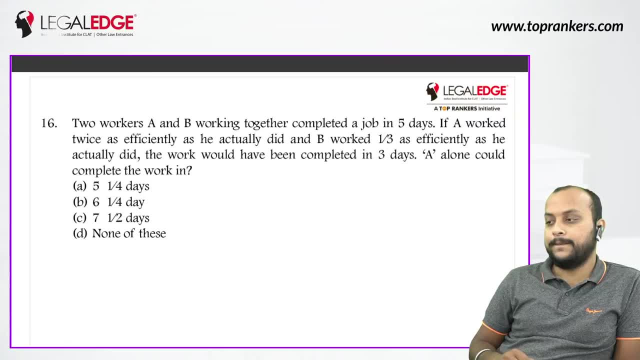 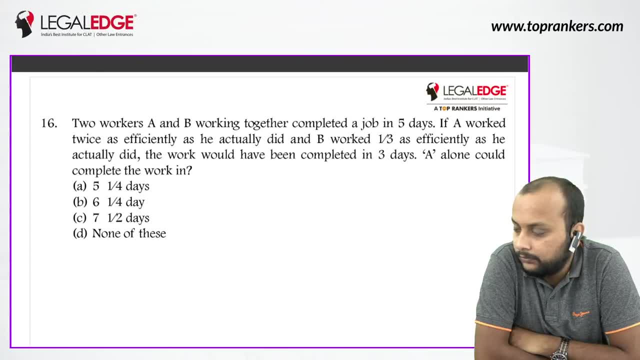 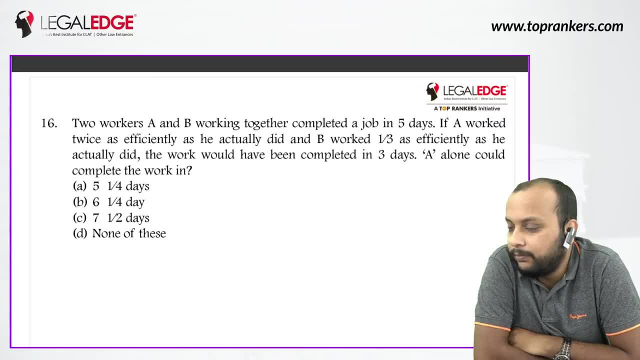 Shankar is saying 6 is to 1 by 4.. Poonam is saying 6 is to 1 by 4.. by 4.. Okay And quickly, quick answers. It's easy, It's common work based. 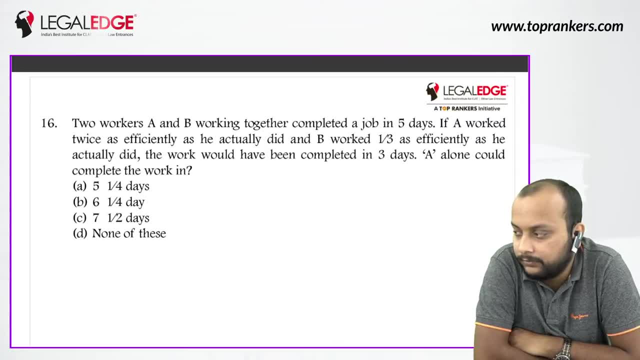 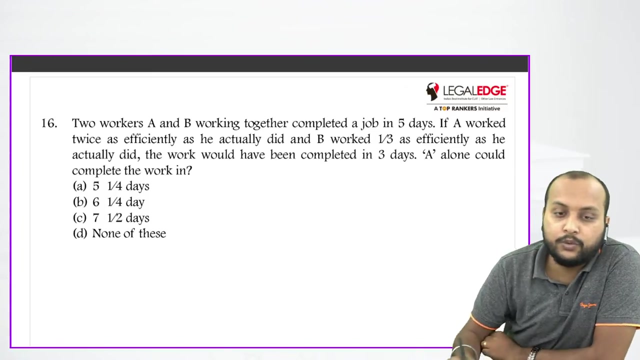 Thank you, You can watch it tomorrow. Now let's focus on the next paper On our elite. Okay, Let me tell you how to do it. Two workers, A and B, working together, completed job in 5 days, So let A one day work. 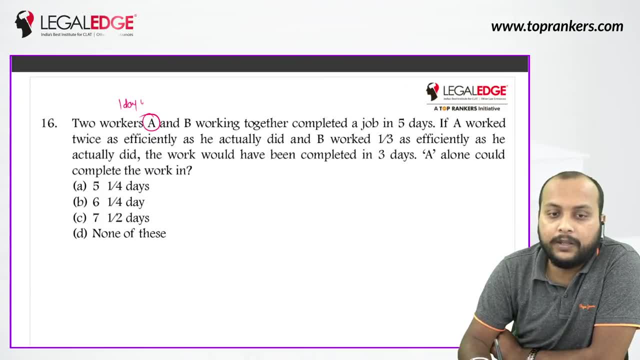 is X. I took A. one day work, I'll take A. only If it's A, I'll take A. And what do I take for B? one day work- One day work, I'll take B. Both of them will work together. 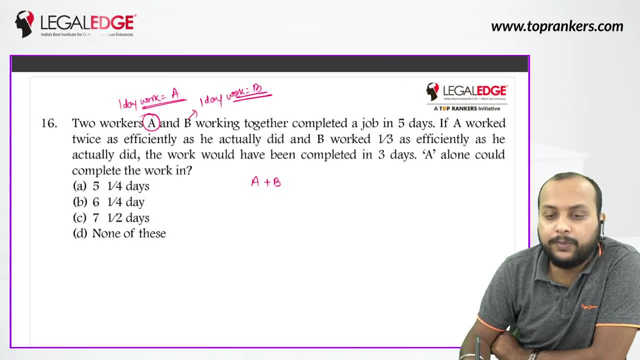 So one day work of A is A, One day work of B is B. If both of them work together, then how much work is there 1 by 5.. Because work is being completed in 5 days. So when work is being completed in 5 days, 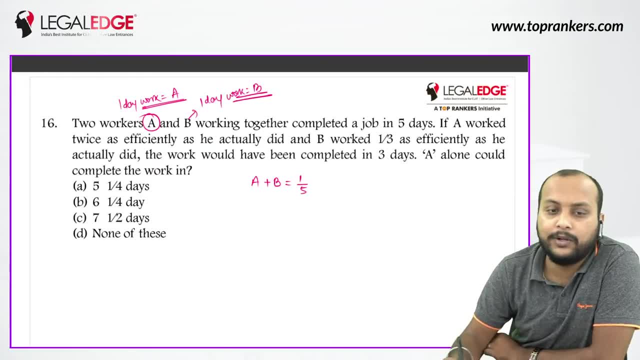 then how much work will be done in one day? 1 by 5.. Next, what did you say? A worked twice as efficiently, So A worked twice as efficiently, So 2A. The efficiency was one day work, So A was A. 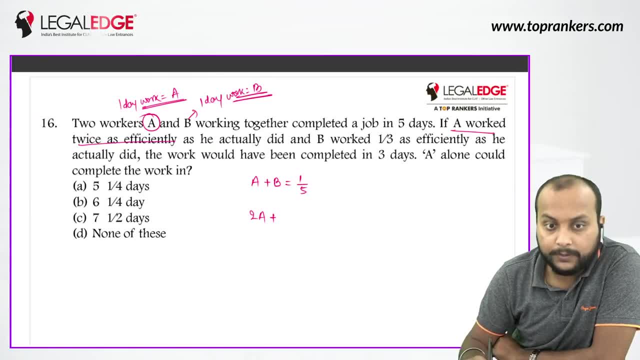 So how much work was done in two days? 2A, 2 into A And B worked one-third, So B worked one-third, So B by 3.. He actually the work we have completed 3 days. So what will happen? 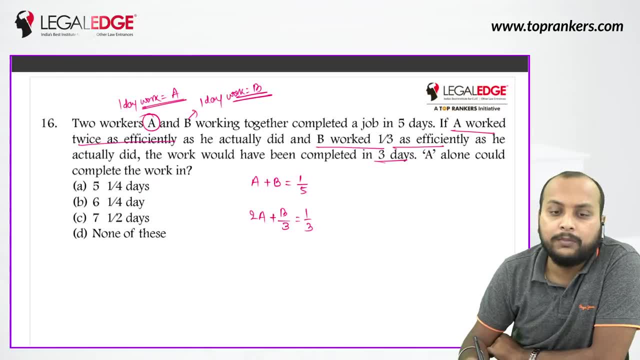 1 by 3.. Solve both of them. Take out the value of A and B. I was asked for the value of A Eliminate B. I was asked for the value of A Eliminate B. Multiply it by 1 by 3 and minus it. 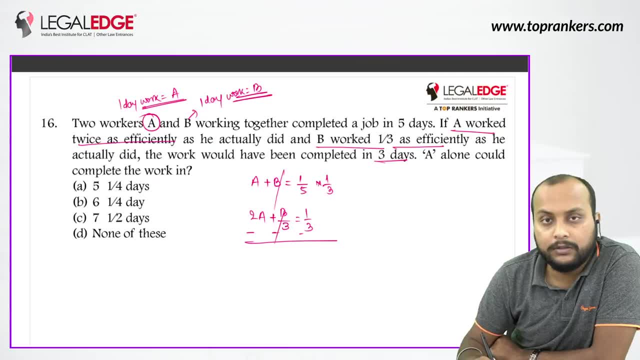 So what happened to B and B? It got cancelled out. Eliminated B and B. So what happened to E? It got eliminated. So what happened to A by 3? What happened to this 2A? So what we have? 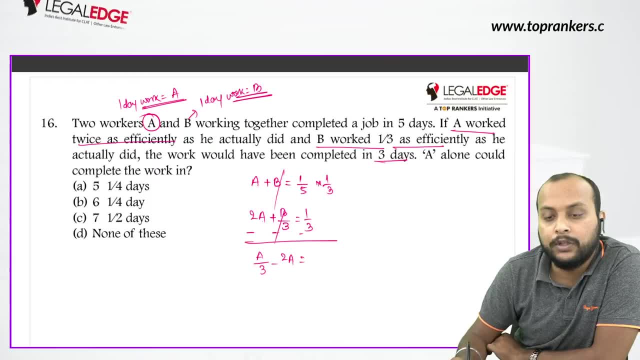 A by 3 minus 2A Equals to What is this? 1 by 15 minus 1 by 3.. See it got negative, But minus minus gets cancelled out Here. what happened? A minus 6A upon 3.. 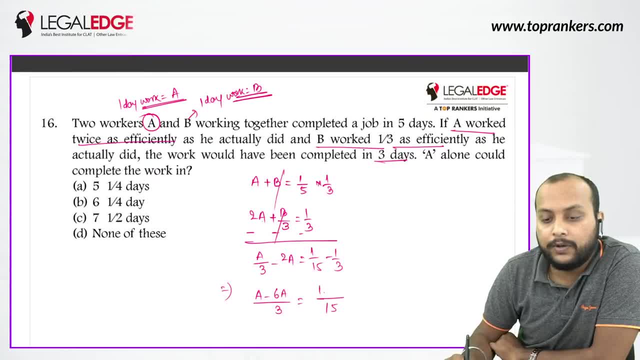 That is equals to What is this? 15 will be its LCM And 1 minus 5.. Calculate What will happen: Minus 5A upon 3 equals to Minus Minus 4 upon 15.. 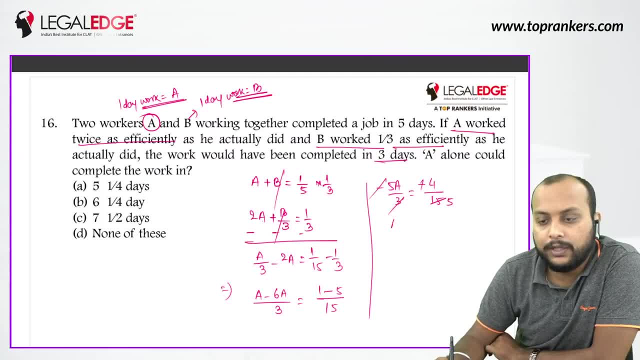 Minus and minus gets cancelled out. 3 goes to 5.. So what is the value of A? 25 by 4. That is equals to 6, is to 1 by 4.. 4 by 25 will come. 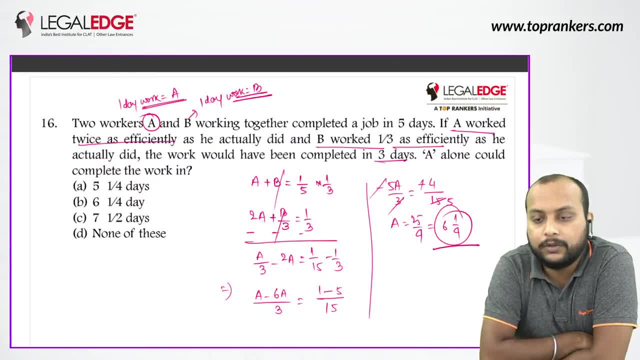 What will that be? Okay, If you take it out from here, it will be something like this: Multiply it, It will become 25 by 4.. What is this 1 by 4.. What is this 1 by 4.. 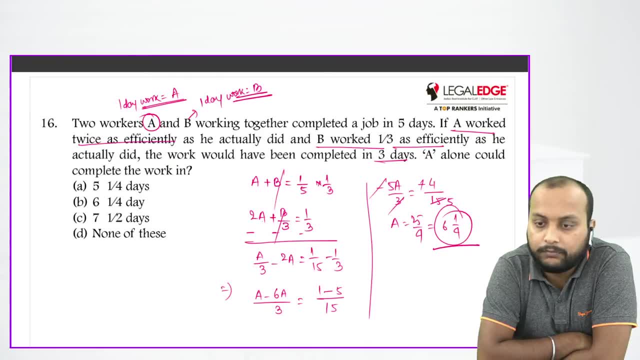 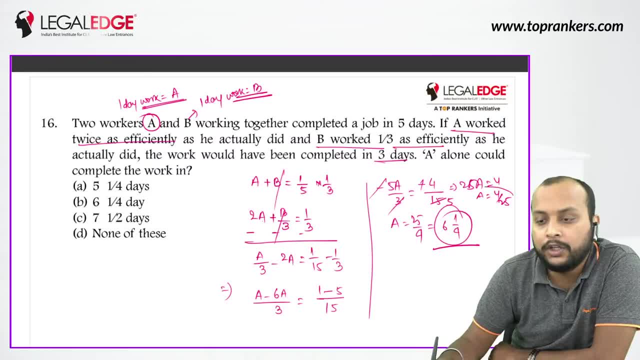 So A equals to 4 upon 25.. So A is one day work. So what is the total day's 25 by 4? that is equals to 6, is to 1 by 4.. Option number B. So correct answer is B. 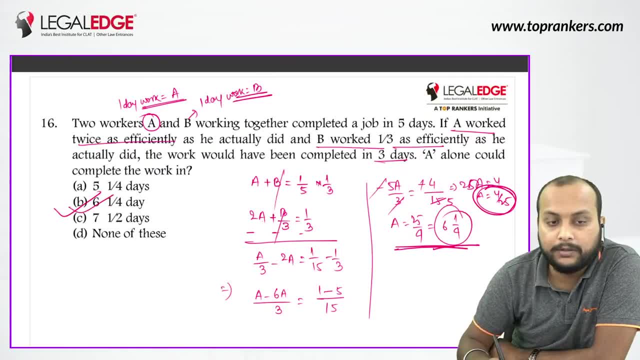 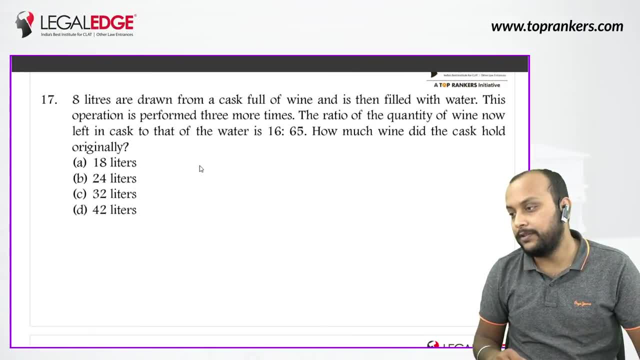 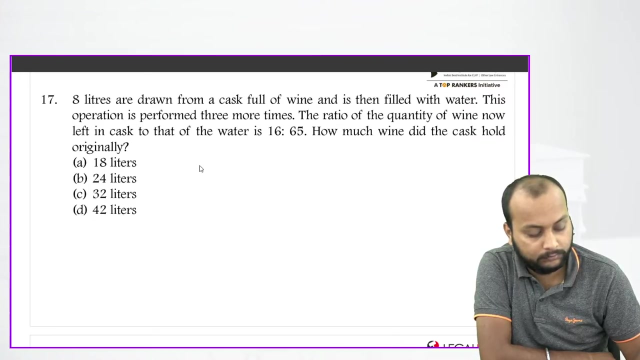 Mixture Mixture, Mixture, Mixture Mixture. Thank you, You answer. Eight liters are drawn from a cask full of wine and is filled with water. This operation is performed three more times. The ratio of quantity of wine now left in cask to that of water is 16 is to 65. 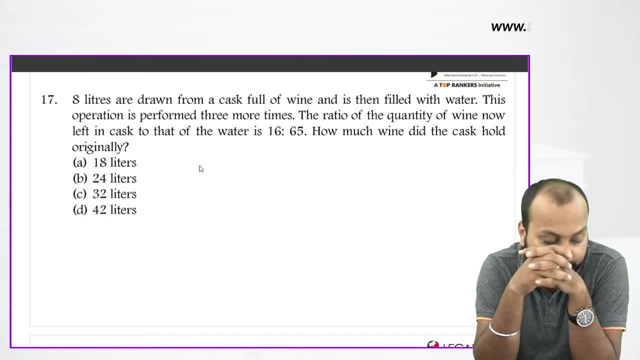 How much wine did the cask hold originally? The ratio of quantity of wine now left in cask to that of water is 16 is to 65.. Will you answer? Shall I discuss, Or are you trying? Shall we Let's discuss. 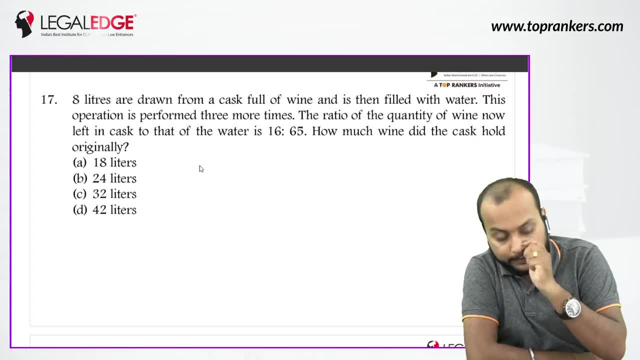 Okay, Eight liters are drawn from cask. Now, understand this question. I will give you a small example. You have a cask. This is full of wine, And how much wine is this? I don't know. Let's say 100%. 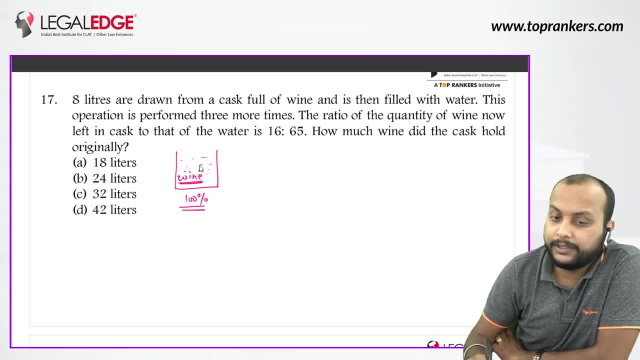 This is 100% wine. Let's assume this is 100 liters. This cask is fully filled with 100 liters of wine. Now I have taken out 8 liters of wine from this cask. So what is left in this cask? 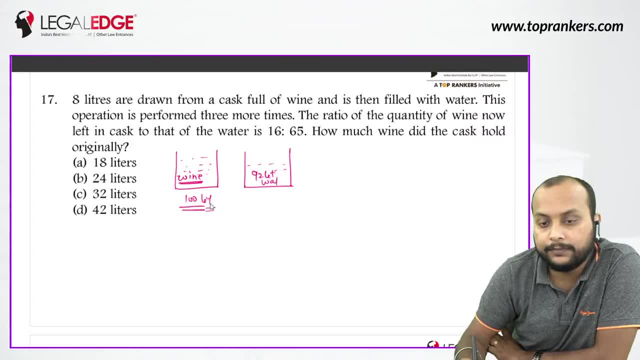 92 liters of wine is remaining. 92 liters of wine, 92 liters of wine. Now you have taken out 8 liters of wine. What did you add in this? 8 liters of water. So we added 8 liters of water. 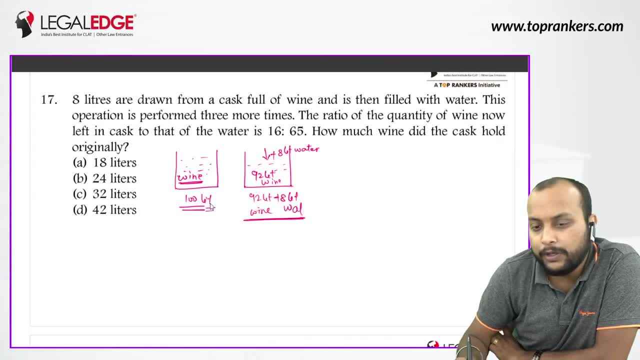 So here we got 8 liters of water. What is the difference in volume? Here the volume is 100 L. here also, the volume is 100 L. What is the difference? In this 100 L, you have decreased the total out of total, ie the concentration of wine. 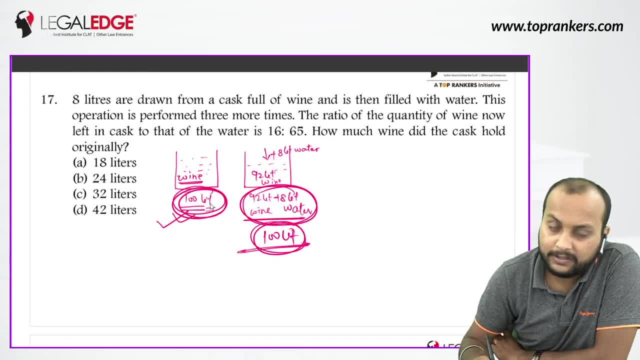 First of all, in 100 L the concentration of wine was 100% Total out of 100 was wine. But now the 100 L mixture is still there. The volume is still 100 L, But in that 100 L the concentration of wine decreases. 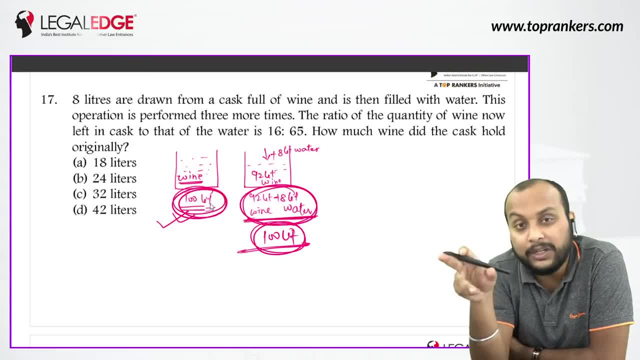 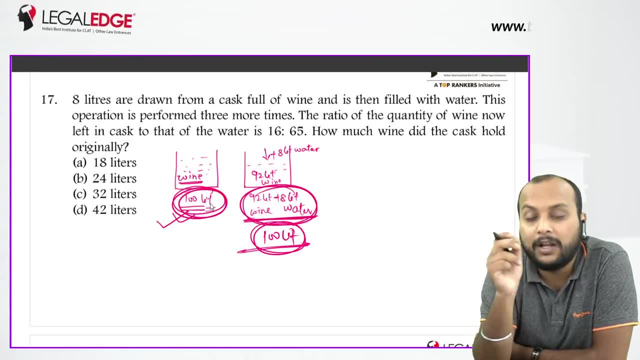 Concentration of wine now becomes 92 L, and previously the concentration of wine was 100 L. This is the difference, Why We took out 8 L of wine and added 8 L of water to it, But there is no difference in volume. 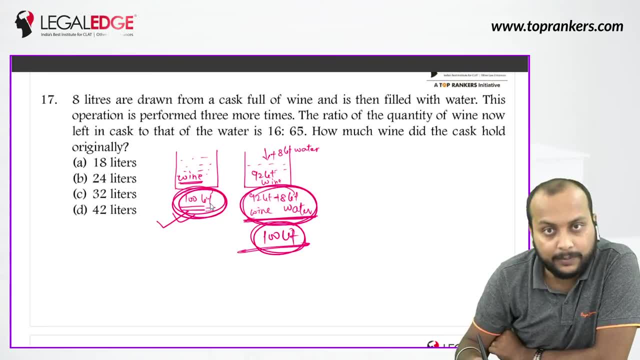 There is no difference in volume displacement. But there is no difference Here: out of 100 L, total. out of total, 100 L is wine. Here, out of 100 L, 92 L is only wine. So concentration of wine decreases. 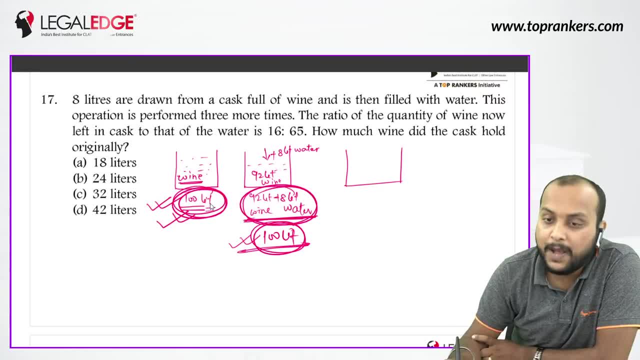 Again. if I do it again Now, here I have 100 L volume, in which 92 L is wine and 8 L is water. This is what we have. This is the 100 L mixture. If you now take out this 100 L, 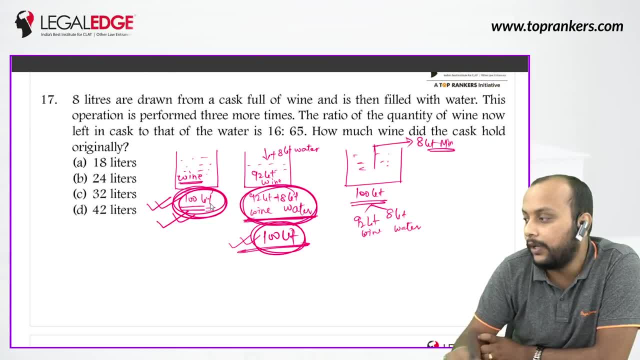 You will withdraw 8 L mixture. You will withdraw 8 L mixture from 100 L of mixture, in which 92 L is wine and 8 L is water. So this 8 L mixture will come out and not the wine will come out. 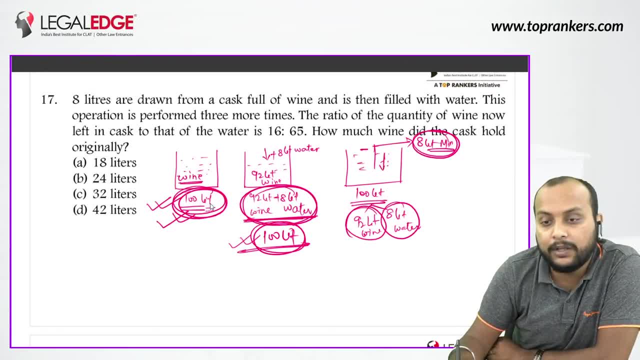 Right Now. again, you have added 8 L. This is minus and this is plus. You have added 8 L water, So again, its concentration will remain 100 L. Sorry. volume will remain 100 L, But concentration of wine will decrease again. 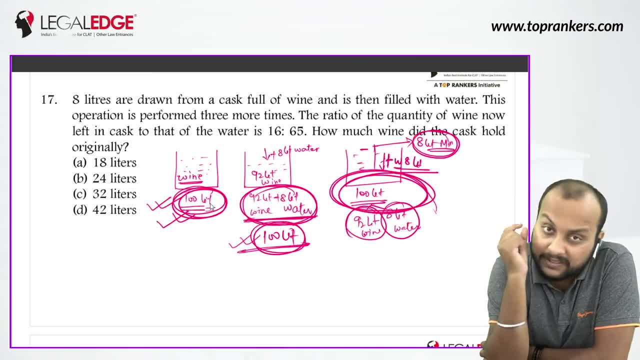 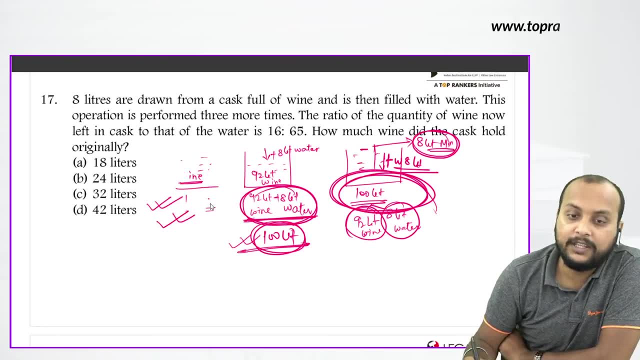 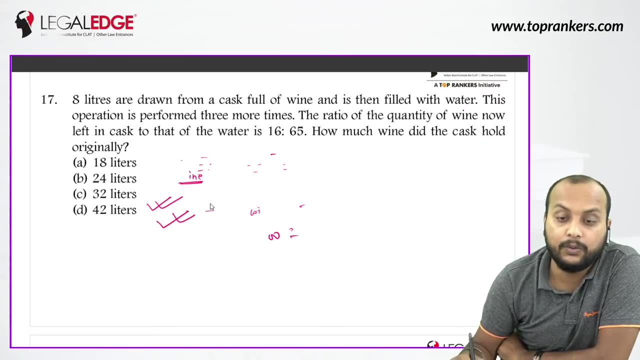 It will change. So only concentration decreases, Never volume decreases, Never volume decreases. What does it decrease? always Concentration decreases, Whatever is initially given to you In that case. So here, at last, we have a ratio given 16 to 65.. 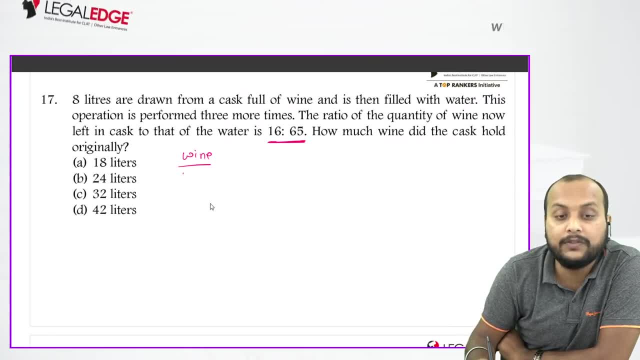 Whose ratio is given. We have given ratio of wine to water 16 to 65. Right, This means that now I have 16X of wine And now I have 65X of water. If I ask you what is the volume? 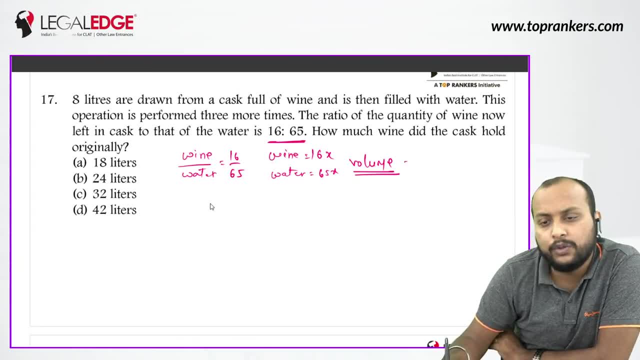 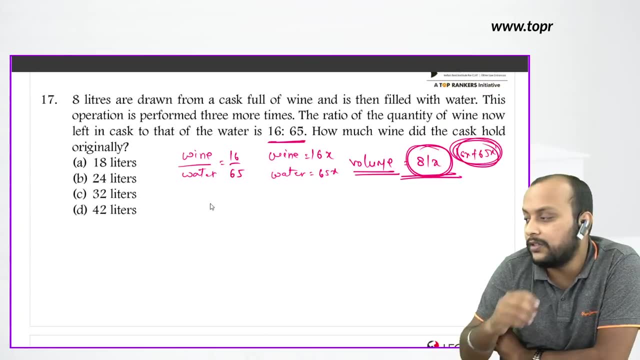 What will be the volume? What will be the volume after all the replacement? So I can say that the volume will be 81X, 16X plus 65X, Because these two things, These two things- 16X and 65X- are in the same cask. 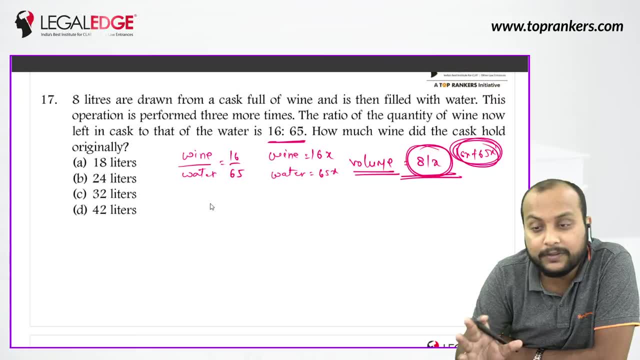 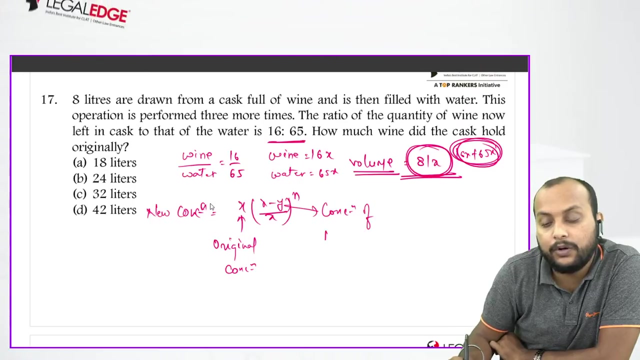 So the entire volume is 81.. Now understand. there is a formula here, Remember it Those who don't know. New concentration equals to X into X minus Y upon X is to power N. Where X is original concentration, Y is concentration of replacing material or element. 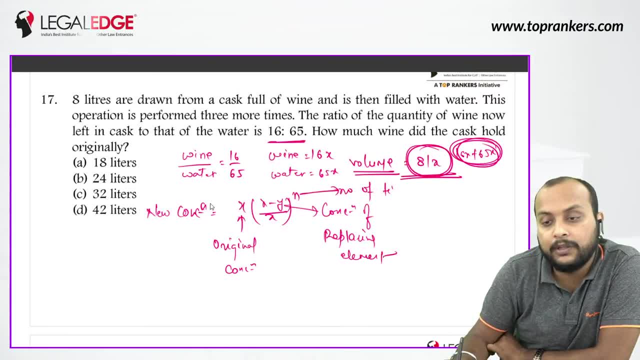 And N is number of times, How many times you are implementing it, How many times you are replacing it. Okay, We have given the ratio of wine and water. That means- I have taken it out- Wine is 16X And volume is 81X. 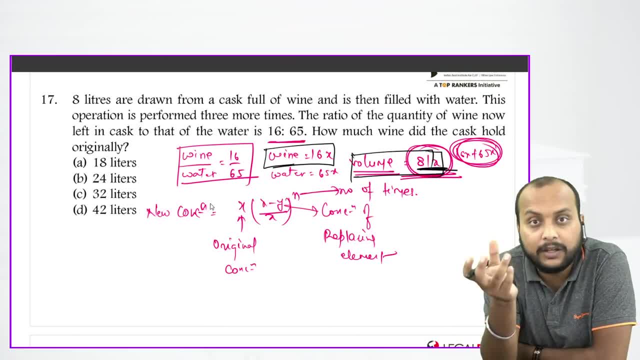 This volume will be the same, Which was wine in the starting. It will change at some point. The first example we took when we ordered wine. After making the cask We saw that the volume of water and the volume of wine is the same. 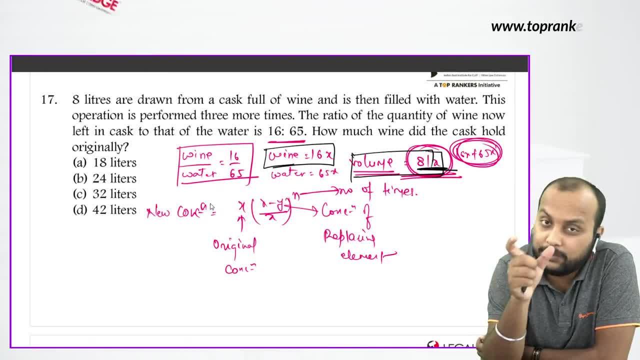 We are adding water by taking out the wine. So the amount of wine in the starting In the same volume, The same volume will be maintained. There will be no change in it. We can say that 81X In the starting. 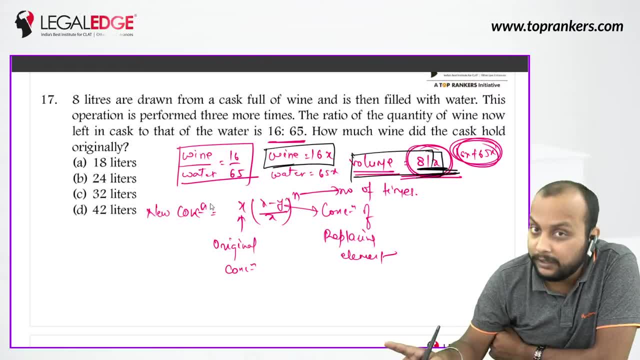 Out of total: 81 out of 81.. They are wine. They are wine. What will be? 81 and 81 in the starting. There will be wine After 4 times replacement, Because it did it once And 3 more times. 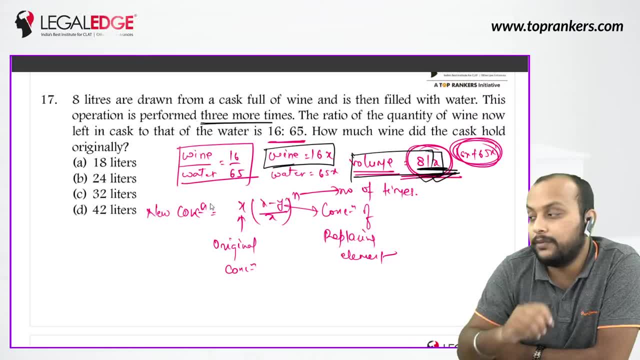 So it did it once 3 more times. So after 4 times replacement We will get 61X. Now here we have 16X, Because after water replacement we have 65X. Okay, So I have. 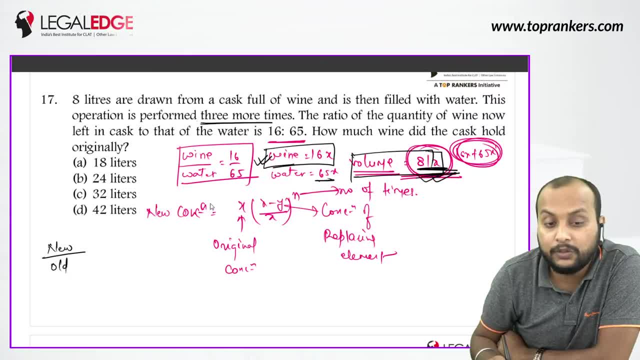 New wine upon old, If we have given a ratio in the starting 16 to 65. Okay, So in the place of this new by old, I take new by volume. If I take new by volume, So what I have. 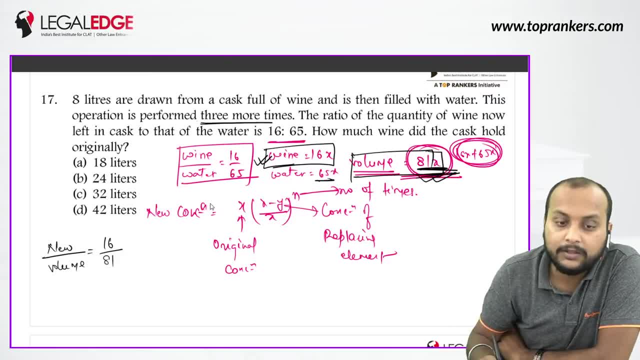 16 upon 81.. The X and the X will be eliminated. Write it down. Eliminate it: 16 upon 81.. What is the formula of new? X into X minus Y. So the formula of new is X into X minus Y by X power N. 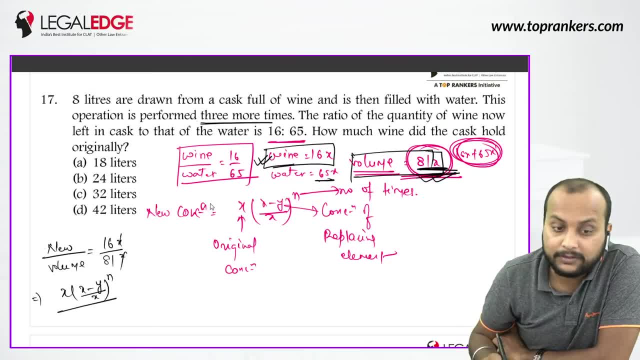 And what will be the volume in the starting Out of X? Total X will be. What is the value of this 16 upon 81.. What will be between X and X Eliminated? Don't know the value of X. 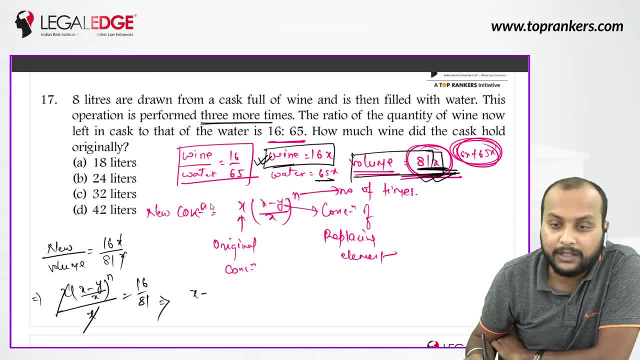 We have to calculate Y. How many liters of water are we adding? We have given something: 8 liters. So what will happen? The value of Y is 8. Divided by X. How many times did you do? 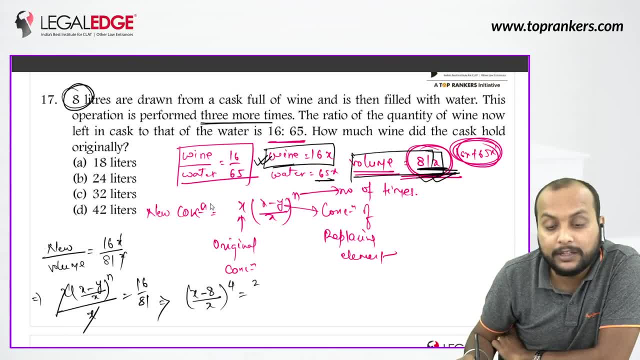 4 times. We can write 16 by 81.. 2 by 3 to power 4.. Base equal, Power equal. What will this become? X minus 8 by X equals to 2 by 3.. Hence, 3X minus 24 equals to 2X. 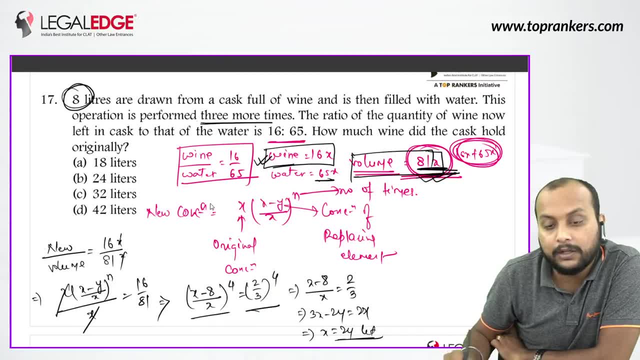 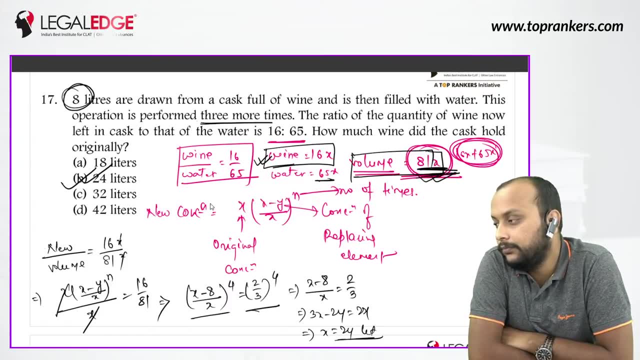 So what is the value of X: 24 liters. Option number B: The power of this ıyı. C, The power of this Y. So how many liters of water are we adding The volume in the starting? 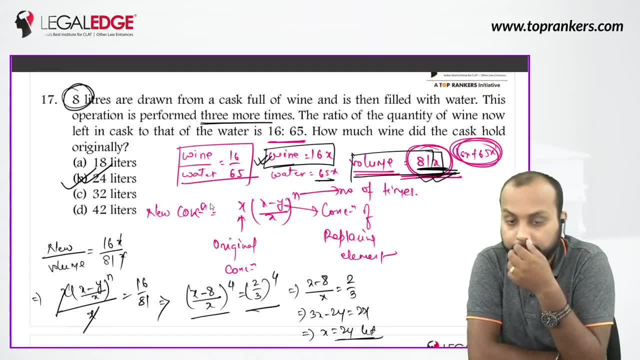 16 upon 81.. What will be the value of X Out of X? Total: No water: No water: 3 by 2 is equal to 2 X Divided by X. What will be the value of X? 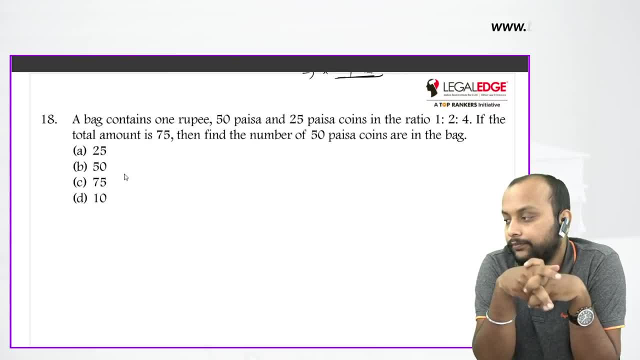 4 by 2.. Y you. You will make a comparison. it will be long, you will be confused because the ratio will be changed again and again. the first time you will make it with 100 liters, you will reduce it from 100 to 8, it will be 92 and 8, then 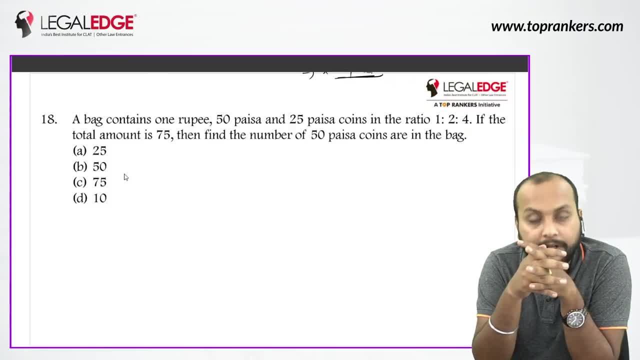 Then after that, if you take out the first 8 liters, then it will be something else. we can't do 84 and 60, because if you take out 8, both the wine and water will be drawn in it. So there it will be. suppose 85 point something and 14 point something. the ratio will be changed next time if you take out 8,, then the ratio will be changed again. 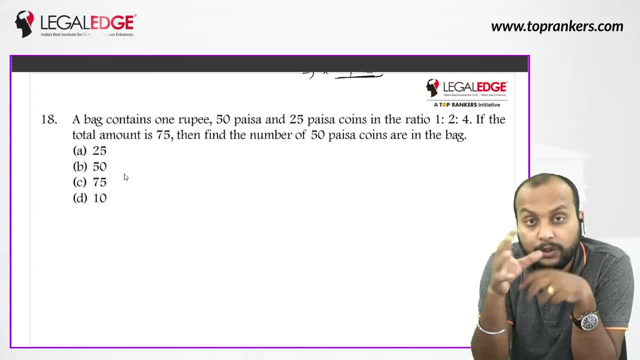 Exactly, 8 liters of wine will not come out. water wine, water wine. two will come out when we will withdraw the mixture from the second time. then it will be complex. So now option number. question number 18 will be answered quickly. 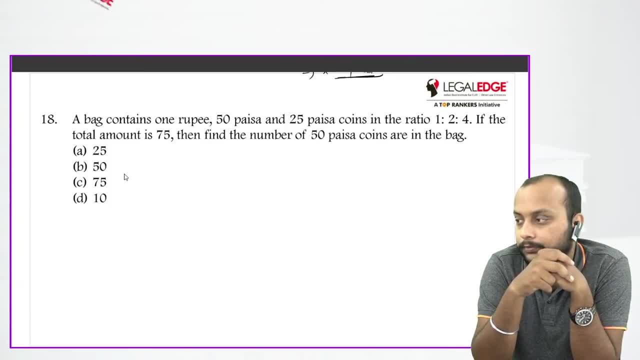 Thank you. The bag contains 1 rupees 50 paise and 25 paise coins in the ratio of 1 to 4.. If the total amount is 75, find the number of 50 paise coins are in the bag. 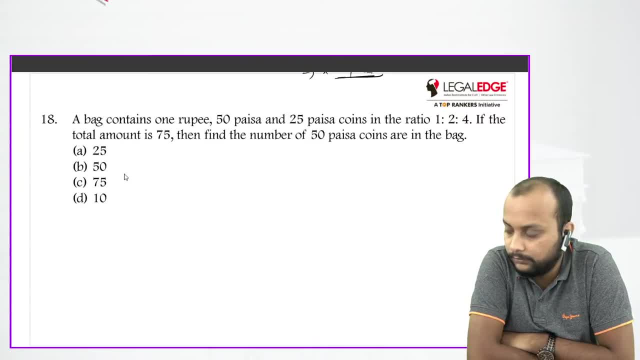 If the total amount is 75, find the number of 50 paise coins are in the bag. If the total amount is 75, find the number of 50 paise coins are in the bag. 4 times the add, See. 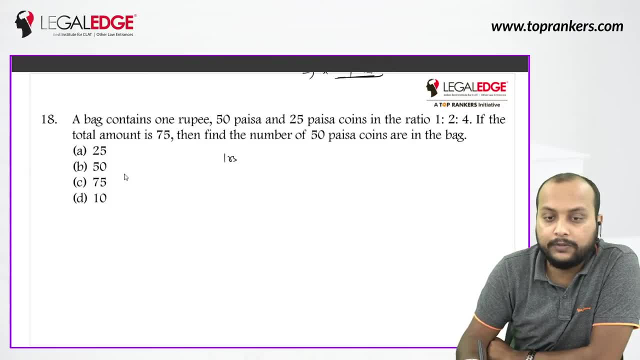 Bag contains 1 rupees. 50 paise is 25 paise In the ratio of 1 to 2 to 4.. If what you need is 2x, 4x, Remember Ooh your coins- get 4x and 2x rupees. 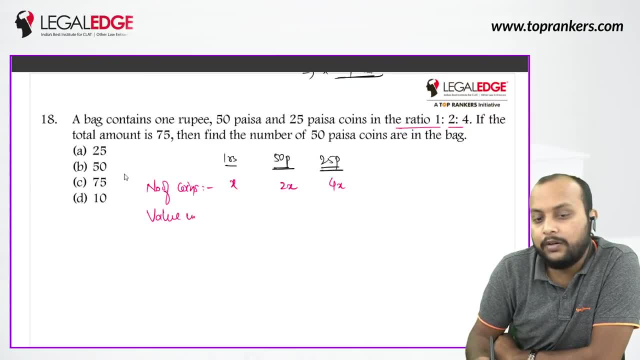 Get the points. What will be the value of 2x coins in rupees? So the value of x will be x only Because 1 coin is 1 rupee. x coins of 1 rupee is x rupees. 2x coin is 50%. 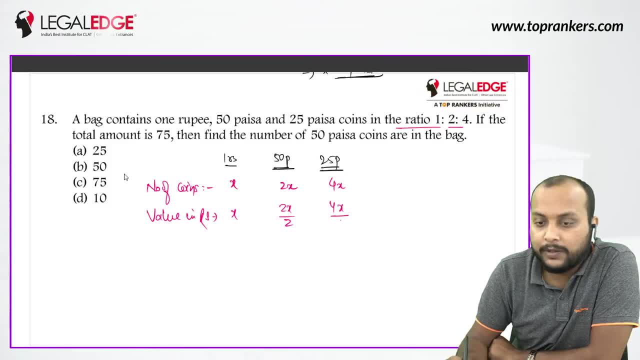 What will be the value Divide by 2 and 4x coin is 25 Divide by 4. So how much is this? So what is x plus x plus x 3x? So what is the value? 75.. What is the value of x? 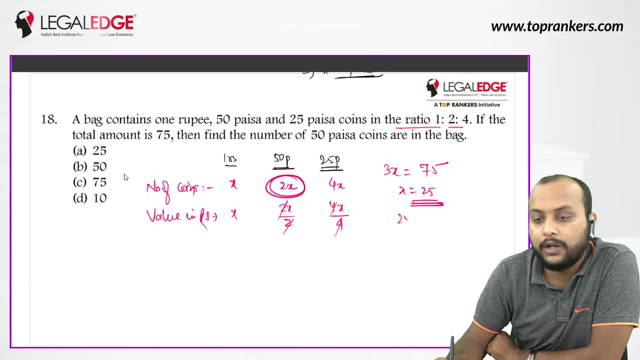 25.. If we ask the number of coins, How much is it? 2x x 25, that is equal to 50.. Option number B. So option number B is the correct answer. That is 50.. Five zero. Take out the value, Add the value. 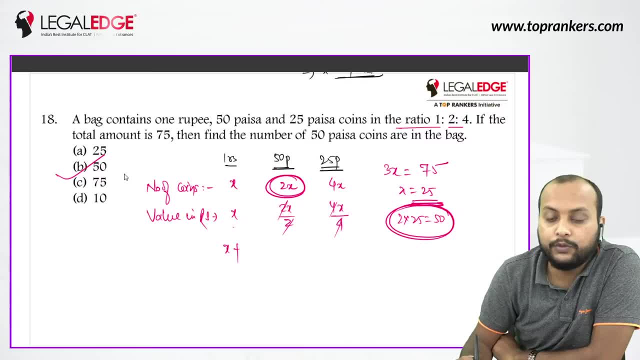 These are the values of 1 rupee x plus the value of 50 is x or the value of 25 is x. What is the total value? 3x? That is equal to 75 Done. What is the next one Now? question number 19. 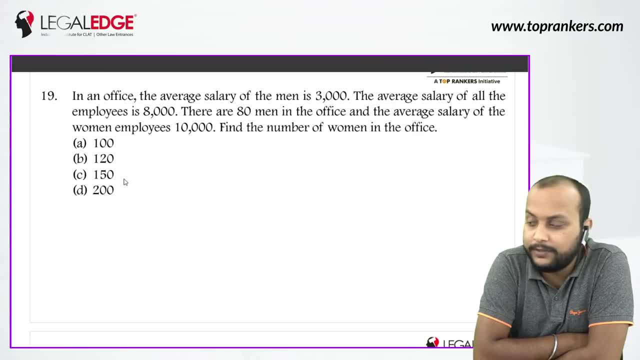 In question number 19. try to make it with allegation method. It will be made with equation method. It is better to practice with allegation method. So please solve the question number 19 with the help of allegation method, Allegation technique, Instead of going with the formula or going with the equation. 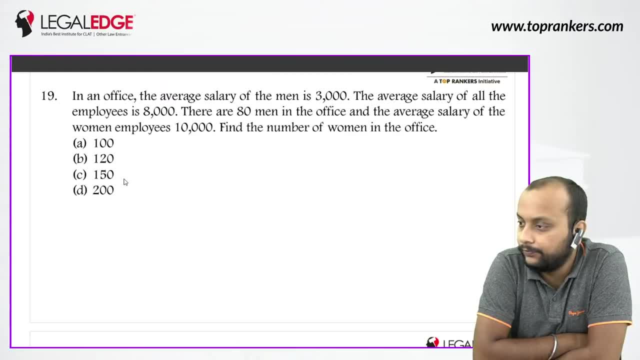 You have to train the right way, So We should be able to do the right way, So We can find the questions with the right way, But We can't find the answers. We can't find the answers Using equations or With the right way, We can find the answers. 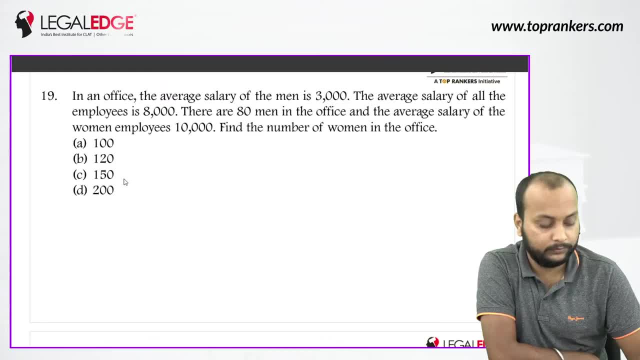 In the right way. In an office, the average salary of man is 3,000,, the average salary of all the employees is 8,000,. there are 80 men in the office and the average salary of women employees is 10,000,. 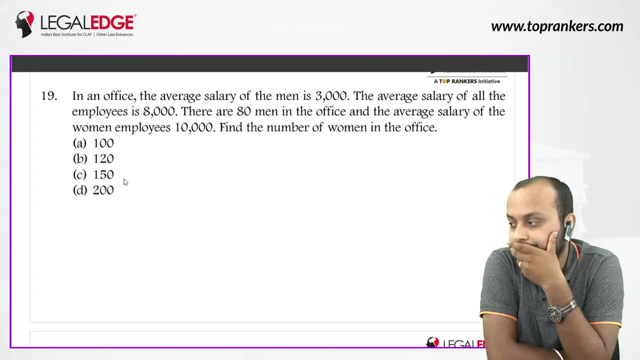 find the number of women in the office. The correct answer is for this question. what will be the correct answer? A, B, C, D. what do you say? what do you think? B 200 and B 120, it seems D. let's see men, 120,. 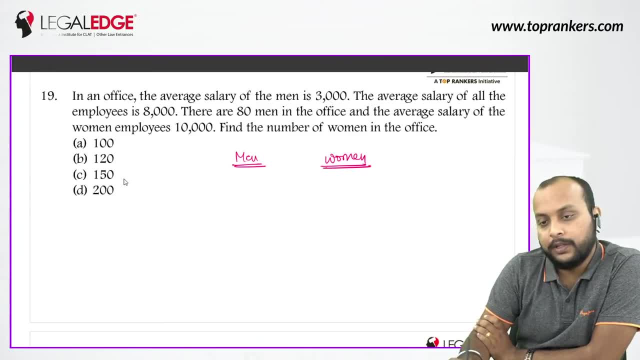 women. how many men are there? 80,. we have to find the number of women. let's see: the ratio is being found by allocation. how much is the salary of men 3,000,? how much is the salary of women 10,000,? how much is the overall salary 8,000,? how much is this 2,000, how? 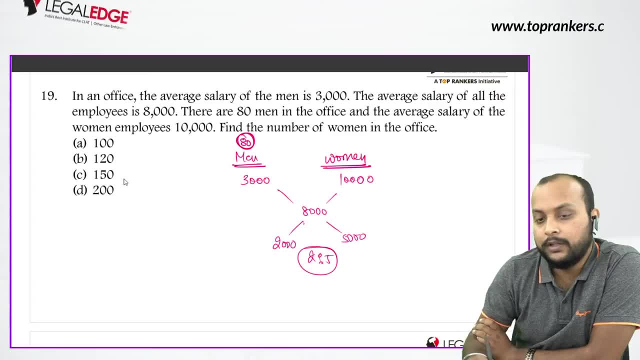 much is this? 5,000, that is what is the ratio. 2 is to 5, then what is the ratio of men by women? 2 by 5.. Men's value is 80,. women's value is W. so 2 by 5, so 40, how much is the value of women? 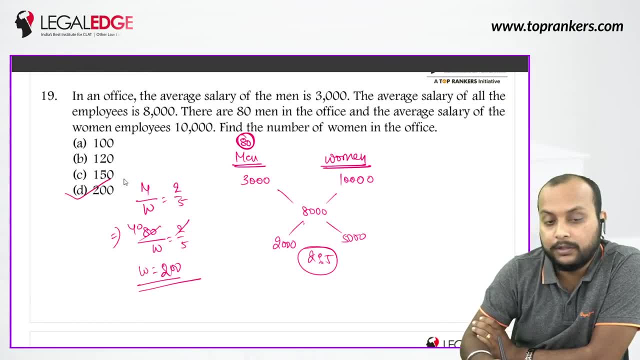 40 into 5, that is equals to 200,. option number D: It is easy, it was easy, but this is easy now. let's assume let the female employee equals to F. so 3,000 into 80 plus 10,000 into F equals to 8,000 into 80 plus F. 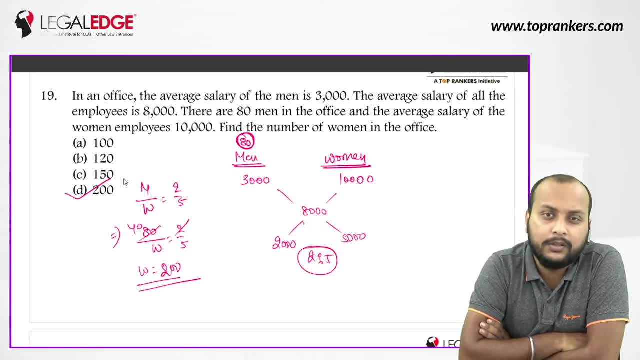 And then we are calculating F from there. otherwise we are calculating F from the female, so that will also be made from there. but it is easier for us if we apply allegations, then it is solved more easily, Isn't it? Is it easy. 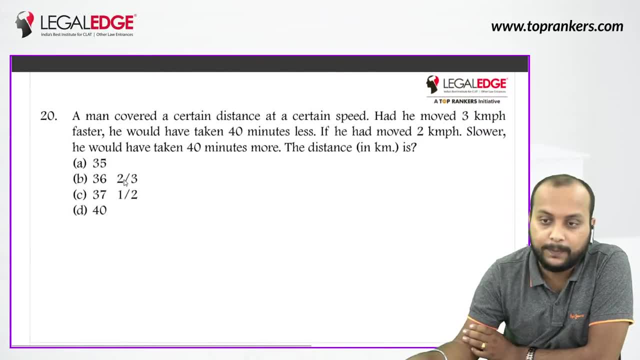 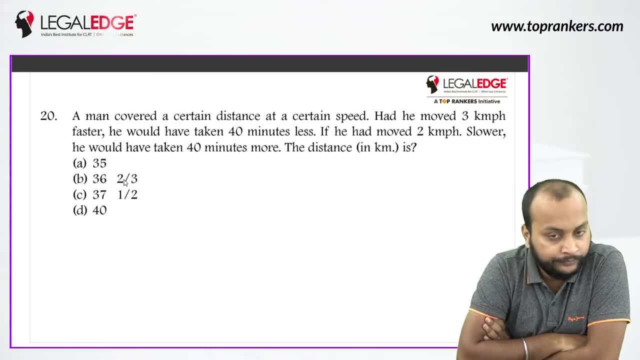 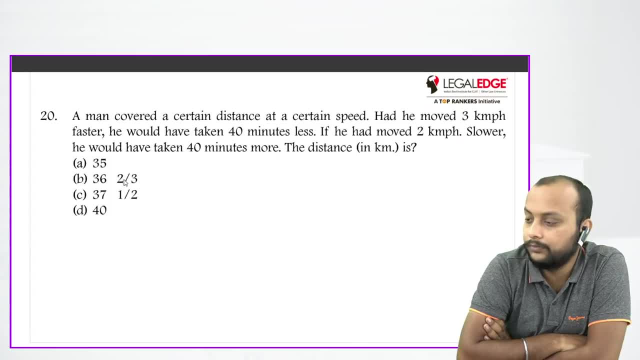 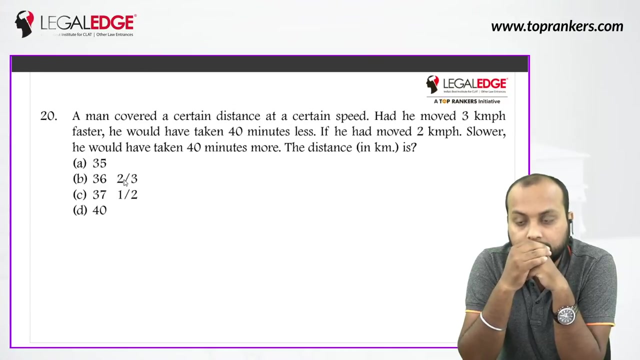 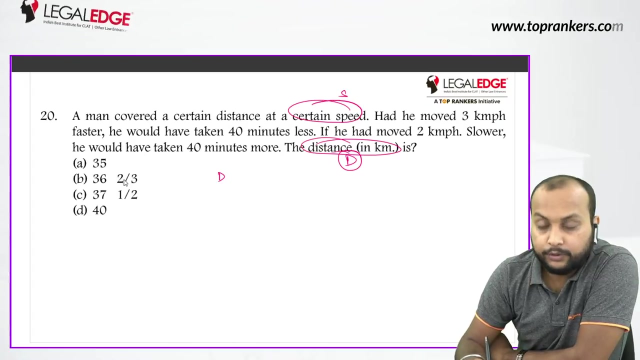 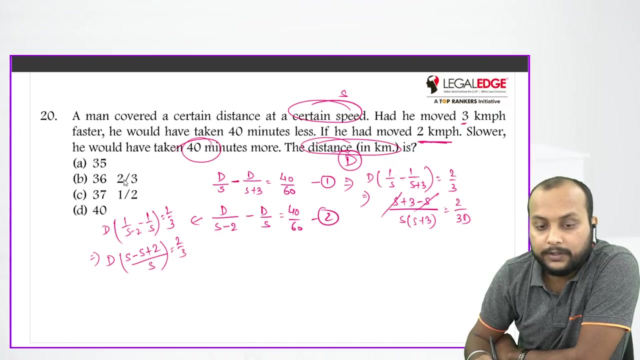 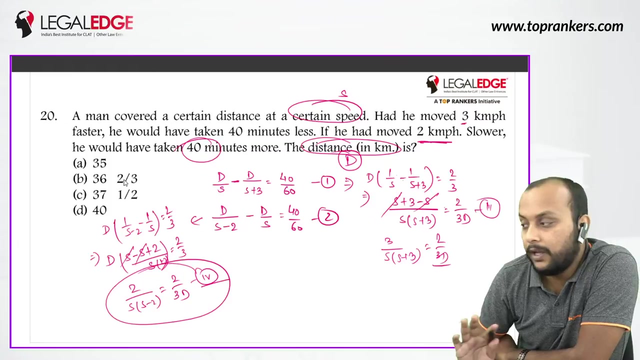 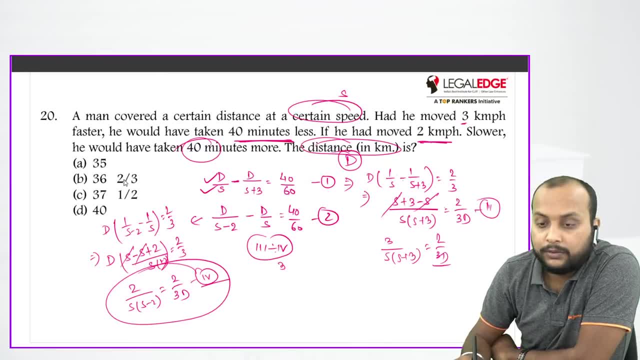 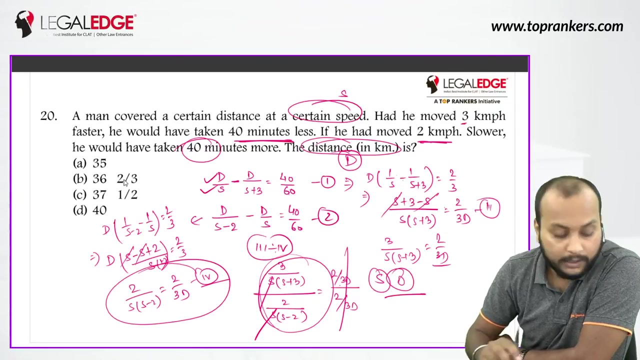 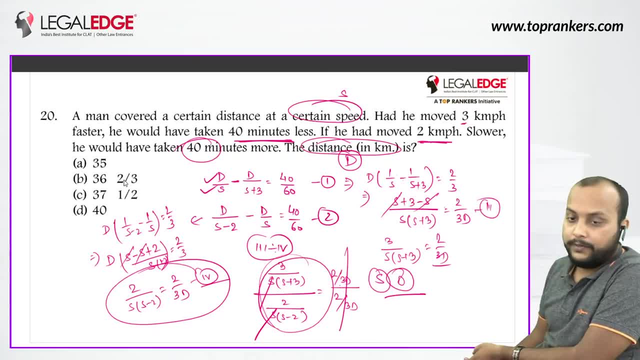 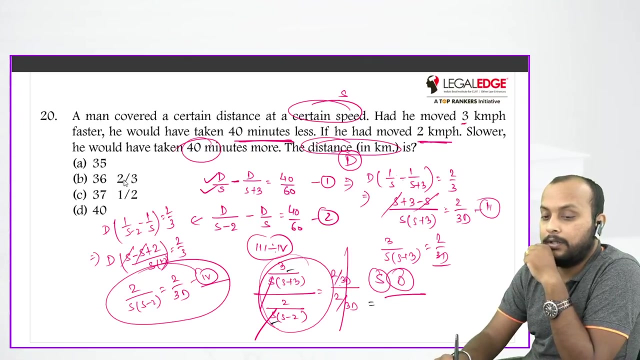 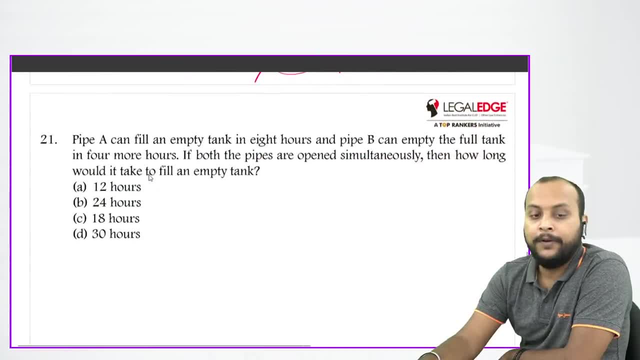 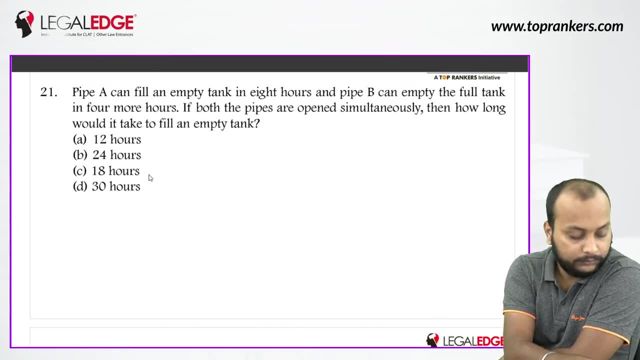 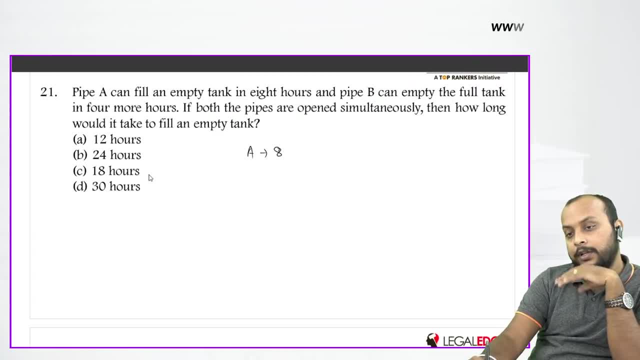 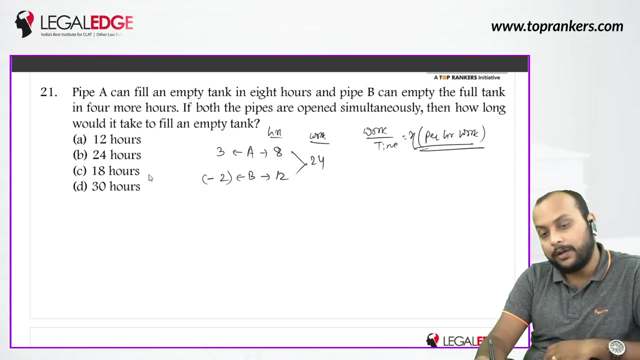 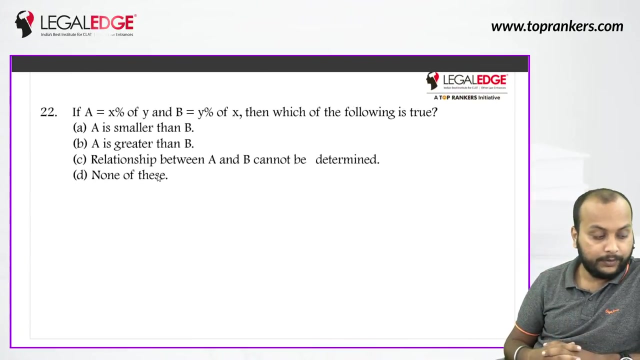 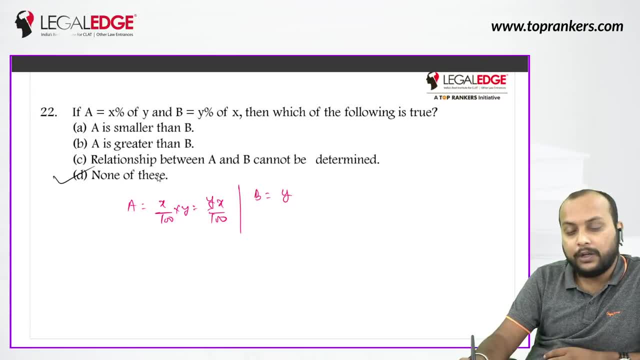 or x by 100, and b equals to y percent of x. so y by 100 into x, y, x by 100. so there is no difference between a and b. so the answer will be: a equals to b, a and b will be equal. so option number d is the correct answer. 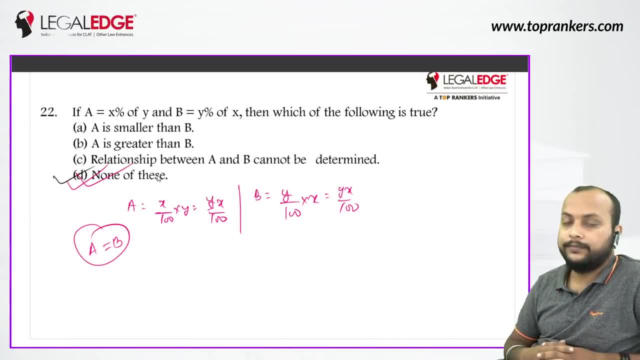 option number d is the correct answer. you can solve it by taking any number. both will be valid. take 50-40. 50 to 40 percent, 20 to 40 percent 20- it will be equal. x a equals to b, both will be equal. 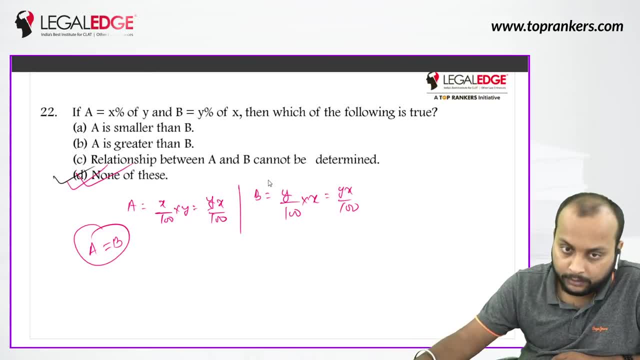 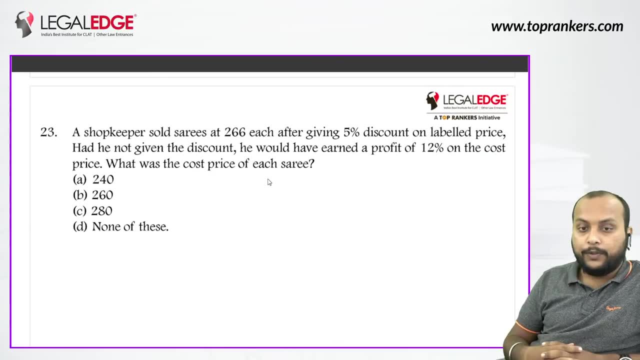 x. a equals to b. both will be equal. do the next one. a shopkeeper sold sarees at two sixes each after giving five percent discount on level price. had he not given the discount, he would have earned a profit of 12 percent on the cost price. 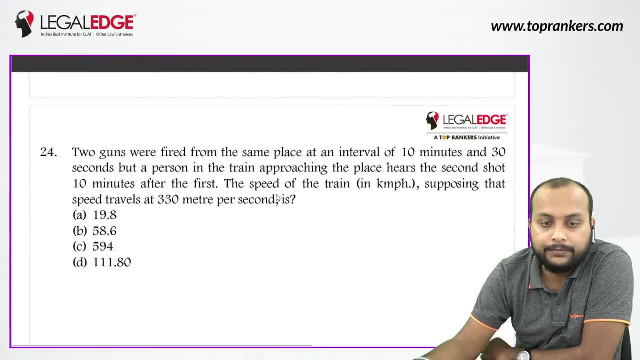 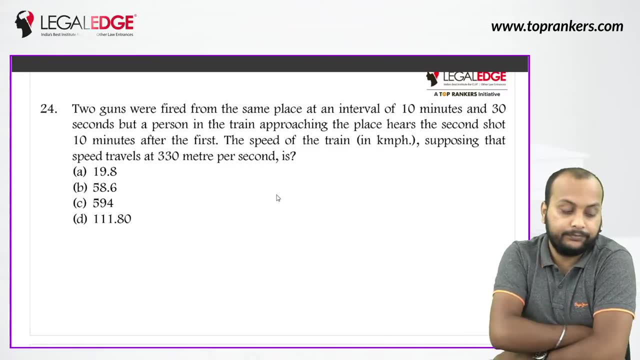 Thank you. 24th: This is based on time-space distance. Two guns were fired from the same place at the interval of 10 minutes and 30 seconds, But a person in the train approaching the place hears a shout 10 minutes after the first. 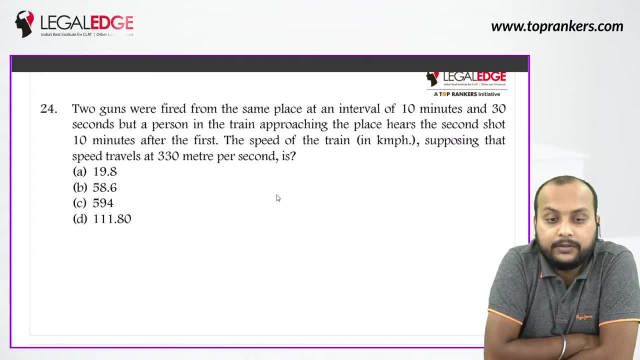 The gunshot is not heard. the speed of the train, supposing that speed travels at 330 meters per second. speed travels. here one word is missing. one word is missing: see last line. the speed of the train supposing that speed of bullet bullet travels 330 meters per second. speed travels sound, travels speed. 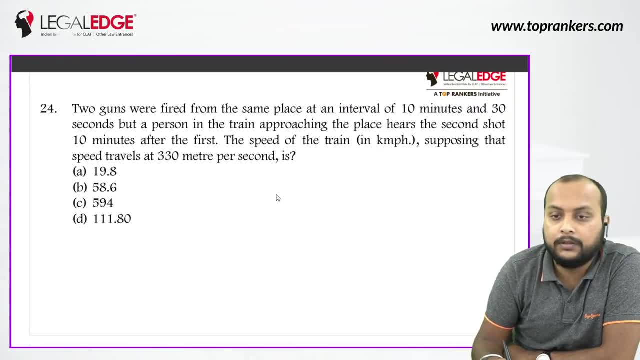 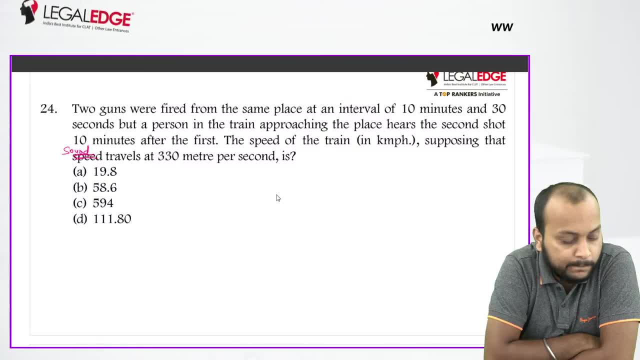 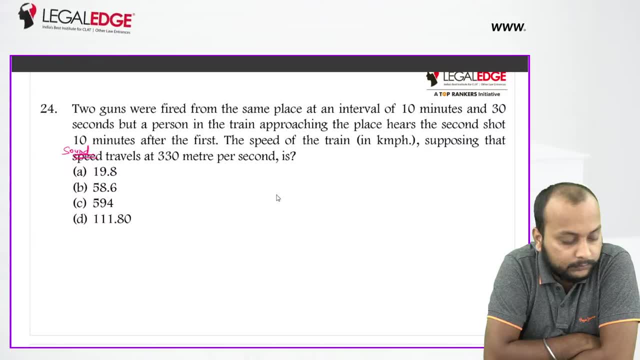 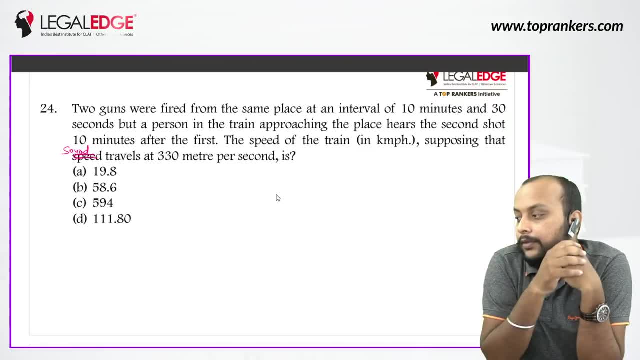 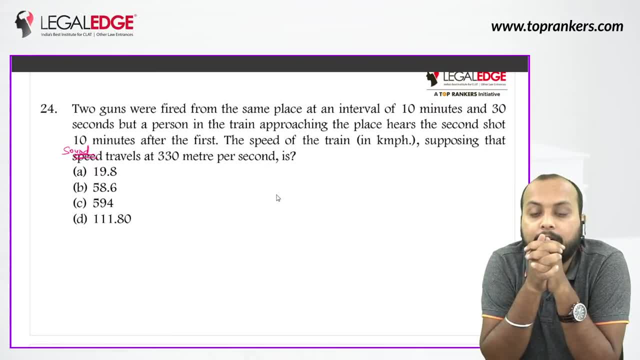 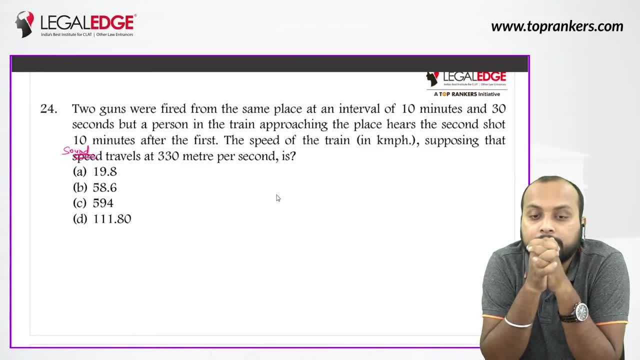 first The speed of the train. suppose that the sound travels at 330 meter per second, is What will be the answer for this question, Number 24.. It is easy. just apply a little logic, understand what he wants to say, it will be solved easily. 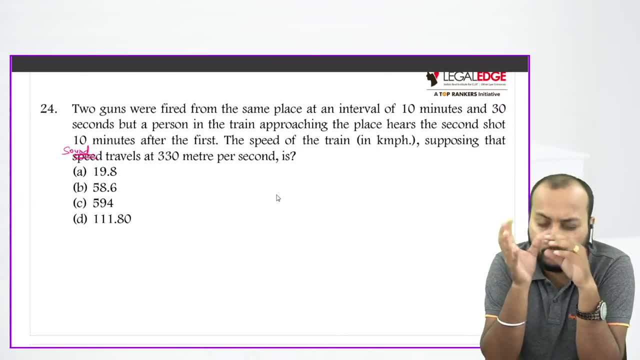 without any calculation. The calculation has been done a little bit. there is no lengthy calculation at all. you will solve it according to easy calculations. Two more minutes for these questions, then I will discuss. Understand, I tell you. At the same time a bullet was voraciously fired from here in this direction and the 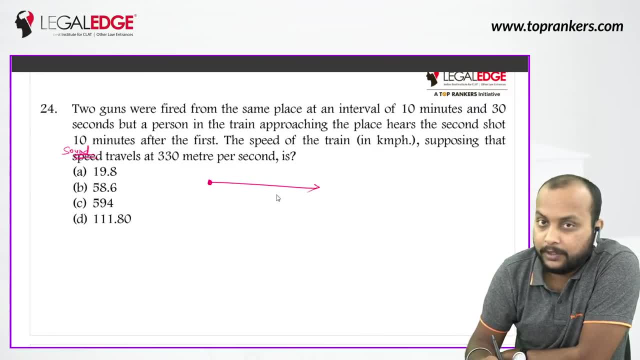 number of bullets was done in this direction, From this direction. the bullet shot was not taken. The score was given in this direction. the idea is still there, So I will tell you after 10 minutes. he is travelling, a train is coming from here. 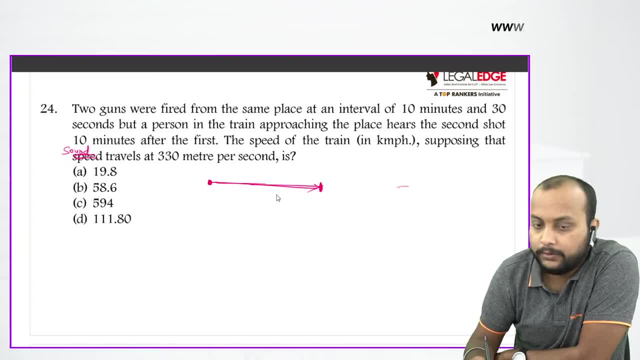 and he heard this bullet here. he heard the sound, but when the other bullet was stolen after this, the train was coming, so it was stolen after 10 minutes and 30 seconds. ok, so he heard the same thing here, at the same place. 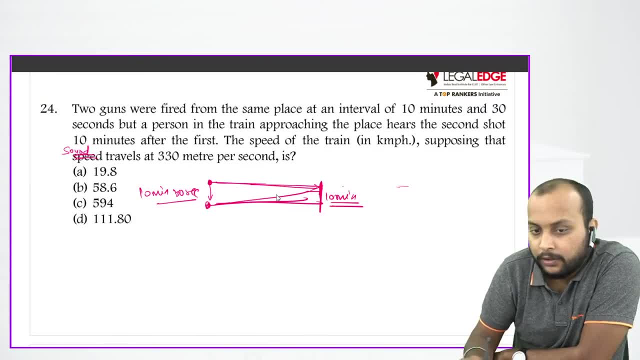 so he heard this gap after 10 minutes and when he fired it from here he fired it after 10 minutes and 30 seconds, but when he heard it after 10 minutes. so the gap of 30 seconds is covered. why is it covered? 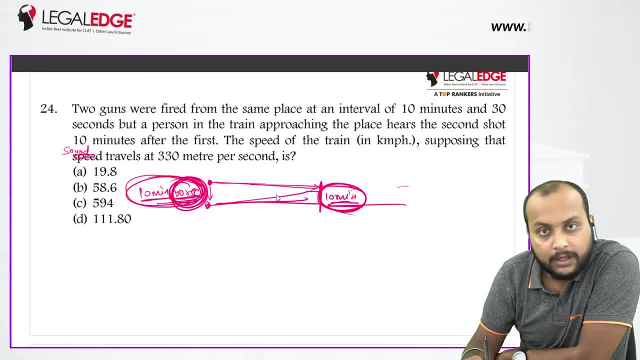 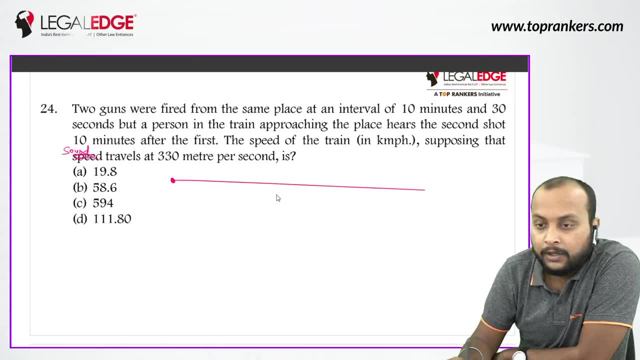 if it doesn't move, if it doesn't come here, if it doesn't come here, understand this: that one bullet, one bullet was fired from here and he heard it here. after how many minutes? after 10 minutes and 30 seconds he heard it. 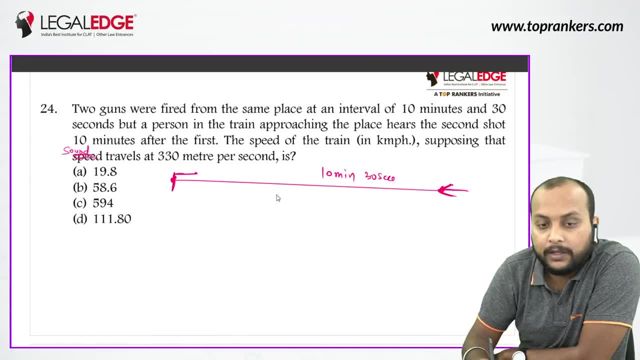 he is coming here and this bullet was fired from here- ok, now from this place. after how many minutes it was fired? so it was heard after 10 minutes and 10 seconds when it was fired. after 10 minutes and 30 seconds it was fired. 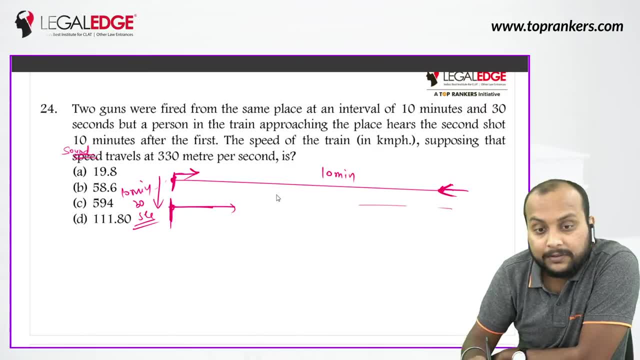 from this place to the other bullet. now it is coming here now after 10 minutes. it was fired. suppose if I had fired it at 4 pm now I fired it at 4.10.30. ok, now it is coming here, so after 10 minutes. 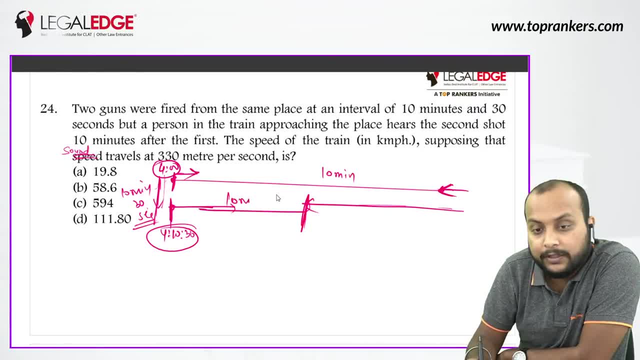 now it was fired, but now it is again fired here, but when it was fired again after 10 minutes, so the gap of 30 seconds. why is it covered? because it was moving in this direction, so till some distance sound traveled, so it also traveled some distance. 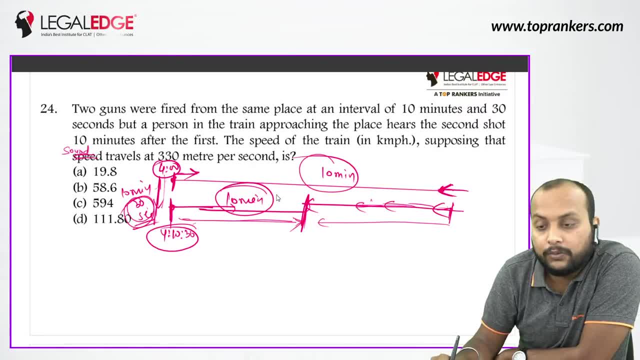 ok, some distance sound traveled and some distance it also traveled. so both of them are in the middle because it is in 10 minutes and 30 seconds. if it was stable here, if it didn't move, then the other bullet would have heard it after 10 minutes and 30 seconds. 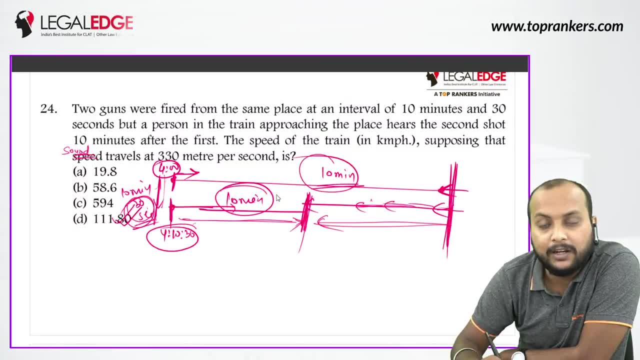 after the time it was fired. it would have heard it now. it was fired after 10 minutes and 30 seconds. so it would have heard it after 10 minutes and 30 seconds if it didn't change its position. now it changed its position, which direction? 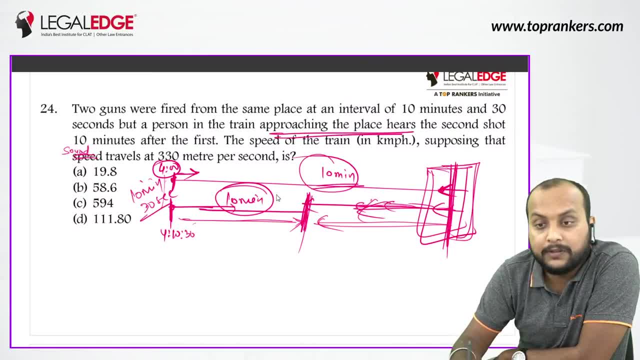 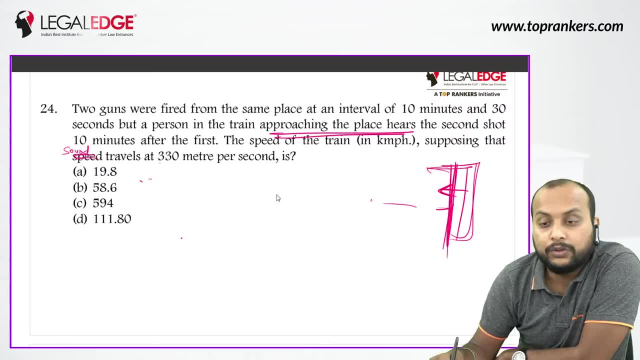 towards the place approaching the places. so it moved in the same direction. that's why it got a gap of 30 seconds. so in 30 seconds how much distance sound would have traveled? in 30 seconds, how much distance sound would have traveled? I am telling you. 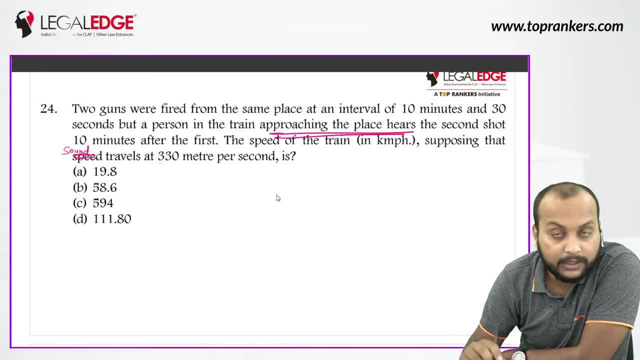 in 30 seconds how much distance sound would have traveled. so sound distance travels: 330 meters per second. so 30 seconds, in 30 seconds, sounds will travel 330 into 30 meters. this will happen because in 1 minute, in 1 second, 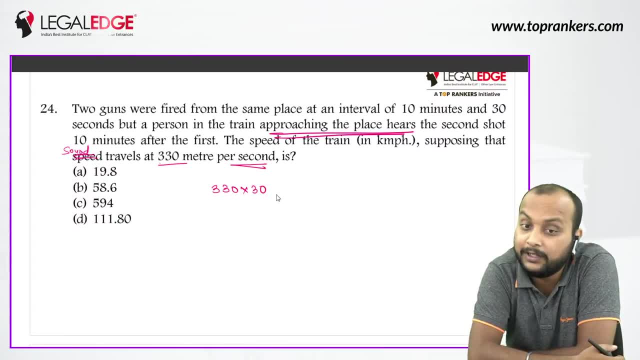 330 meters, so in 30 seconds. how much distance sound traveled? 330 to cover the same distance. how much time did the train take? 10 minutes. then 10 minutes was constant and the third gap came: the distance sound is covering in 30 seconds. 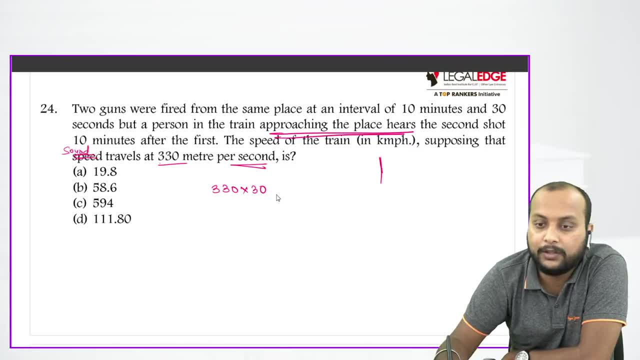 it is covering in 10 minutes. I will make another diagram. don't get confused. this is the distance now. it went from here and heard from here this train was coming and this sound was going. if this person was stable here then it heard the bullet from here after 10 minutes. 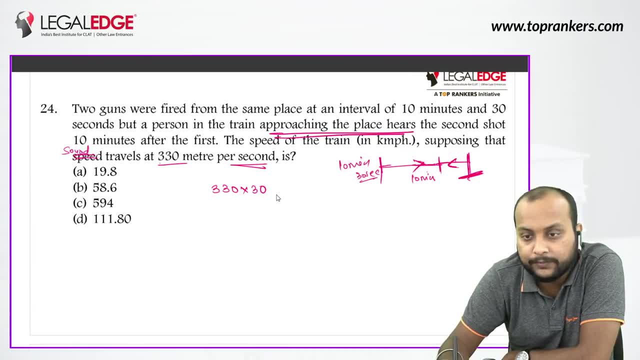 but it was fired after 10 minutes 30 seconds. so here, where it heard, it heard the sound to cover this distance. to cover this distance, sound takes only 30 seconds, sound takes only 30 seconds in 10 minutes 30 seconds. the person standing here- 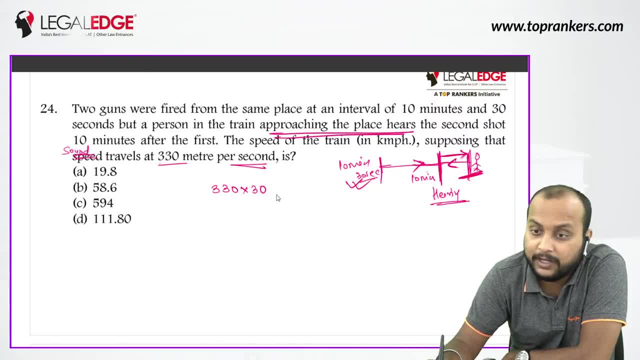 would have heard this, but this did not happen. this person moved from here and came here, so it took 10 minutes to travel this distance. then what happened? in 10 minutes it was cancelled, so the distance sound is traveling in 30 seconds. the same distance. 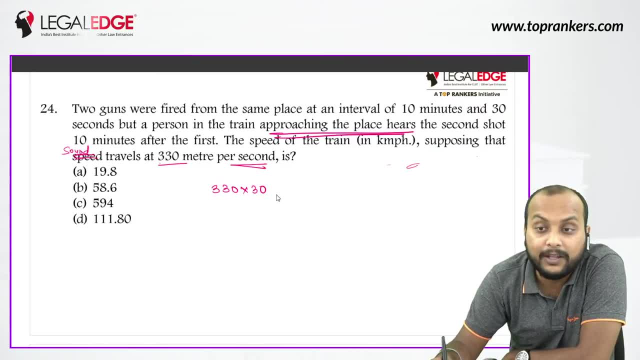 in 10 minutes. the train is traveling. so the distance of the train, what is the speed of the train? x km, x km per hour, x km per second, x meter per second. the speed of the train is x meter per second. x meter per second, x meter per second. 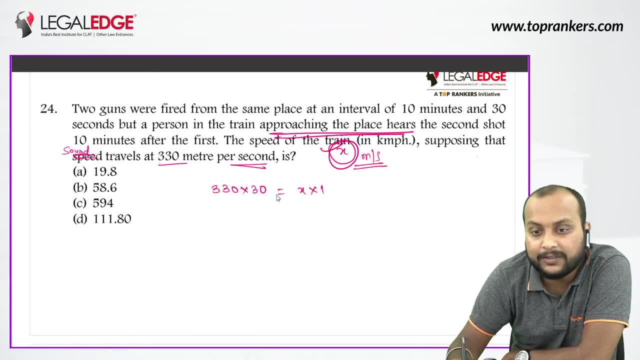 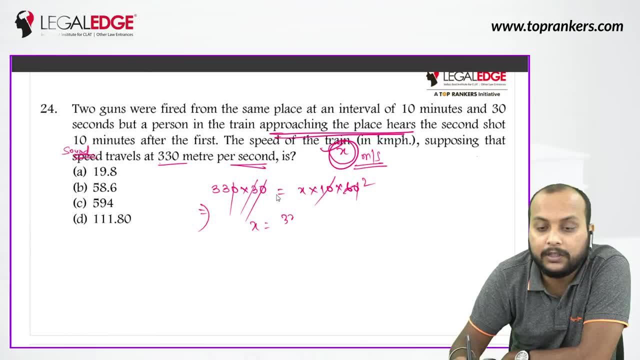 x 3 x 2, so the value of x is 33 by 2 meter per second. so what will you do? multiply 33 by 2, multiply 33 by 2, multiply 33 by 2. divide by 10. do not cut. 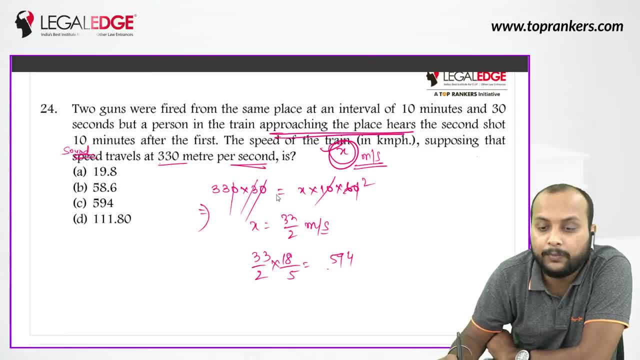 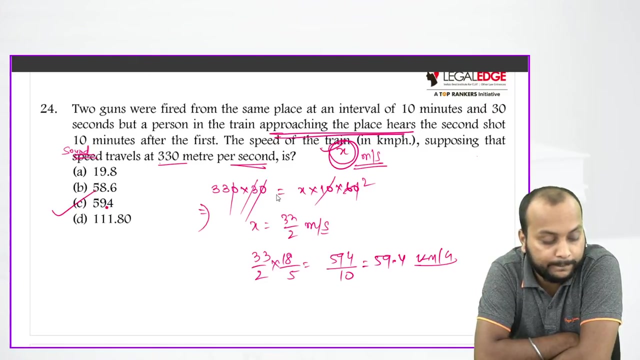 18 x 3 is 54, 5 x 5 is 54, 59.4 km per hour. option number C: 59.4. printing missing 59.4. you can do it, but you have to calculate the distance. here only x is calculated. 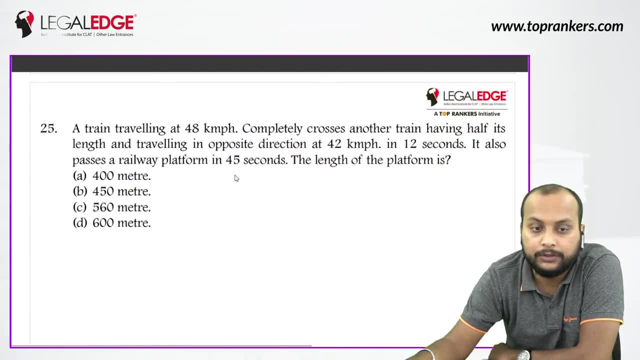 speed is calculated. ok, now 25, same pattern. cam is on distance. i am explaining the distance of 10 minutes and 30 seconds. city: where are you from, from where you are? please tell me the place. i will explain it again. difference of 10 minutes and 30 seconds. 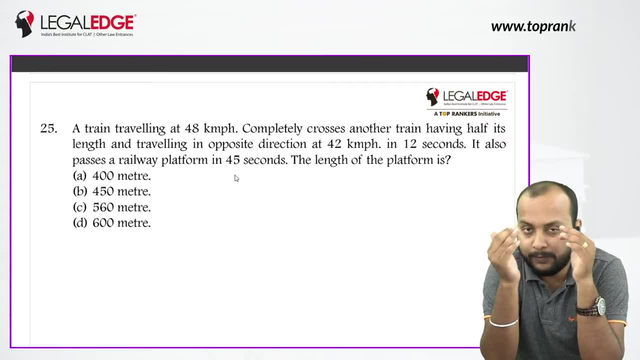 i am taking it normally. a print is coming from Delhi towards Bhopal and i fired a bullet from Bhopal towards Delhi. i fired a bullet. i did not fire a bullet, i fired a bullet from Bhopal towards Delhi and a person is coming from Delhi by train. 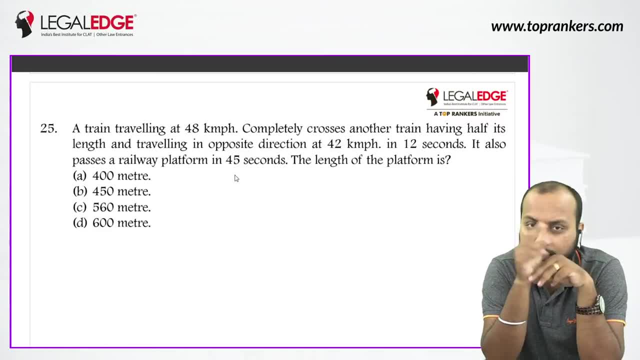 you are coming from Delhi by train, so i fired a bullet in 4 pm. you heard the sound that a bullet was fired. after that, i fired a bullet after 10 minutes and 30 seconds, at 4.10.30, and you heard the bullet. 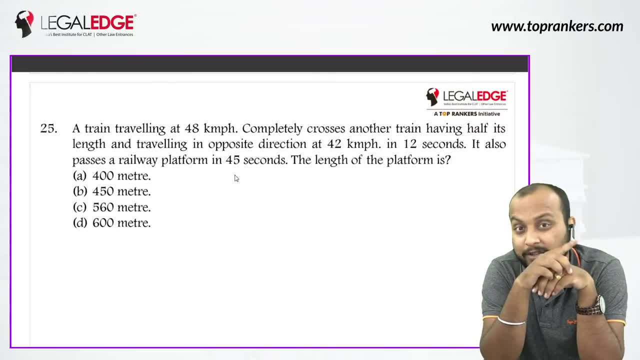 after 10 minutes. i fired a bullet at 4.10.30 duration. you heard it after 10 minutes, 30 seconds gap. why, if you were in Delhi, you would have heard it after 10 minutes and 30 seconds. ok, you would have heard it. 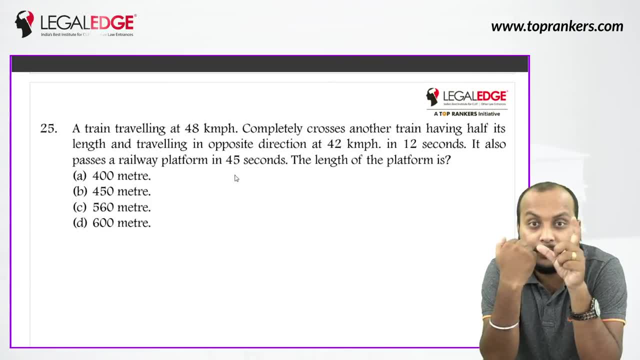 but you came towards Bhopal so your time was decreased because the speed of the sound is high and the speed of the train is low. so the distance you covered in 10 minutes. same distance if you were in Delhi, you would have heard that sound after 10 minutes. 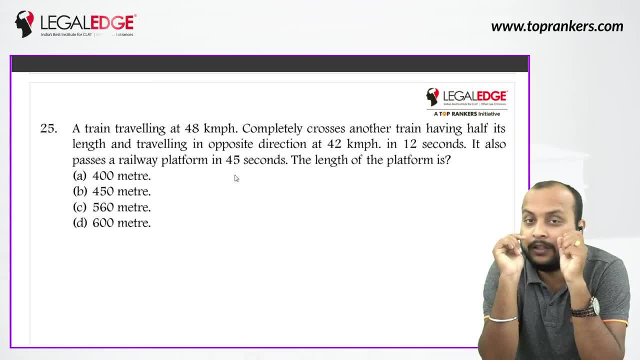 you would have heard that sound after 10 minutes 50 seconds and if you include the distance you covered in 10 minutes, the distance you covered in 10 minutes, you think the sound you heard in 10 minutes and in Delhi you heard it in 10 while. 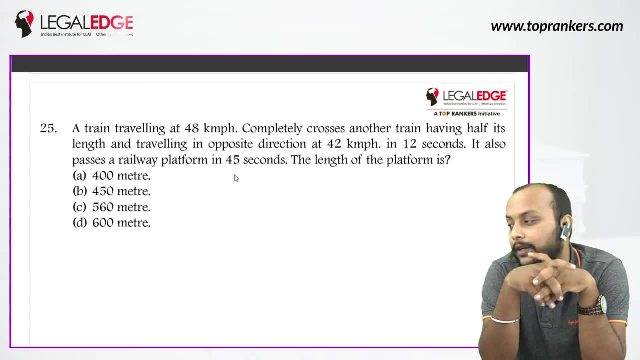 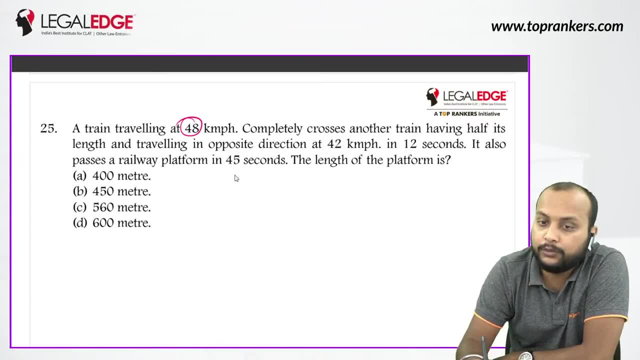 deho ek train ki speed hai 48 duse, train ki speed hai 42 kilometre. padavar mein hai direction. kaunsa hai opposite speed? kya hoge plus dono train kya hoge direction mein hai. opposite direction mein hai ek dusre ko cross kar rahi hai kitne seconds mein? 12 seconds mein. 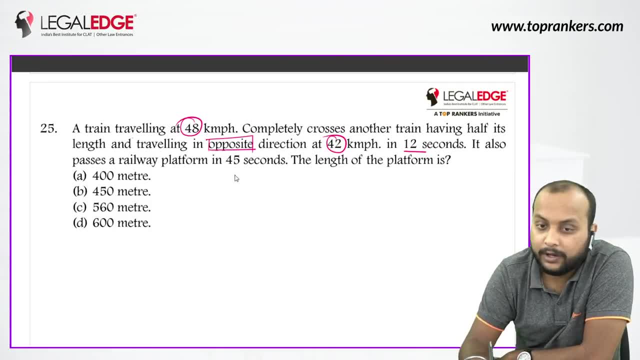 length kya hoge dono train. ke addition, a train travelling completed, another train having half of length. toh first train train maano a hai ye train, a hai iski length, apan maal lete hai x, x by 2, so x plus x by 2, ye kya minjaga hamare distance upon speed. speed kya hoge 48 plus. 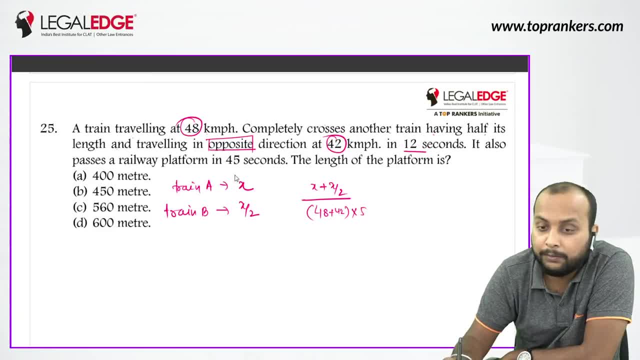 42 kilometre padavar mein hai. kya karoge meter per second me convert karoge kitna time leki 12 seconds. kitna time leki 12 seconds calculate kar sakte hi se ye kitna aega 3x by 2 upon? 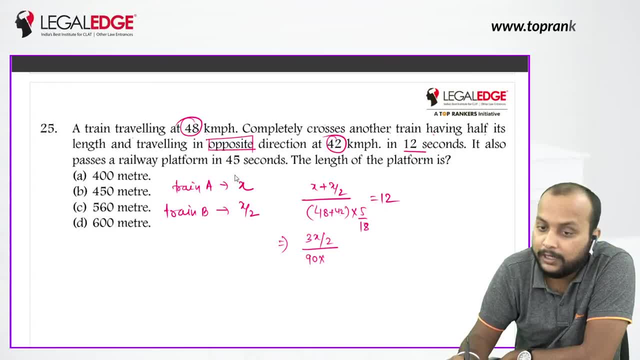 48 plus 42 is 90. so 90 into 5 by 18 equals to 12. so deko ye 18 se lage a ye 5 chala gaya. kya aaya tumhare pos equation: 3x by 2, niche aya haega 5 into 5, 20, 5 into 2 kitna aaya 50, that is equals. 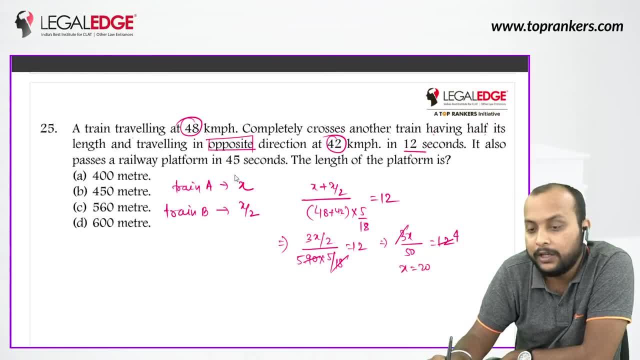 to 12, 3 se gaya ye 4 to x ke value kitne aye 200 meter. toh length of train kitna aega 200 meter. ek length kitne aage 200 meter. iski length kitne ho jage 100 meter. tomse uske. 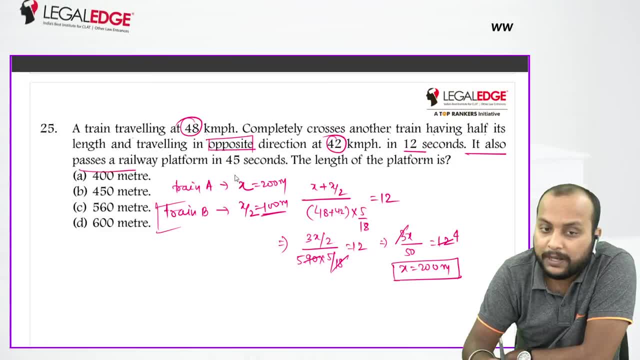 pari pujha nahi hai. iske pari usko cross kiya tha. It also passes the railway platform in 45 seconds. So to cross the platform, what is the distance? Length of train that is, 200 plus length of platform, which is L. 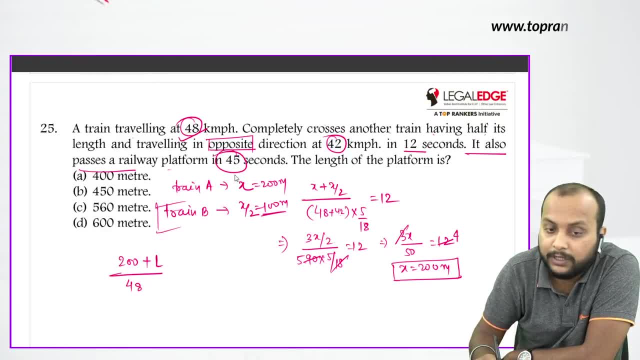 Speed of train is 48 km per hour, So 48 into 5 by 18 in 45 seconds, So time is 45. Distance upon speed equals to time. Take the platform from here. Understood, I understood. 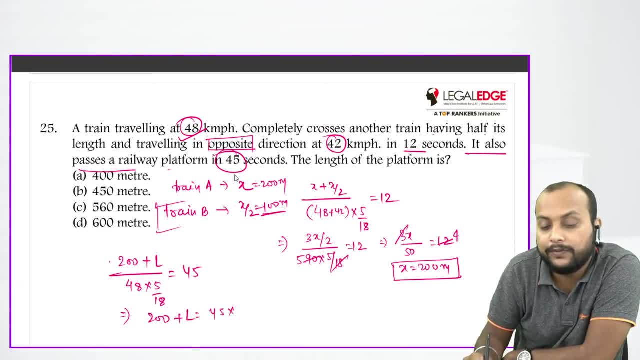 Understood, Which means 200 plus L equals to 45 into 48, into 5 by 18.. So 9 into 5 and 9 into 2 and 2 into 9.. So what will be the value of L? 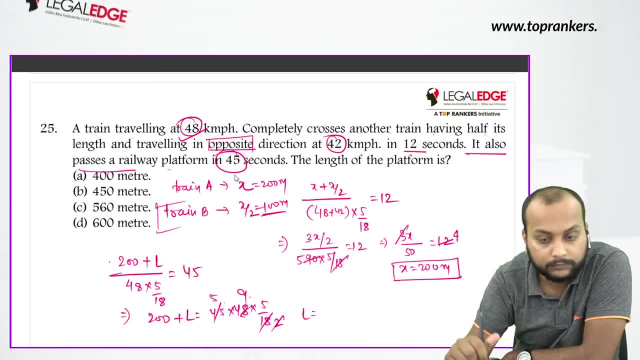 25 into 9,, how much is it? 225.. 2 into 24.. 24 over 1.. Yeah, Okay, 1200. 600.. 600 minus 200, that is equals to 400 meter. 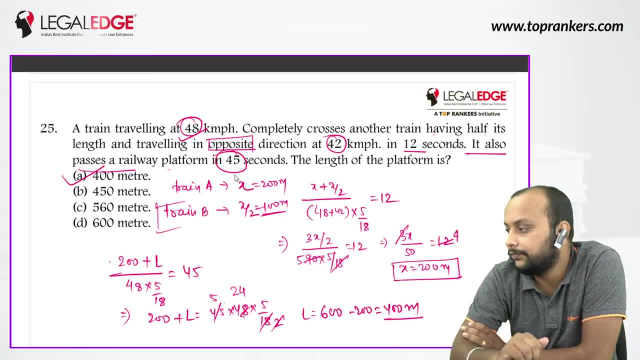 Option number A. The relevance of mid questions is to find the length of train. A answer will be D, not A. 600 meter is the length of platform plus length of train. So length of platform is 400 meter. Option number A: 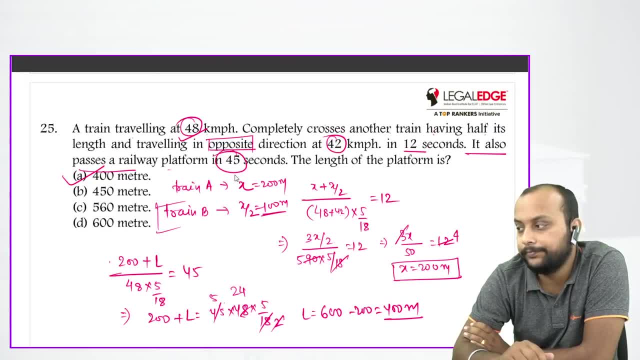 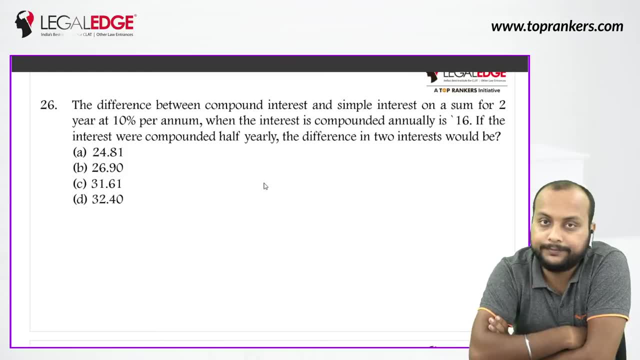 600 is the addition of the length of train and platform. 600 is the addition of 400 plus 200.. Platform length plus length of train plus length of platform equals to 600.. So length of train is 200, hence the length of platform is 400, not a 600.. The difference between compounding a 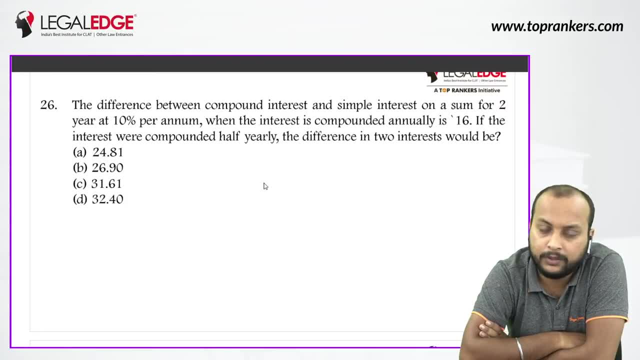 simple interest or a sum for two years at 10% per annum. when the interest is compounded annually, it's 60. If the interest were compounded half yearly, the difference in two interests would be the same. The difference between compounding a simple interest and a sum would be the same for. 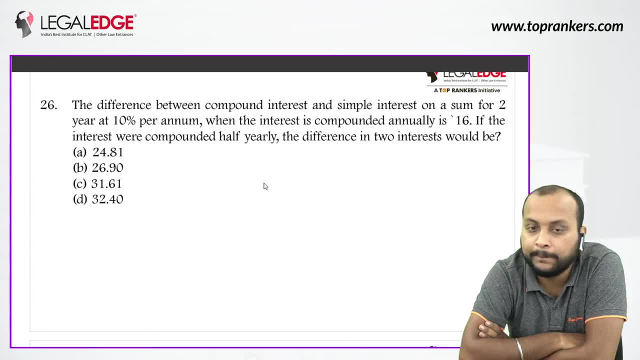 a period of time. If it's compounded during the term, it's the same period of time to a potentially long term term. This should be a good sign, and it should also be a good sign that we're going to go through the business as a whole. I don't know if any of you have heard about 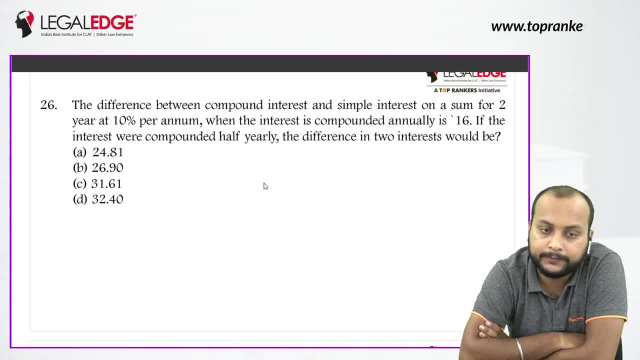 the judgment of the GDS. They have some great arguments, but I understand what you're saying because it's in the GDS. It's only 25,000 years. We're not going to go through the judge's judgment. So it's not like I'm going to go through the GDS's judgment and it's not going to be 50,000 years. 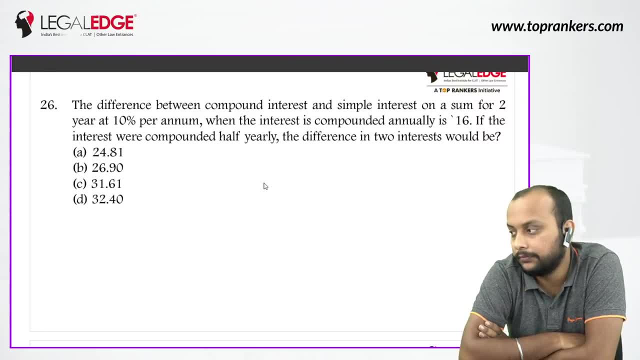 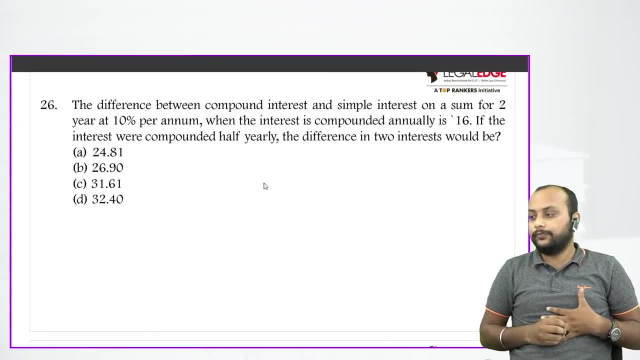 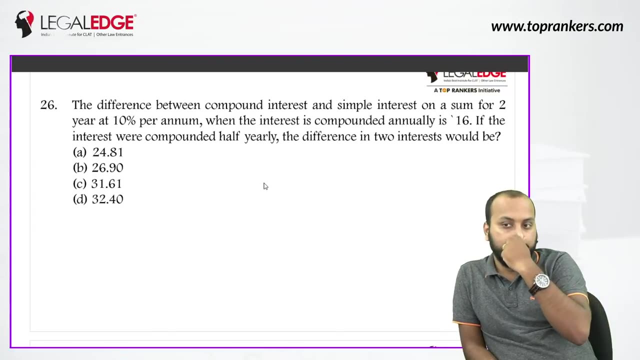 you? What is the answer? Question number 26.. Question number 26.. How will you do it? Only 2.40 will be wrong. Anyone else? Difference between compound interest and simple interest on a sum for 2 years: 10%. 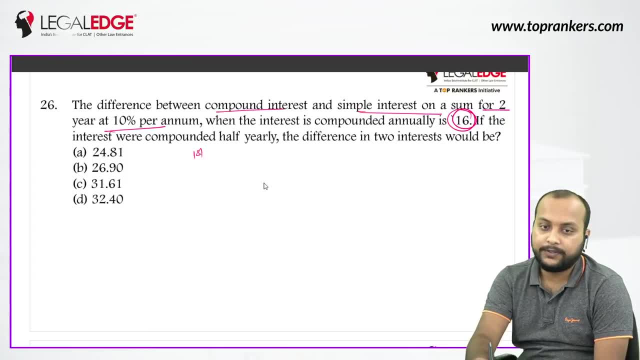 You know one thing: First year, SI and CI are equal. Are they equal? Look, Let's take a chain rule. What will happen First year? Second year? First year, interest is 10%. SI and CI are equal. SI will be 10%. 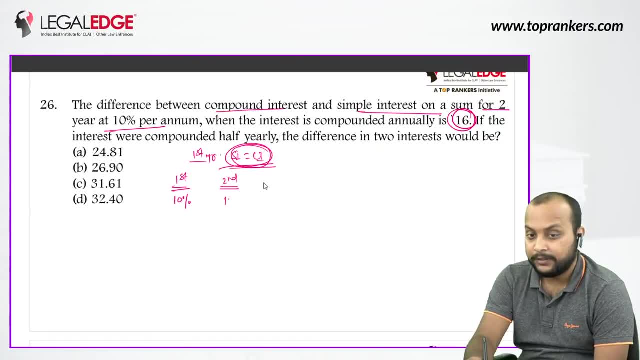 CI will be 10% Next year. 10% interest will be available. Compound interest is interest on interest. Interest on interest is compound interest. Now, 10% of 10% is 1%. Second year interest is 11%. So 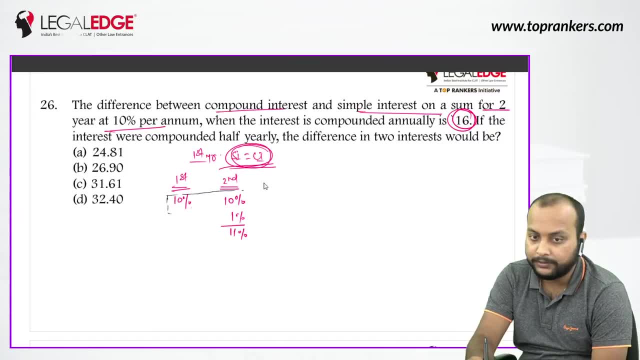 Look, This is our simple interest: 10%, 10%, Because simple interest is always simply counted on principle. And what is our compound interest? This one, 10% and 11%. What is compound interest? Compound interest is also compound interest, along with interest. 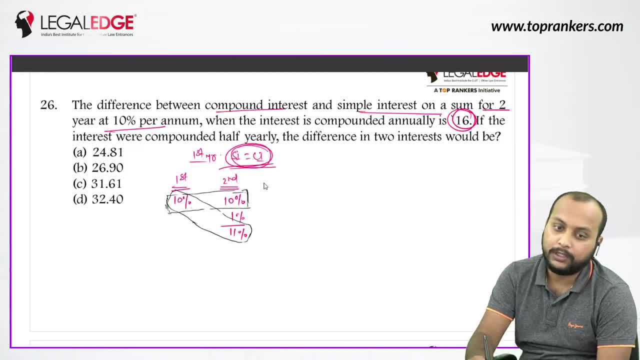 interest is also calculated on interest, along with the principle. So in two years SI is 20% And CI is 21%. What is the difference? 1%, See, If interest is 1%, then the rate of interest is 1%. 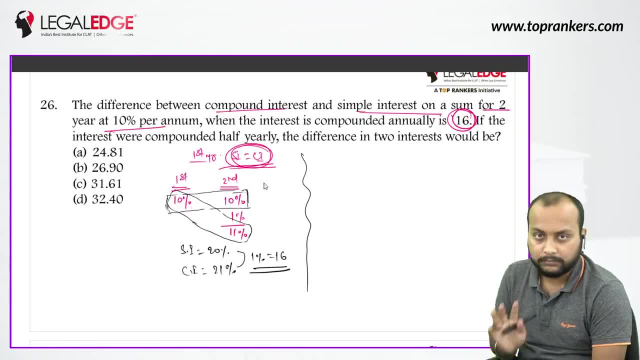 At the end. If interest is 1%, we have given the answer to the 1% of interest which has given the value of 16.. Okay, It is done. Whatever we have to take out is done. Now, when interest is half yearly calculated. 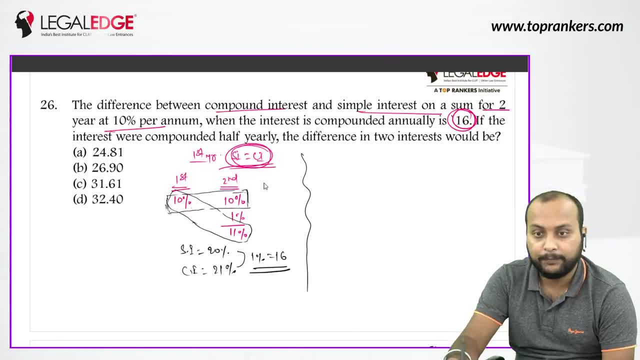 then the year is doubled and the rate is half. This is the method. Rules are Now. what is the compound of this Half yearly? So what will be rate Half? So what is the rate now? 5%. 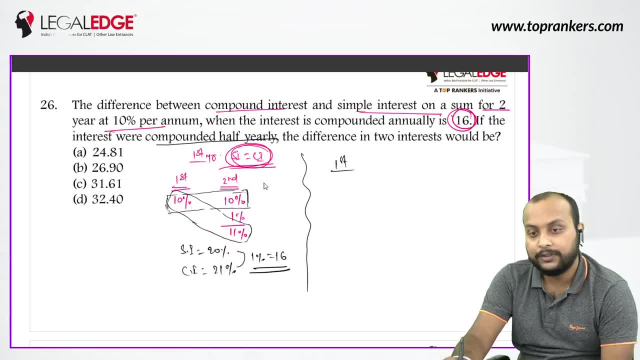 double. so from 2 to 4 years. so 1st, 2nd, 3rd and 4th, first year interest is 5%, 5%, 5% and 5%. so what you get is SI. again, SI is 20%, but CI is not 20%. now I will calculate CI: 5%- 5%. 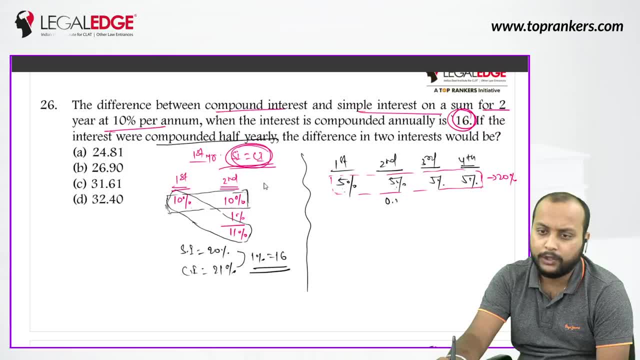 in 2nd year, you will get 5% of 5, so what you get is 0.25%, so what you get is 5.25%. similarly, if you go here 5%, so 5% of 5 is 0.25%, and 0.25%, then 5% of 5,. 5% of this 5, then 5% of this 5,. 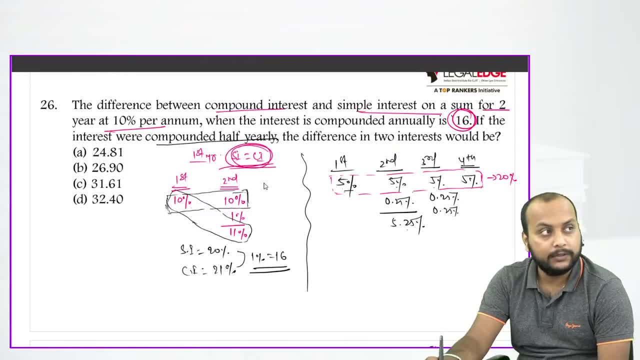 and then 5% of this, 5, right. 25% of 5 is how much? 0.0125%. so 5% of 5,, 5% of 5,, 5% of 5, or 1.25%, whatever it is, 1.25%. if you add this, then it will be 5.5 bar 625%. so the difference. 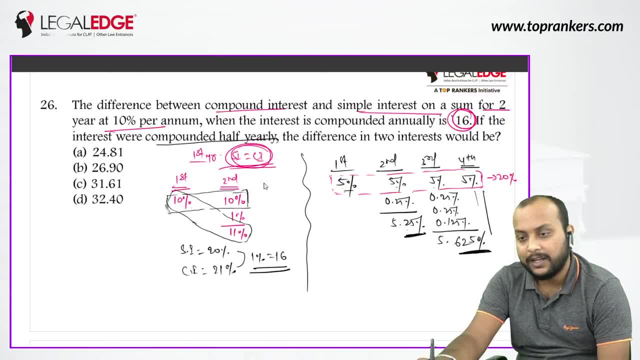 will come this: 0.25, 0.625,. again, here a difference will come. equate the summation of that with this: that 1% equals to 16, then the value equals to what? so the answer will be 24.81,. rest, you can go. 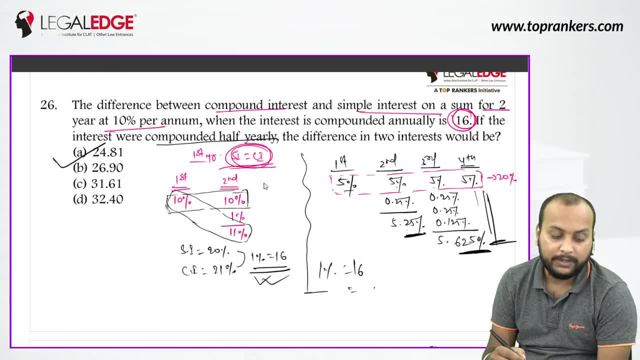 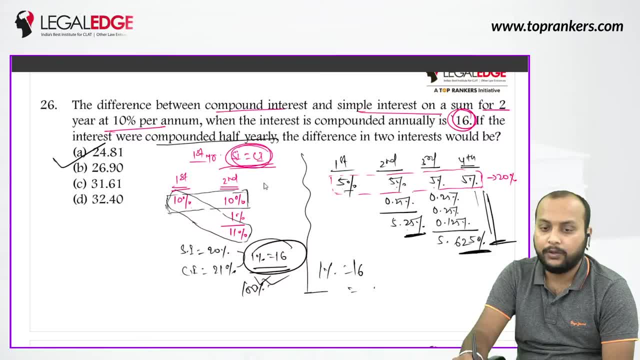 like from here, 1% equals to 16, if you take out 100% then the principle will come, that is 1600, if you go to the formula, then 1600 principle 1 plus, so the rate will be 5 by 100 is to power 4,. 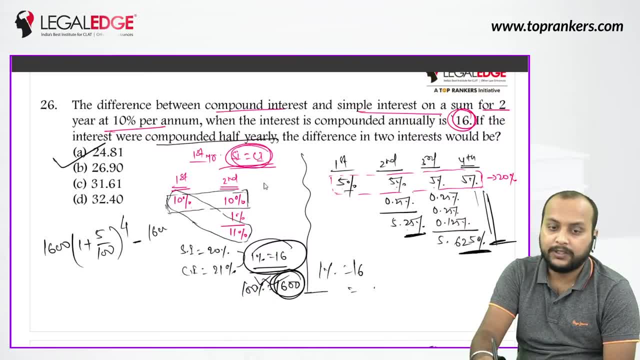 this is CI and minus SI will be 1600 multiplied by 5, multiplied by 4, divided by 100, so this will give you SI minus CI difference, the difference between the two, and you will see the difference. it is good, it is Calculative. 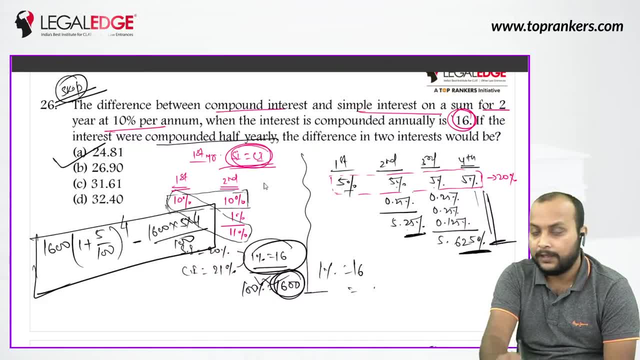 when this will come in the paper. you have to do this in the elite, you have to do this in the skip. that's why I have done this, because there is more calculation. if I am also going to the method of its easy, which is easy, basically, it is compounding. 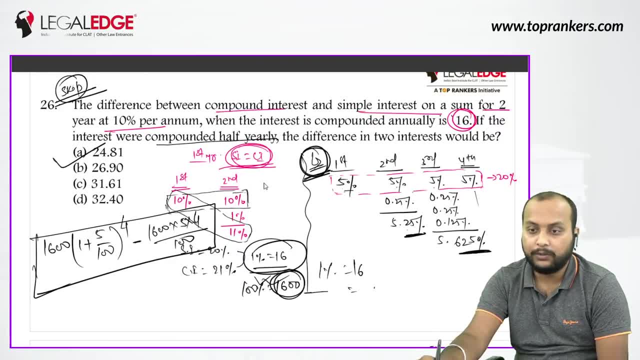 We have calculations increasing in that too. if I complete it a bit, see, this will come 0.25%, 0.25%, 0.25%, then 5% of 0.0025, 0.125%, 0.125%, 0.125% and 0.0625%. add them all and the difference will be 0.25, 0.625, we will equate them and it will be 24.81.. 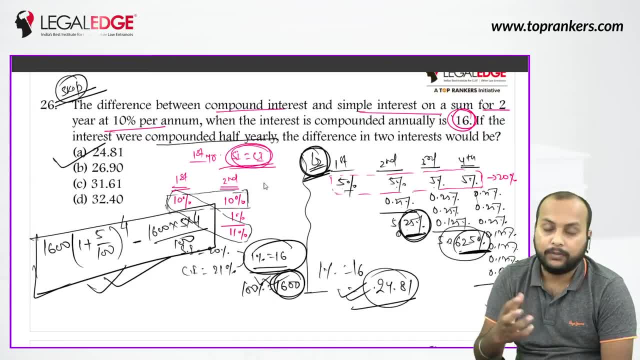 Or if you go in this, the same value will come from here: 24.81.. From the formula, our chain method is very easy Because we have given 2 years here, so it is 4.. Most of the time we ask 1 year's questions here. 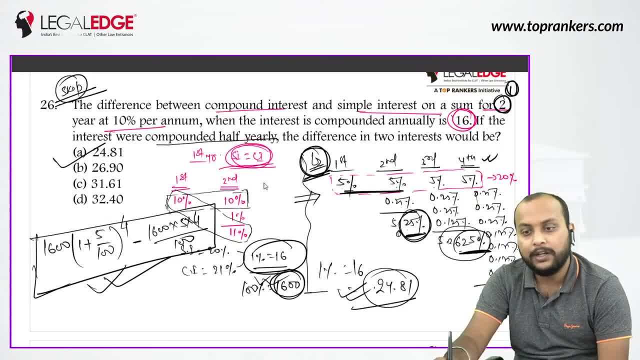 When we ask such questions, our work time is more than 2 months, So we will calculate it. If we had asked for 1 year, then it would have been easy, But we asked for 2 years, so it went long and you got more calculations. 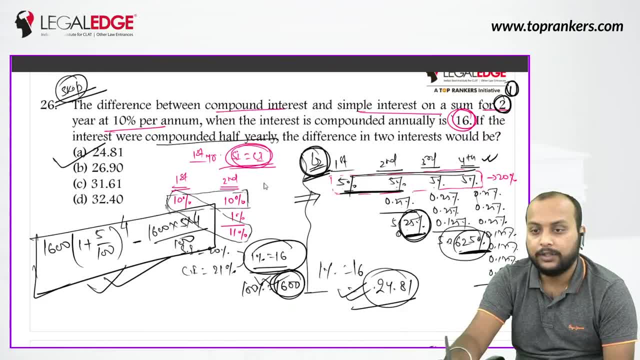 Let me tell you the CI calculation of the third year. again. In the third year, basically, you have to get 5% interest in the principal. This 5% interest will be given to you. If you get 5% interest in 5%, then this will come here. 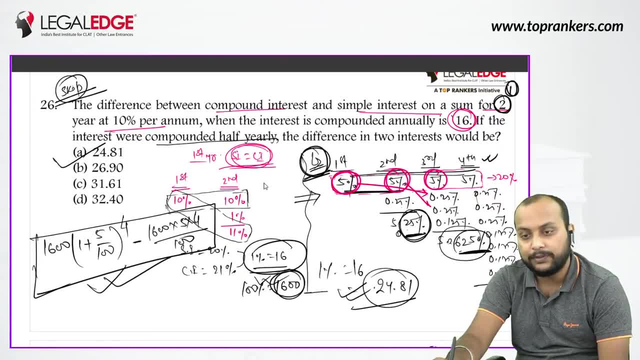 After that, if you get 5% interest in the second year, then this 5% will come here, And if you get interest in its interest, then this interest will come here. If you add all these, then this value will come here: 5.625%. 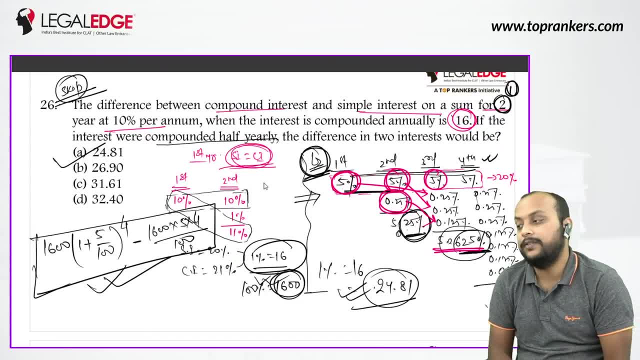 Okay, In this way we calculate its compound interest. This is a chain rule. This is called the chain method, Right? So this is easy as compared to the normal formula method of solving questions. There is another method. If you remember the powers, then do the power 4 of 1.05.. 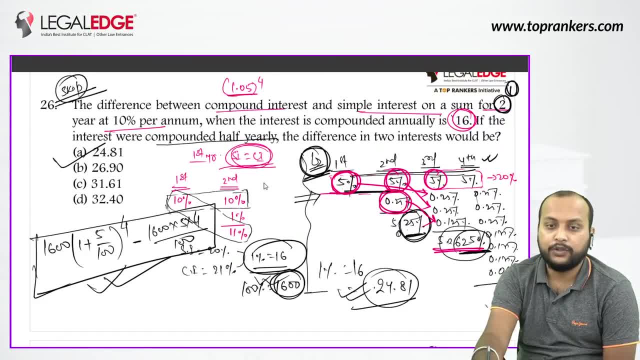 There is a 5% interest rate, right? So do the power 4 of 1.05 for 1 year. Power 4 of 105.. If you know how to do this, then you can do this too. So the third method of 1.05 is method 3.. 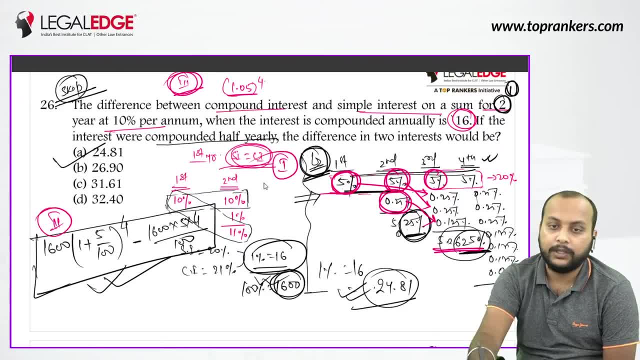 This is method 1.. This is method 2.. And this is method 3.. So let's do the power 4 of this. If you have 5% interest, then it will be 1.05.. So do the power 4.. 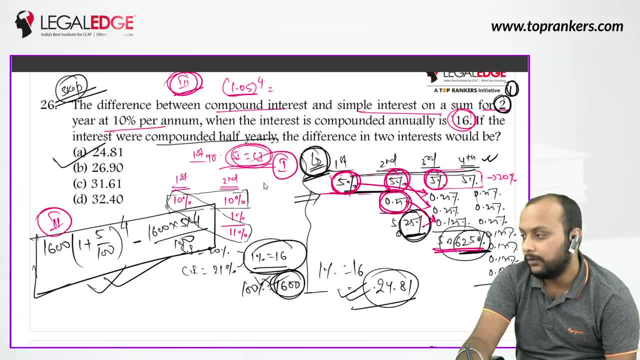 Now, what will be the power 4 of 1.05?? Can you square it? Can you square 1.05?? What will be the square of 105? 110.25.. 110.25.. No, it will be 1.1025.. 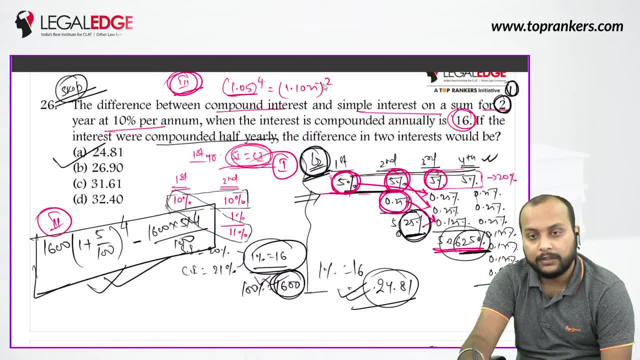 Again. we will square it one more time. I had squared it, That is, I wrote the square of this power 4.. I squared it. Now you will square it 1.1025.. So the value will come here. It will be calculated in difference. 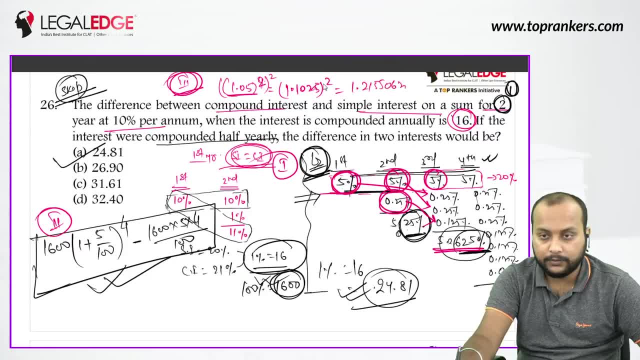 It goes 1.21550625.. So you will equate this value of difference with 16.. That is, 1% equals to 16.. Then 1.21550625.. 1.21550625 equals to what? 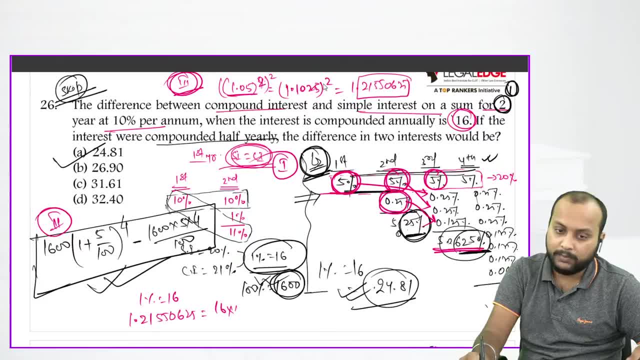 So 16 divided by 1, multiplied by 1.2155.. So this will give you the answer, Actually, whatever the answer will be. So this will give you the answer. Calculate the square, So 21.84.. So this is a long calculation. 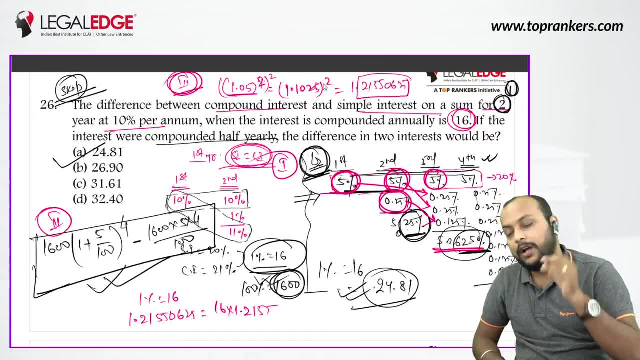 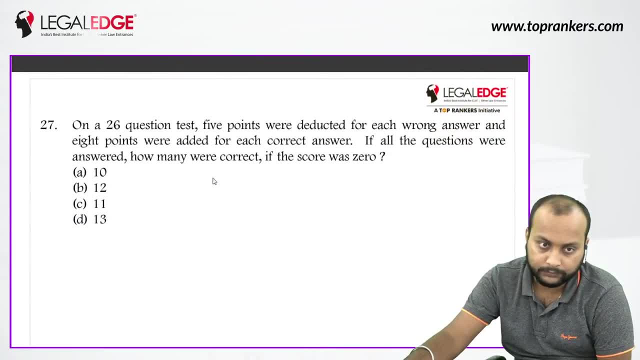 When you ask the question of compound interest, close your eyes and skip it, Because it will take time. The rest of the 9 questions will be lost. Thank you, 7. 27.. The question tells 5 points were deducted for each wrong answer. 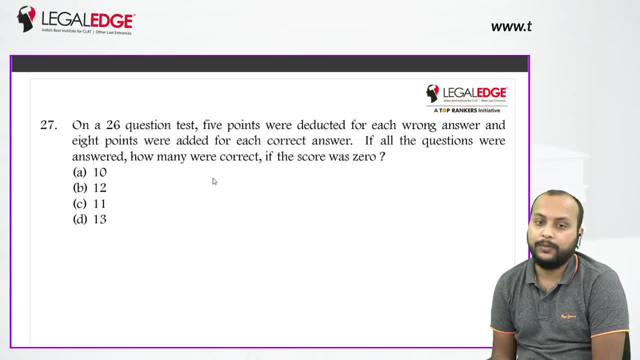 And 8 points were added for each correct answer If the questions were answered. All the questions were answered. So now we are getting 8 points for right and 5 points for wrong. Zero has come. You can't know that? you must have done more wrong. 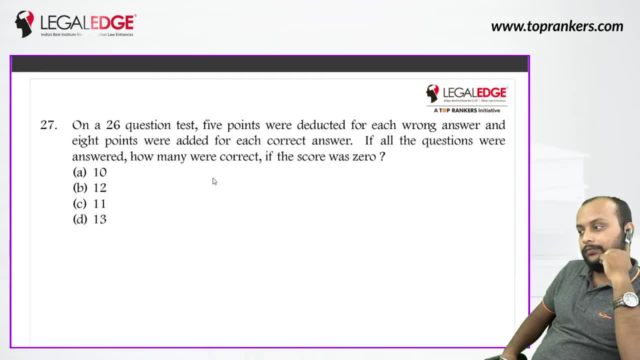 You can solve this problem easily with the help of options. Yes, 10 is the correct answer. You have 26,. right, Take the first option. If you have asked for correct, then correct, incorrect and total Correct. Take the first option. 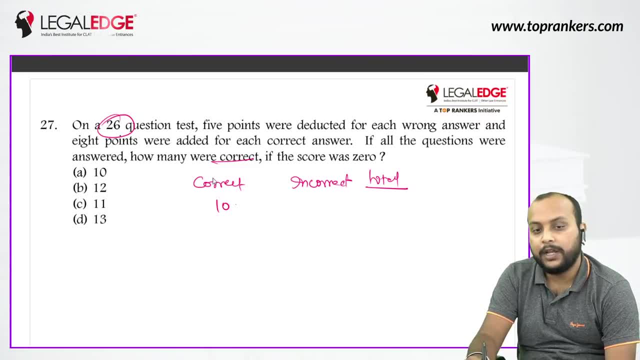 See, if you correct 10,, then how many marks will come. 10 into 8,. 80 has come, So how many total mark questions are there 26.. So if you correct 16, then what will be 16 into 5?? 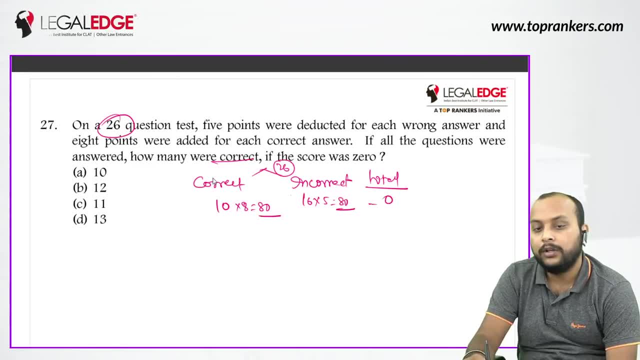 It will be 80. So what will be 80 minus 80? Zero. If you take the other question, 12,, then what will be 12 into 8? It will be 96. So how many questions are left? 14.. 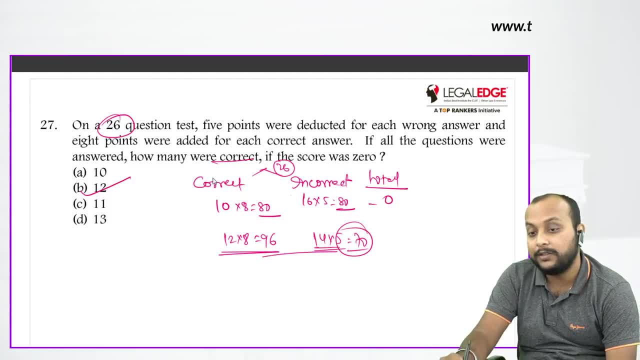 So if you multiply 14 by 5, it will be 70. So its marks have increased. How many have increased Plus 26. It has brought 26 marks. So what will be the answer from this list? 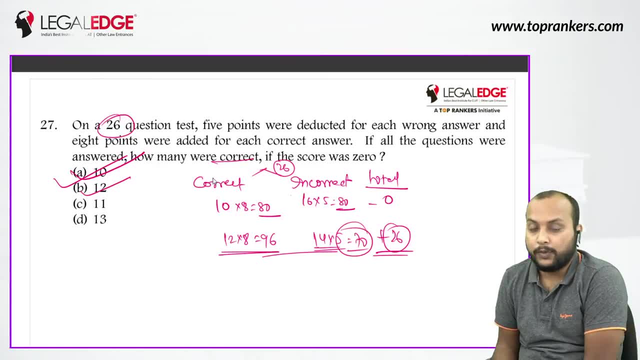 Go with the options, You will solve it easily. So, question number 27,. option number A: 10 is the correct answer. 10 is the correct answer. Okay, Let's go, then. All the very, very, very, very best. 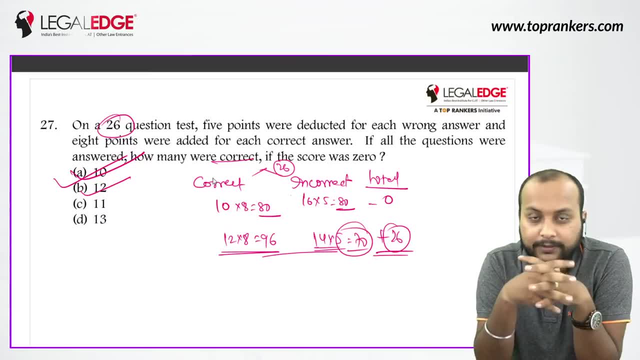 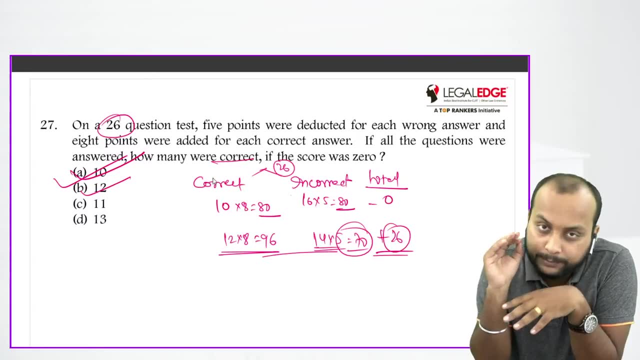 Wish you a very, very, very good luck for your elite examination. Prepare well. All the preparations are done. Now you have to just practice. Keep your mind stable, Always keep the clad papers of those whose clad papers are broken or something has happened. 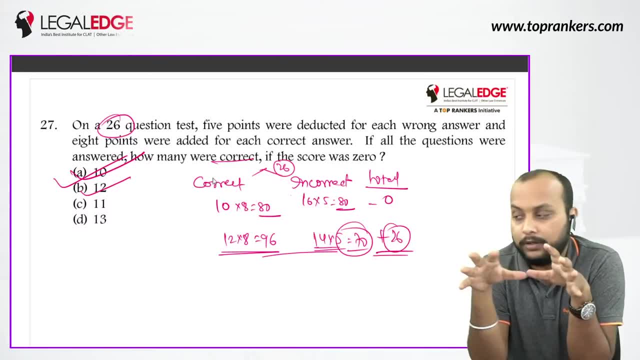 above or below. Mainly reasons- mostly- I am saying not everyone is like this, I am telling in generalized terms- Reason behind that was pressure Management of time. Someone was complaining that 10 minutes of time had been wasted. It happens. 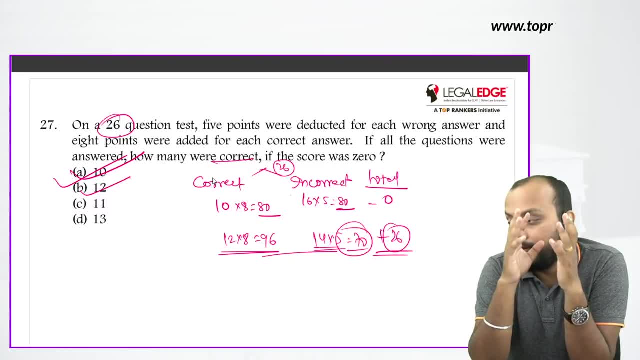 Make it a mind-makeup and go, Yeah, That thing make you think that it will happen. It will happen in offline. Sign will come. You will get the OMR Right. Mr Faizan Mustafa had said that at 2 o'clock. the transparency envelope that you will be given, 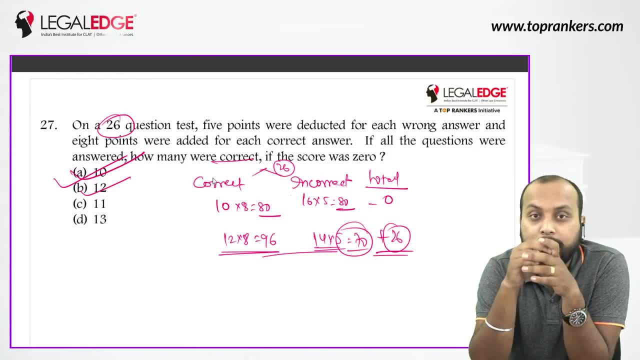 to break it, to seal out it, to remove the papers, In that you have to remove the OMR and paper, In that you have to remove the OMR and paper And you have to remove the OMR and paper. 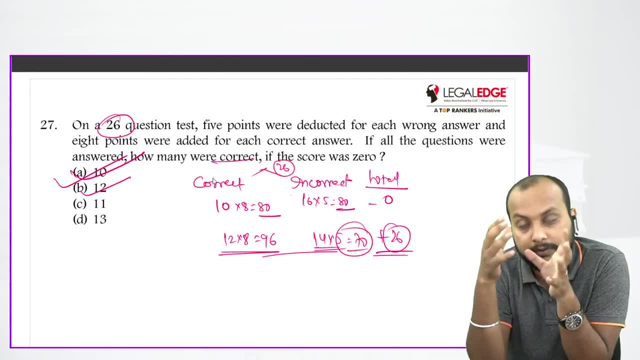 Because you will have to take it out. You will have to do this. You have to do this. You have to do this. You have to come and do it. You will have to do this. there will be OMR and paper, both. 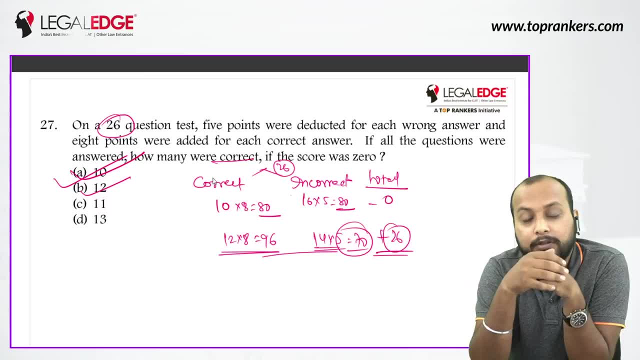 so mostly, if all the exam centers followed that, then you will get OMR only at 2 o'clock to fill the form. I am talking about CLAT paper, so you will not get extra time to fill OMR. in some centers OMR is given first. 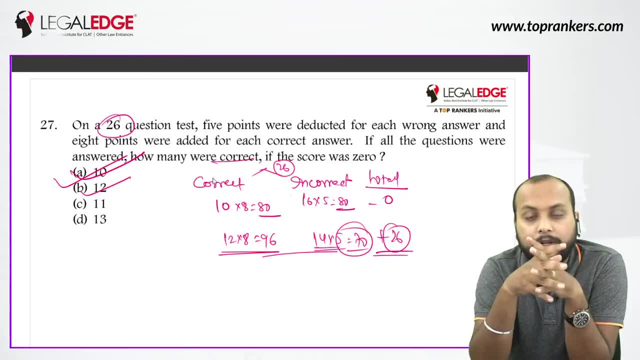 that was called by the center. but for this you have to be mentally prepared. keep a buffer of 10 minutes from the beginning. do this in practice mode. if we talk about math sections then we have to give 10 minutes in the math section- 10 minutes. 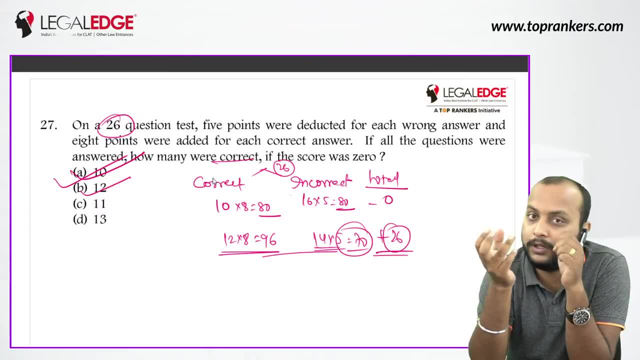 try to put the timer and start putting the questions from now, in 10 minutes. not 10 questions. you have to attempt 9 questions. one question will definitely be calculated. there is a guarantee. this is the background of the elite, like many people. one question is calculated. 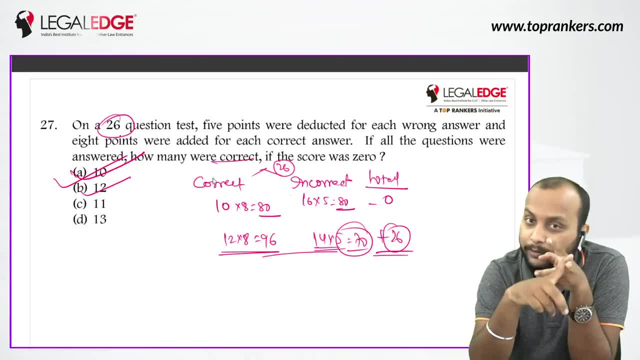 either the level of difficulty is tough or they ask the calculation if it is done, if there is a mistake or if it is clicked. if there is a shortcut method, same try to attempt in the calculation. otherwise, 9 attempts out of 10 minutes you have to do. 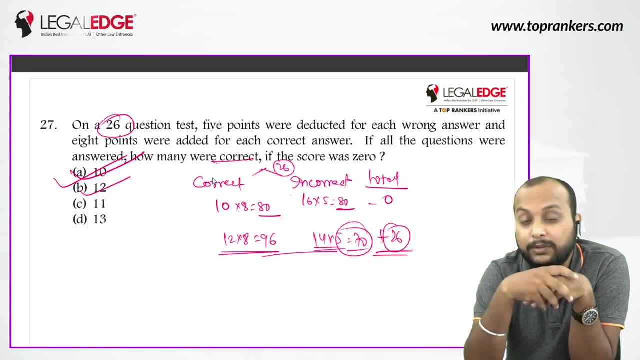 right. you can do 9 attempts easily. 4 to 5 questions are on easy to moderate level. 4 to 5 questions are on easy level. 3 to 4 questions are on moderate level and 1 and 2 questions are on difficult side. 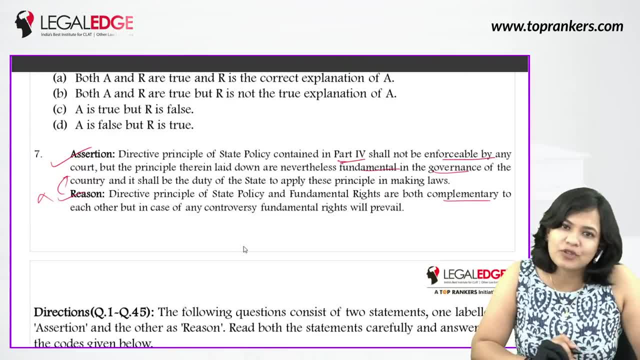 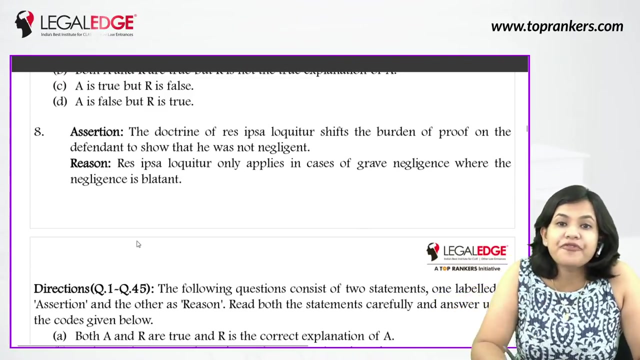 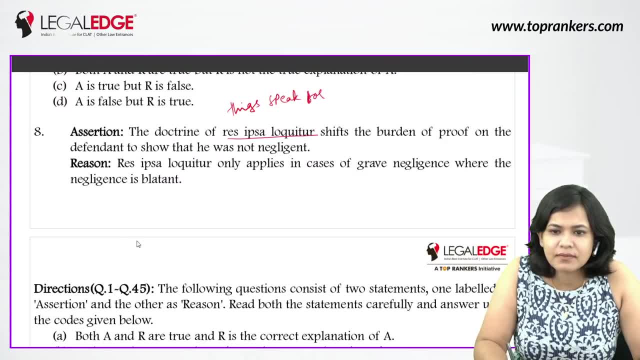 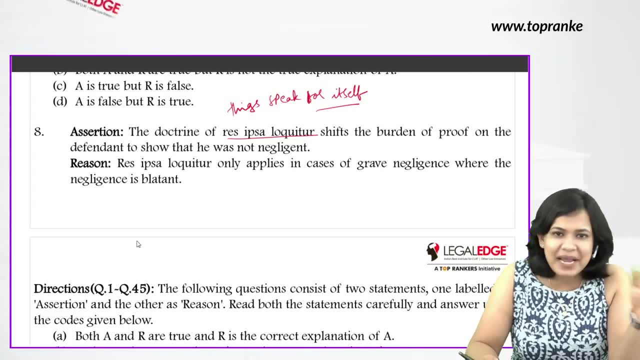 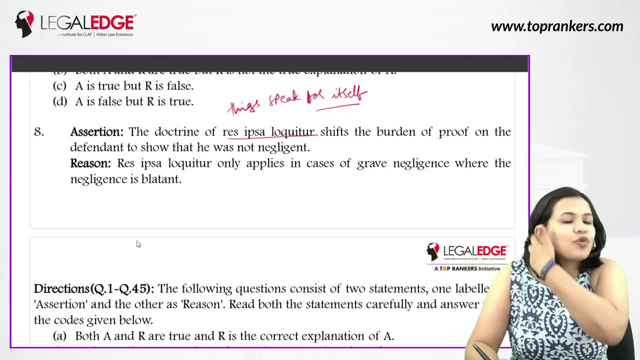 a all far all things that you can see on the face and you don't need to prove it, like when you were having a stomach ache, you had an appendix problem. you had an operation and the appendix was removed and you were still facing trouble. you can actually see a pair of scissors in your stomach. 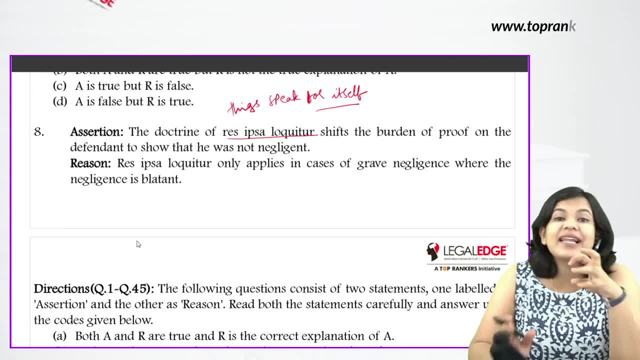 last time when you had an operation, the doctor negligently left the scissors there. if you can see the knife in it, then you have to prove that the doctor was negligent, because if you can see on the face that the doctor has done something wrong, then the Recipient Locator is applied. 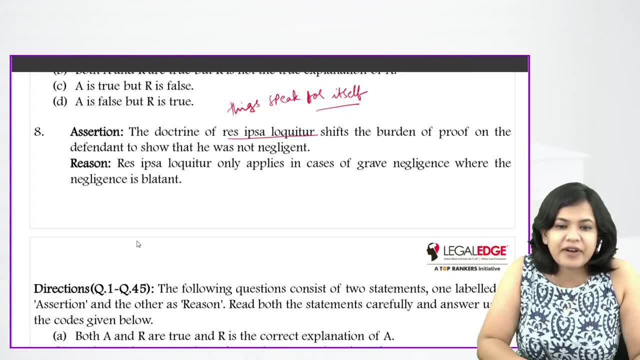 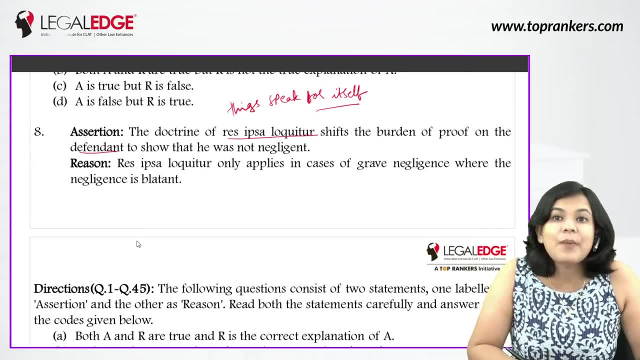 so it says that the doctrine of Recipient Locator shifts the burden of proof on the defendant to show that he was not wrong. so the whole burden has now been lifted on the doctor. that tell me when you were not negligent, because it is clearly visible on the face that you have done negligence. 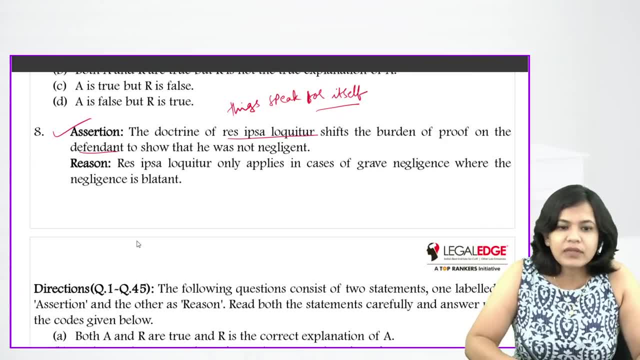 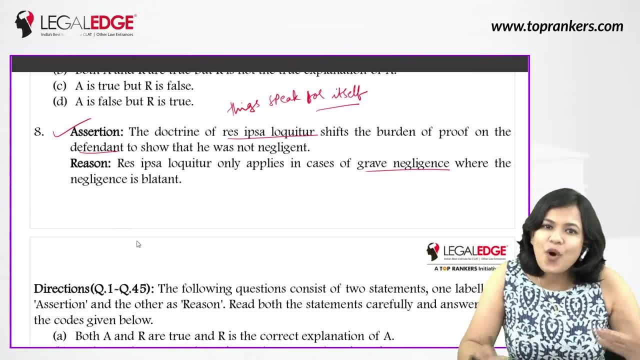 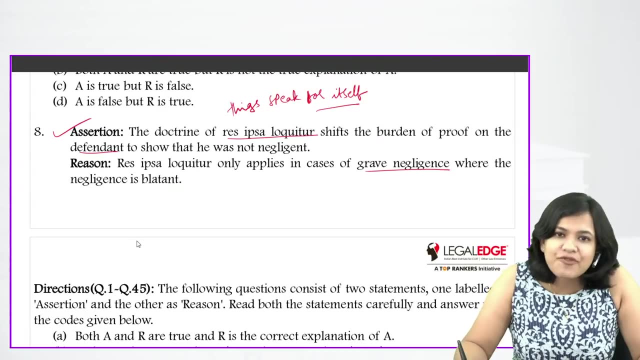 so is this statement correct? yes, next, it says that Recipient Locator only applies in cases of grave negligence. no, Recipient Locator has nothing to do with grave negligence and small negligence. Recipient Locator in general applies in all negligence cases, whether they are grave or small. 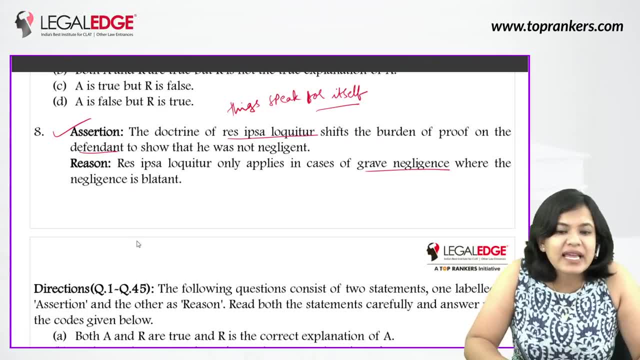 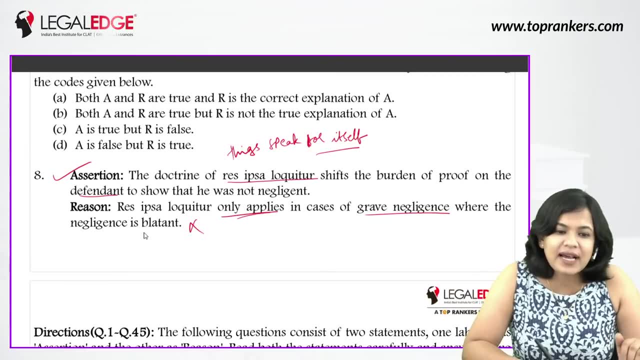 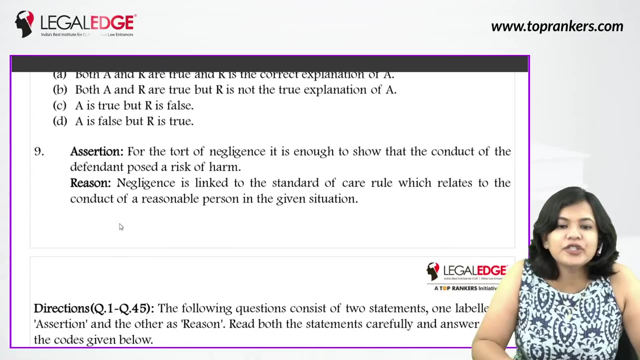 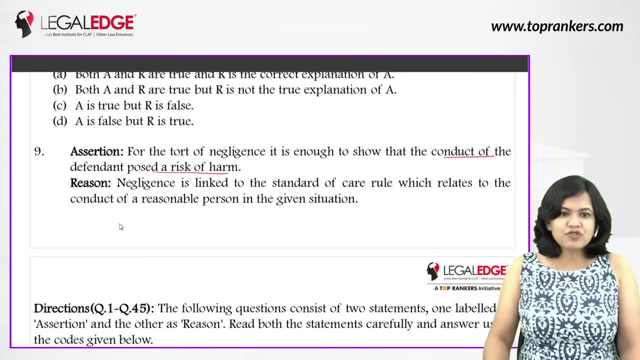 Permanent law isn't a crime. if you say I have to file a negligence case, then I should merely do the following. he's the person. as you see. he wasもし we were to possess harm. it was sembing that he could do some grea by then. ati actually bre arribi. 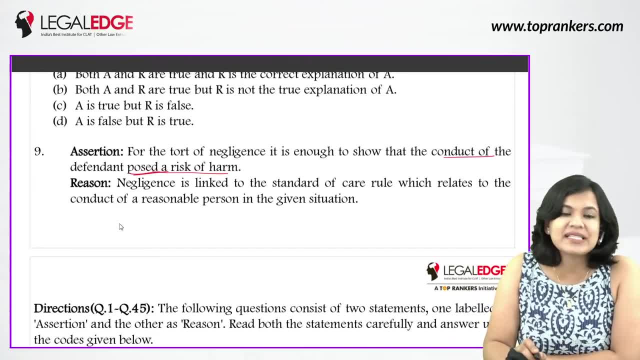 The duty to breach, when would actually be considering him as a threat or service of harm? It's that, simply, his work is not enough. we are just knowing that this person looks that he would cause us trouble is not enough, And this statement is wrong. Now, if this statement is wrong, then I have. 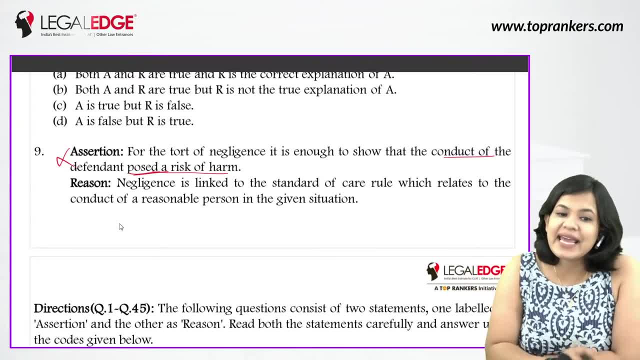 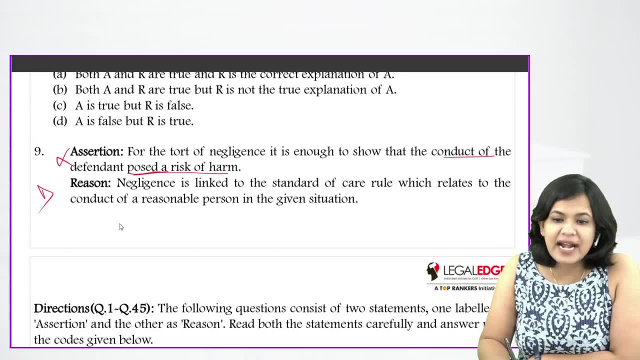 seen more. So I just told you that there is no need to worry. If A is wrong, then the answer will be D by itself. But let's read the reason. Reason says negligence is linked to the standard of care rule, which relates to the conduct of a reasonable person in a. 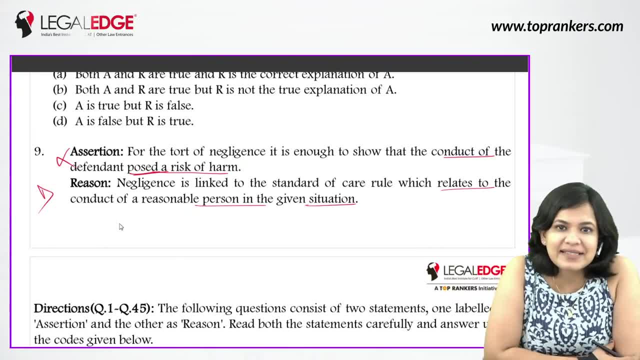 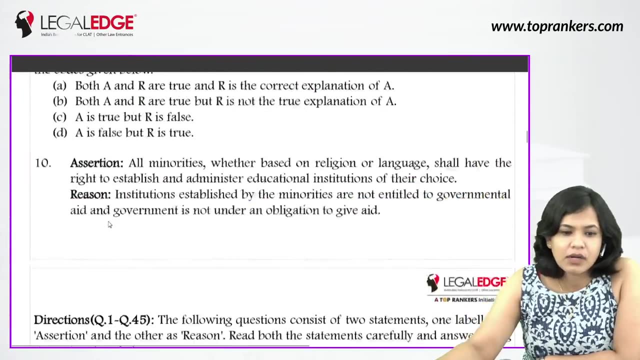 given situation. Yes, we trust more on conduct than on that thing. What we were apprehending is not enough. The actual conduct of a person should be bad. Then we will say that he is liable for negligence. So answer is option D. Coming to the 10th question, it says all. 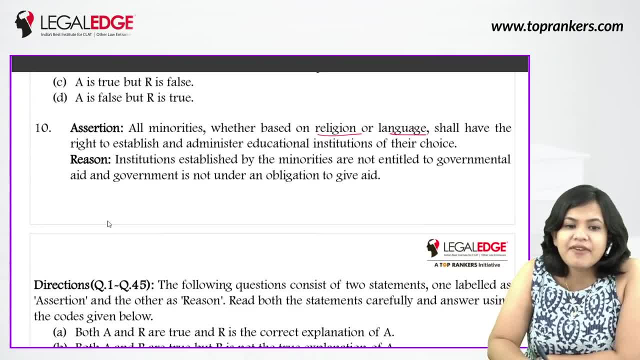 minorities, whether on religion or language, shall have a right to establish and administer educational institutions of their choice. Now let me tell you one thing: Religious minorities are allowed. If you want to make institutions of your religious minority, then you can make them. Now let me tell you one thing: Religious minorities are allowed. If you want to make institutions of your religious minority, then you can make institutions of your religious minority. Now let me tell you one thing: Religious minorities are allowed If you want to make. 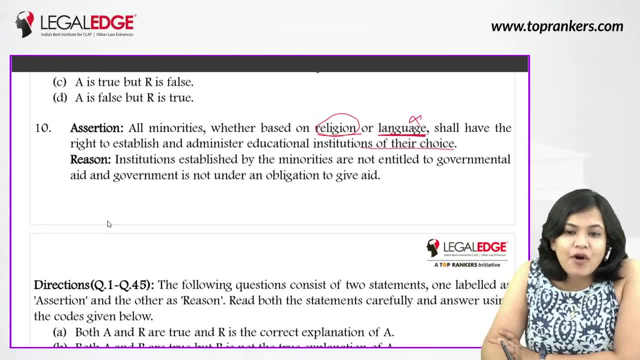 institutions of your religious minority, then you can make institutions of your religious minority. Now, let me tell you one thing: Religious minorities are allowed. If you want to make institutions of your religious minority, then you can make institutions of your religious minority. Now, let me tell you one thing: Religious minorities are allowed If you want to make. institutions of your religious minority, then you can make institutions of your religious minority. Now let me tell you one thing: Religious minorities are allowed. If you want to make institutions of your religious minority, then you can make institutions of your religious minority. Now let me tell you: 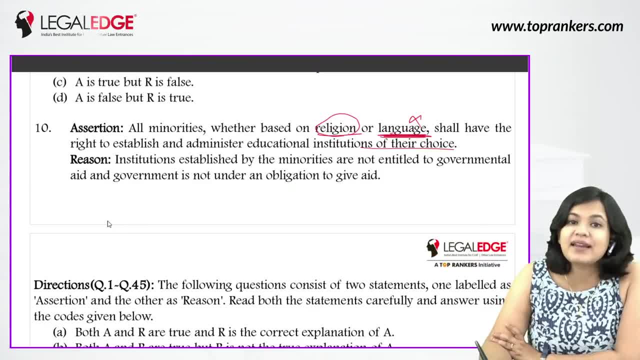 one thing: Religious minorities are allowed. If you want to make institutions of your religious minority, then you can make institutions of your religious minority. then you can make institutions of your religious minority. Now, let me tell you one thing: Religious minorities are allowed If you want so Überster. 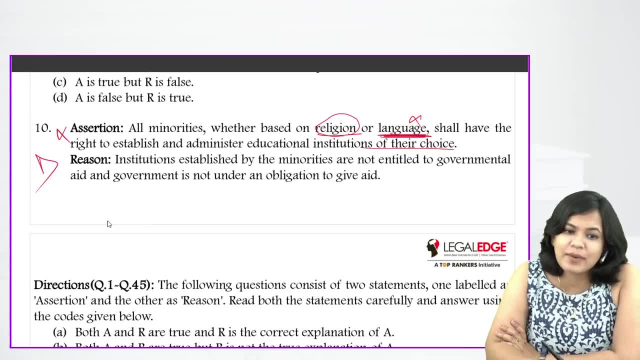 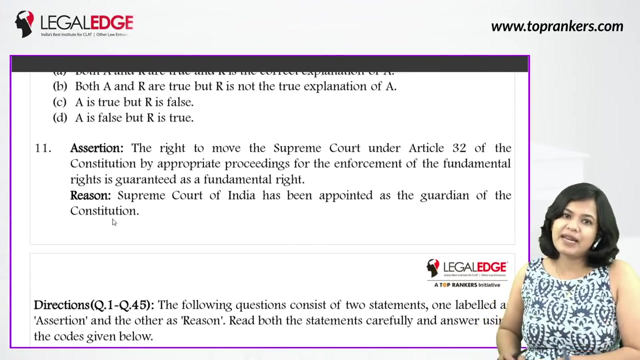 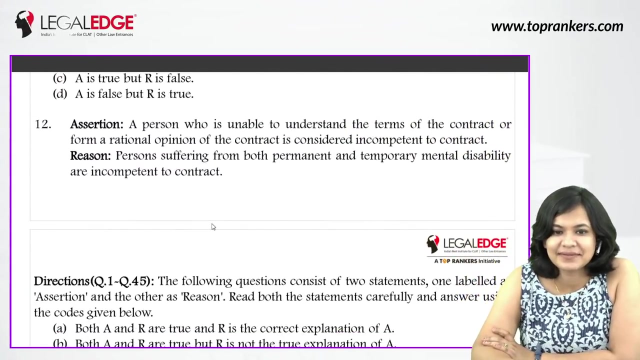 Recht, then you must か learnACH understood yes and correct D. Come to question 11.. Solve 11 questions 11.. A After 11th 12th. D After 11th 12th. 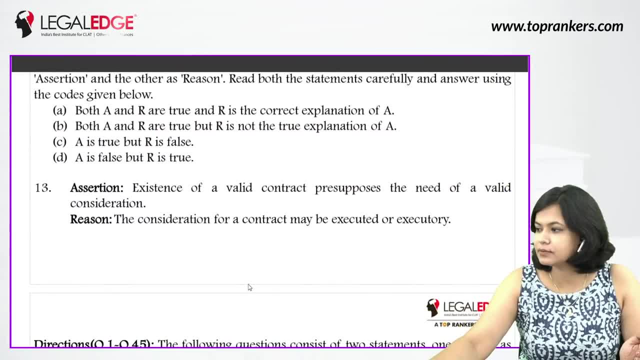 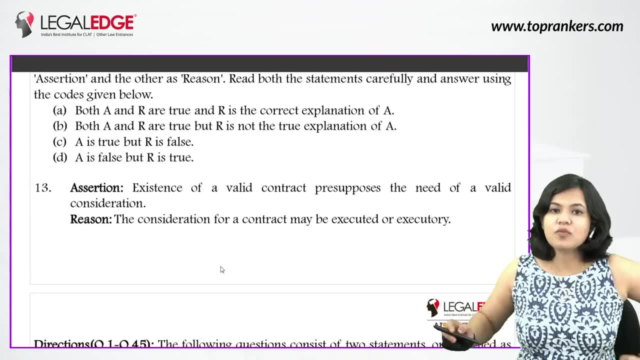 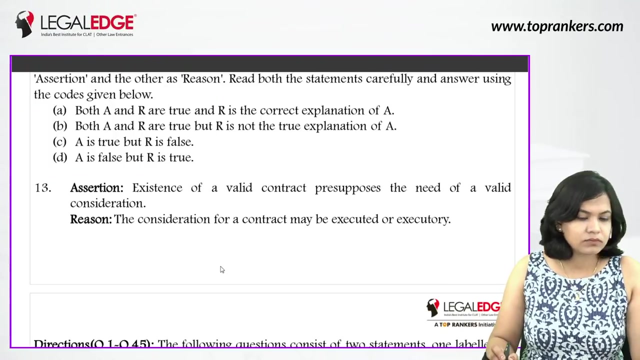 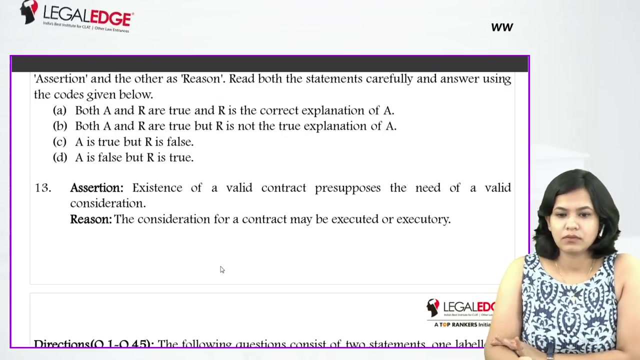 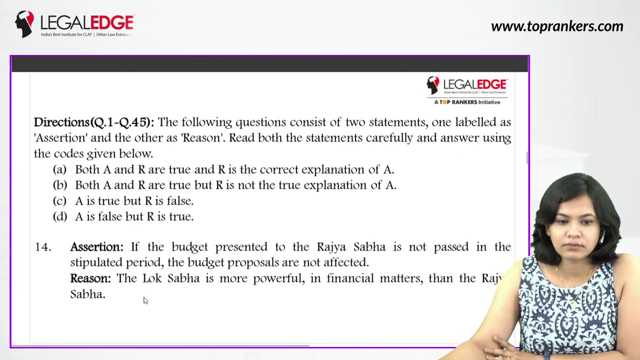 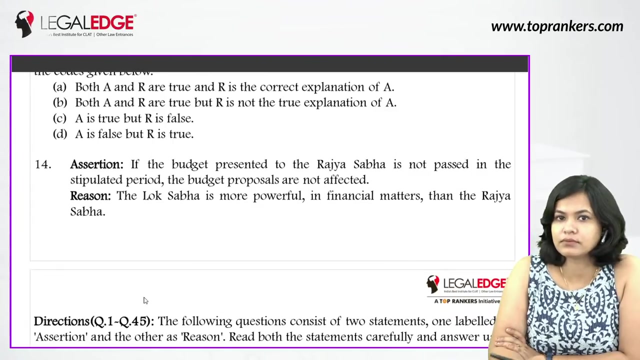 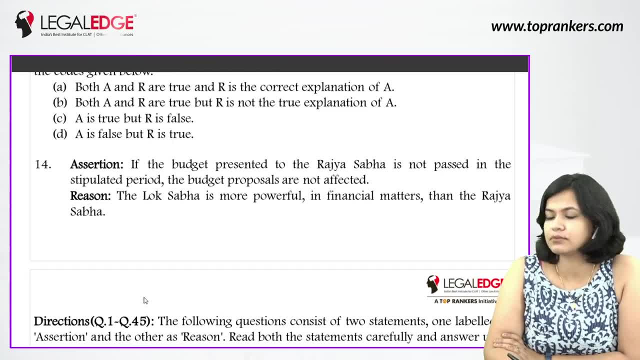 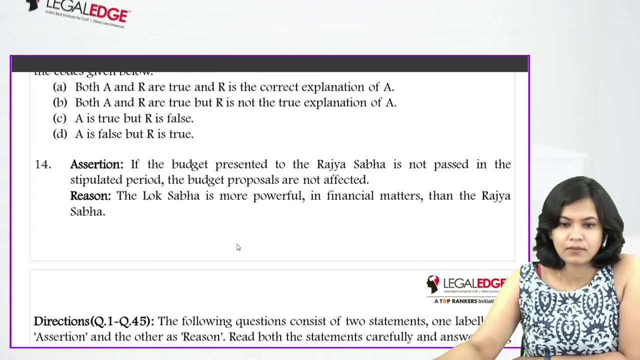 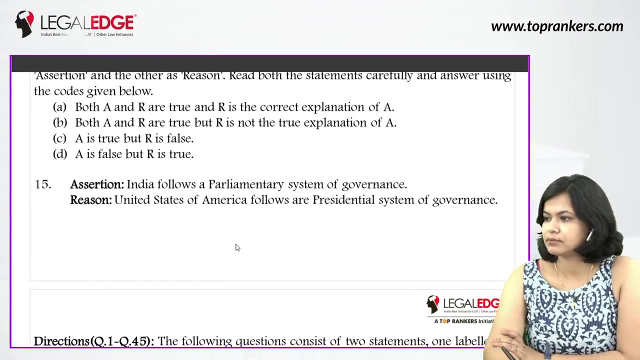 Today it's just a session reason. Today it's just a session reason 13th, 14th, 15th, 16th, 17th, 18th, 19th, 20th, 21st. 22nd, 23rd, 24th, 25th, 26th, 26th, 27th, 28th, 29th, 30th, 31st, 32nd, 32nd. 31st, 24th, 25th, 30th, 31st, 26th, 24th, 25th, 26th, 27th, 28th, 29th, 30th. 31st, 30th, 32nd, 31st, 34th, 35th, 35th, 36th, 36th, 36th, 37th, 38th, 39th. 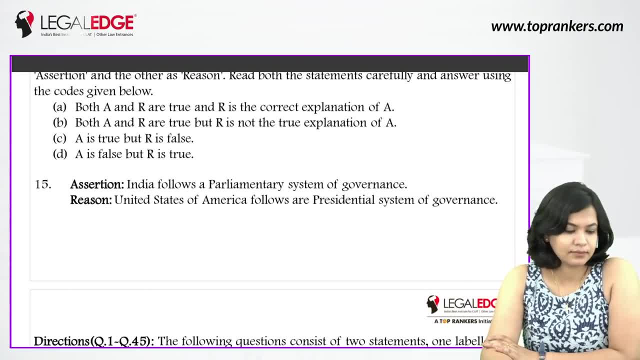 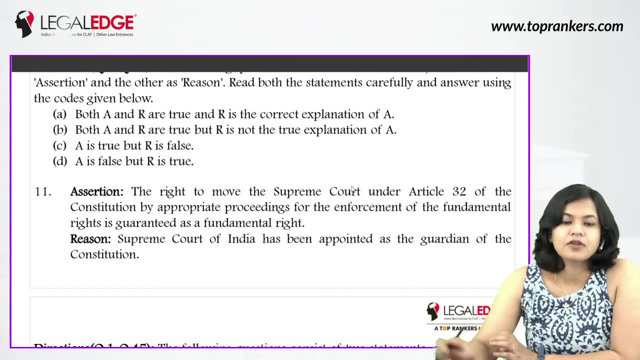 40th, 40th. 11. The right to move to the Supreme Court under Article 32 of the Constitution by appropriate proceedings for the enforcement of the fundamental right is guaranteed as a fundamental right. Yes, we have the option of writ petition If there is any violation of the fundamental. 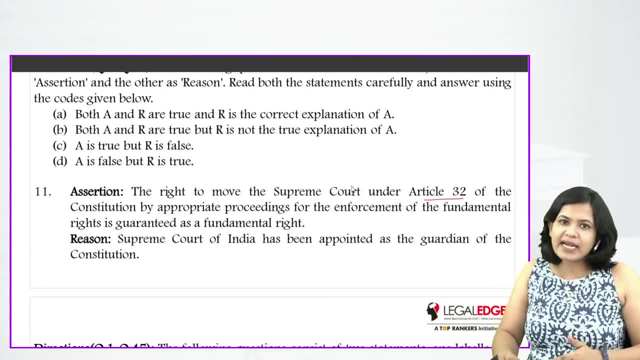 right. if the state violates it, then we can go ahead and file a case of writ against the state for the violation of fundamental right. Is this right? Yes, this is absolutely right. Supreme Court has been appointed as the guardian of the Constitution. Has the Supreme Court? 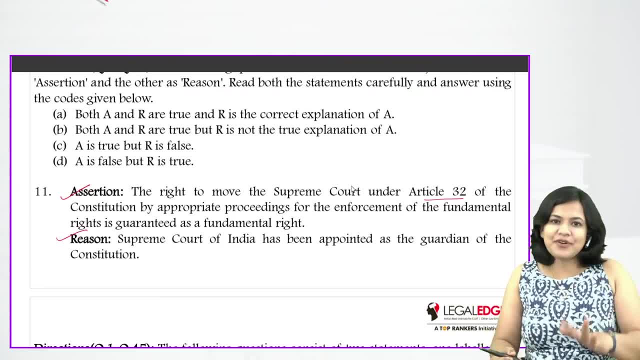 appointed the guardian? Yes, Now, this is one of those questions which you have to ask yourself. But if you connect this, then you will understand that, yes, both of the statements go hand in hand. How It is explaining the reason, the assertion. The assertion says that in Article. 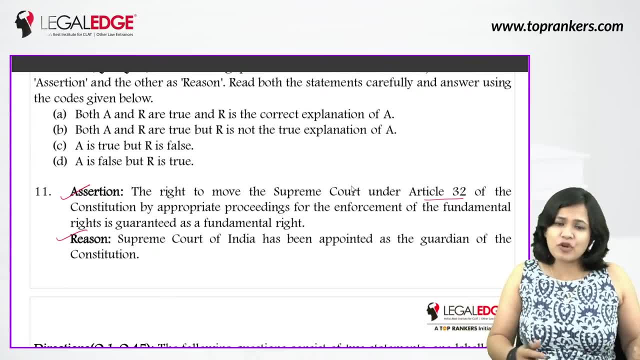 32 of the Constitution. Article 32 is given under which you can go and file a case in the Supreme Court for the violation of fundamental rights. And why can you file a case in the Supreme Court for the violation of fundamental rights? Because the Supreme Court is the protector. 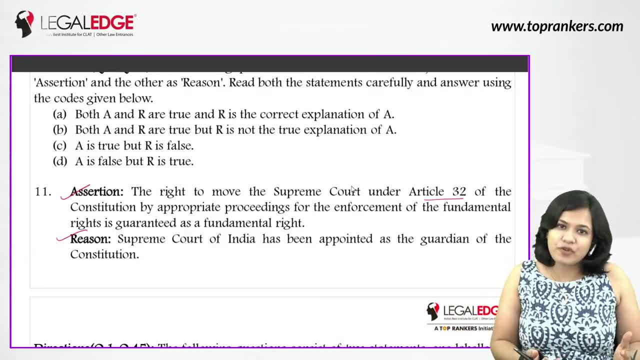 of the fundamental right, So you can file a case in the Supreme Court for the violation of the Constitution. Supreme Court is the guardian of the Constitution, And is that why the ultimate power is with the Supreme Court? Yes, So are both these statements right, Both. 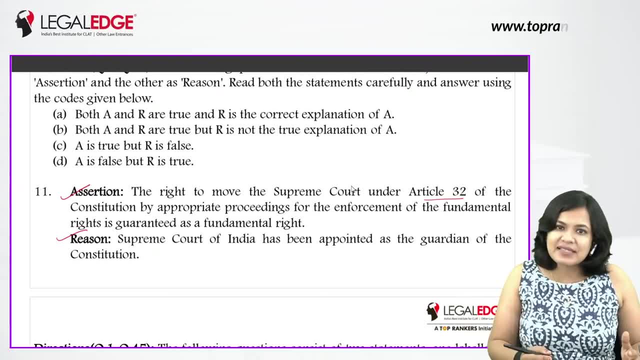 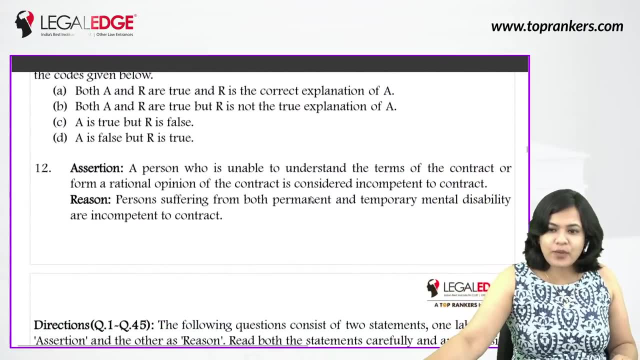 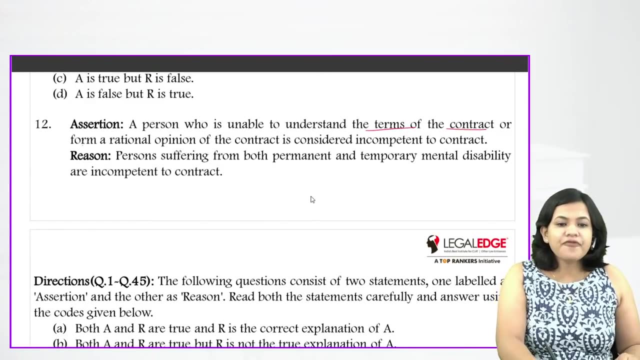 the statements are right. Does reason explain the assertion? It does So? answer would be option A. Moving on to the 12th question. 12th one says: a person who is unable to understand the terms of the contract or form a rational opinion Is the person who is unable to understand the terms of the contract or form a rational opinion. 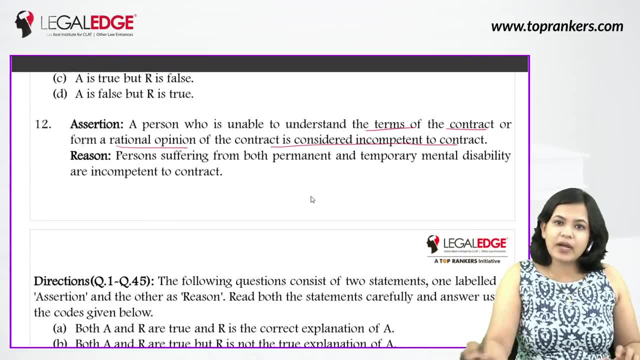 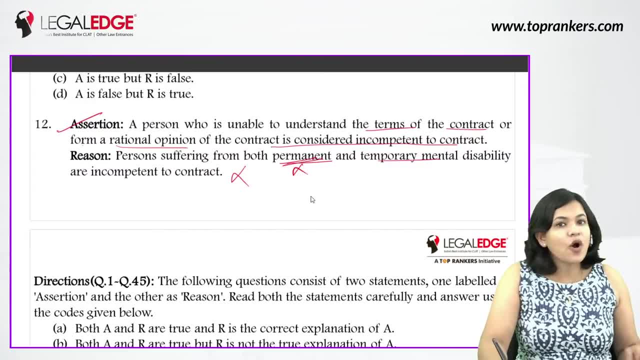 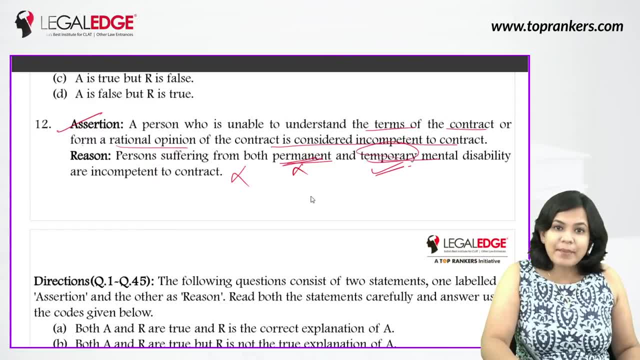 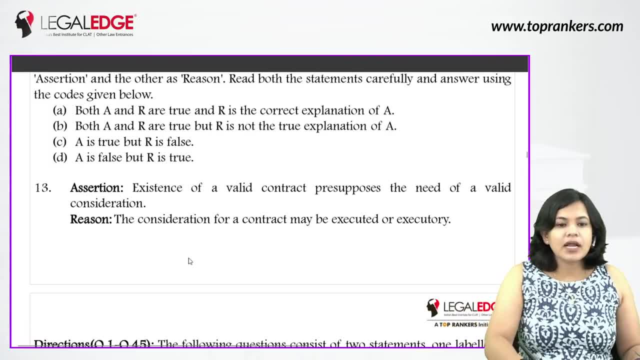 for you to understand that. what kind of questions will be there? now coming to question number 13: 13 says existence of a valid contract presupposes the need of a valid consideration. of course, if there is a valid contract, then we will expect that there will be a valid consideration also. 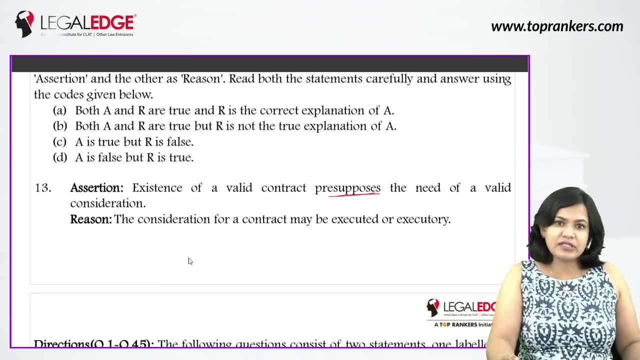 now, definitely there is an exception that some contracts are done without consideration, but we are talking in general, in general, whenever there is a contract, then is there a valid consideration? with a valid contract, yes, it happens in general. the consideration of a contract may be executed or executory executed means such a consideration which is past you. 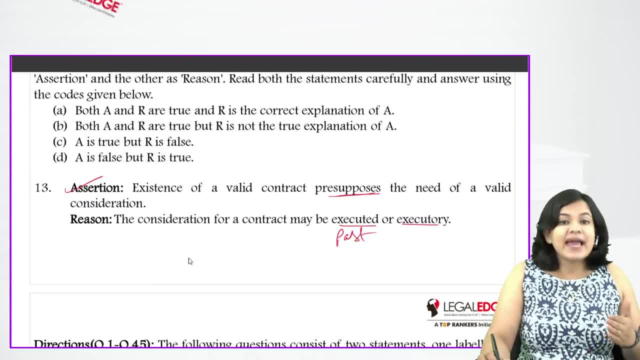 have already paid the money. you are getting the work done later. executory. you are getting the work done now. the money you are paying or the consideration you are giving, you will pay in the future. you will pay in the future. so whatever consideration is executed- executory. 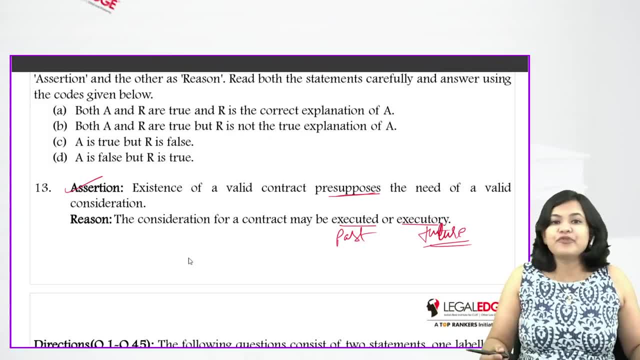 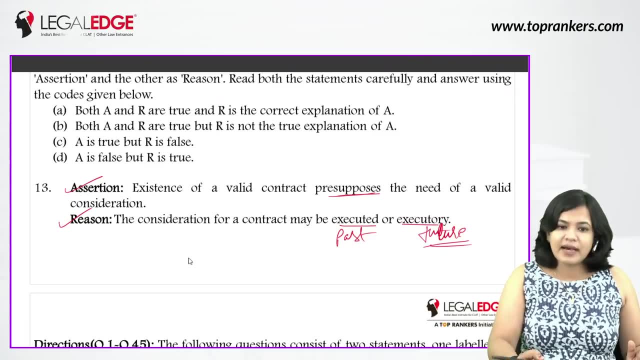 can it be? yes, yes, it could be in past, it could be in future as well, or these two statements are correct. now, does reason explain the assertion? no, it does not reason. assertion says: existence of a valid contract presupposes the need of a valid consideration. because consideration 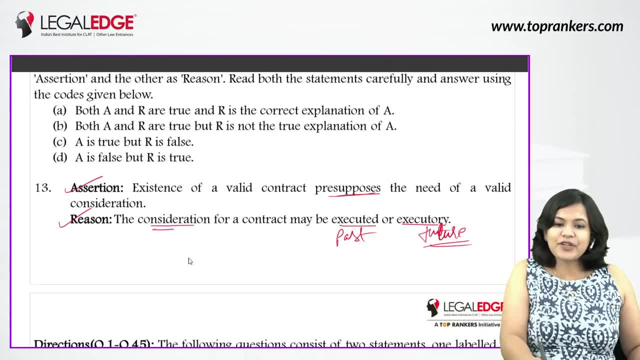 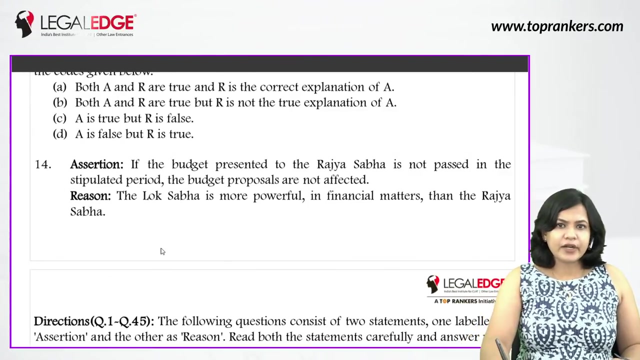 for a contract may be executed or executory. no, this is specifically talking about consideration. on the contrary, this particular statement is talking about the existence of a valid contract. are these two different concepts? yes, so answer would be b coming to the fourteenth question, fourteenth says: if the budget presented to the rajasaba 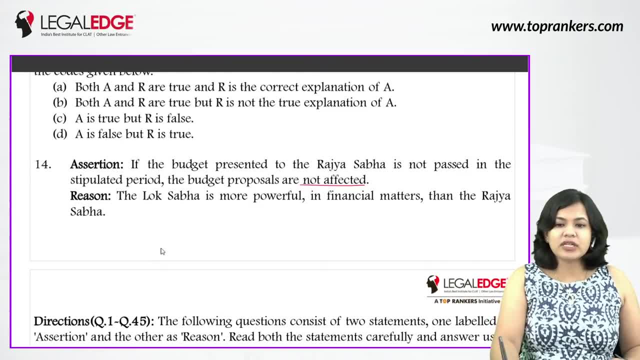 is not passed in the stipulated period, the budget proposals are not effected. yes, because whatever the money matters, does the loksaba handle all those money matters? yes, then is this statement right? this statement is correct. the next statement says: loksaba is more powerful in financial matters then Rajya Sabha. is this statement also correct? yes, but but reason does. 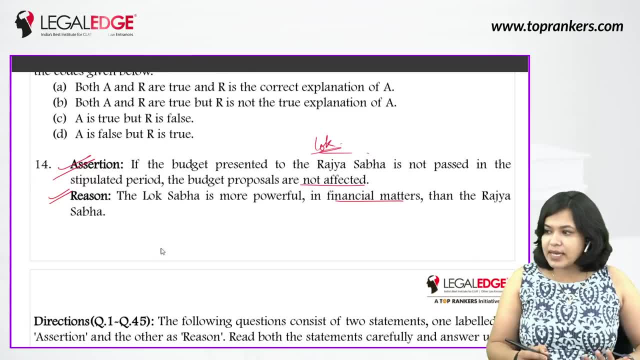 not explain the assertion here. reason does not explain the assertion here. I'll tell you why. assertion specifically: bol rahe hai ki Rajya Sabha mein, agar koi budget jayega, thik hai. toh stipulated time mein pass nahi hua. toh bhi usko koi kuch effect nahi karega, wo jaisa budget ka. 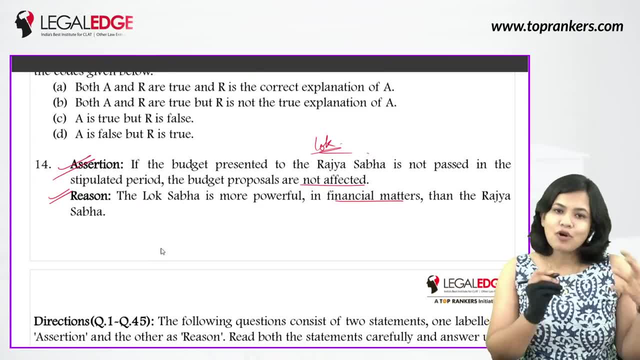 proposal hai, wo jaisa ki jaisa hi rahega, iska Lok Sabha ka more powerful hone se koi leena dena nahi hai. so both the statements are correct, but reason does not explain the assertion, and this is the reason. the answer should be B. 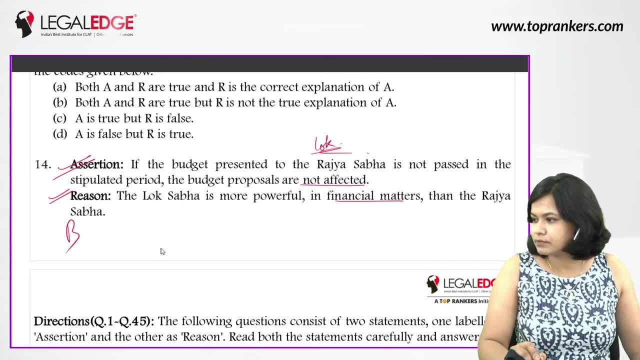 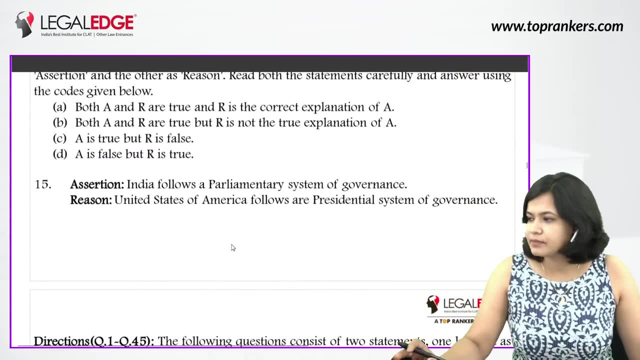 Tomia. in case of gift, a contract for gift, where consideration doesn't matter, Rudrika not much. but yeah, there's a possibility that other exams might give you itne difficult wale. toh assertion isan na bhi dek kya wo bohot simple se assertion isan de sakte hai. 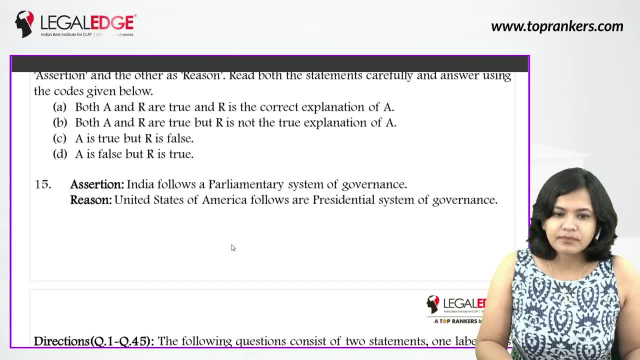 ha toh jo dusri exam se waha pe bhi tumhe kaam aa sakta hai. the 15th question says: India follows a parliamentary system of government. yes, parliament hai amare paas wo laws banati hai. wahi legislature hai toh, e toh sahi hai. 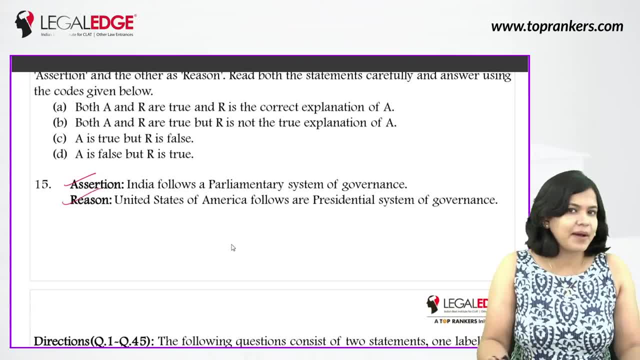 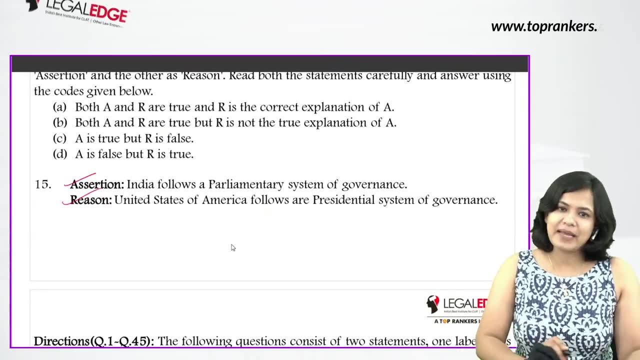 US me presidential form of governance hai. ha bhai, ye bhi sahi hai. aur ye boh ho aur thi easy question hai: dikhe, ki India me parliamentary system hai, US me presidential system hai. dono statement sahi hai, but dono ko kahe ek dusre se kuch leena dena nahi hai. 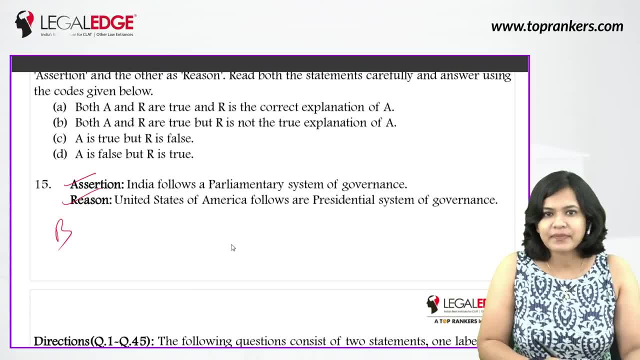 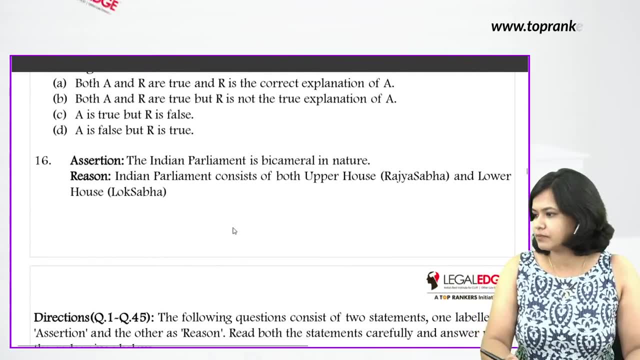 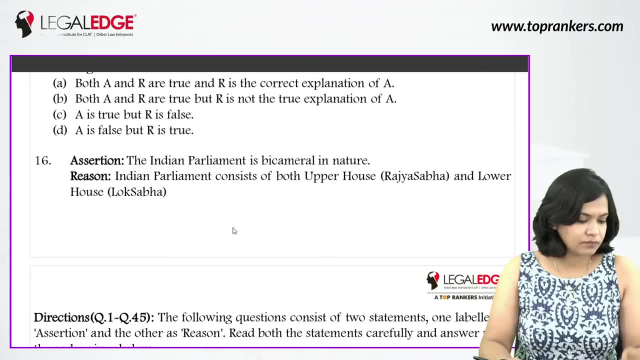 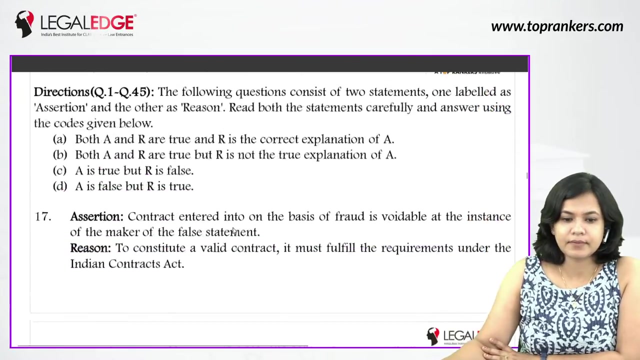 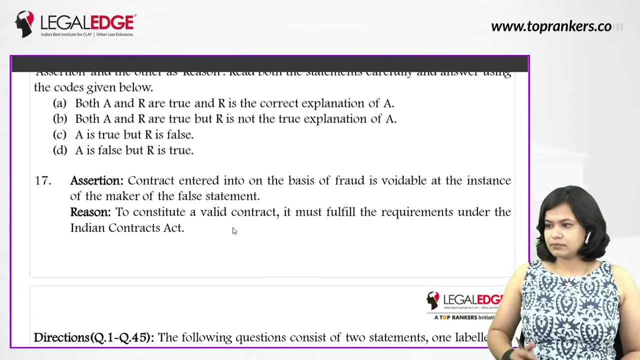 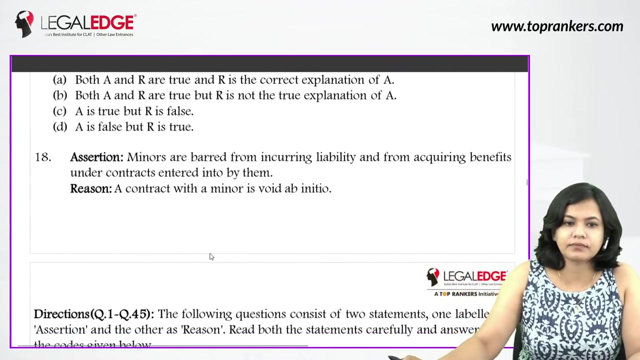 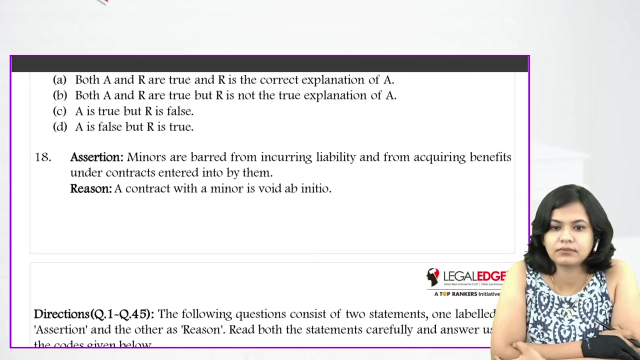 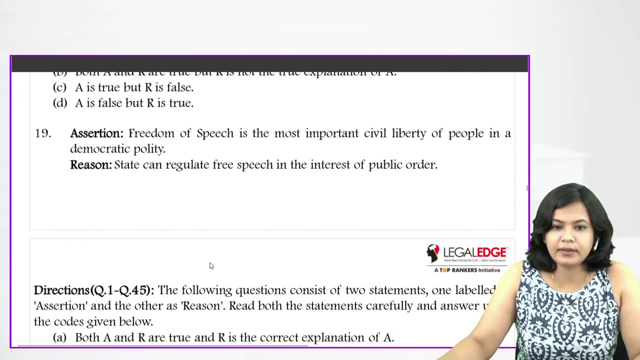 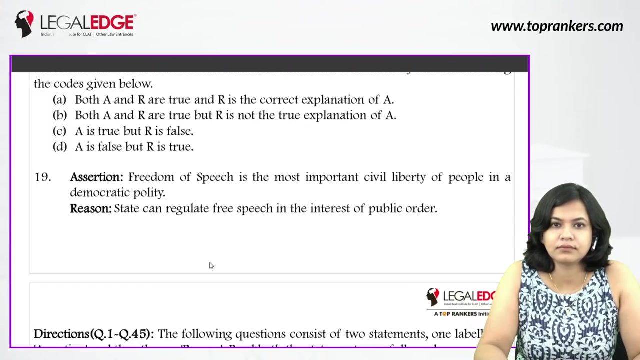 matlab reason is not explaining assertion, so answer is B. pretty easy here. chalo 16th, pe aao. solve 16th, 19th, done. you will have to solve faster for me to go faster. ok, 20th, ok, 20th, ok, 20th. 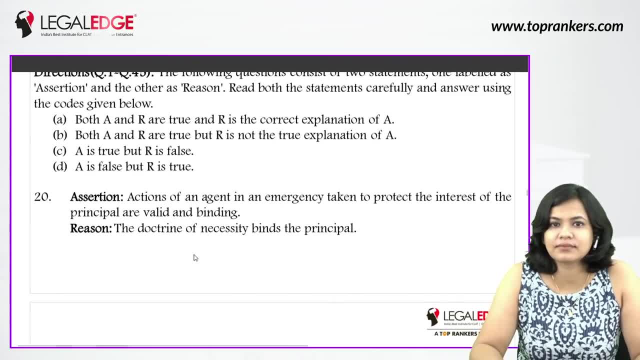 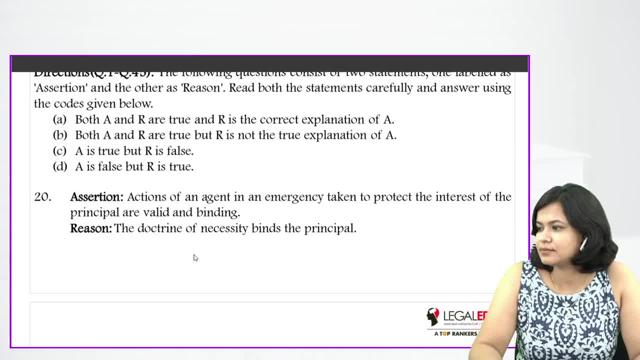 ok 37th, ok 38th, ok 28th, ok 31st, ok 32nd, ok 34th, ok 33rd, ok 38th, ok 48th, ok 39th. ok스를, ok 42nd, ok 59th. 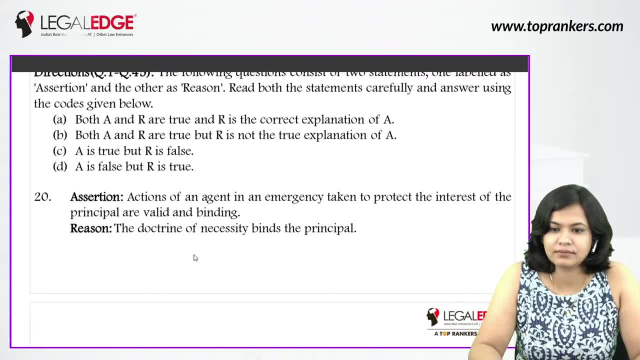 ok. 43rd ok 61st ok 42nd ok. 45th ok. 7th ok. ap 12th ok 85th ok. 49th ok 1st ok 6th. ok结res ok 51st okASE ok 51st. 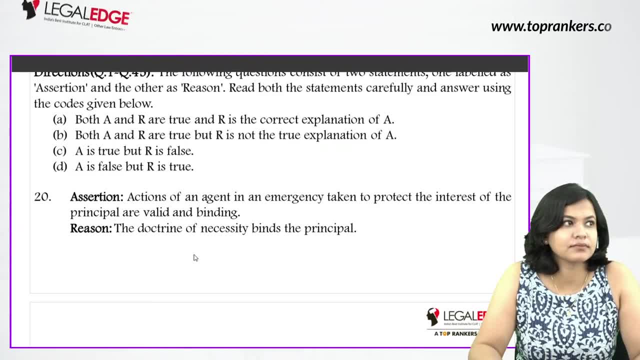 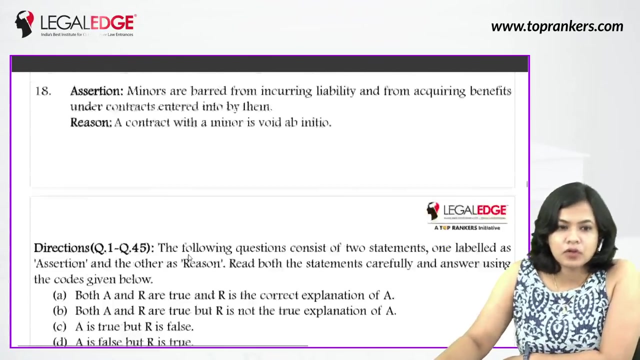 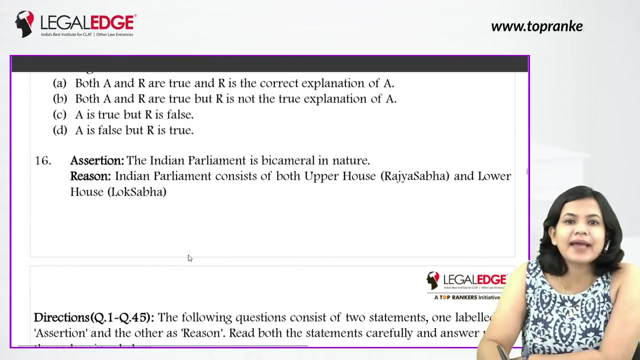 ok. 2nd, ok 42nd ok. 16th, ok, 42nd ok. ж coordinated ok. 1st, ok, 14th, ok, 14th, ok 15th. you So going back to question number 16.. Question number 16 says the Indian Parliament is bicameral in nature. 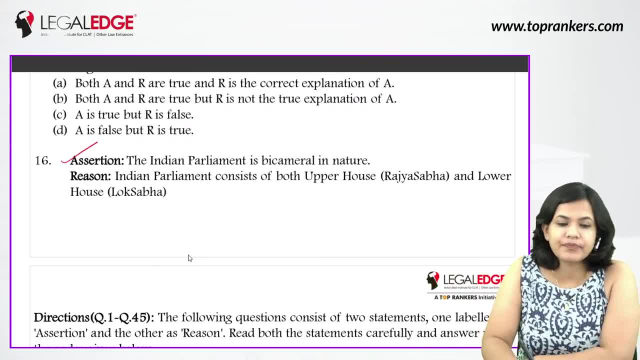 Okay, This is a good example. The reason: Indian Parliament consists of both upper house and lower house. This is also correct. Now Indian Parliament is bicameral. What is the reason for that? It is bicameral because we have two different houses. 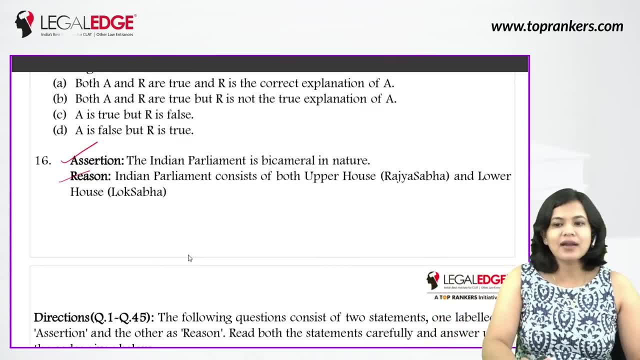 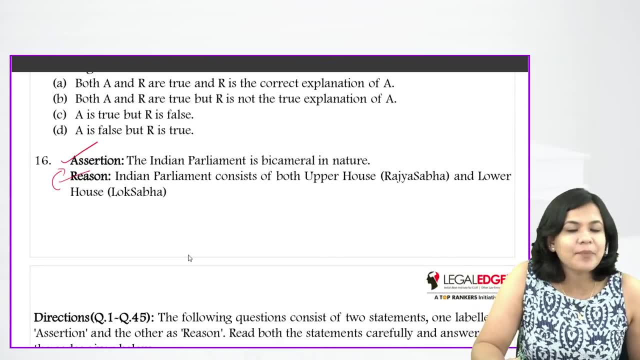 And what are those two different houses? Those two different houses are the Lok Sabha and the Rajya Sabha. So is this the reason? Is it an assertion In India? we are saying that Indian Parliament is bicameral in nature. That is true. 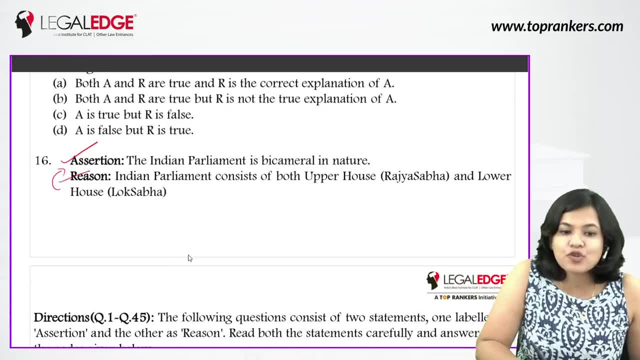 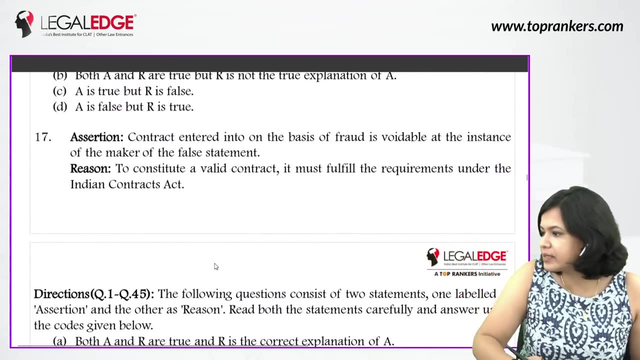 Yes, So because both of them are true and also reason explains the assertion. The statement of reason is a proper reason for the assertion. There is a proper explanation too, So the answer would be A. This is also pretty easy. Coming to 17th here. 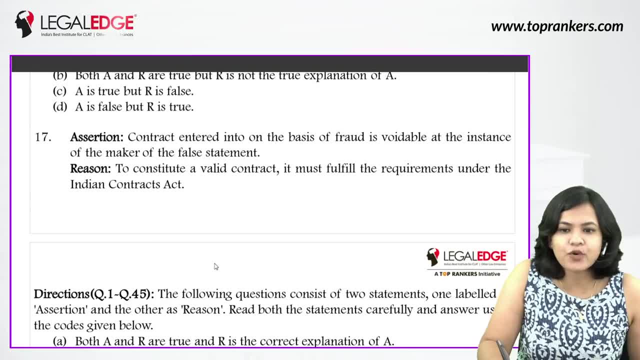 Come on 17th says contract inter into on the basis of fraud is void At the instance of the maker of the false statement. Now, a lot of you couldn't get this particular statement correct Because you didn't read it carefully. 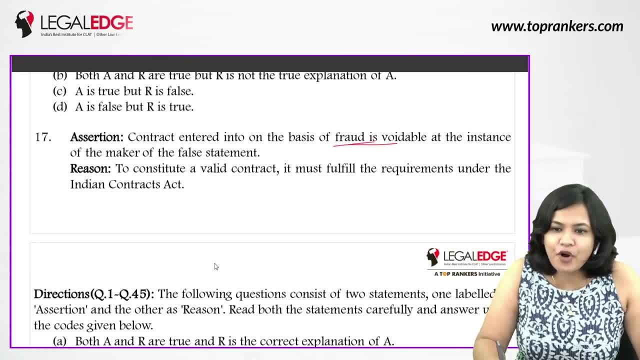 It says: contract inter into on the basis of fraud. If someone has done fraud, then such a contract is voidable, Which is true. Yes, such contracts are voidable. At the instance of the maker of the false statement, That means the one who was lying, he will say that the contract is voidable. 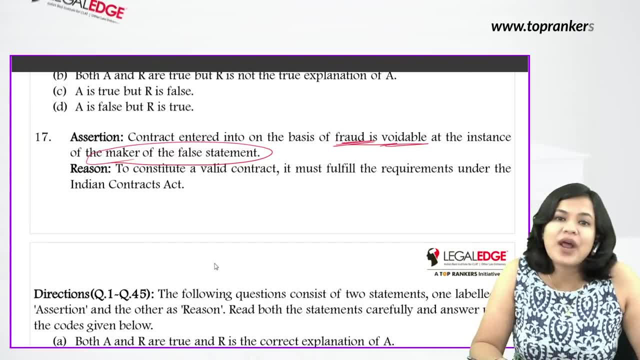 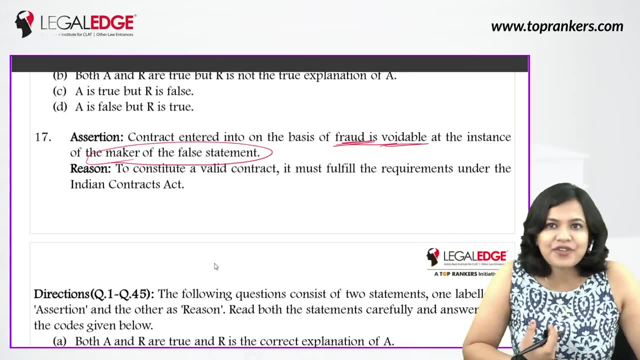 No, It is at the other, The person who has been told the statement. It's at the person. It's at the instance of the person with whom the fraud has happened. So if Aditi has contracted with me And Aditi has lied to me, 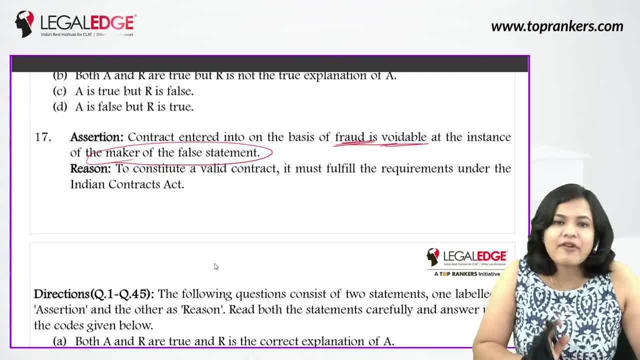 So it will be the responsibility of the witness, Because he decides whether to validate it or invalidate it. So is he the maker of the false statement, That means the one who is lying, who is doing fraud. he is doing it voidable. 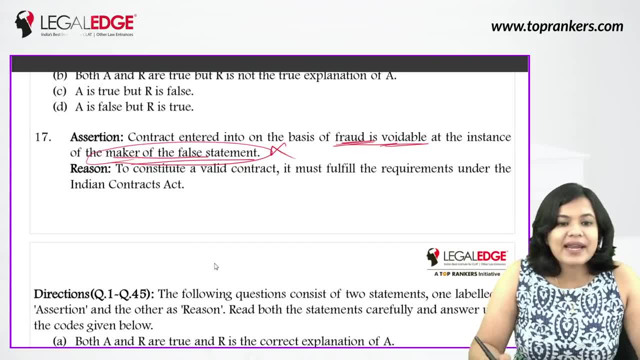 Is this right? No, This statement is wrong. Now, if A itself is wrong, then the answer is easy. But okay, let's see the other statement too. It says: to constitute a valid contract, it must fulfill the requirements under the Indian Contract Act. 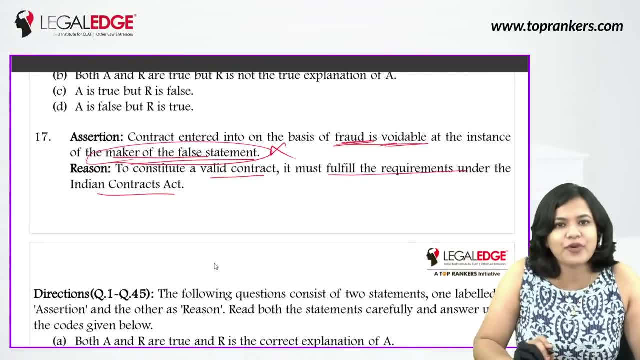 Of course, the things given in the Indian Contract Act. if it is fulfilled, then only the contract will be valid according to the Indian Contract Act. So this is right, This is wrong. So A is false, R is true. 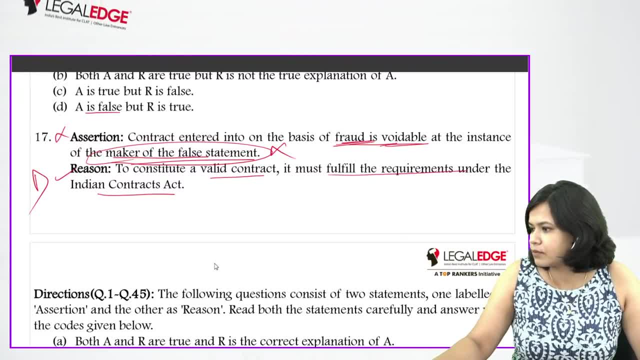 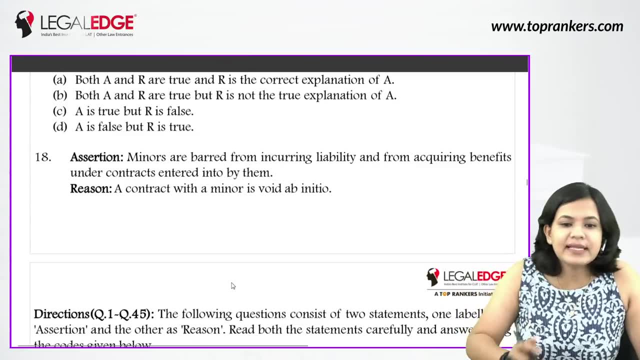 Answer is D. Now 18 says minors are barred from incurring liability And from Acquiring Benefits under the contract entered into them. This is again one of those tricky statements which you need to read carefully: That brother minors are barred from incurring liability. 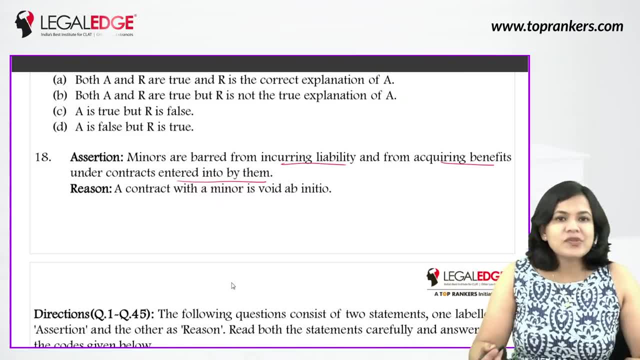 Yes, If you have done any contract with minors and any liability is arising from it, then we say that the contracts that are done with minors are void And that's why there is no responsibility of minors. This part up to here is this right. 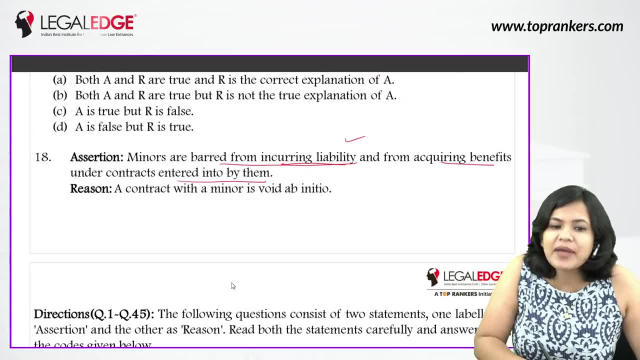 Yes, Further, he is saying, are barred from acquiring benefits under the contract entered into them. This part is wrong. If there is a minor whose parents have made a contract for him, like your parents have paid the fees in your school, they would have entered into a contract with the school that you should educate our child. 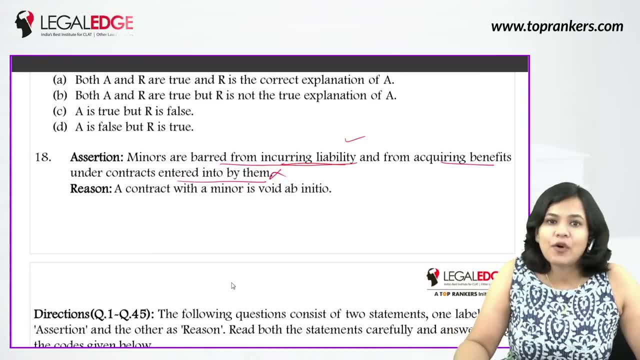 So the benefits of education that you are getting? yes, for that you don't need to make a contract yourself. So the minors can still get the benefit out of a contract. This portion is correct. This portion is wrong. So the first statement is wrong. 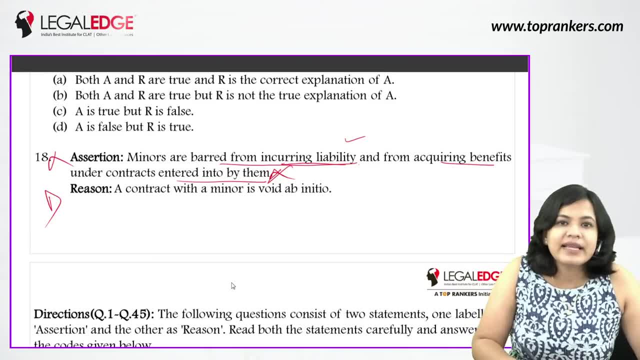 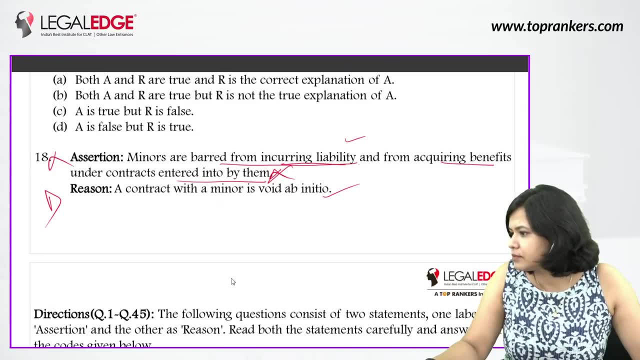 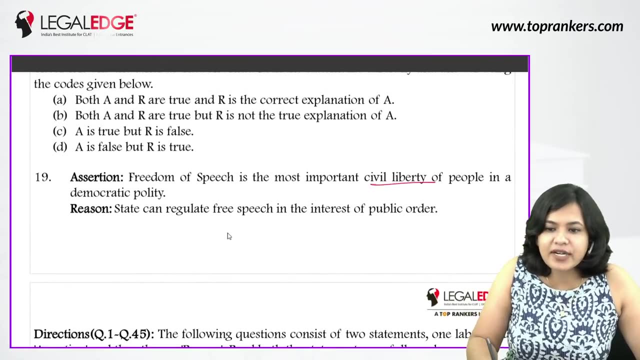 If the first statement is wrong, then the answer will be D. Let's see the reason below. The reason says contract with minors are void of initiative. So this is correct. Next says freedom of speech is the most important civil liberty of people in a democratic quality. 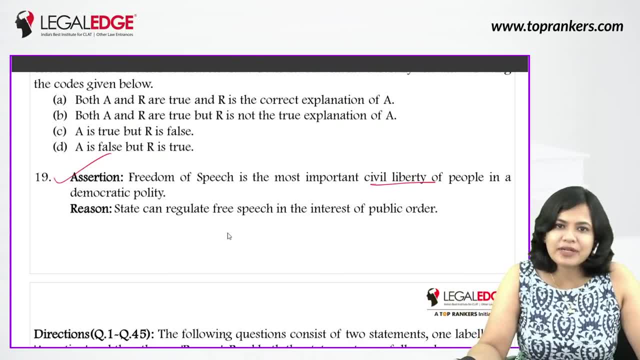 Of course, freedom of speech is the most important thing. That's why democracy is democracy. State can regulate free speech in the interest of public order. This is also correct. that state can regulate. Now, this question is also such that you might have read it and thought that these two are different. 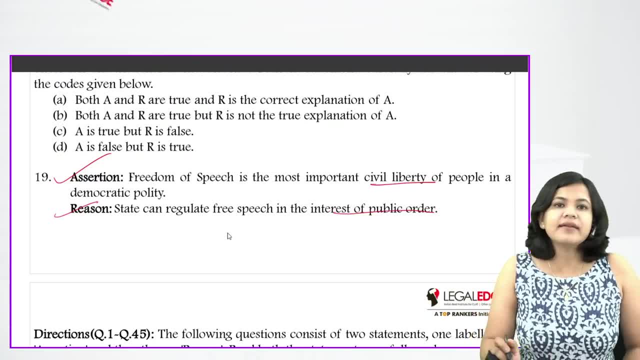 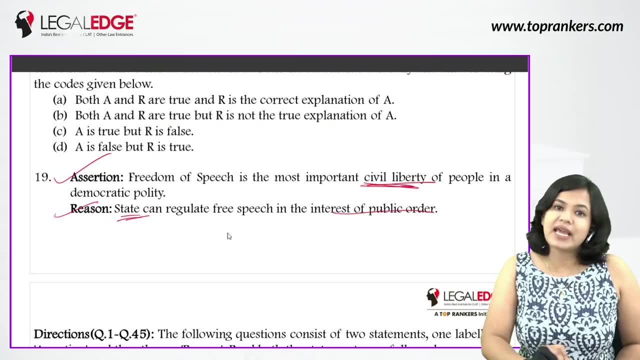 But if you actually think about it, you will understand the relation between the two given statement here. State is regulating. that's why it is civil liberty. It is such a liberty that state is regulating, And state is regulating that's why it is given to us as a liberty. 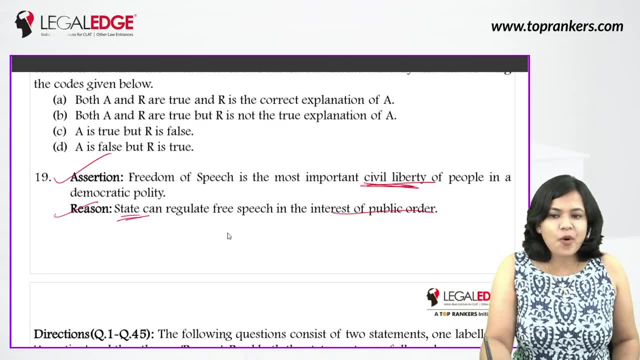 So if I read this, that freedom of speech is the most important civil liberty of a people in a democratic quality, Because state can regulate it. State can regulate it in the interest of the public order. State can regulate it for the people only. 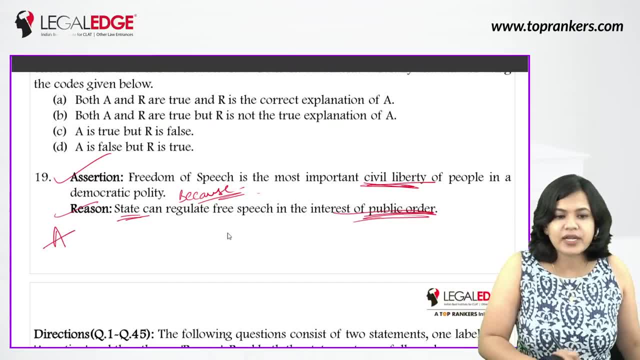 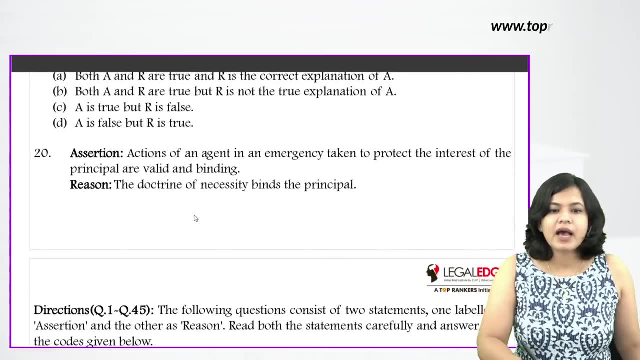 So is this correct? Yes, So answer is option A. Coming to 20th, Actions of an agent in an emergency taken to protect the interest of the principals are valid and binding. Yes, This is not talking about any random agent. in general, 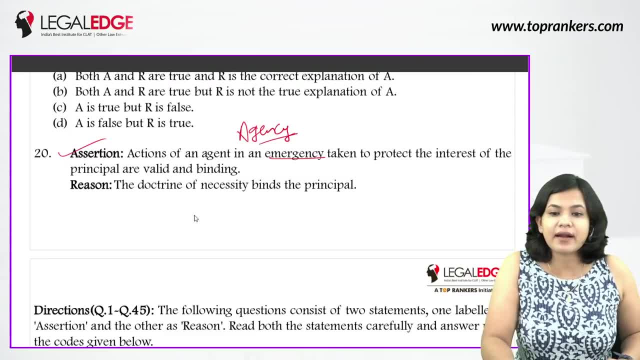 This is talking about the agent who signed the contract of agency. I'm going to give some examples. In my farmhouse there are many prototypes of mangoes And the mangoes you'll find in the market of the refrigerator. I was sending the mangoes from Bhopal to the market of Delhi. 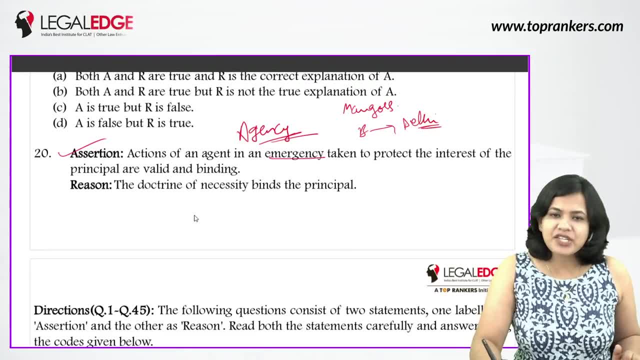 This thing. I used to sell them in the market of Delhi. I hired a truck driver to sell these mangoes to the market of Delhi. This truck driver's name was Aman. Aman wasais a truck driver When Aman was walking in the truck receiving the mangoes from Bhopal. 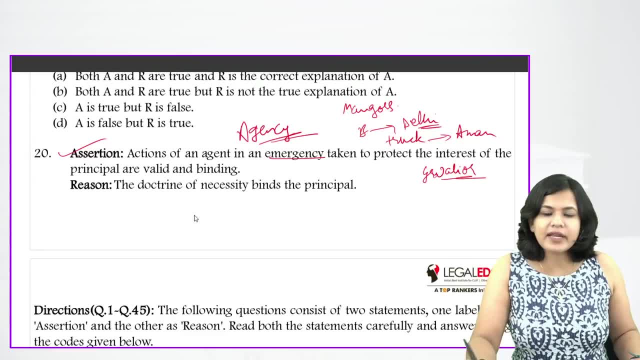 Near Gwaluru, somewhere near Gwalior, there is a strike or landsliding or something like that, due to which the roads are closed and you can't go ahead now. that particular moment he understood that this is an emergency situation and mangoes being perishable goods. 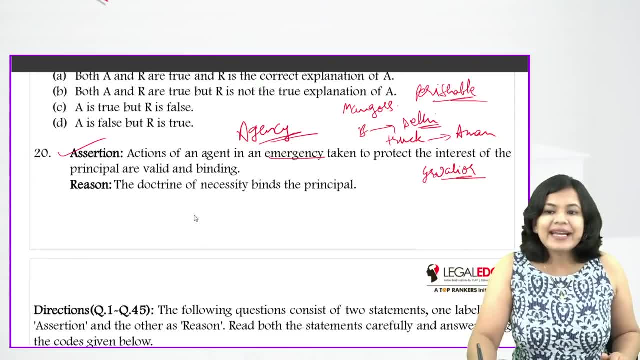 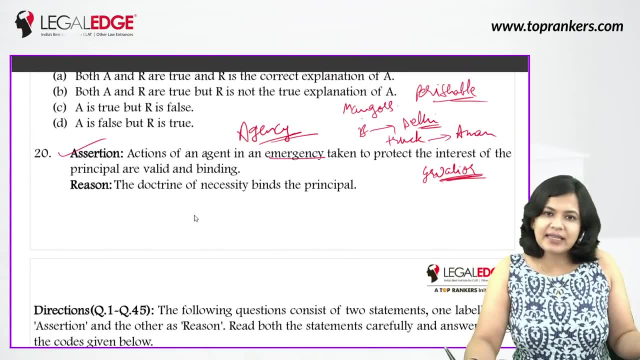 goods which will rot. he decided to sell the entire contingent of mangoes in the Gwalior itself, thinking that if I wait till I reach Delhi, mangoes will rot and it will be completely lost. so it is better to sell it at the same price, which is being sold in Gwalior. 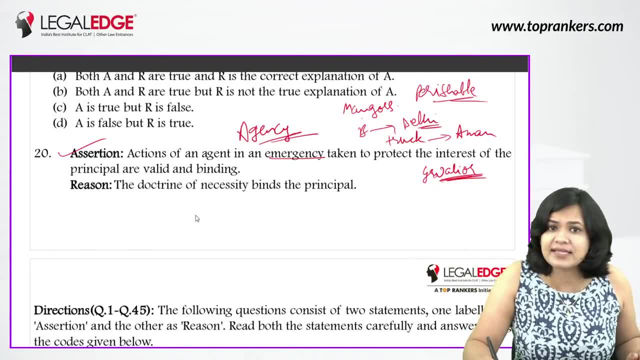 did he take some action in case of emergency? yes, and while he took an action in case of emergency without telling the master, without telling me, was he working on my behalf to protect my interest? yes, so he is saying that actions of an agent in an emergency taken to protect the interest of the principal are valid in binding. 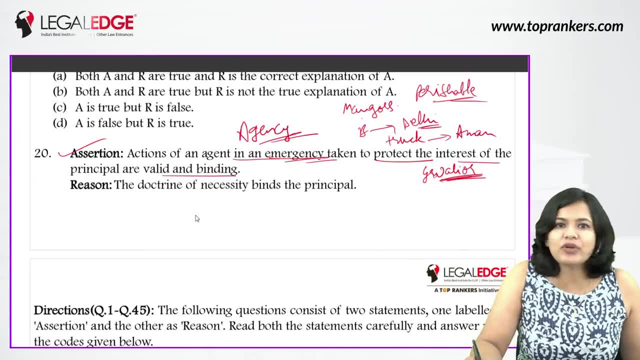 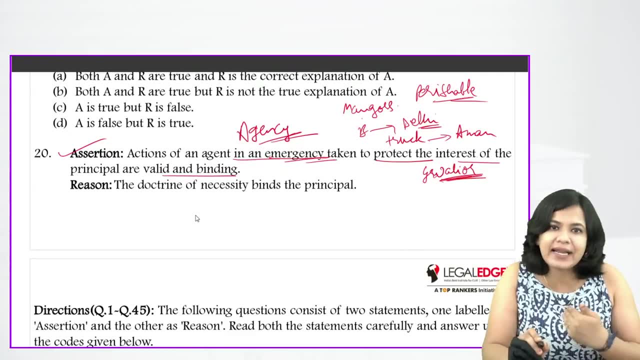 is this valid or binding? yes, so now if I say that, how did you sell it? this is not right. I cannot do that. that particular act which he did is binding on me. he is saying that the doctrine of necessity binds the principal. and why is this binding on me? 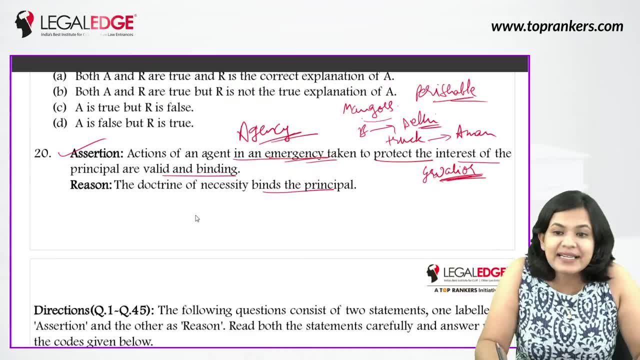 because here doctrine of necessity is applied. it was a necessity to get rid of the mangoes before they actually get destroyed or get rotten. so was it a necessity at that moment? yes, so both the statements are true, and if I put because in C, is it making any sense or not? 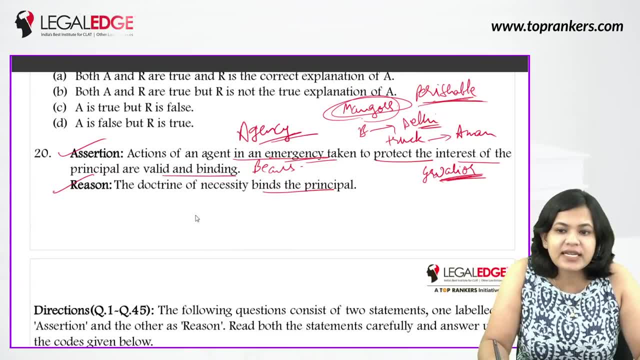 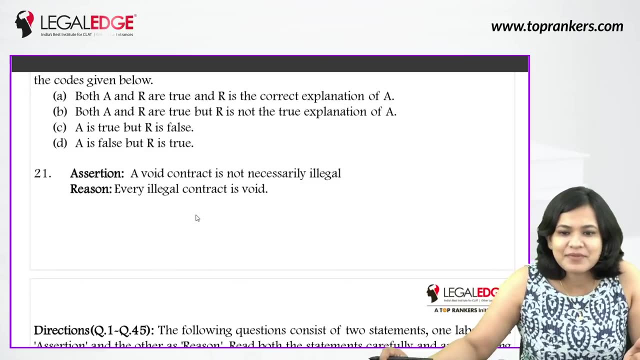 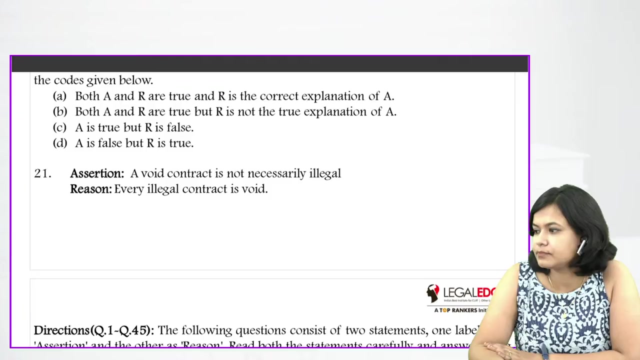 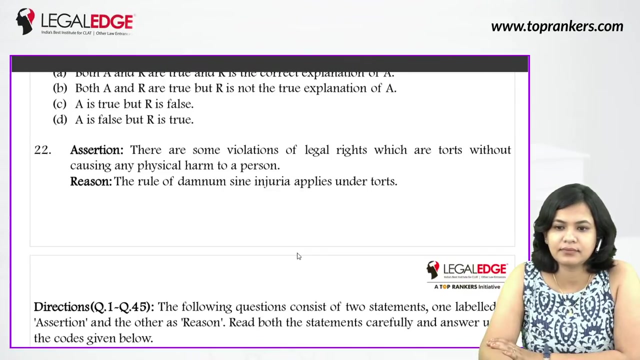 so actions or binding of an agent in an emergency taken to protect the interest of the principal are valid in binding, because doctrine of necessity binds the principal. yes, so answer would be A solved 21st. oh, just a small question, solved 21st. fast, I'll give you the answer. 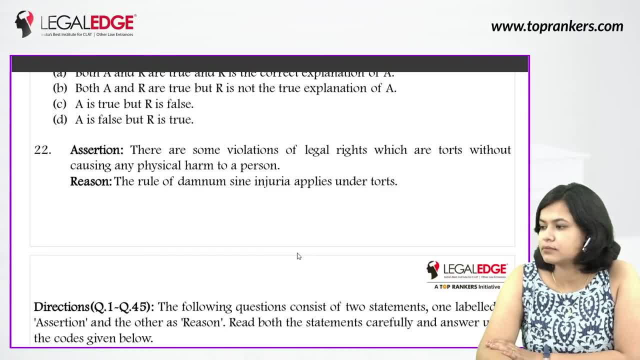 my question is: if the first question was, if the last question was the first question was, shall I delete the first question or the last question or the last question? what does that mean? does it mean that the first question was: should the principal be you? 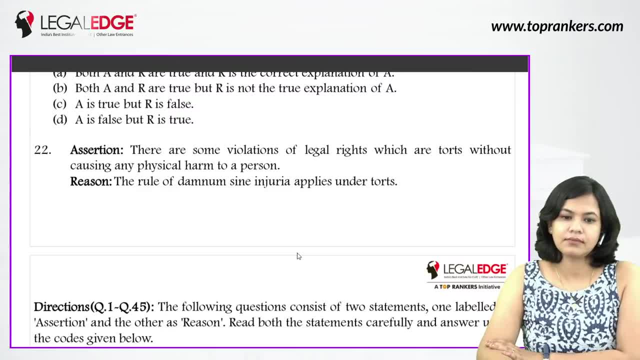 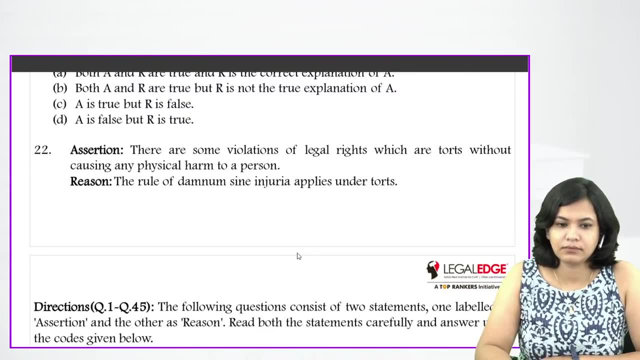 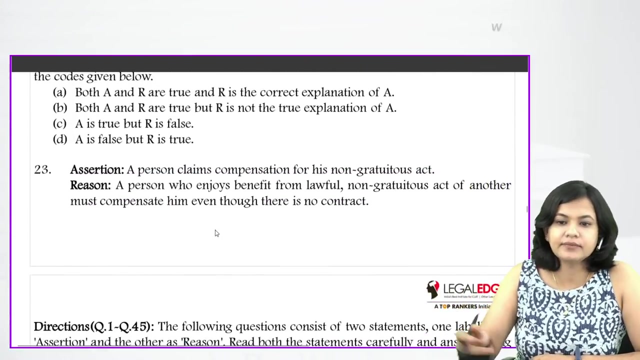 let me make this clear whether or not the principal is you and what how the principal is as well. Okay, 23., 24., 25., 26., 27., 28., 29., 30., 31., 32.. 33., 34., 35., 36., 37., 38., 39., 40., 41., 42., 43., 44., 44., 45., 46., 46., 47.. 48., 49., 50., 51., 52., 53., 54., 55., 56., 57., 58., 59., 60., 61., 62., 63., 62.. 63., 64., 65., 66., 67., 68., 69., 70., 71., 72., 73., 74., 75., 76., 76., 77., 78.. 79., 80., 80., 81., 82., 82., 83., 84., 84., 85., 86., 87., 86., 87., 88., 98., 89.. 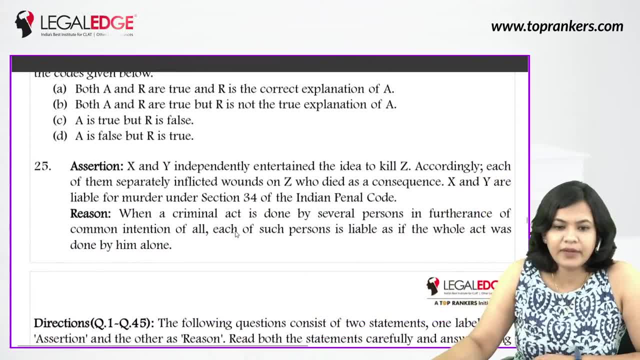 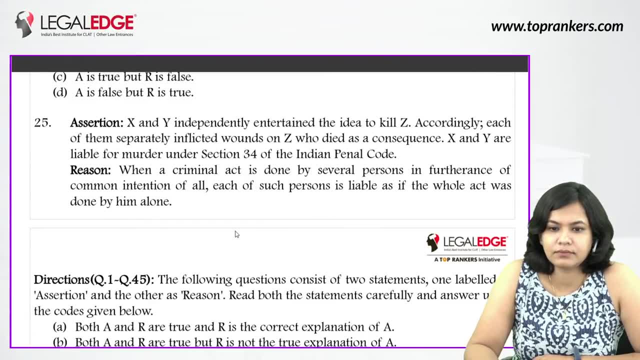 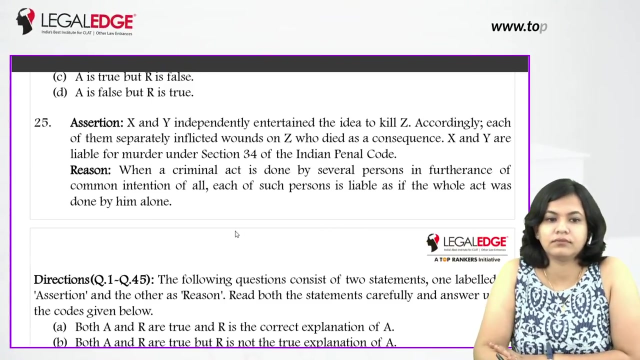 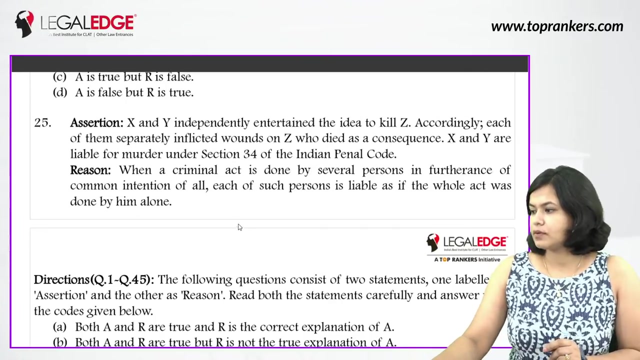 90., 90., 91., 93., 94., 94., 95., 96., 97., 98., 99., 100., 100., 100., 100.. you and 25th. okay, so moving back to 21st question. 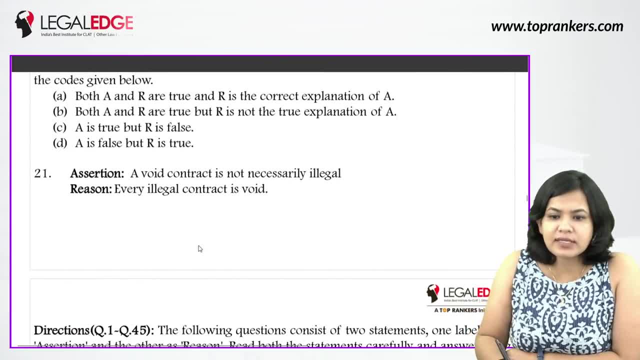 a void contract is not necessarily illegal. of course, illegal contracts are those contracts in which there is some kind of offense or some kind of work that our penal laws do not allow. but apart from this contract is not allowed, there can be some kind of contract that you have done with some unsound mind person. 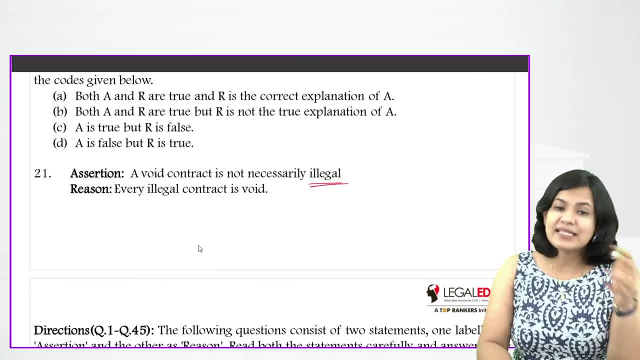 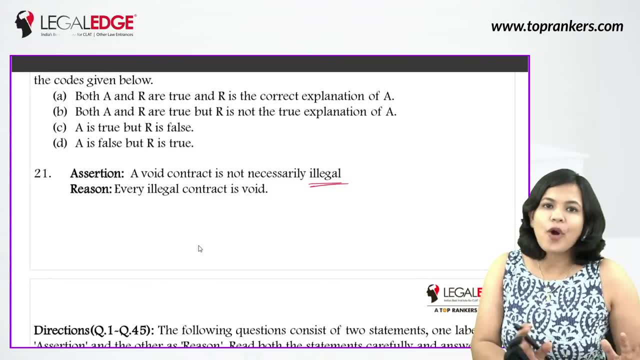 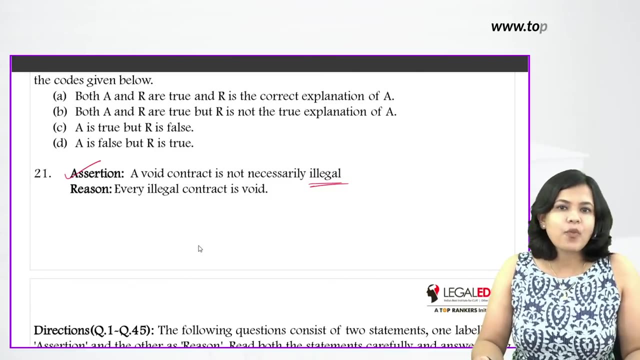 or some contract that you have done with some bankrupt person, or contract that you have done with some minor. these things are not illegal, but are they void? yes, so every time a void contract is illegal, it is not necessary, which is true, every illegal contract is void. 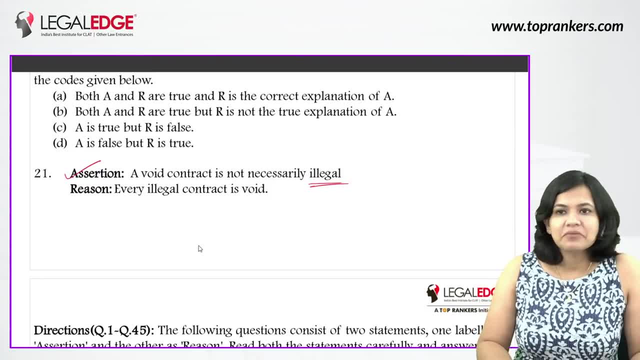 yes, whenever there is an illegal contract- someone was given a bribe that take 2 lakhs and kill someone- this kind of contract is illegal. and are all these illegal contracts are void? yes, but both of them are two different, independent statements, so answer would be B. 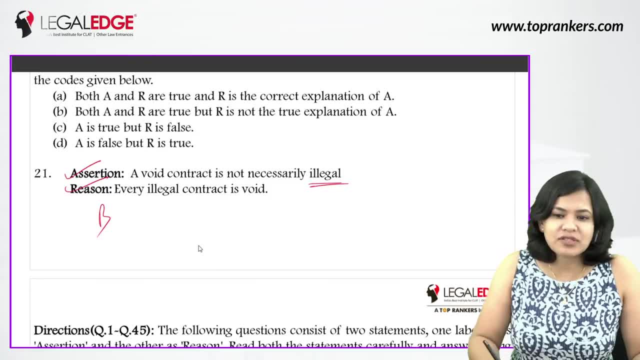 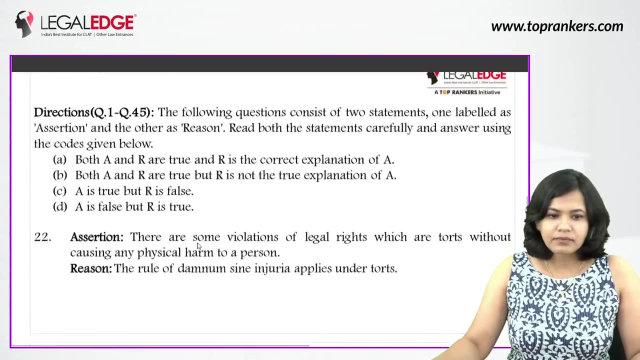 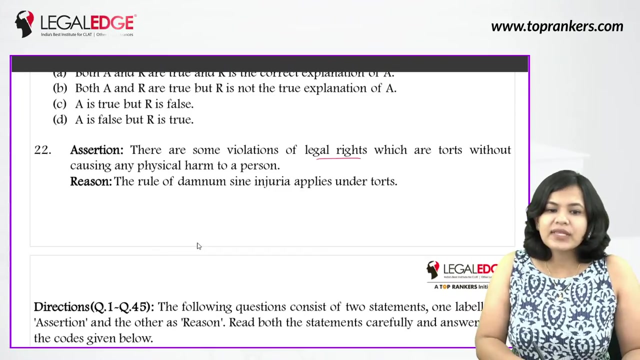 because you can read it yourself. a void contract is not necessarily illegal, because every illegal contract is void. this contradicts itself, or it feels like it is not going with it, and obviously it is not explaining it. its explanation is different. so, 22th, there are: there are some violations of legal rights which are taught without causing physical harm to a person. 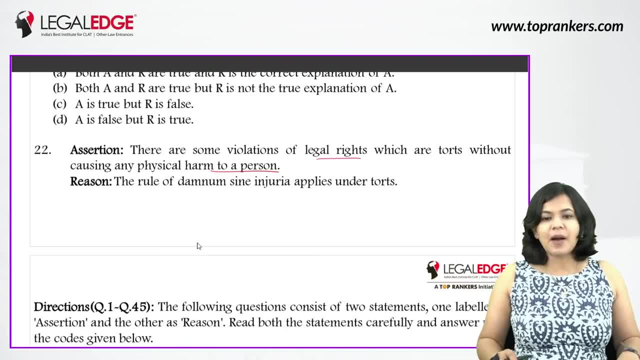 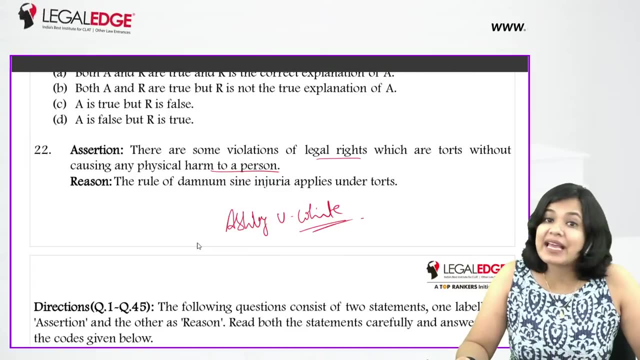 yes, it happens that there are some cases where your legal rights are violated but you did not get any physical harm. and there is a very famous case as well, Ashby vs White, that vote case, that a person goes to vote but he is not allowed to vote. 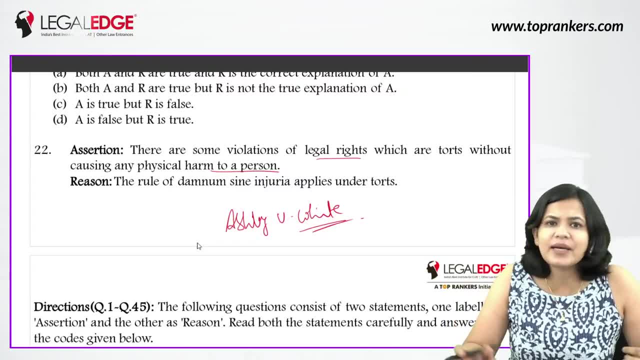 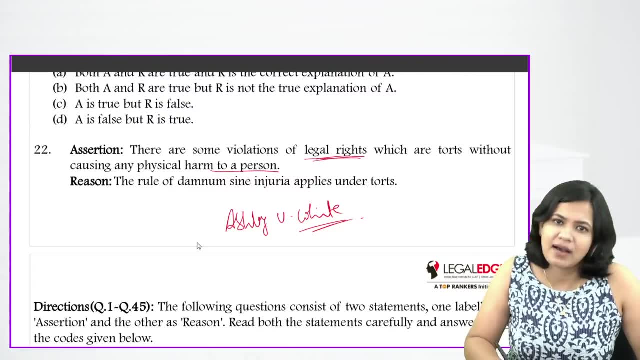 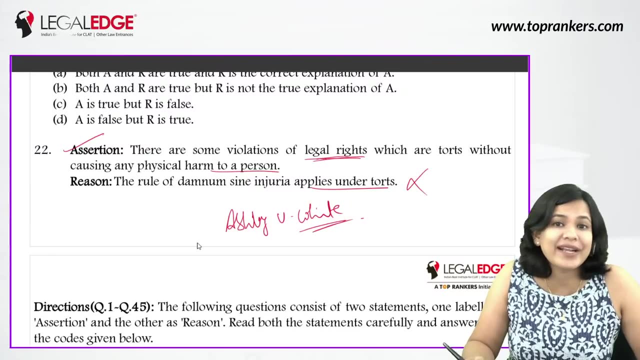 even then, your candidate won, so you did not get any loss. but when you were not allowed to vote, did your legal rights get violated? yes, it happened. reason: the rule of Damnam sine Injuria applies under tort? no, it does not. Damnam sine Injuria means: 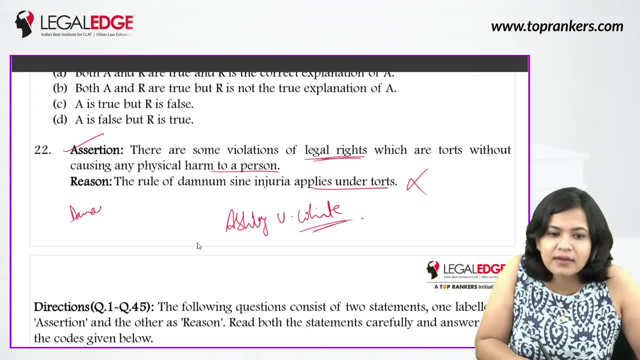 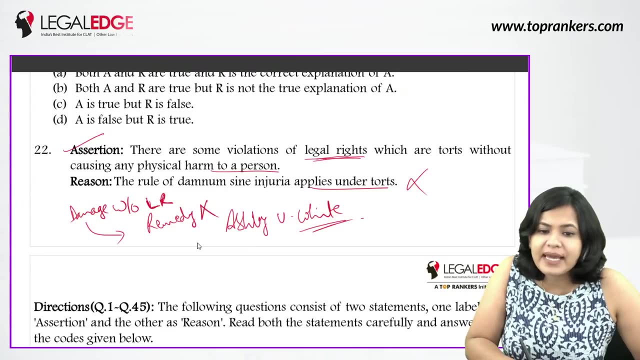 that you have been damaged without violation of legal rights. your legal rights are not violated, but you have been damaged. and when your legal rights are not valid and you want to apply this rule and you want to ask for remedy, so will you get any remedy? no, there is no remedy in this. 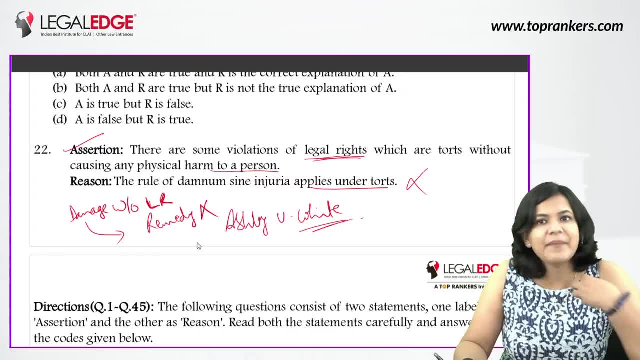 this is Gloucester grammar school case that I had my own school in the city. all the children of the world used to study in my school and then a competitor came. he opened his school and gave better services from my side. the children withdrew and took admission in the school of the other person. 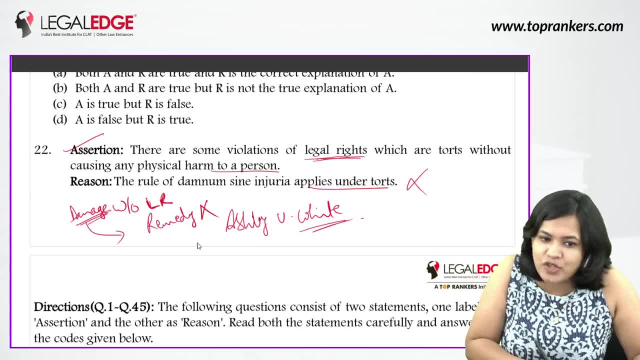 I had financial loss. I was damaged, but did my legal rights get violated? my legal right to profession or to run my own business? did it get violated? no, this did not get violated. so if I ask for remedy in the court, that please apply this rule and give me remedy. 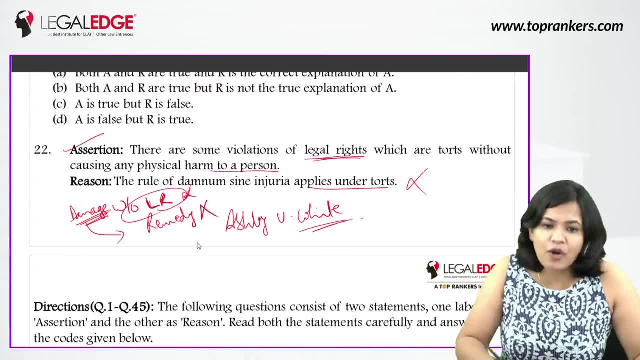 provide me some remedy for the loss? will the court give no? so if you say that Damnam sine Injuria applies under tort, no Injuria sine Damnam applies in tort. Damnam sine Injuria does not apply in tort. and because this statement is wrong, 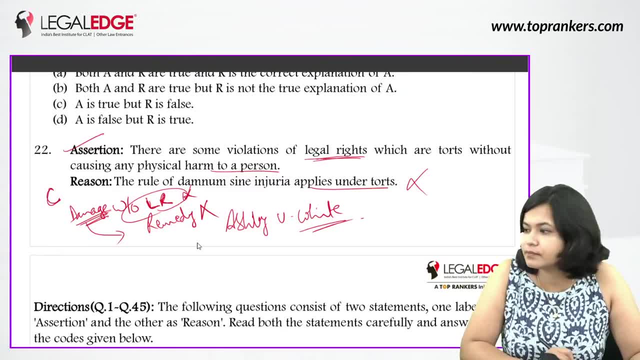 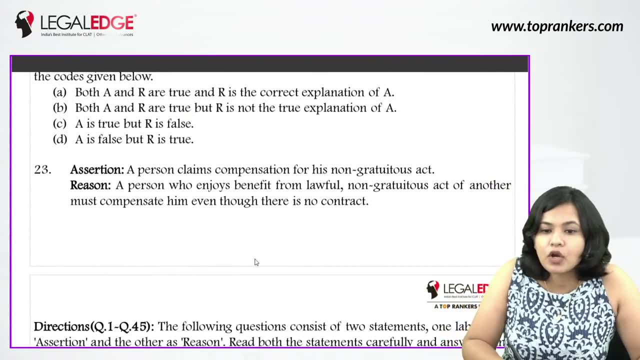 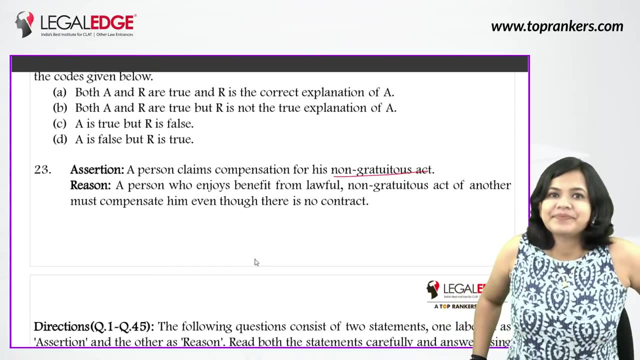 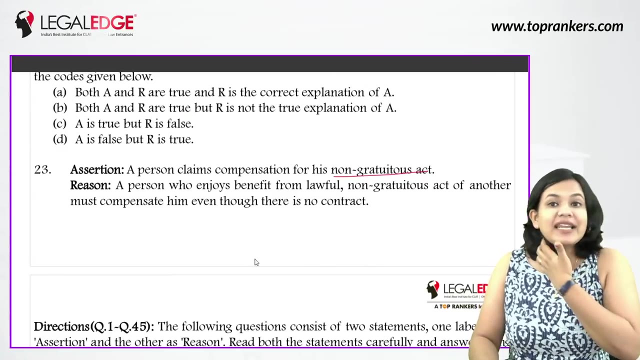 the answer would be C 23. a person claims compensation for his non-gratitude. a person claims compensation for his non-gratitude. any such work which I have done on humanitarian grounds or by thinking that I have to do it on a generous grounds, I have not done it by thinking that. 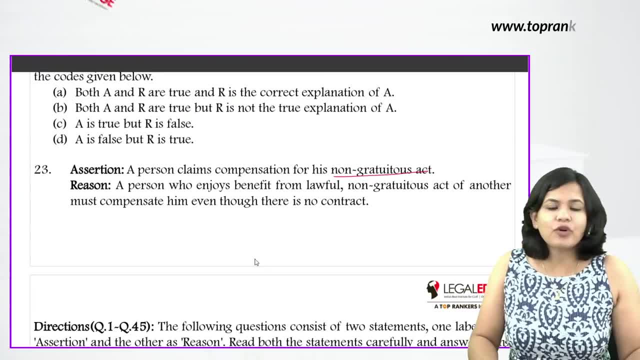 I have not done it by thinking that it is non-gratitude to us, so can I? I can claim compensation whatever extra work I have done for you. can I ask money for that? yes, a person who enjoys benefit from lawful non-gratitude act of another. 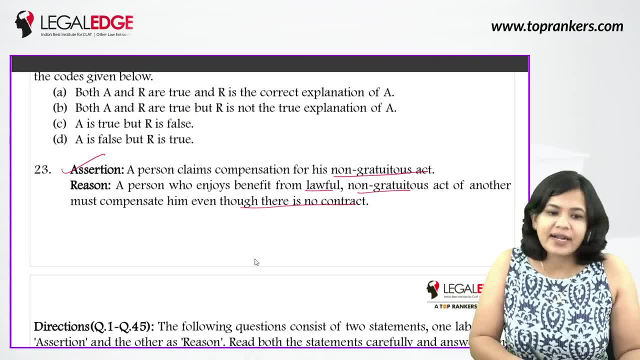 must compensate him even though there is no contract. yes, is he talking about quasi-contracts? yes, these are quasi-contracts, such contracts which you did not properly talk to the other person on terms and conditions, but here some person has done something like this for you. 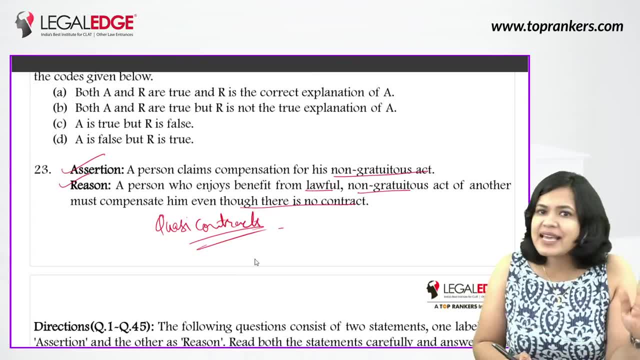 by which you are getting benefit, and he was not doing this work generously for you. he was doing this work with the thought that you will give him that money. suppose I want RD Sharma. I am preparing for some exam. I need RD Sharma and I do not have RD Sharma. 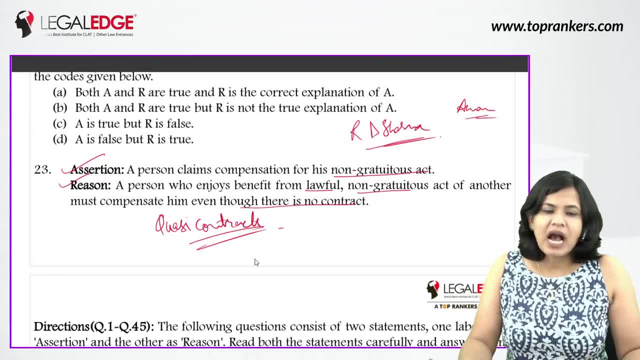 so I told someone- let's say there is a student named Aman in my class. I told Aman: if you will get RD Sharma, then tell me now. he checked at the shop near his house. he had two available, so he thought let's take one for Sakshi ma'am. 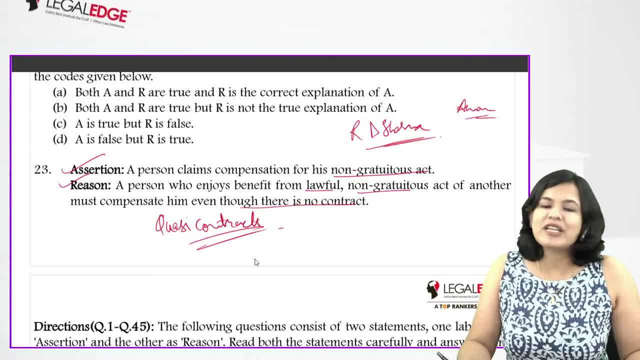 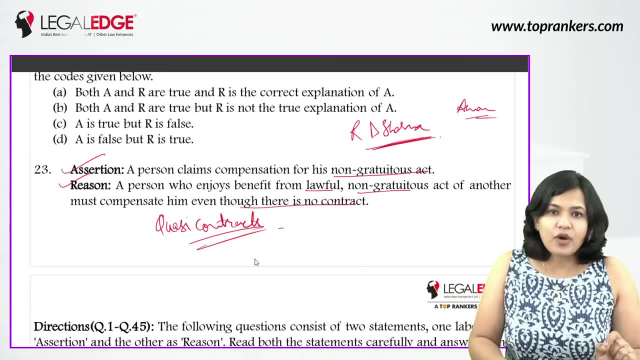 when he took it. then he gave me a gift. he was not taking it as a gift. he was expecting that ma'am will give him money. so when he will give me this book, am I bound to pay him? yes, I am bound to pay him. so if you read this with because 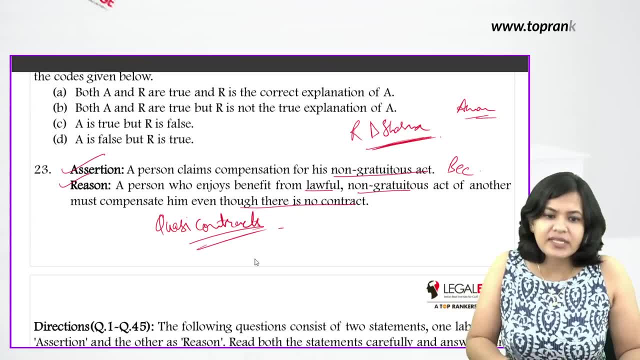 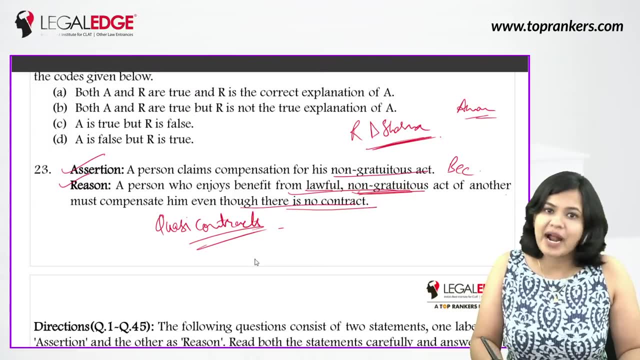 try it. a person claims compensation for his non-gratuitous act because a person who enjoys the benefit from lawful non-gratuitous act of another must compensate him even though there is no contract. yes, the answer would be: Arnav R is wrong, because it does not apply under torts. 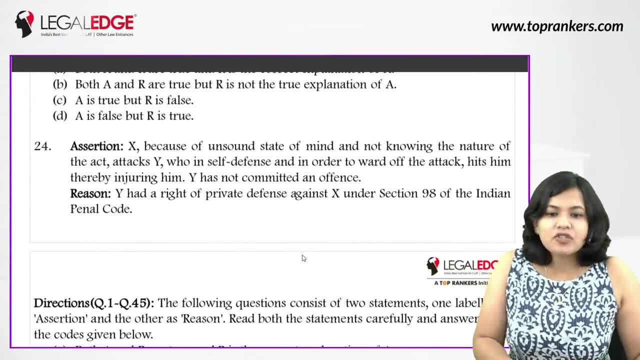 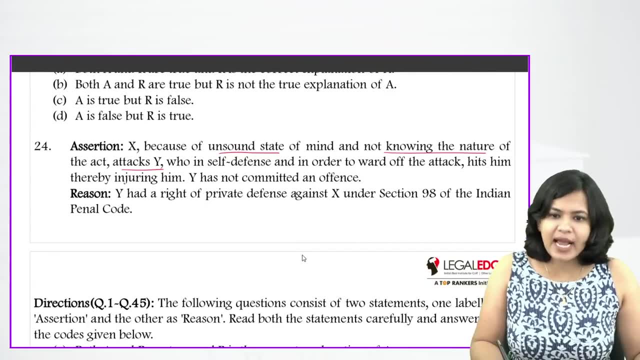 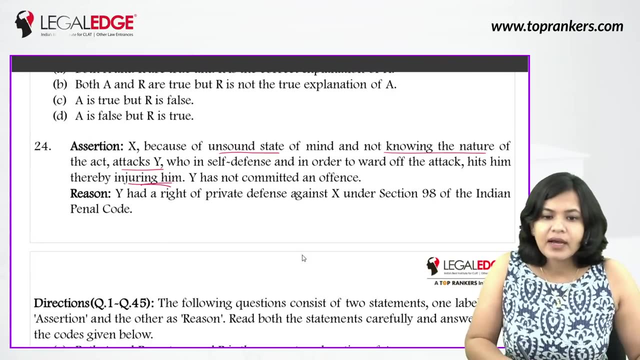 24 X because of unsound state of mind and not knowing the nature of the act, attacks Y? X is an unsound mind. he attacks Y Y counter attacks his self-defense and hits him, thereby injuring him. he injures X? Y has not committed any offense. 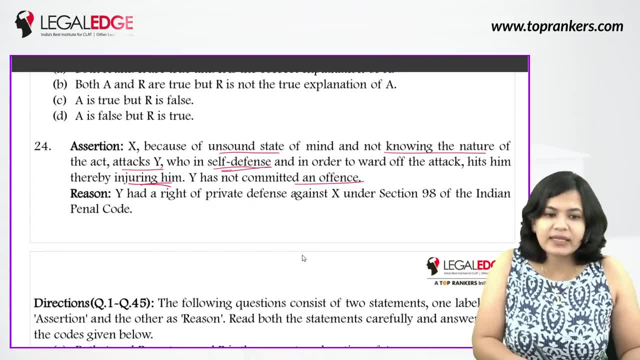 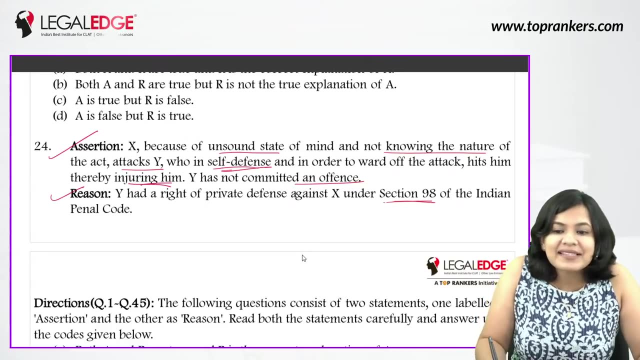 obviously Y was enjoying his self-defense so he did not do anything wrong. is this right? yes, Y had a right to private defense against X under section 98 of the Indian Penal Code. does he have a private defense in section 98?? yes, and does he have a defense in section 98? 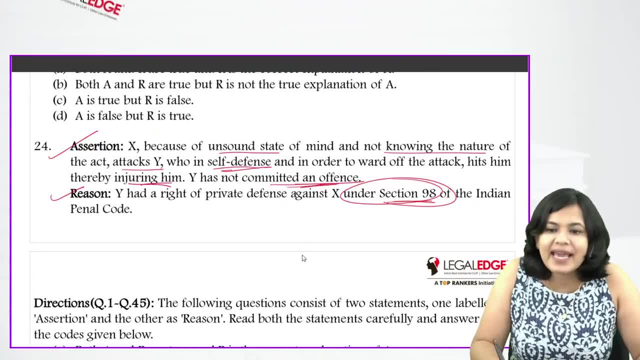 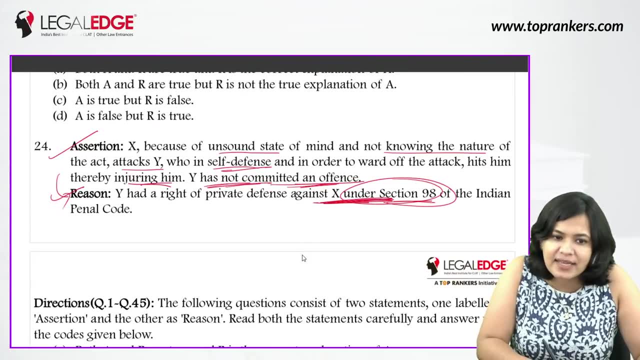 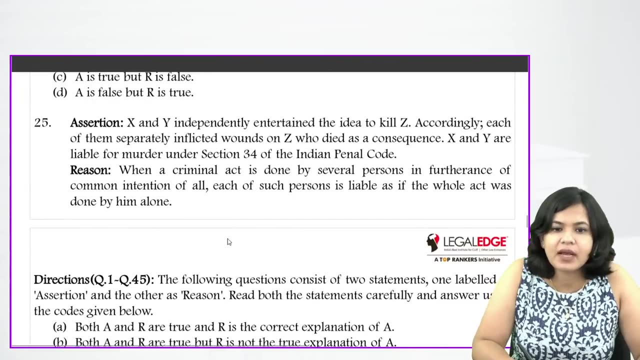 that is why we are not considering him as an offense. yes, the defense given in this section is the reason why we are not punishing Y and because this is his reason, the answer would be A yes, 25 X and Y independently entertained an idea to kill Z. 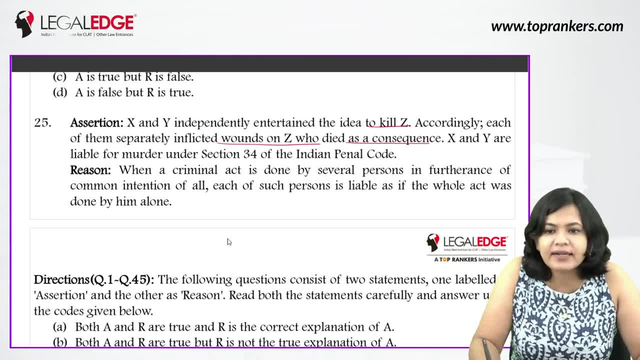 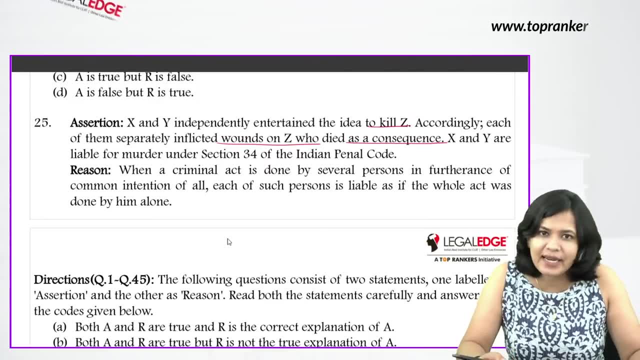 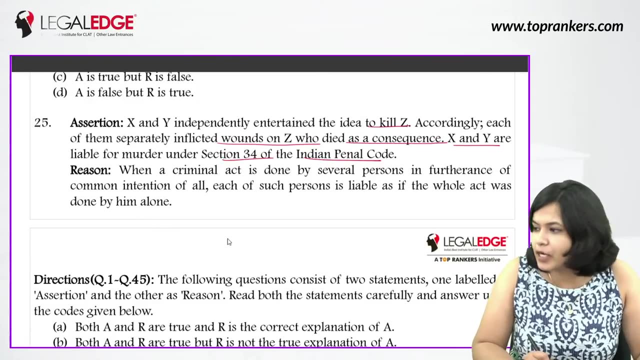 according to each of them separately infected wounds on Z, and Z died of consequences. X and Y did this work, thinking differently, but there independently. they inflicted this wound and because of that he died. X and Y are liable for murder under section 34 of Indian Penal Code. 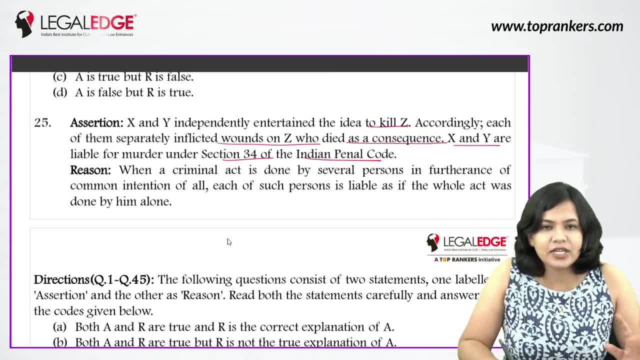 now in section 34, we talk about common intention. section 34 is about common intention. so will they be liable for common intention? yes, they will be liable for common intention when a criminal act is done by several persons in furtherance of common intention of all. 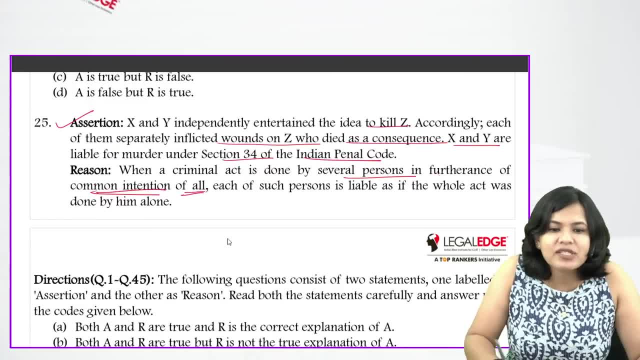 everyone has the same intention. are all persons liable for that act? each of such persons is liable as if the act was done by him alone. is this right? yes, the answer would be A. now I would not recommend or I would not tell you to go ahead and learn all the sections. 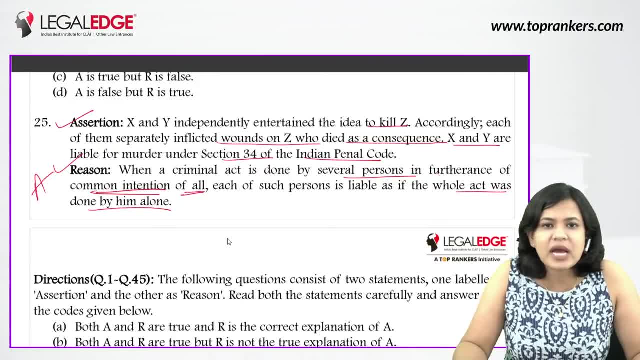 but in the past they have given few questions where they have asked some sections in assertion reason. so okay, now, two days before, after getting so tensed, learning all the sections and doing any such act can be harmful in itself. it would be dangerous, so do not worry. 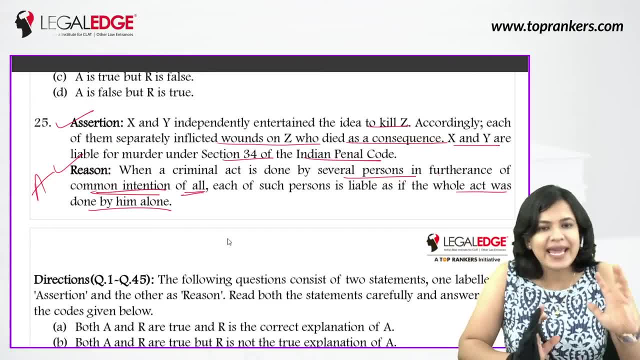 when it will come. think about it, there will be one or two such questions in general that do not do any such act, which is totally new for you, because two days before the exam, starting anything new always and always backfires. so do not do that. I am explaining you questions here. 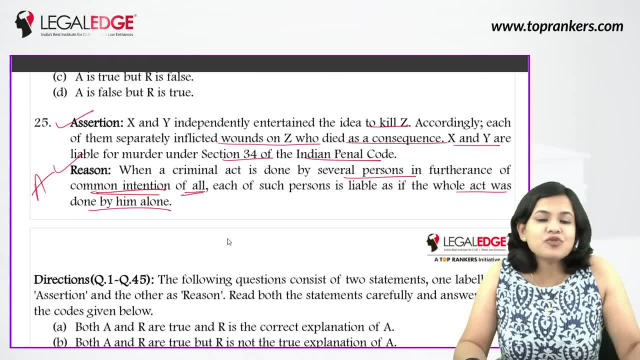 for the obvious reason that if you ever see any section, do not think that this is totally out of the blue. no, there have been times when they have asked sections somewhere, but especially not in 2-3-4 years. so that is why there are just one or two questions. 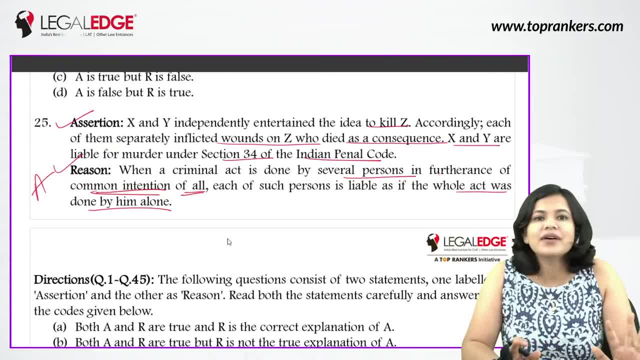 which has sections. here is, just to you know, make you comfortable, if at all there appears any section in your exam, but in general you don't have to worry about that. there would be plenty of other questions which will not talk about sections and you can easily go ahead and solve them. 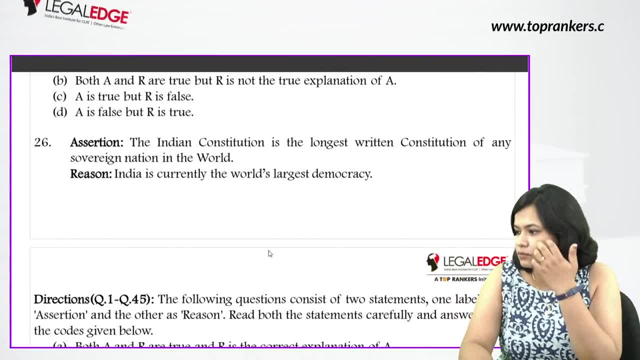 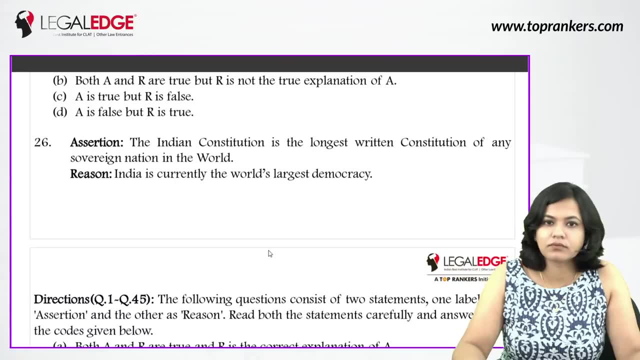 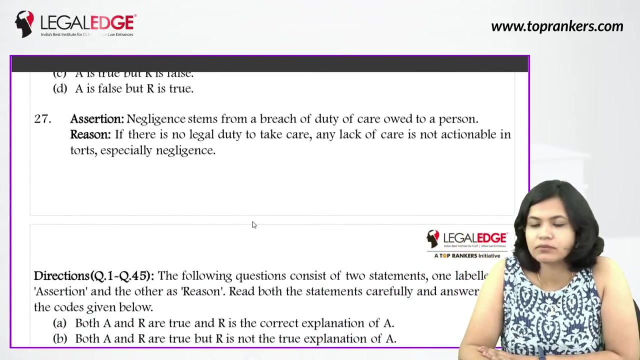 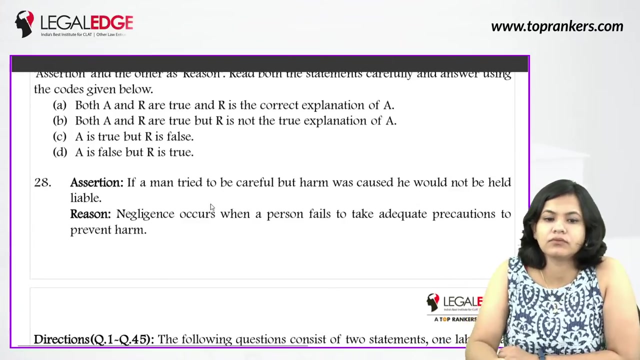 come on, solve 26th. 26th starts now. 26th: 26: 26 answers, 26 answers, 26 answers executive: Come to 26th. come to 27th. Thank you 28th, 29th, 30th. 31st, 32nd, 33rd, 34th, 35th, 36th, 37th, 38th, 39th, 40th, 40th, 40th 40th. 44th, 46th, 47th, 48th, 49th, 50th, 51st, 51st, 52nd, 52nd, 53rd, 52nd, 57th. 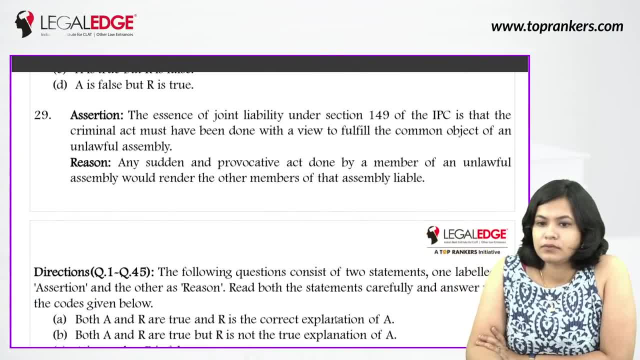 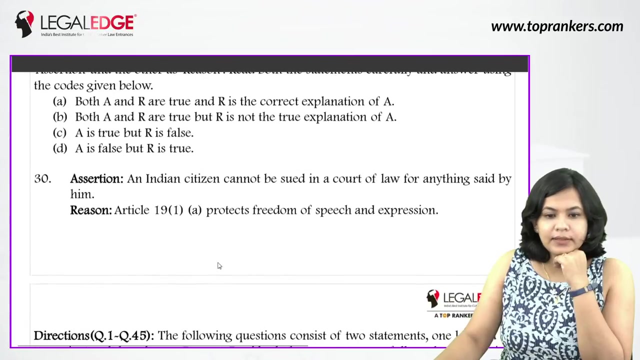 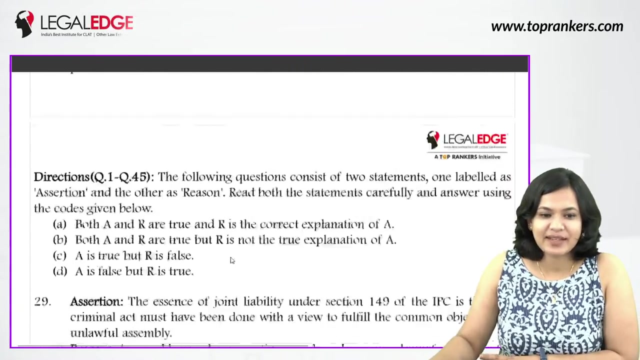 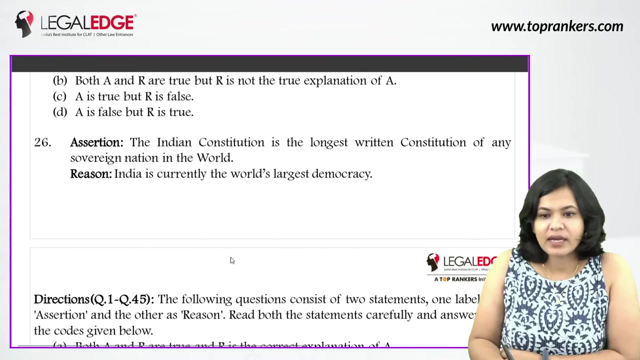 56th, 56th, you and i'm done. okay, so 38, it's easy again. so 38, so, so, so, so, so you, you have to read it carefully, okay. so, going back to question 26, the Indian constitution is the longest written constitution of any sovereign nation in the world. 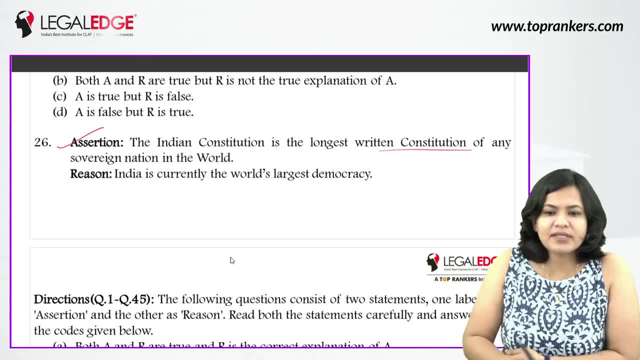 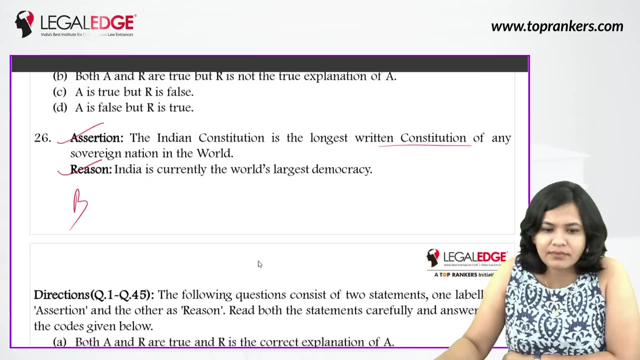 yes, it is correct, India is currently world's largest democracy. this is also correct, but constitution being very lengthy and long and India being the largest democracy: are these two different things? yes, and because these are two different things, the answer would be B, very simple: negligence stems from a breach of duty of care. 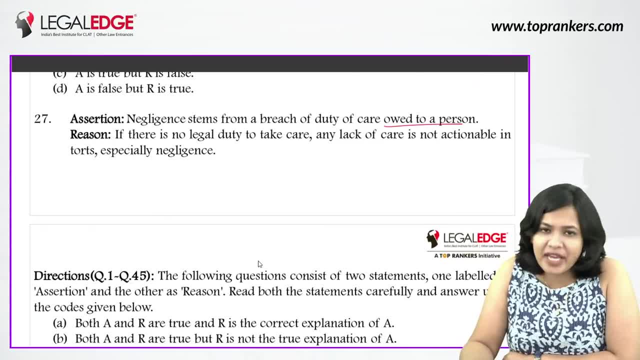 owed to a person when my duty of care will be made for someone and if I breach that duty, then only there will be negligence. this is correct if there is no legal duty to take care and any lack of care is not actionable, in taught especially negligence. is this also correct? yes, 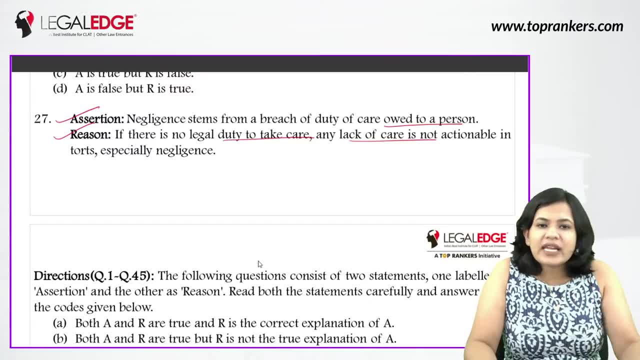 when my duty was not made. I had no connection with that person, I had no responsibility. then I can't be liable for that. now put because- and try reading it so negligence stems from a breach of duty of care owed to a person. because if there is no legal duty to take care, 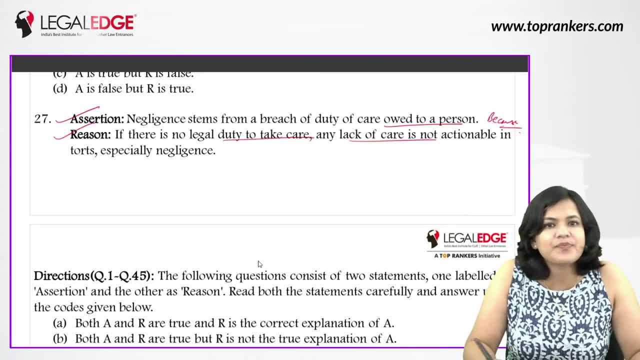 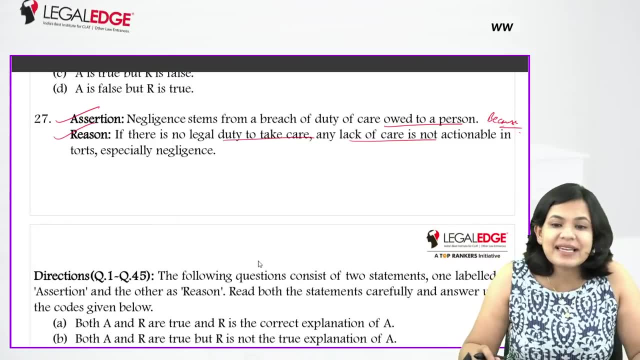 any lack of care is not actionable in taught, especially negligence, of course. if there is no duty of care, then how will there be breach, and if there is no breach, then how will there be negligence? is it necessary to have breach of duty of care for negligence? 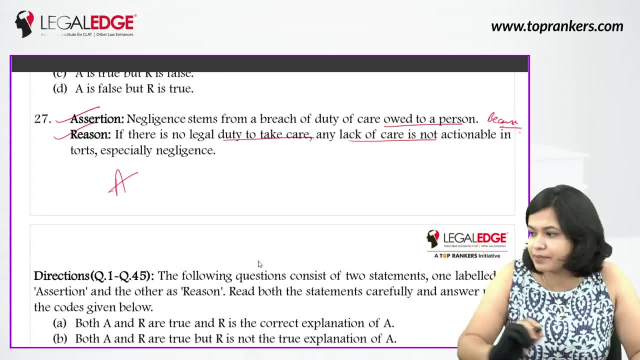 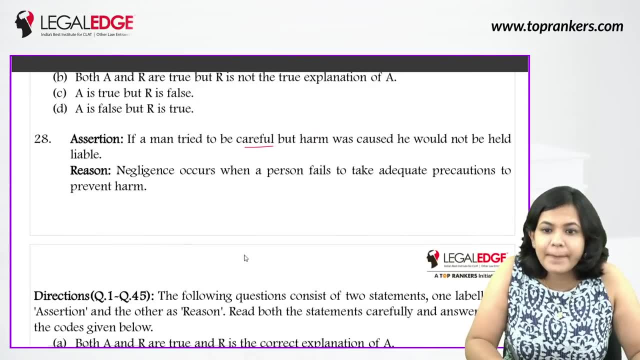 yes, the answer would be yes. the answer would be yes, coming to 28th. coming to 28th: if a man tried to be careful but harm was caused, he would not be held liable means I had taken care of him, but if something goes wrong then I am not liable. 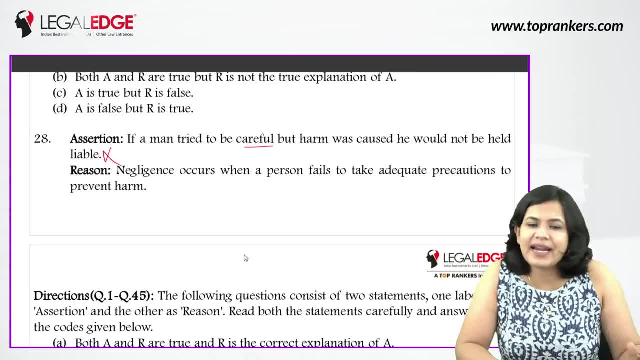 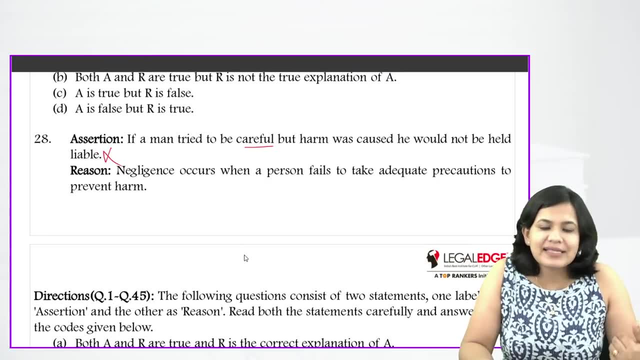 this is not correct. you will feel that it is correct. but being careful is not enough. your duty of care in general is important. let's say I live on 4th floor. I live on a 4th floor. I have kept pots on the edge of my balcony. 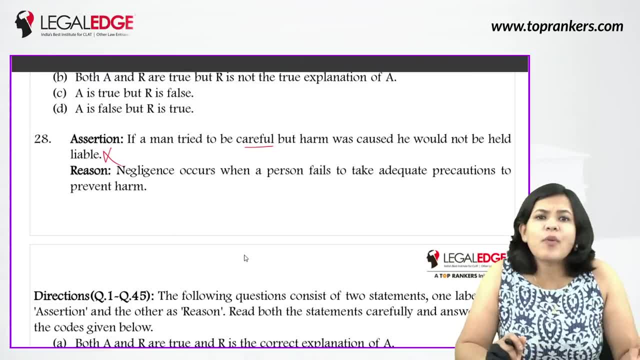 I have kept big pots. I had kept pots very carefully. I was very careful in placing the pots on the edge of the balcony. the point was when you kept it on the edge of the balcony. did you make a mistake then? yes, because if you have kept it on the edge of the balcony, 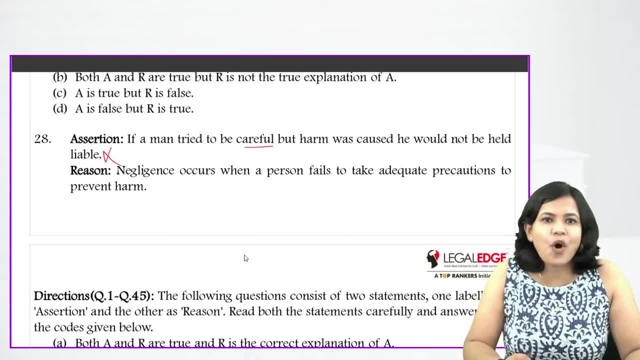 no matter how carefully you have kept it. what if there is a strong wind or a strong storm and it falls and someone was standing downstairs? I was careful, but what I did? was it wrong in itself? Yes, so my being careful is not enough. 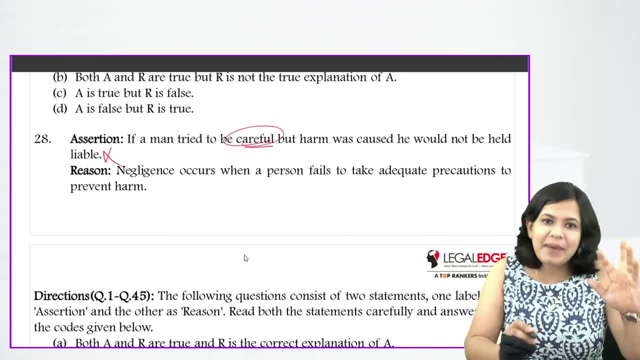 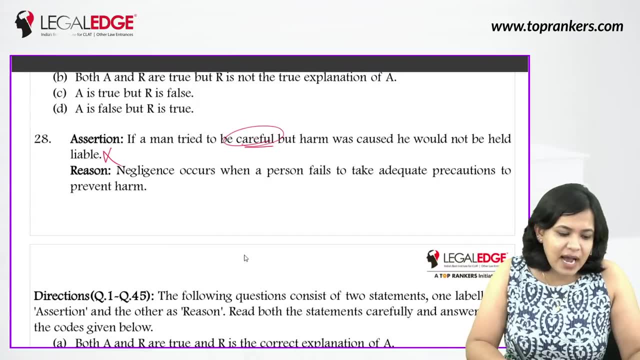 It is necessary to fulfill my duty of care. If I am careful and if I have not fulfilled my duty of care, then I will be liable. Negligence occurs Now. if this statement is wrong, then the answer is D, But let's see the reason. 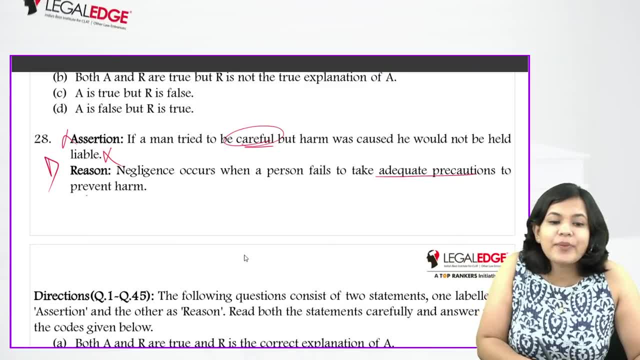 Negligence occurs when a person fails to take adequate precautions to prevent harm. Yes, my being careful is not enough. I have to make sure that I fulfill my duty, And when I fulfill my duty do I have to take adequate precautions. 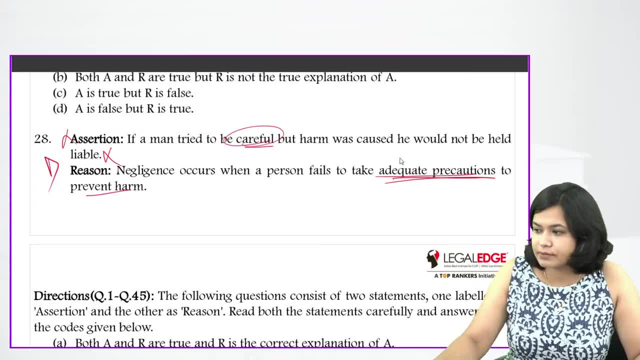 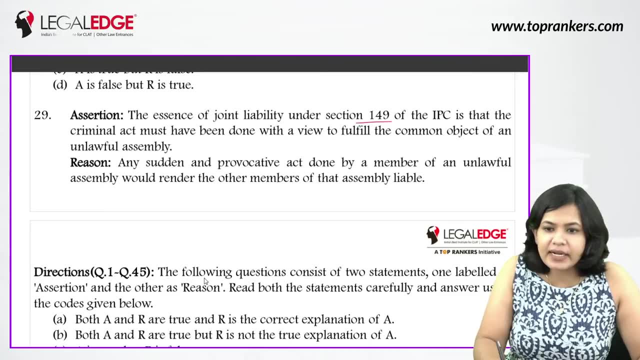 Yes, I have to take adequate precautions. 29th, The essence of joint liability under section 149 of IPC is that the criminal act must have been done with a view to fulfill the common object of an unlawful assembly. Okay, we are talking about an unlawful assembly. 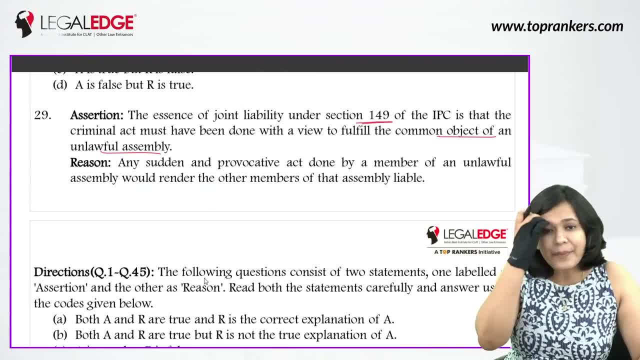 You must have read section 149 in general somewhere in current legal affairs, Or you must have read some article Because unlawful assembly curfew. these things are discussed every day Since the pandemic started. this has been discussed everywhere. So is this statement right? 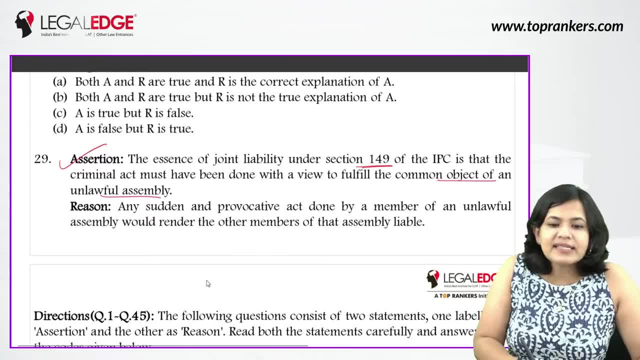 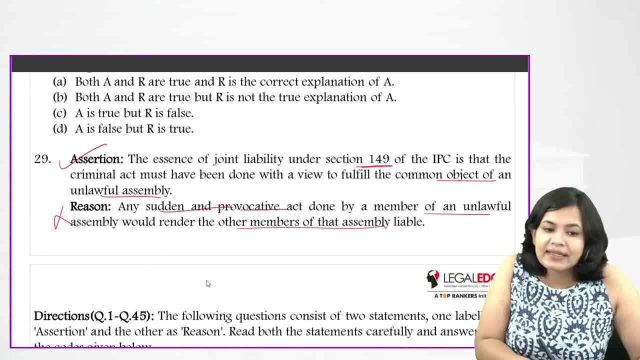 Yes, my being careful. Any sudden and proactive act done by the member of an unlawful assembly would render other members to be liable. This is wrong. There was an assembly of 10 people. One of them started a riot. This does not mean that all 10 people are liable. 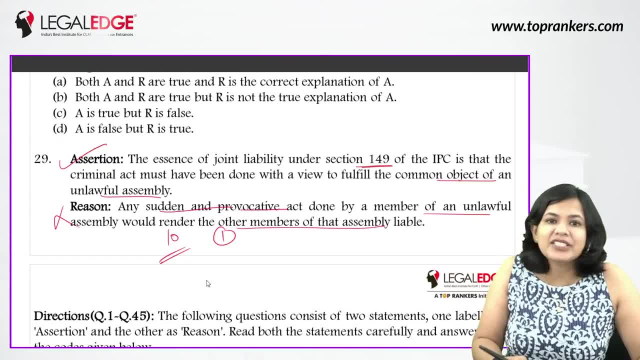 Specifically for an unlawful assembly are more than 5 people, or all the people whom you want to libel. is it important to riot everyone? Is it important to do something wrong to everyone? Yes, If someone does one or two things, it will not be enough. 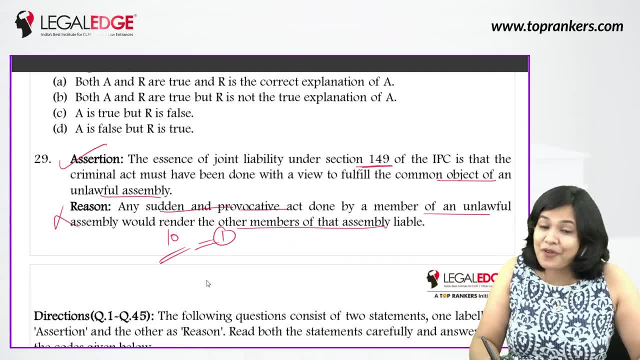 So if he is saying that sudden and proactive done, provocative, done, act done by any member of an unlawful assembly would render other members of the assembly to be liable, No, this is wrong. The person who did it will be liable. Not everyone will be liable. 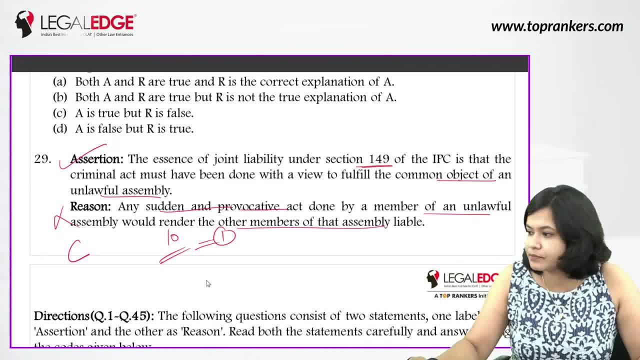 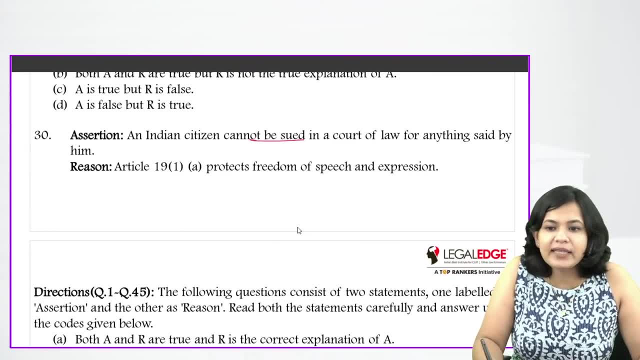 So the answer would be C 30th. An Indian citizen cannot be sued in the court of law for saying anything, for anything said by him. This is absolutely wrong. You will say any answer. All things are not mass. There is a certain restriction over your right. 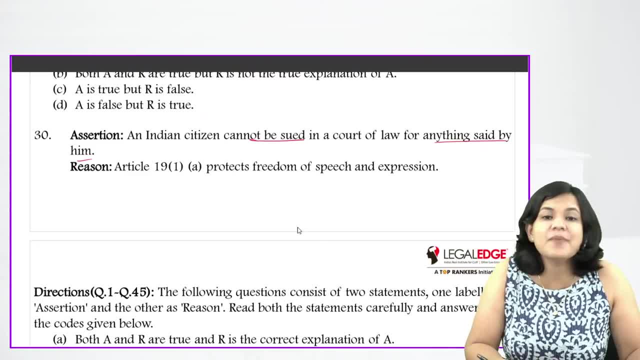 You have a right. You have freedom of speech and expression, but it is something which is subjected to reasonable restriction. So we are saying that you will never have a case. Is this wrong? Yes, this is wrong. You will have a case. 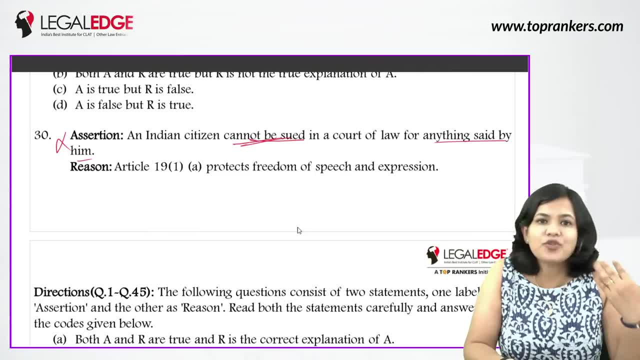 You will do sedition, You will have a case. You will do defamation, You will have a case. If this is wrong, then the answer is D. The reason is that Article 19 protects freedom of speech and expression. Yes, it does protect freedom of speech and expression. 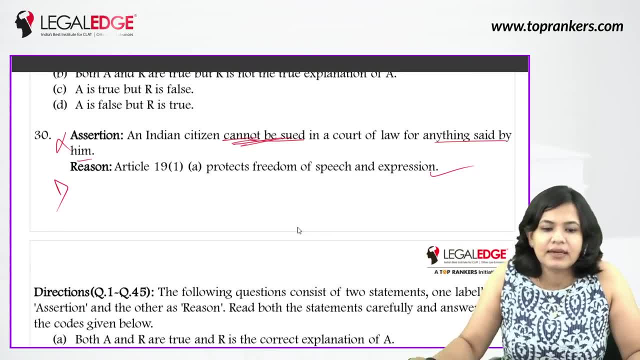 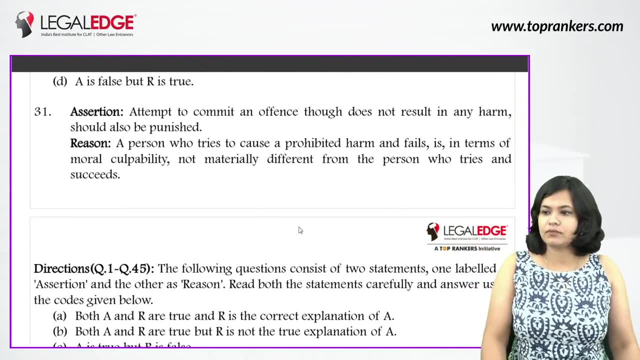 But can you be punished? Come to 31.. Sorry, 31 Fast Solved. 31 Solved 31. You solve them fast Because it has been more than 1 hour of solving the same kind of questions, So it's less time. 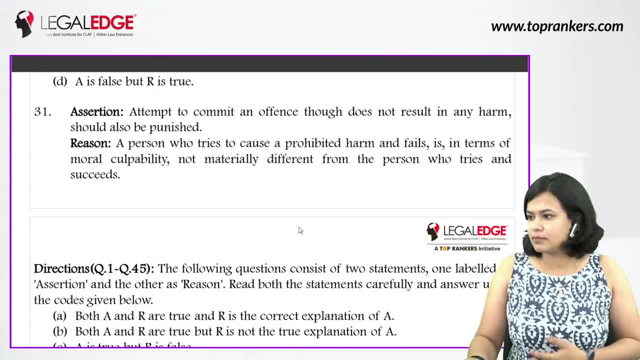 You have to solve it quickly. You have to solve it quickly. You have to solve it quickly. 31's answer: Sheetal. I did explain that when the session began, so you can watch the initial parts of the session. 31's answer: Sheetal. I did explain that when the session began. 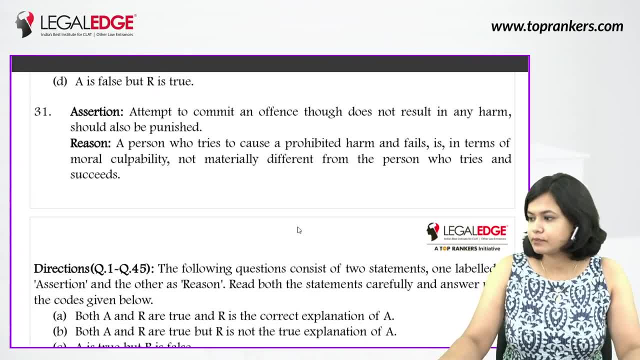 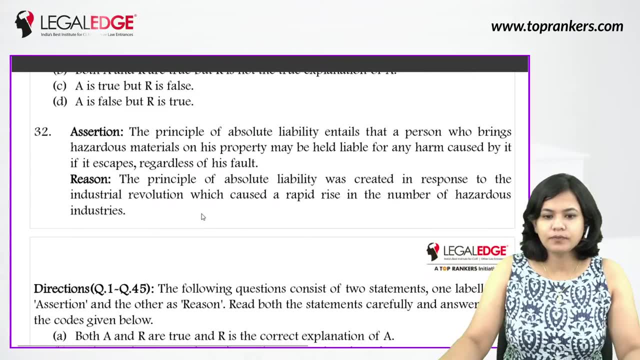 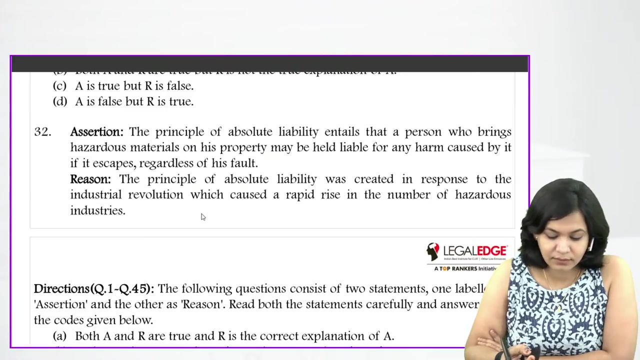 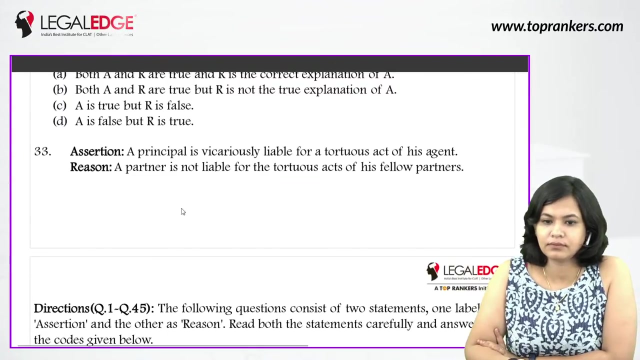 31's answer: Sheetal. I did explain that when the session began, so you can watch the initial parts of the session. 31's answer: Sheetal. I did explain that when the session began. 31's answer: Sheetal. I did explain that when the session began. 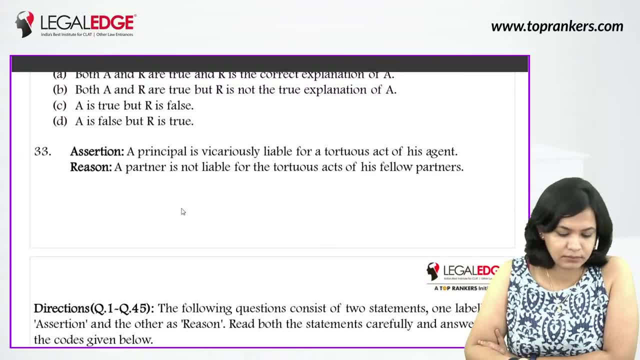 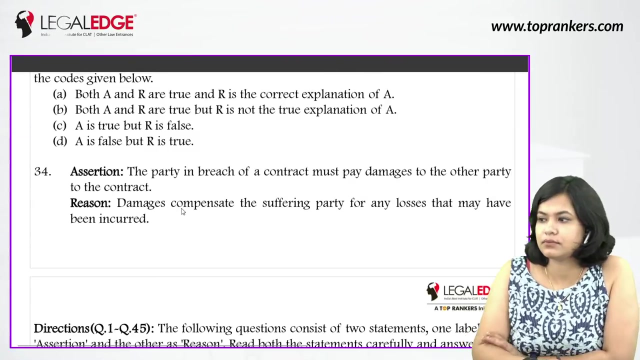 32's answer: Sheetal. I did explain that. when the session began: 32's answer- Sheetal. I did explain that. when the session began: 33's answer- Sheetal. I did explain that. when the session began: 33's answer- Sheetal. I did explain that when the session began. 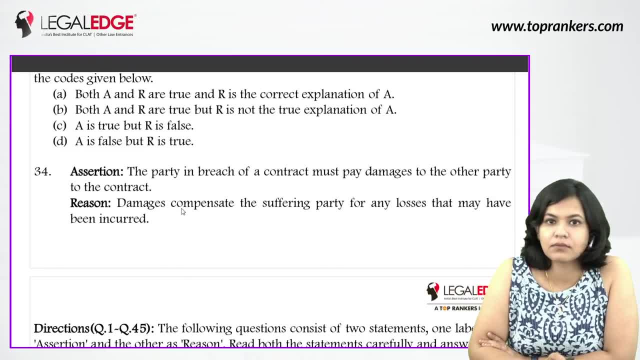 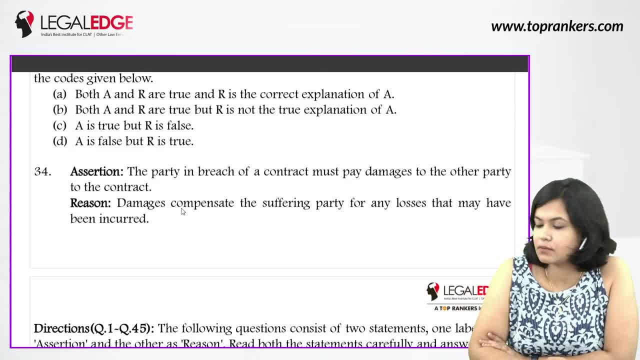 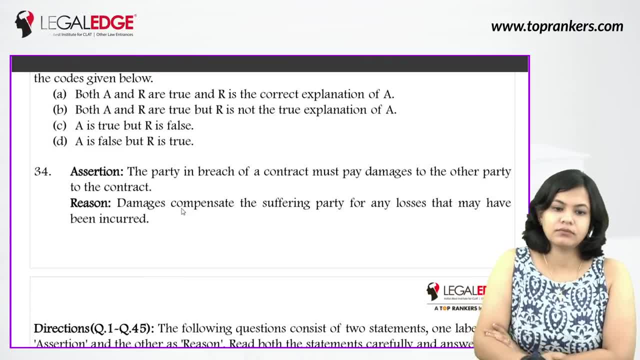 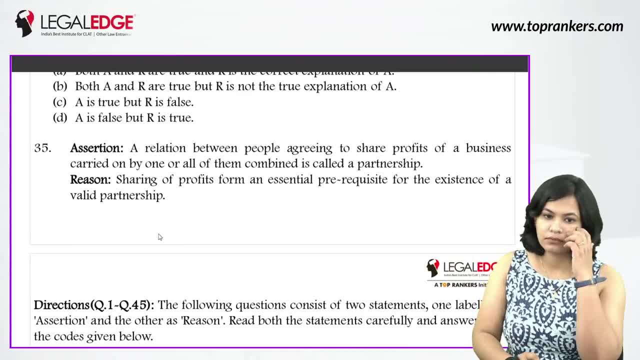 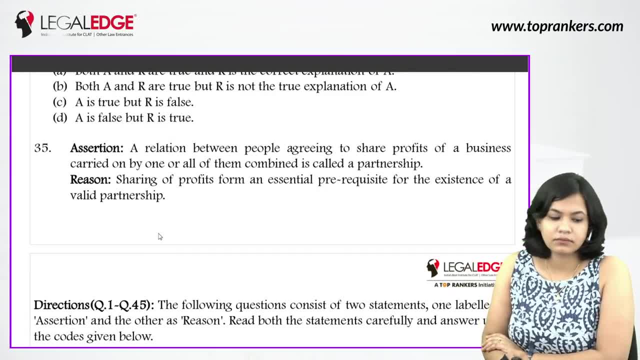 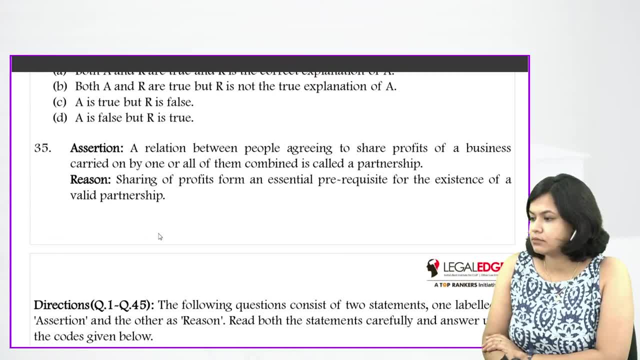 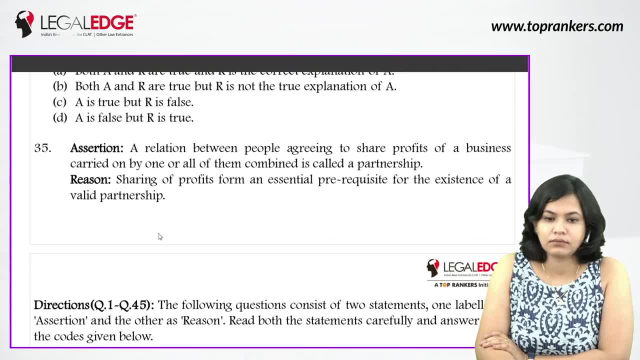 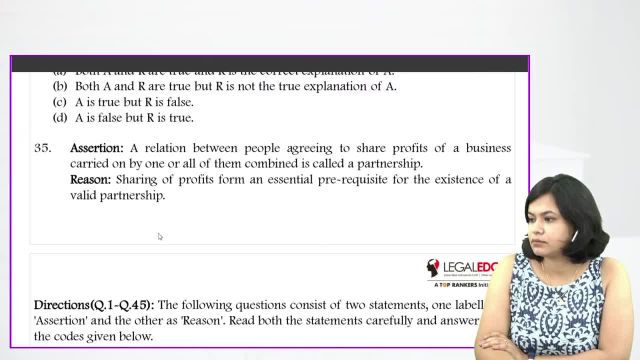 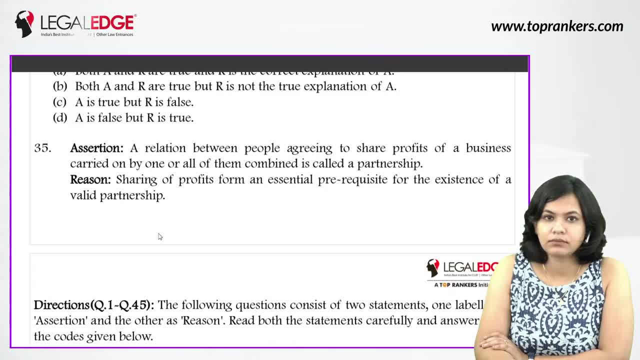 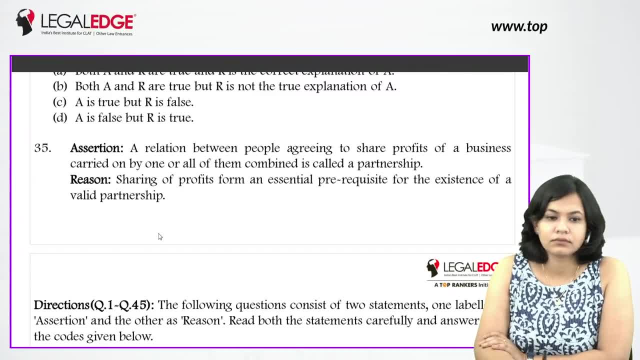 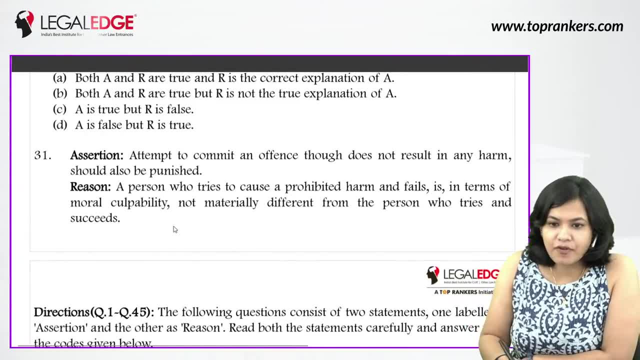 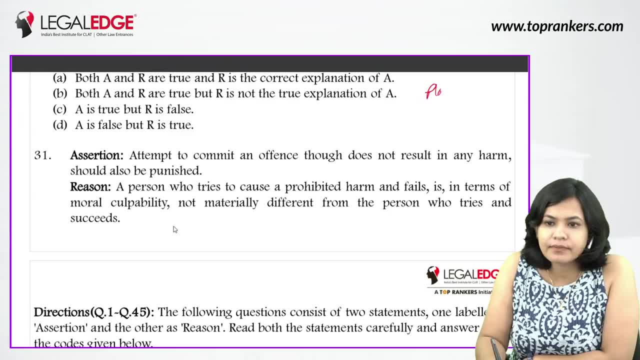 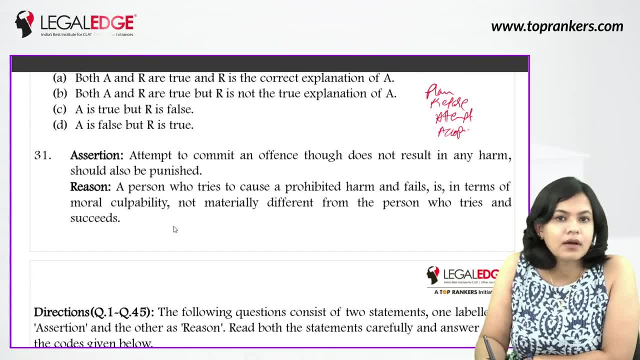 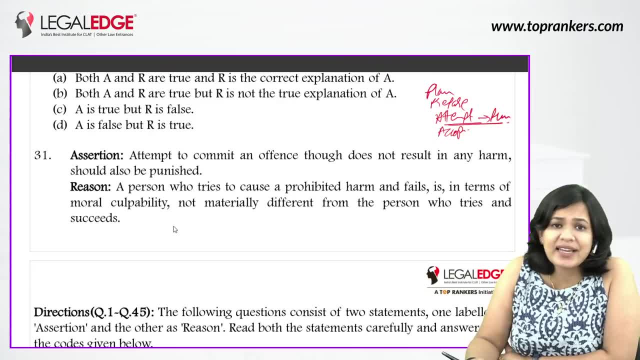 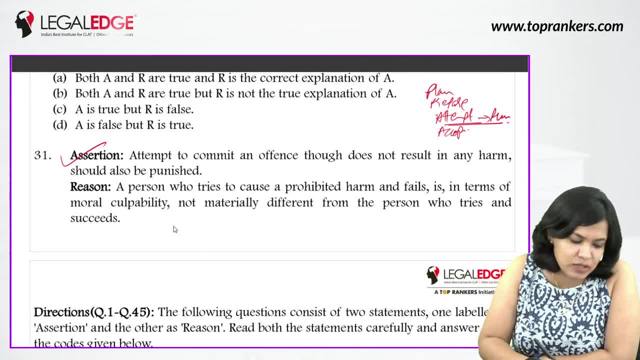 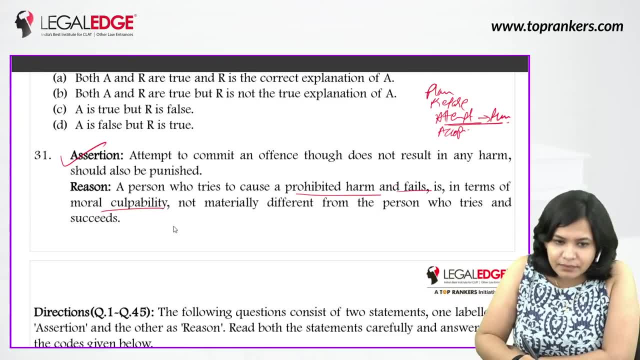 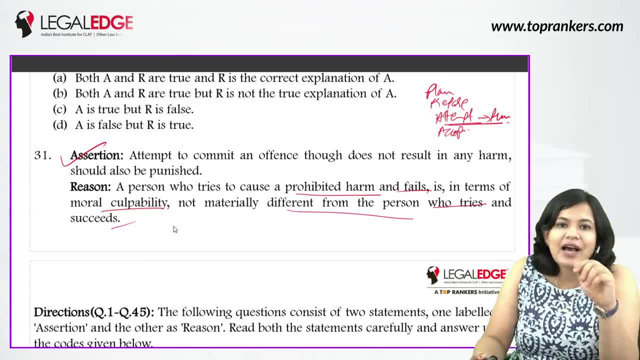 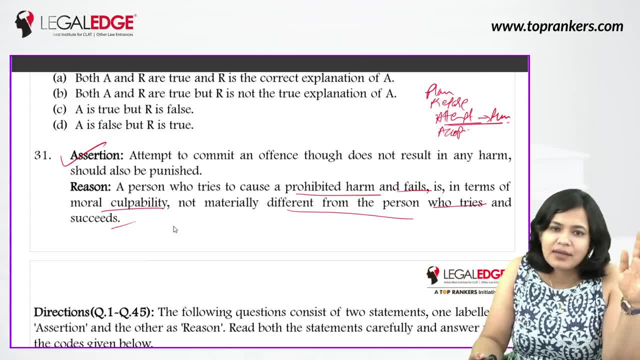 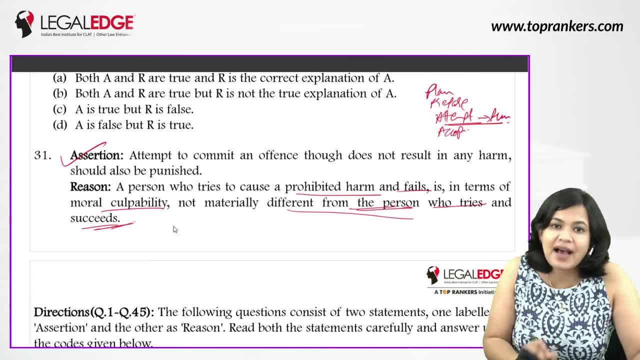 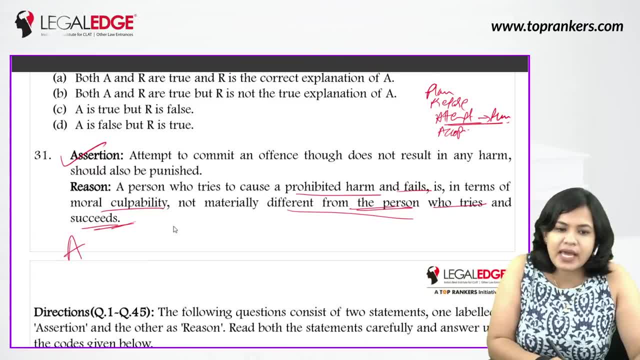 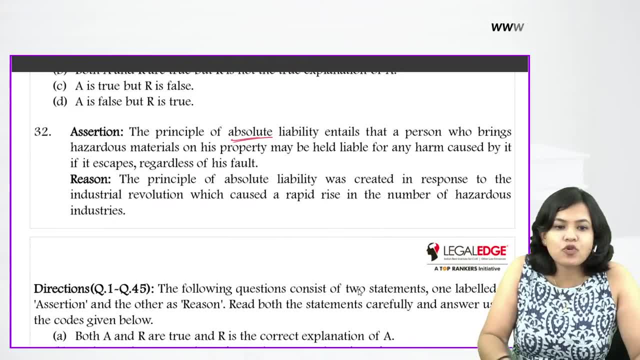 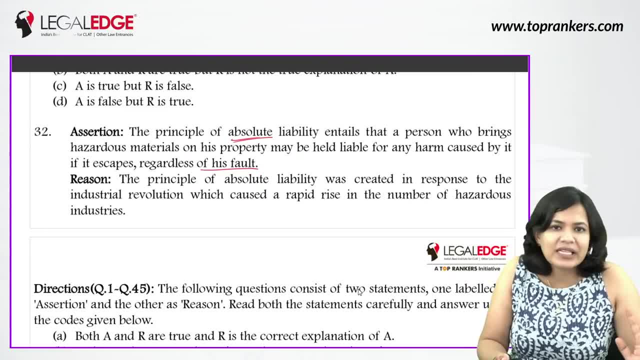 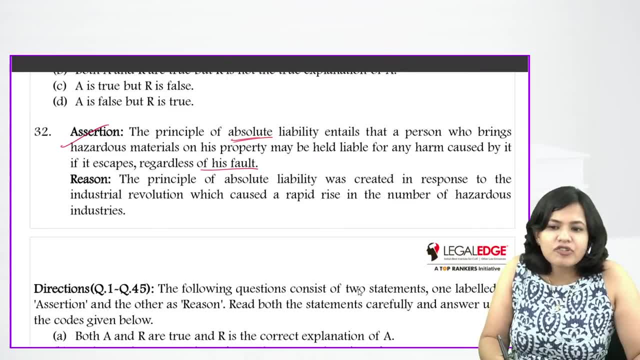 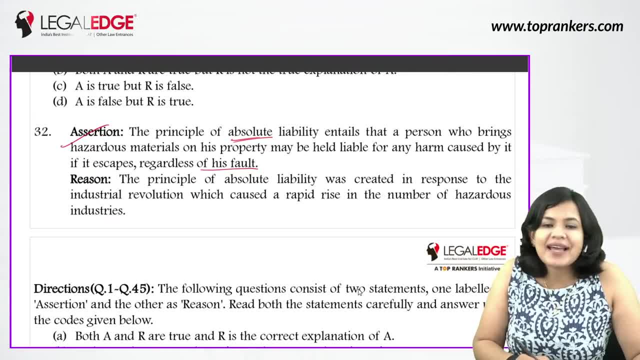 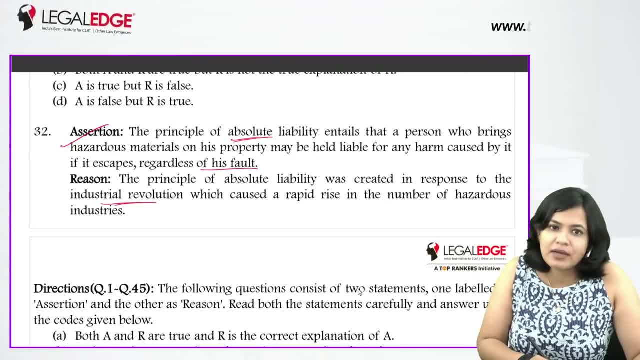 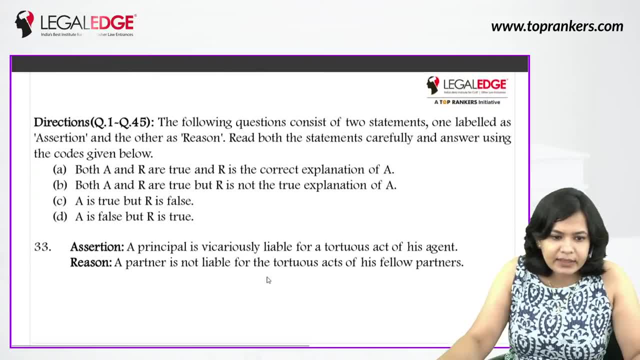 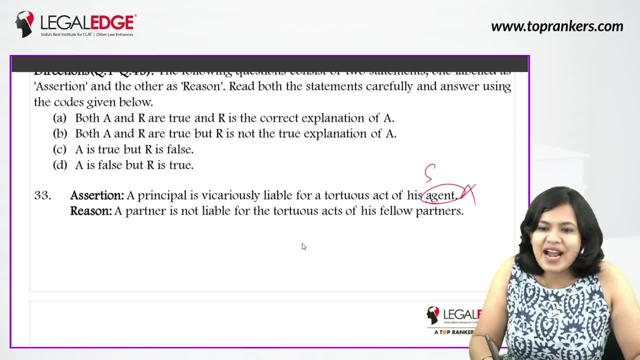 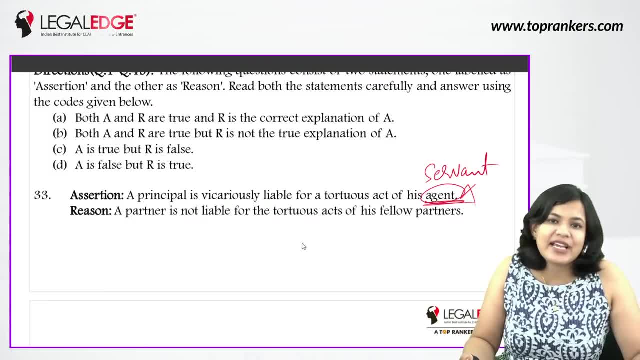 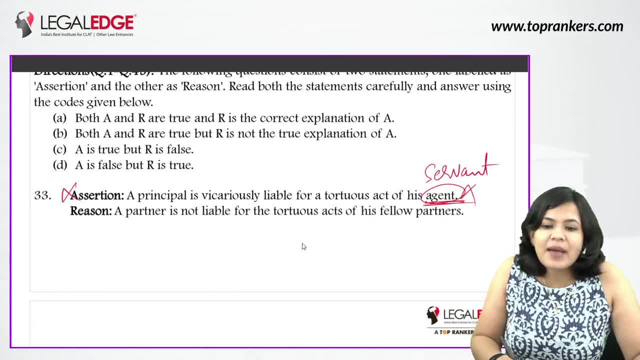 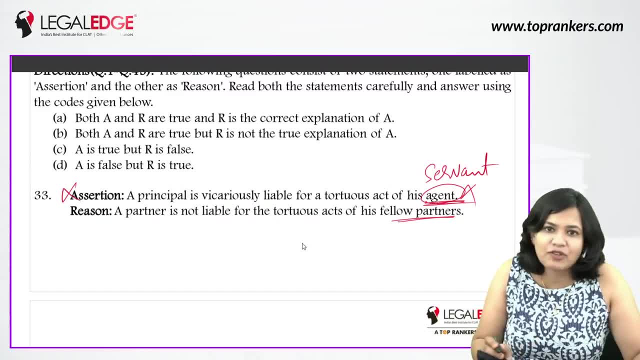 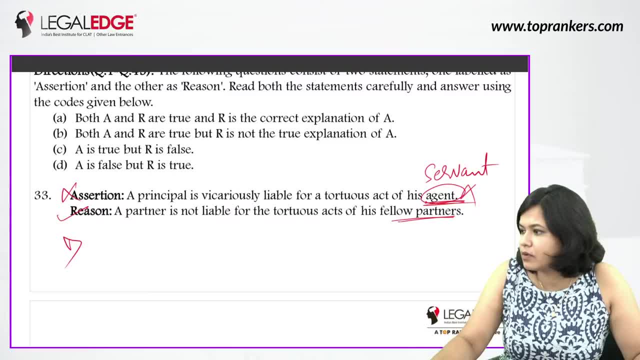 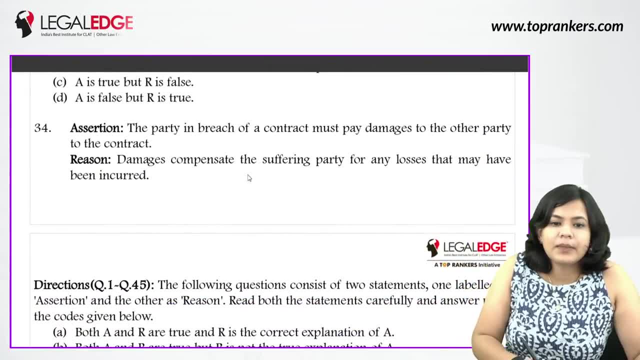 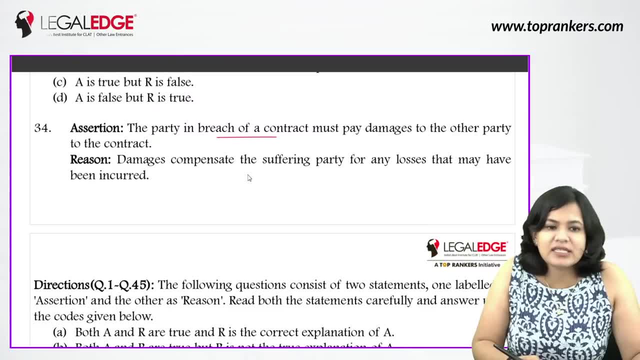 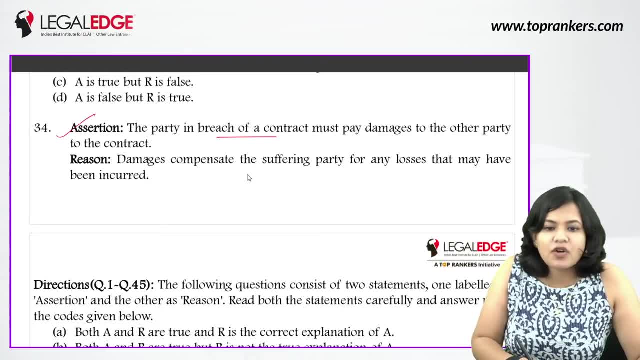 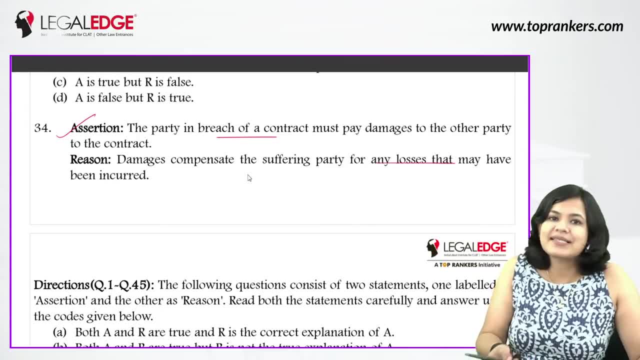 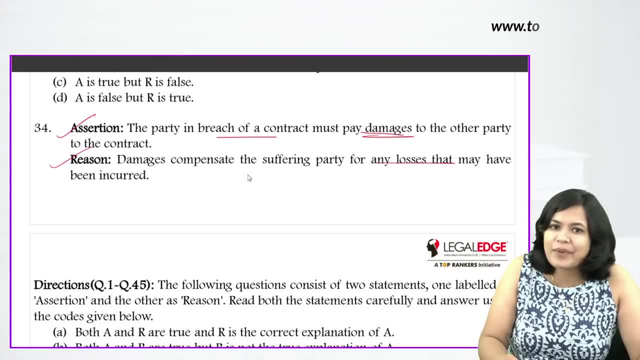 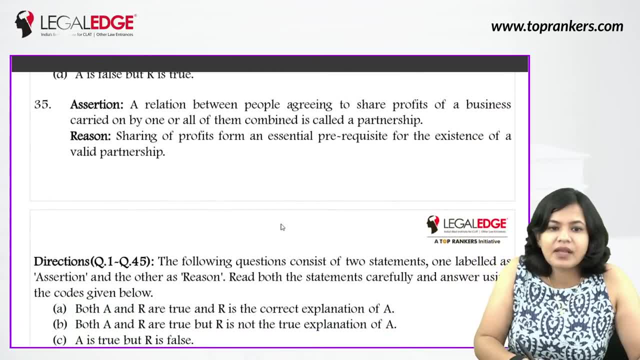 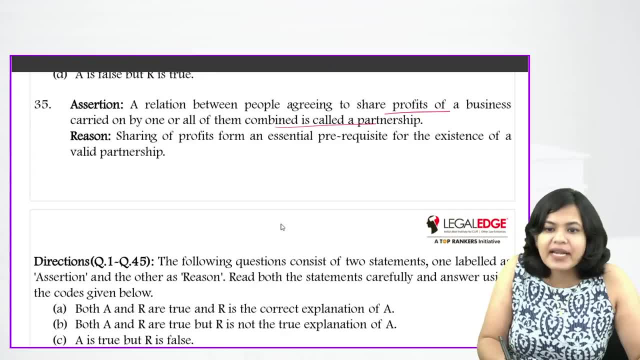 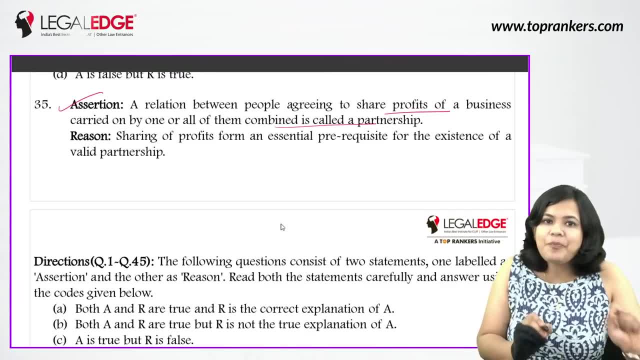 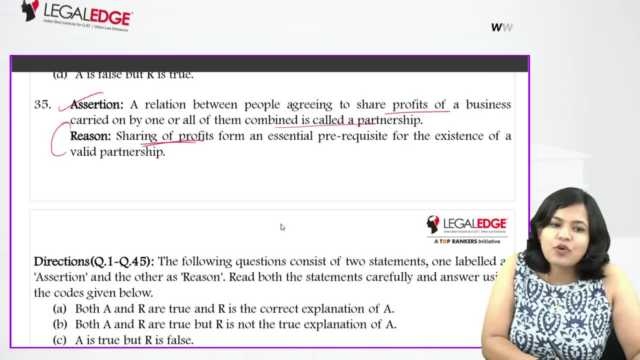 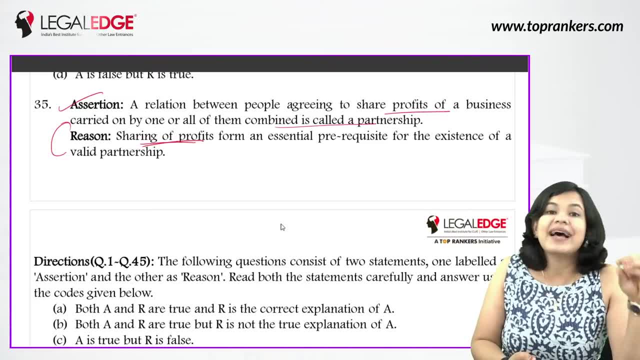 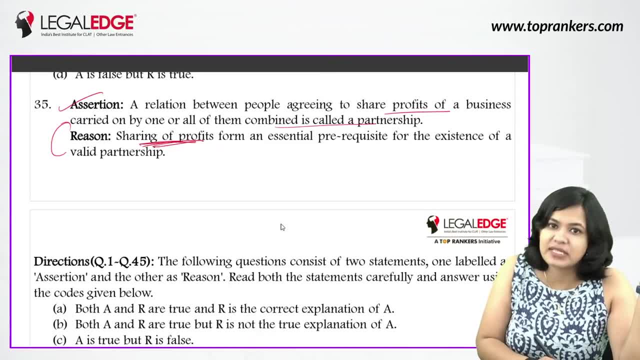 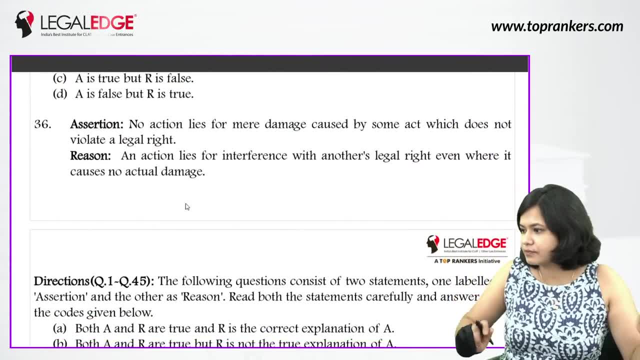 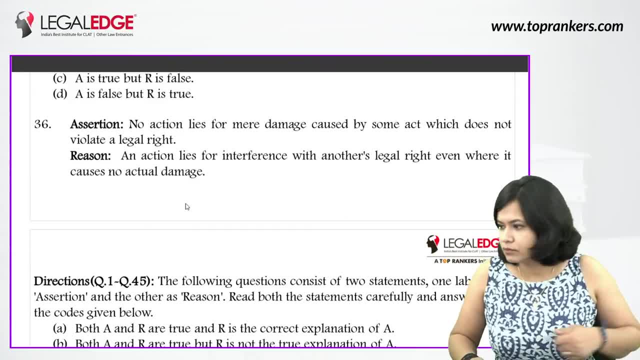 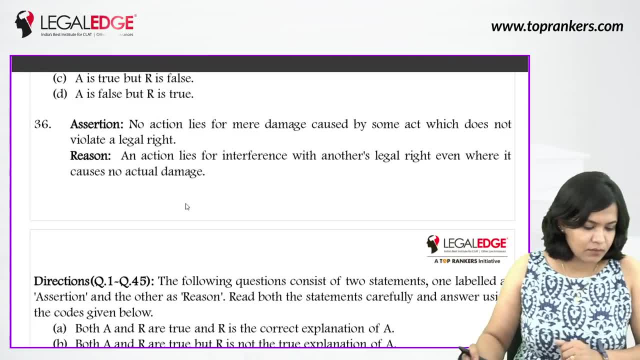 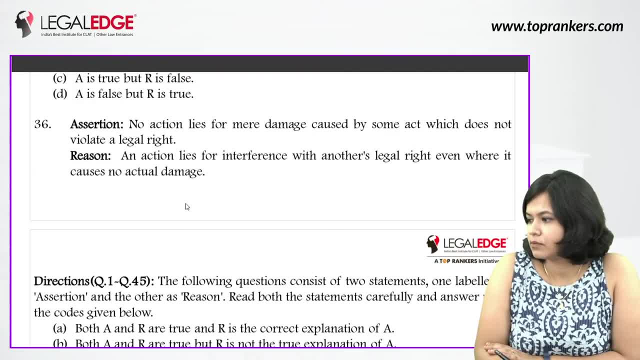 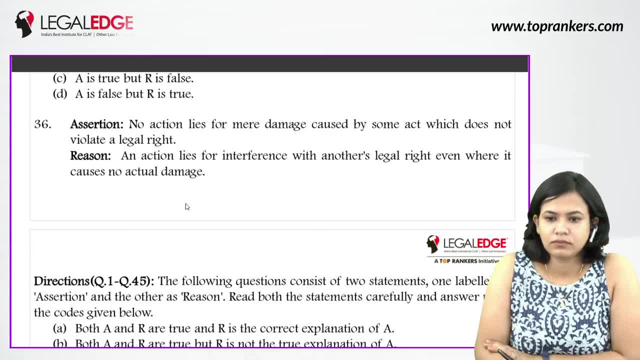 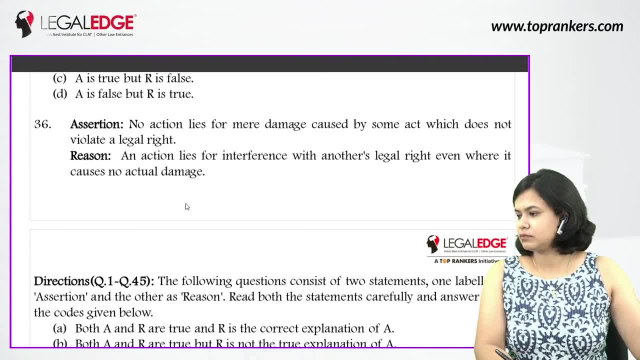 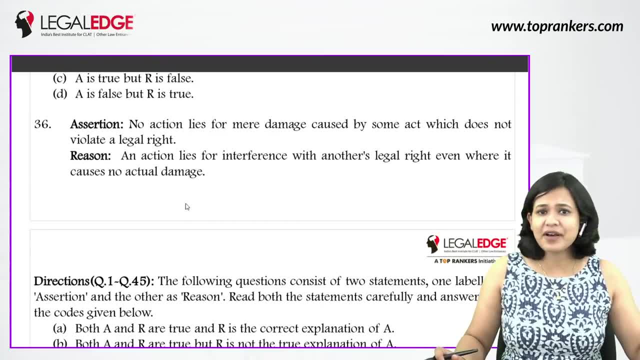 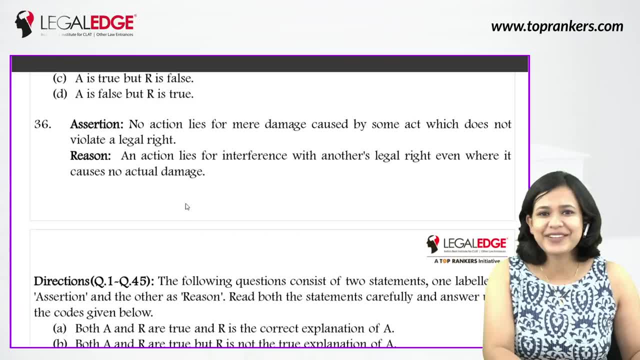 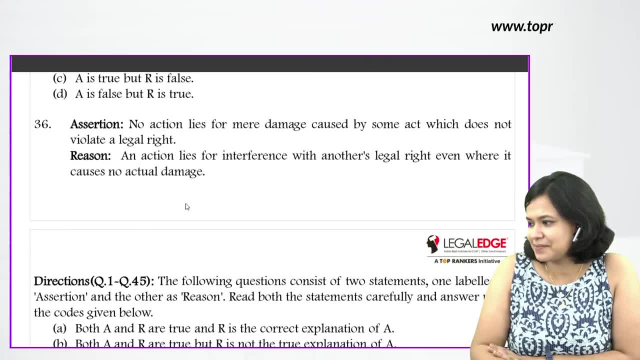 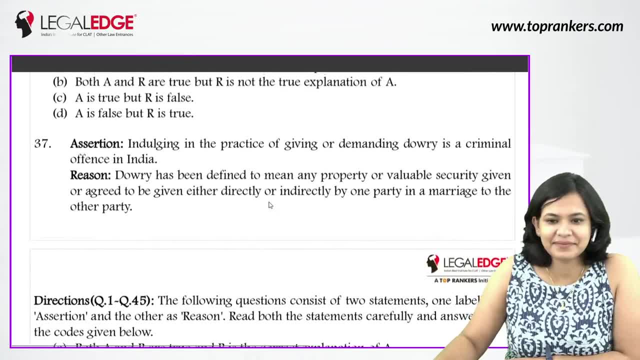 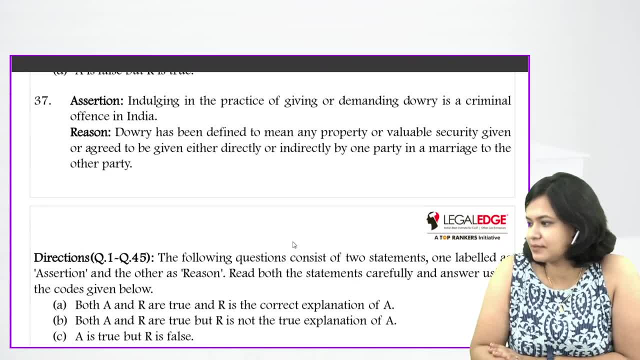 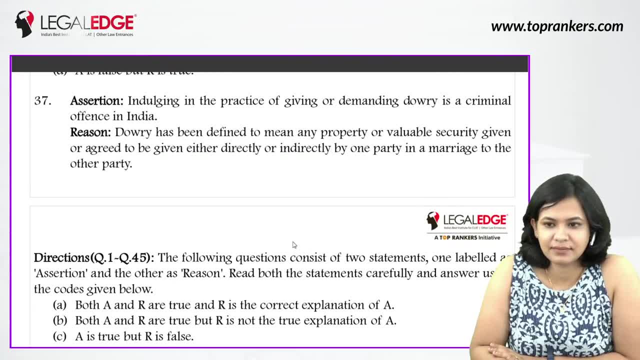 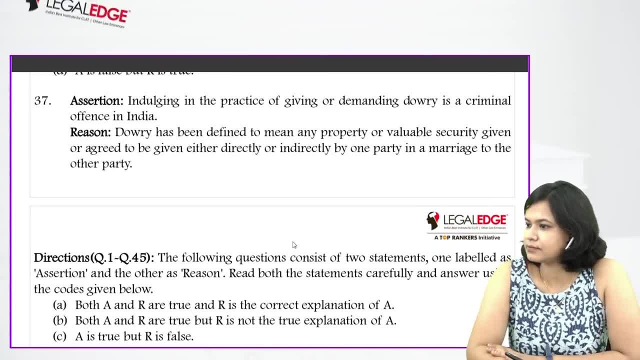 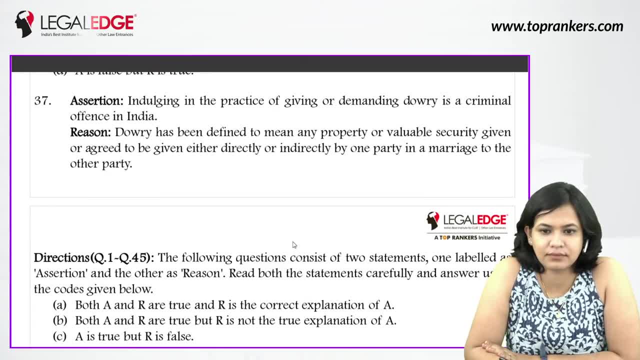 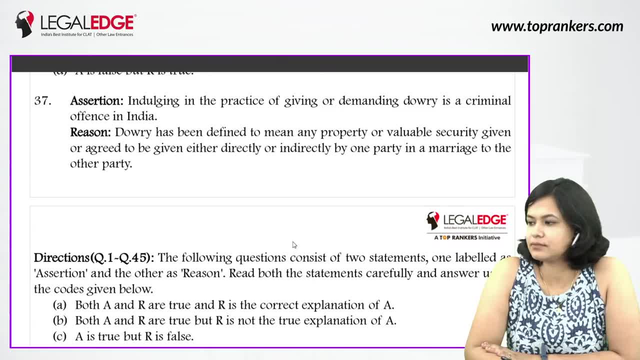 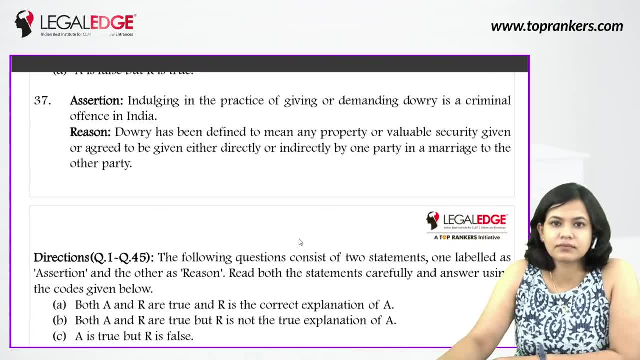 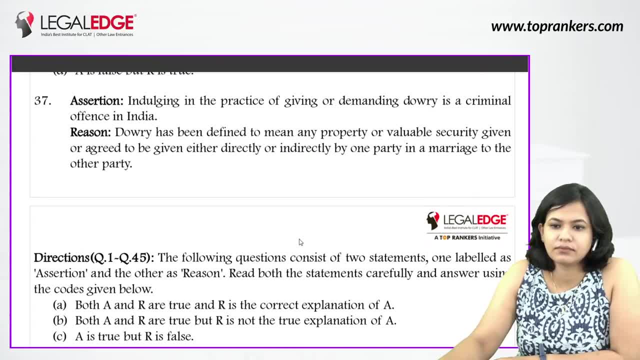 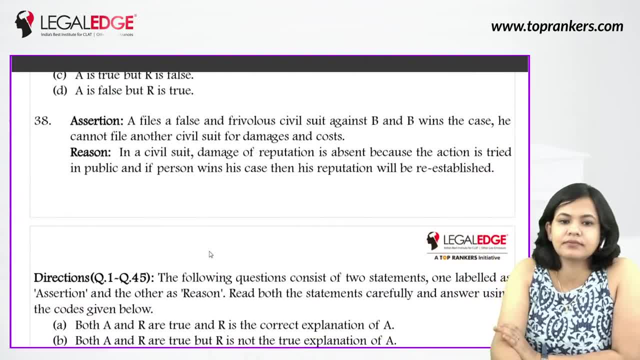 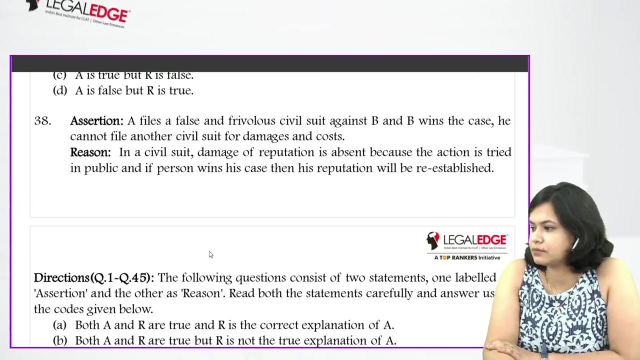 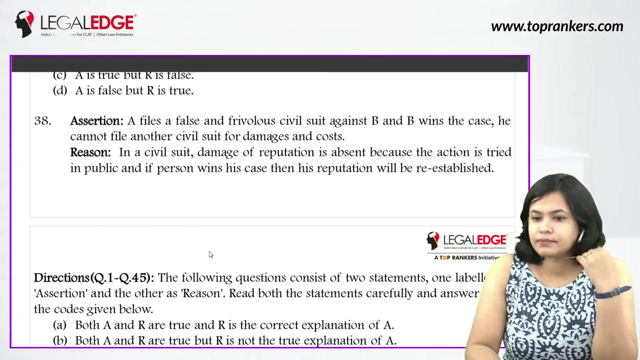 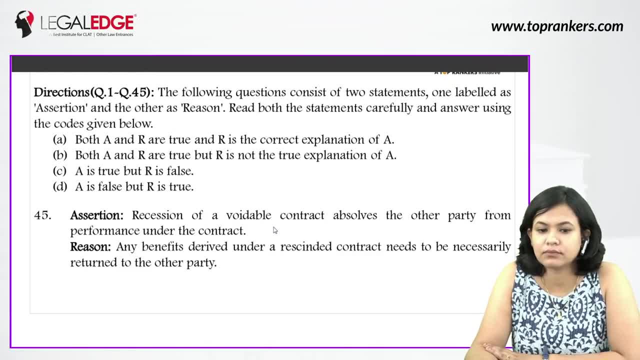 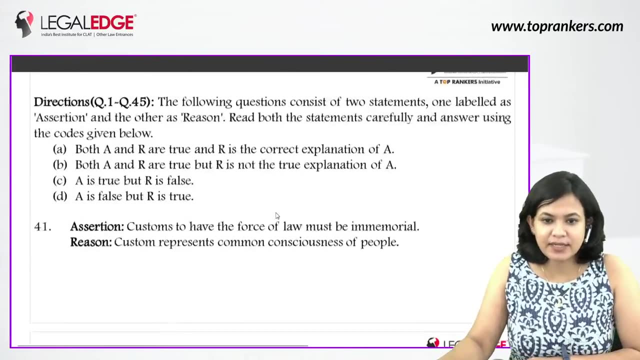 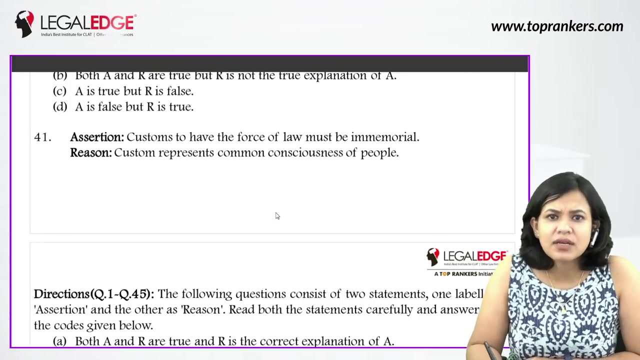 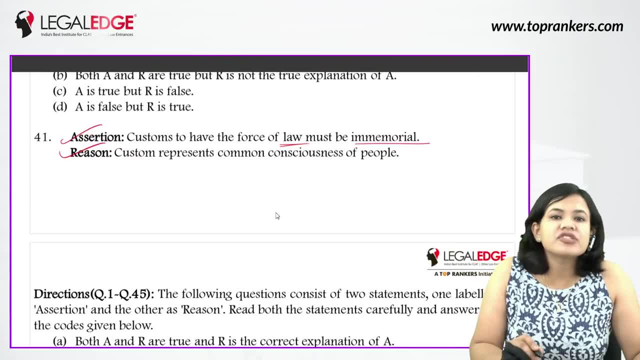 And secondly, it should be an acceptable norm, not just the consciousness, but also acceptable norm. People should have completely accepted it. Plus, it should also be reasonable. There are some customs that are unreasonable, like Satipratha. Do we make it a law or not? 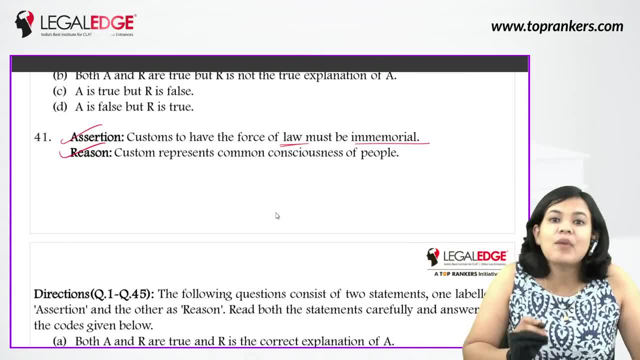 Customs that are reasonable, that are going with the society. we consider them only. So these statements are true, but they are not the reason. So the answer would be B 42.. An exchange of promise between two parties is a bilateral contract. 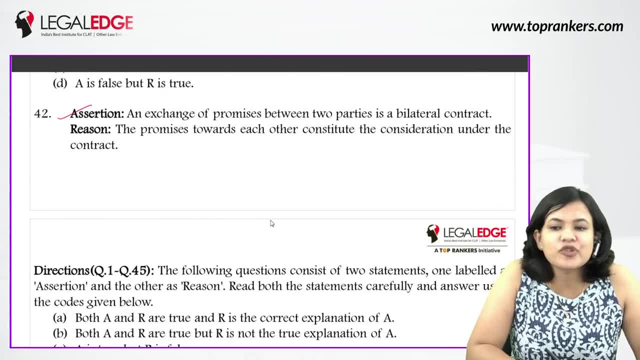 Yes, it is a bilateral contract. The promise to each other constitutes a consideration under the contract. Yes, and that is why it is bilateral. I told Aditi to buy RS Agarwal for me. In return for that, I will give you another book. 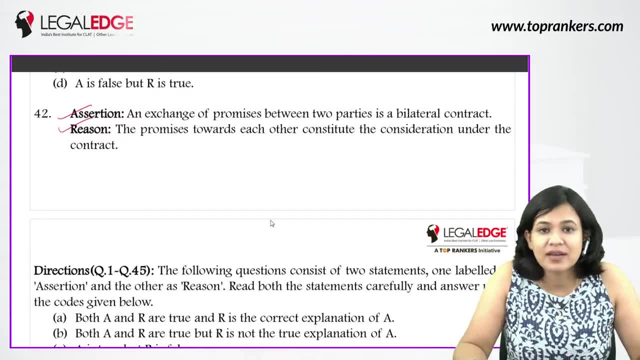 Here we are not giving money to each other, We are just exchanging books. And while we have promised to exchange books, is our promise of exchanging books working as a consideration? Yes, And this is the reason why this entire contract is called bilateral. 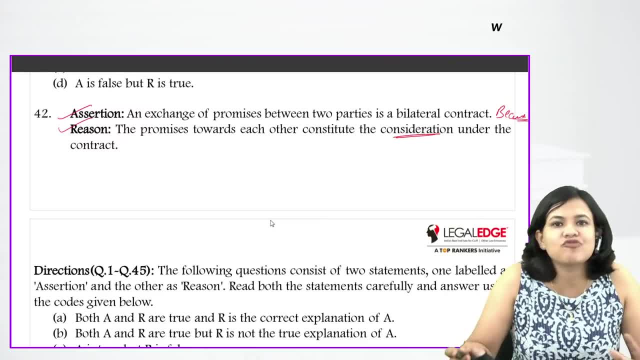 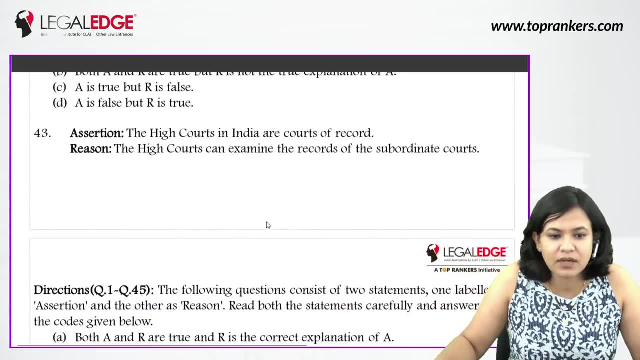 Because no one is giving money from both sides. Both parties are making some promises for each other from both sides. So the answer would be A 43. High Courts in India are the courts of record? Yes, High Courts can examine the records of the subordinate courts. 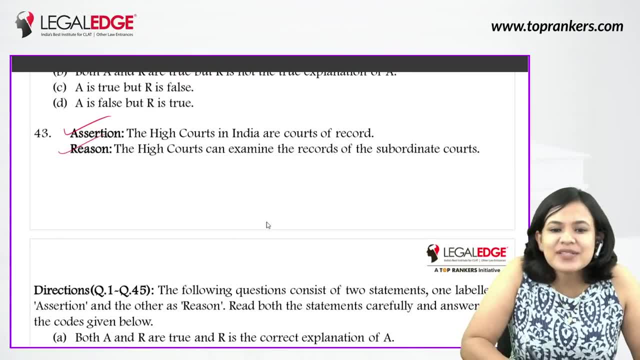 Is this the reason? No High Courts and Supreme Court in India are the Courts of records, Because they can punish for contempt of court. This is a thing that you remember and you will ask whether you are going to get it or not. Contempt of court. 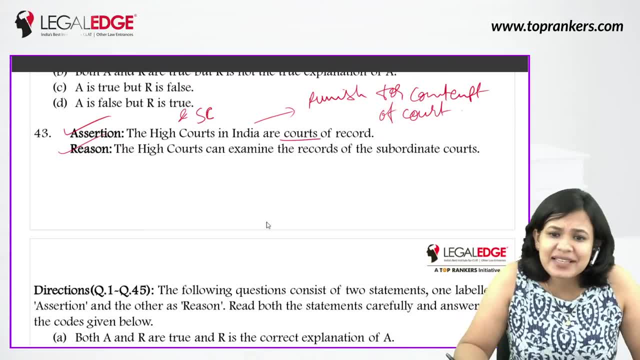 For contempt of court and supreme court punish. that's why they are called court of records, not because they examine the records of subordinate court, district court and sessions court. they examine, but this is not the reason, but because both statements are correct, the answer would be: 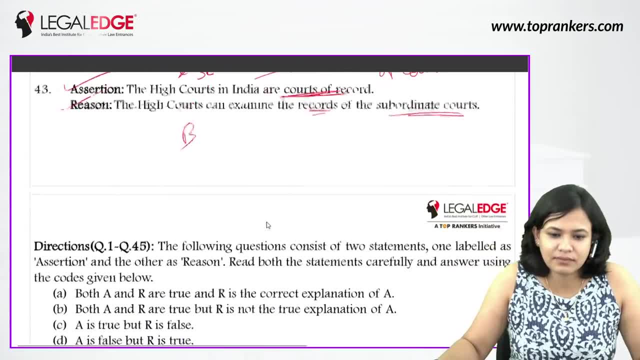 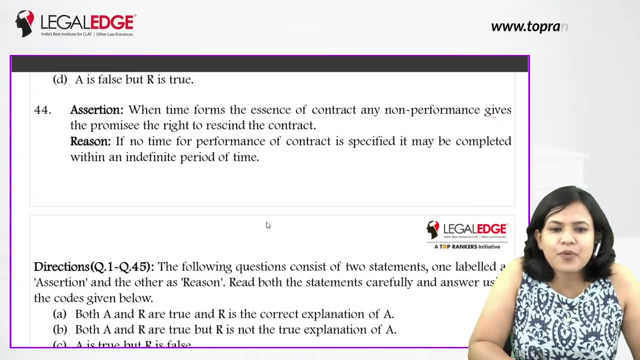 B 44, when time forms the essence of the contract. any non-performance gives the promise C the right to rescind the contract. rescind means cancel it. I told you that in two days delivery is required. if you don't give delivery in two days can I cancel the contract of. 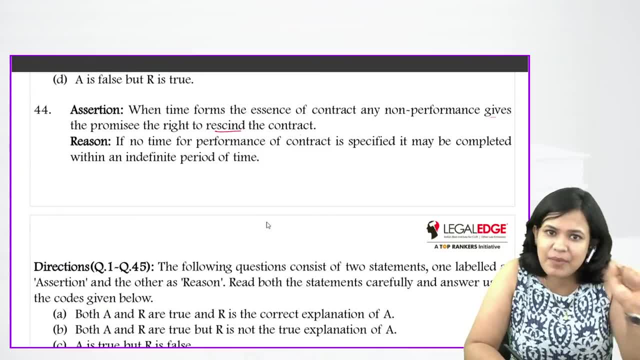 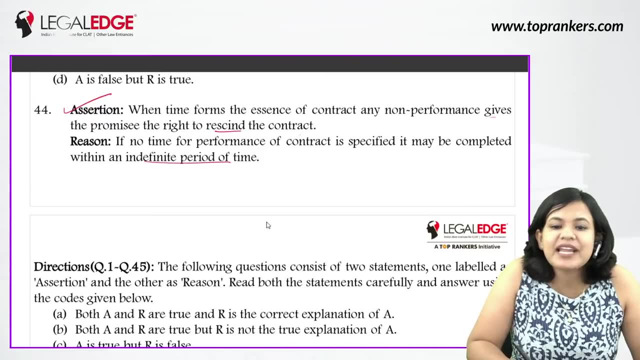 course, because was there time essence in it? was time important? if no time for the performance of the contract is specified, it may be completely within infinite period. no, not infinite, no indefinite period. it is not like I had done a contract that for me, CLAT 2022, give 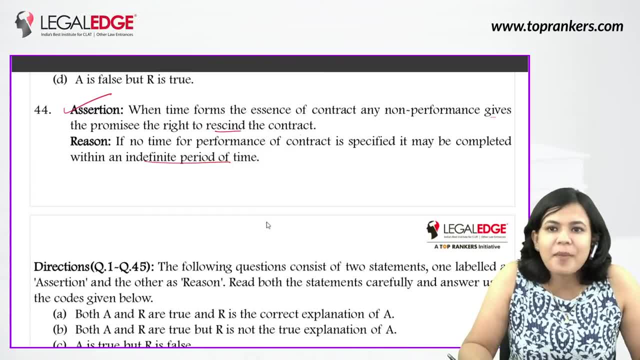 me a particular material. you are giving me material in 2040, then the pattern of CLAT has changed. the exam is completely changed. then the pattern of CLAT has changed, then the order has also become different. such indefinite period is also not there should. 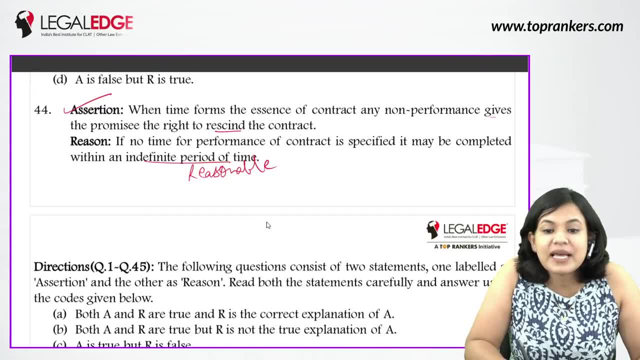 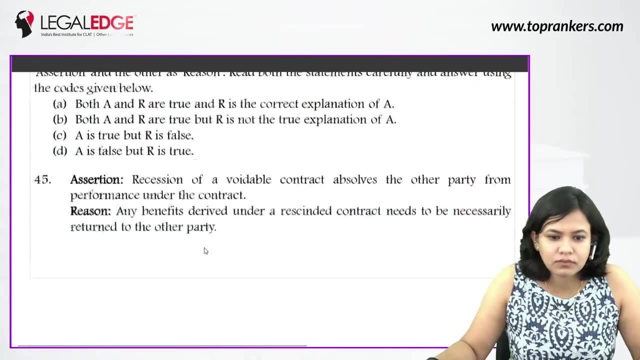 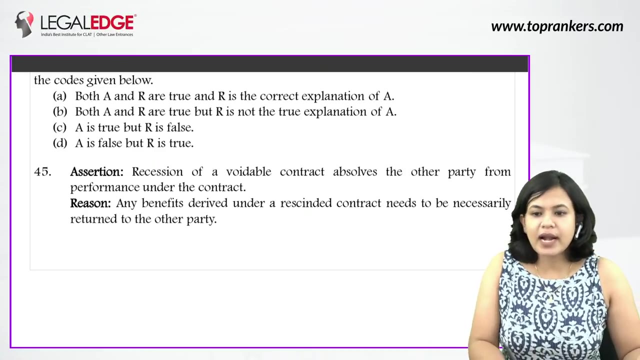 there be a reasonable period? yes, and will that reasonability differ from contract to contract? yes, because this is wrong. the answer would be C. C: the restitution of avoidable contract meaning cancel the avoidable contract absorbs the other party from the performance of the contract. 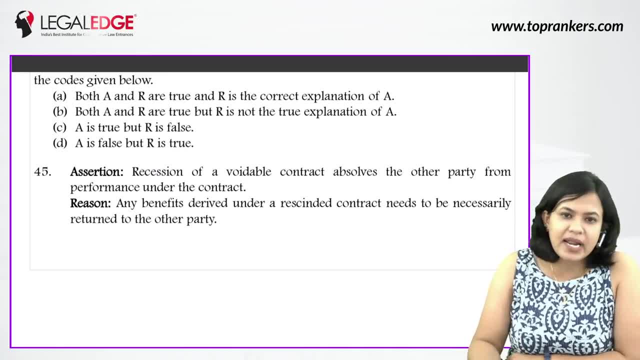 Of course, if you had a valuable contract that you said that no, we don't want to increase it because there was a fraud with me or there was a mistake with me, then the performance of that contract does not need to be done by the other party. 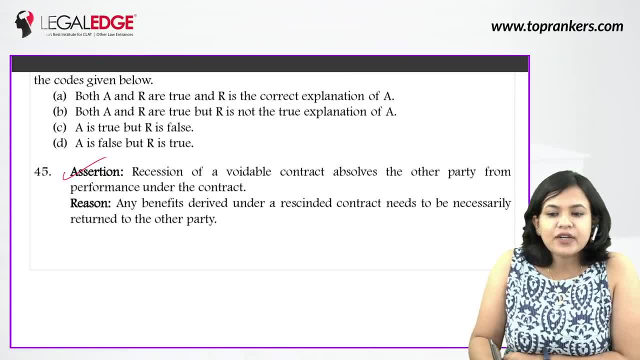 Yes, no, it is correct. Any benefits derived under the resident contract needs to be necessarily returned to the other party. Yes, if I had given some advance and later I came to know that there was a fraud with me, I said no, no, no. I don't want to increase this contract, but the 10,000 rupees that I have given in advance, should I get it back?